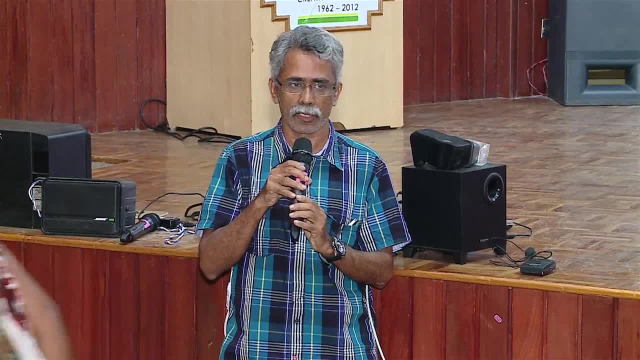 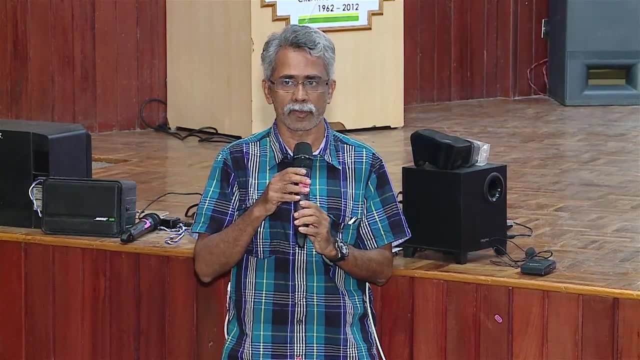 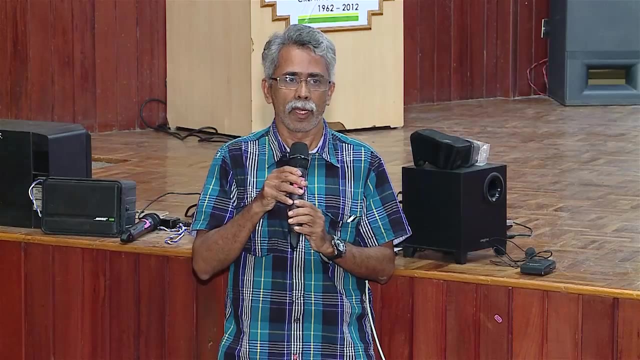 years of teaching experience. You do much, much more teaching than we do. Our idea is to share our insights about mathematical topics, So we have a lot of topics which you would be teaching, You have been teaching, And so that's the main aim, And we like to make it informal, So there is no formal inauguration. 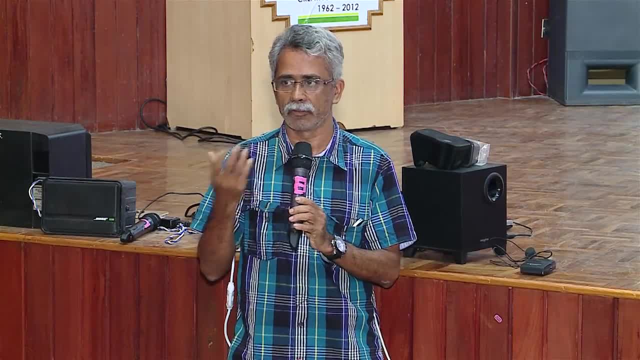 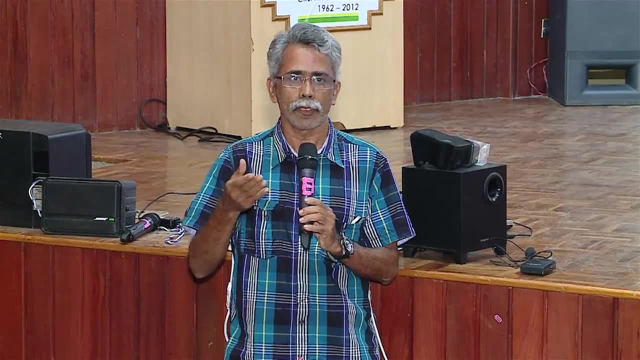 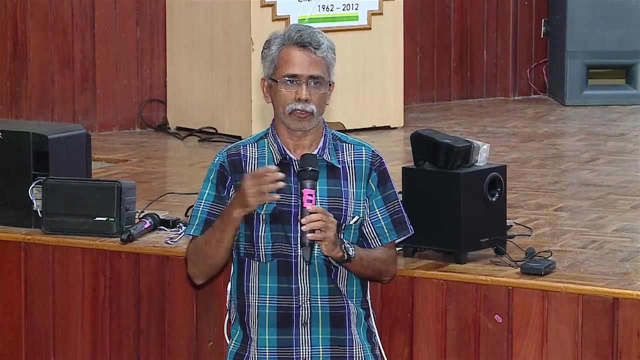 We value your time And so we don't believe in inauguration and so on. So you feel free to interact with faculty members here And also you can talk to each other, And if you have any questions or questions, please feel free to ask. 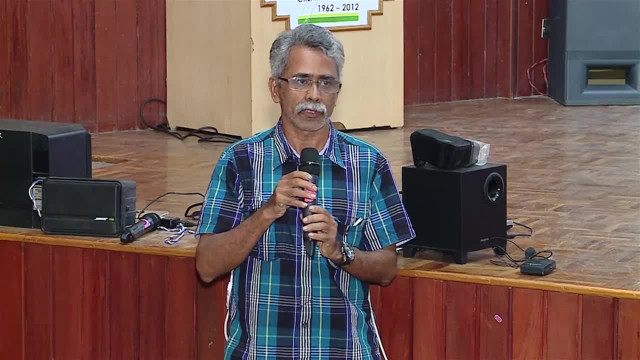 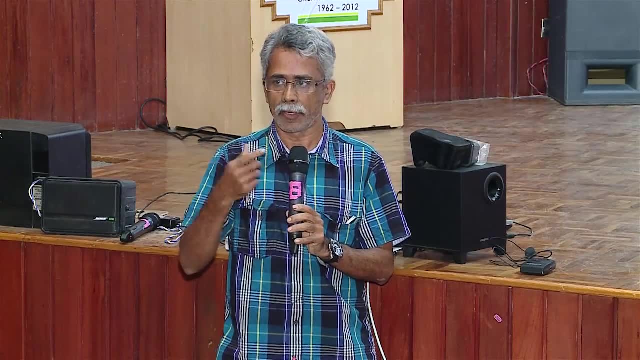 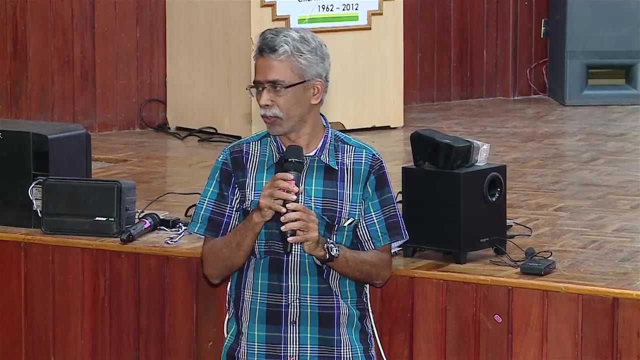 If you have any questions about something, you can ask us. There is also a discussion hour tomorrow in the evening, as was mentioned in the timetable, about our outreach program. There is some write-up in the notebook given to you, at the last page, I was told, So I. 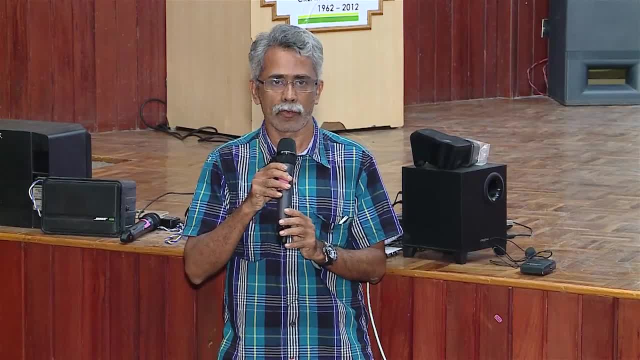 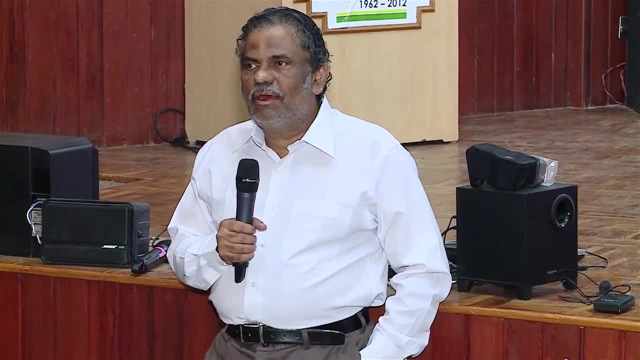 now request our director, Professor Balasubramanian, to say a few words about activities of IMSE. Balasubramanian, Yeah, About this program. Yeah About this program. Of course, Parameswaran has already talked enough- And this institute- 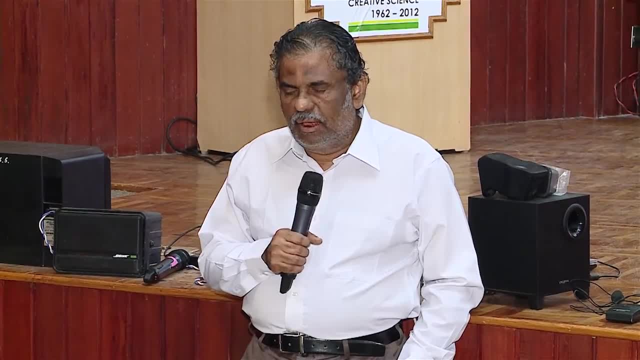 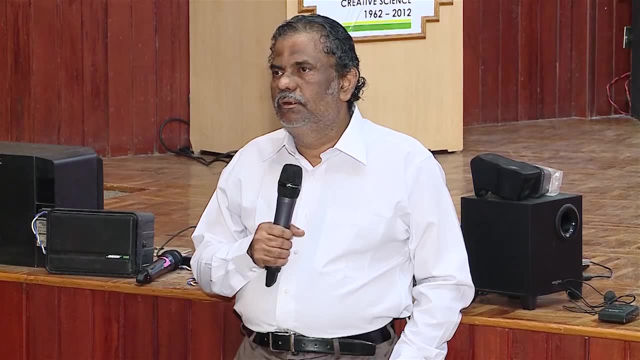 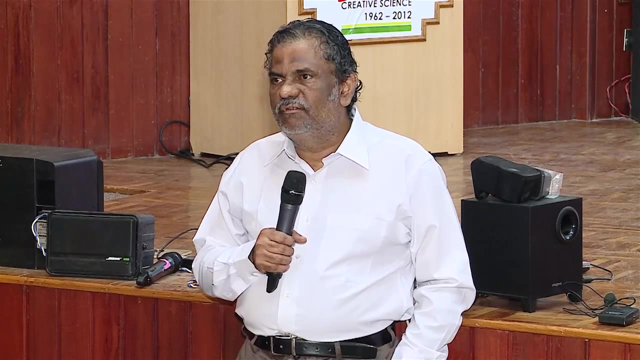 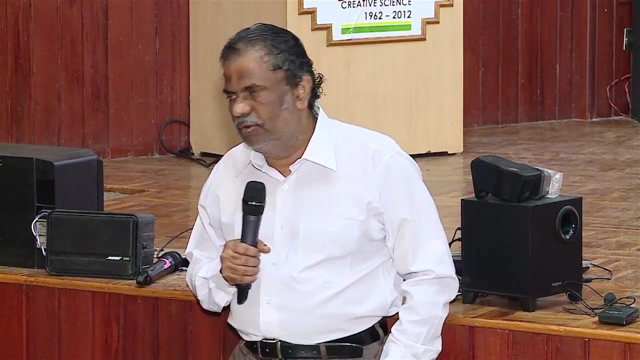 has taken as a responsibility of having good outreach programs and to be able to interact with the mathematics students, mathematics teachers in the high school, college level, within the city to a large extent, And as well as in the national and international level to a certain extent. And this national level, which we do by having some visitors, 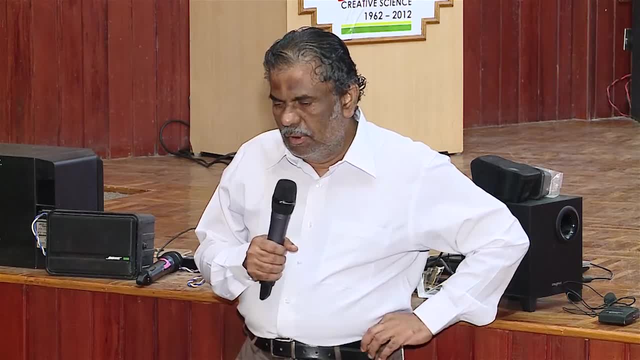 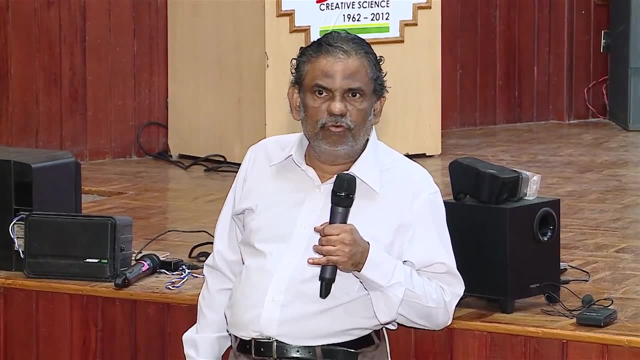 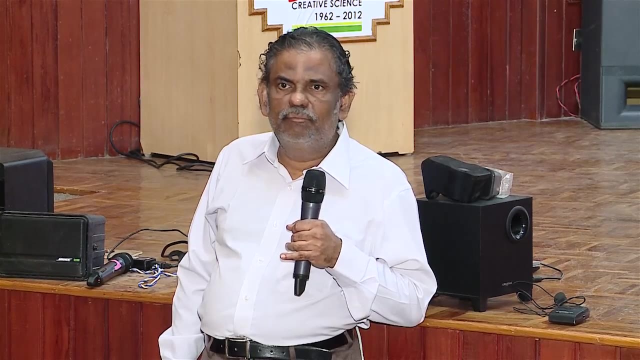 programs, adjunct professors, associates and so on and so forth, And the students also. we have some visiting students who are doing PhD And first of all I should thank the Department of Atomic Energy, which gives us the funding As well as the support of the. 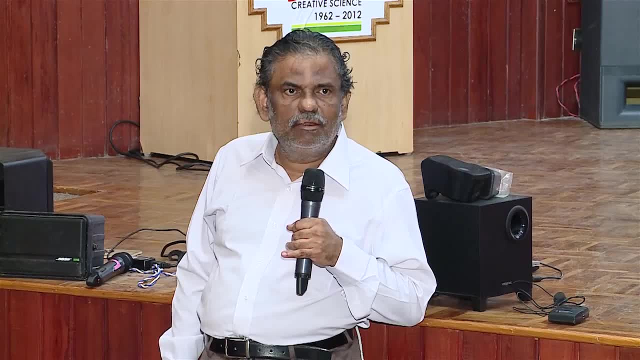 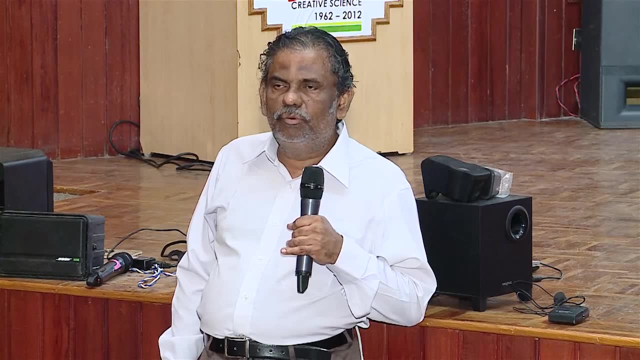 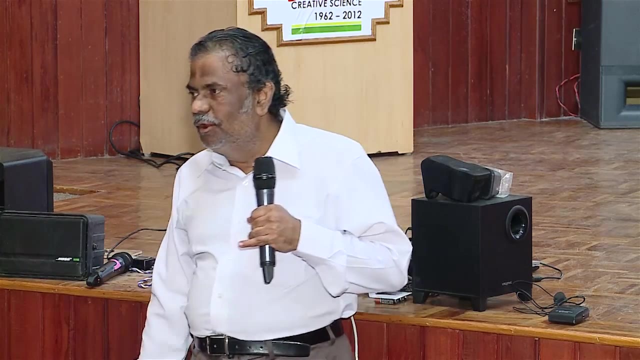 Department of Atomic Energy, as well as encourages to do all this, And, in fact, of the DAE Institute. this particular institute seems to be more well known for its outreach program, mainly due to people like Parameswaran and Raghavan as individuals and probably the Theoretical 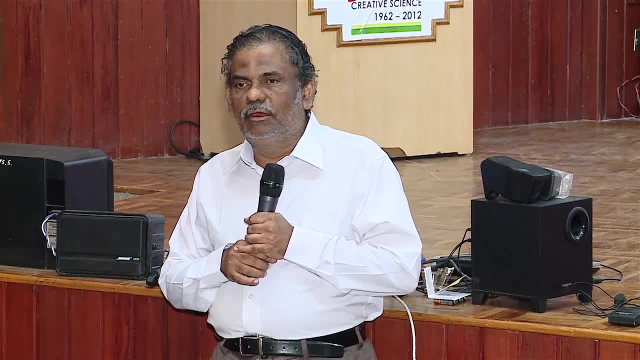 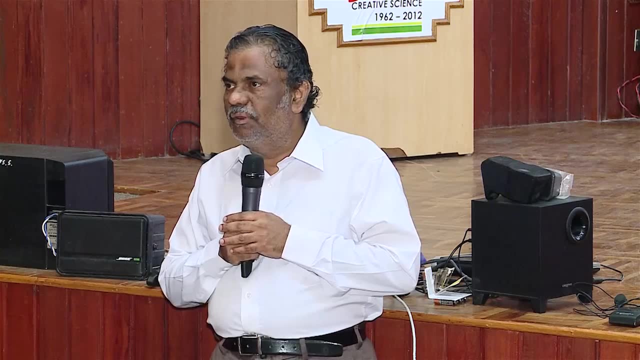 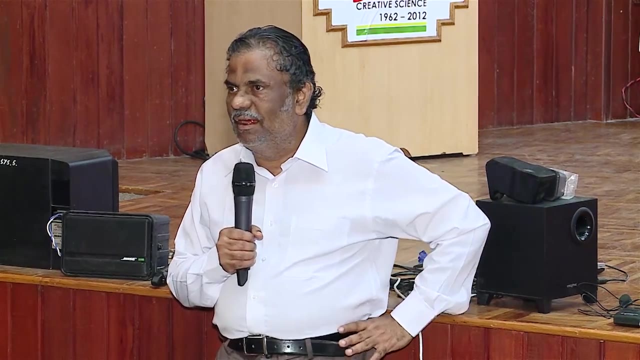 Computer Science as a group, which they are doing a lot of outreach programs, And Parameswaran Shankaran Vishwanath has been instrumental in running such programs every year. last year also they did it And I should really thank them, express my appreciation. 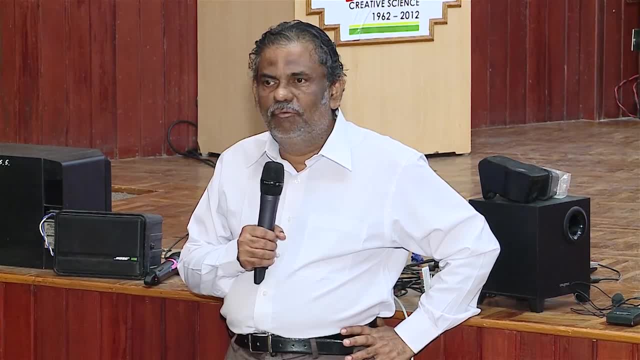 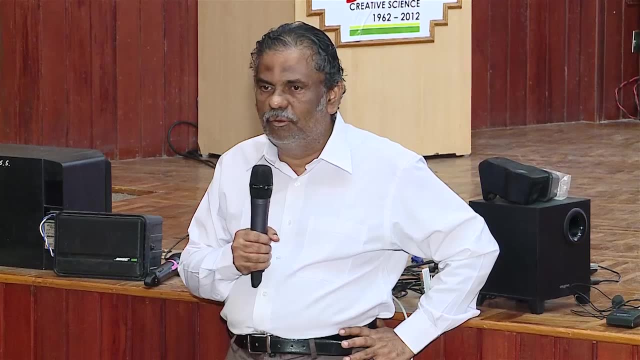 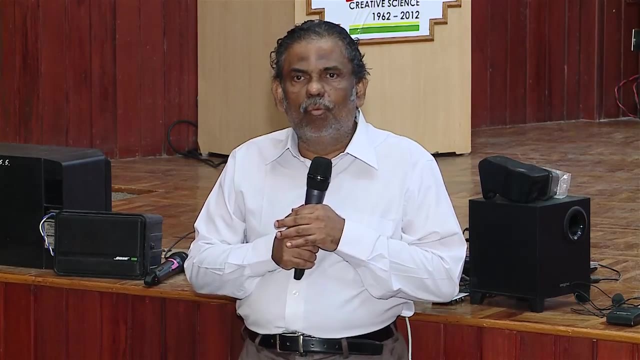 for them, And also I should appreciate those who have offered to give lectures here, including Meena and Vishwanath and Srinivas and Annirban, who will be giving lectures on this And exactly has permission and said that we are all open anytime you want. you can sort of 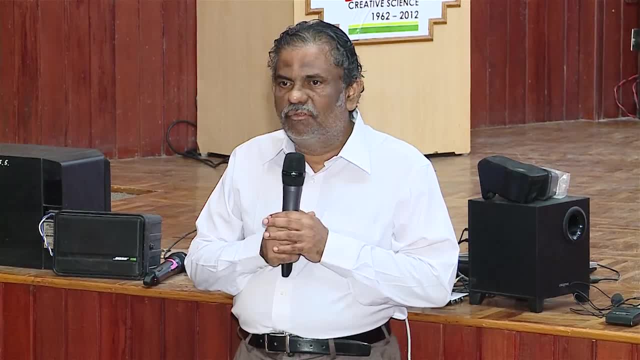 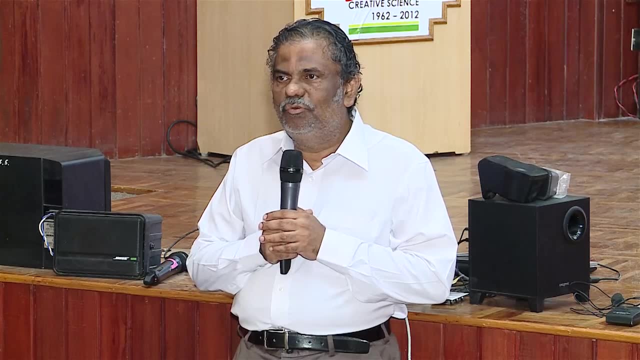 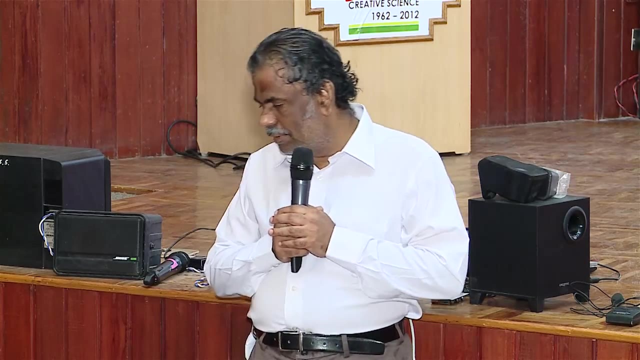 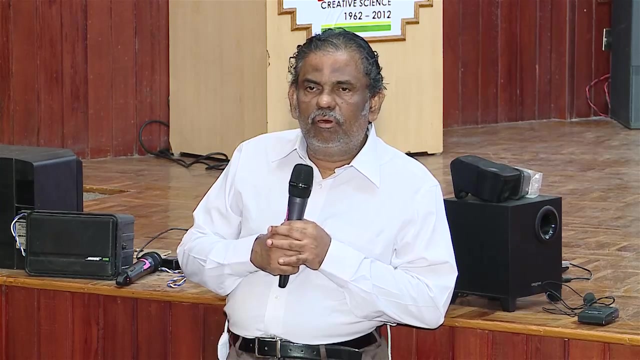 discuss any of your problems with any of the faculty members here, and we have a library and I do not really know how useful this library would be for you. it may be of a slightly highly advanced level, but, however, let me say one more thing which is very important: that for mathematically inclined students, this is: 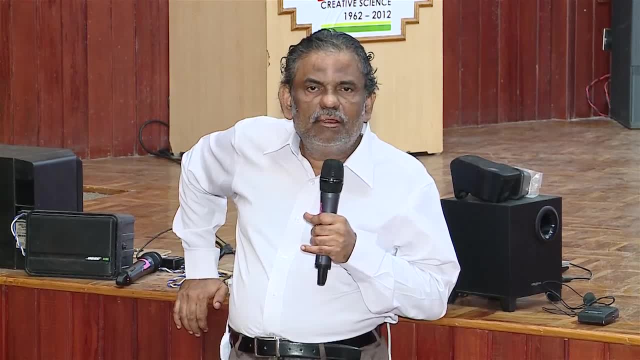 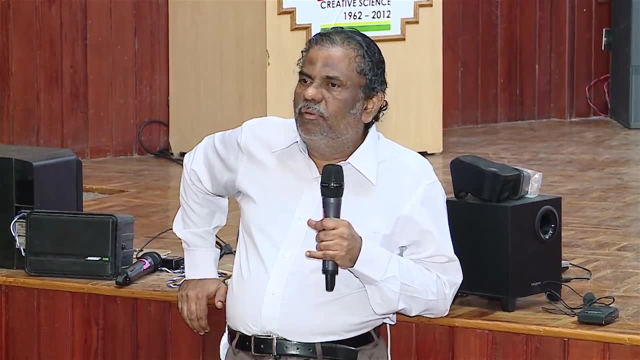 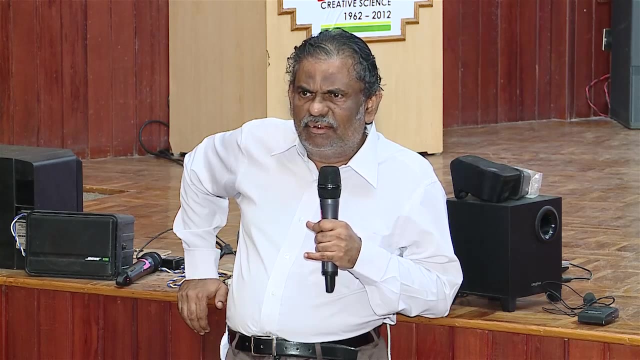 true only for mathematics, but even for physics, chemistry, etc. there are something called Olympiad programs. okay, these Olympiad programs first of all takes place in the national, in the regional level, and then all those 30 people are selected- in the regional level, I assume- and then all those. 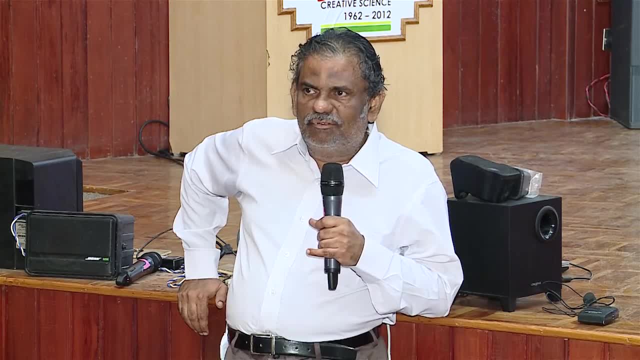 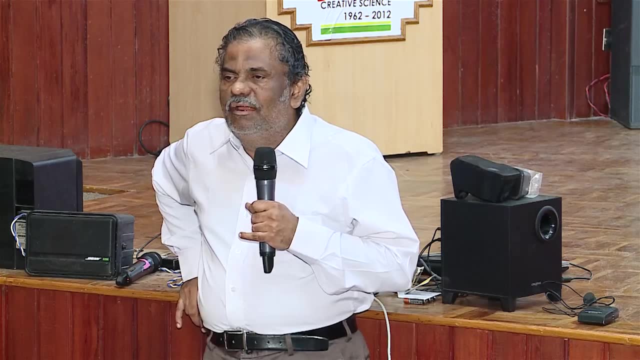 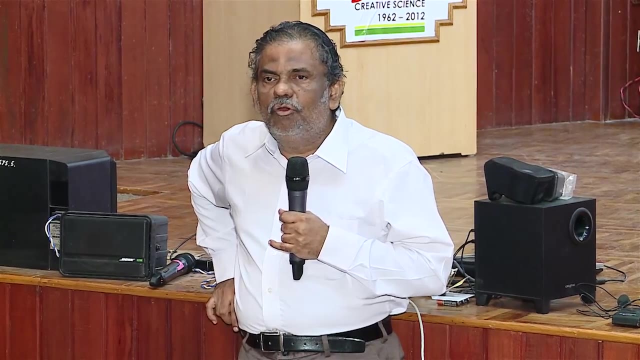 competent national level and out of which 30 are selected, and then out of this 30, then again another training is given and six are selected, and six goes to the so called the International mathematical Olympia. and the same thing is true, of course, the physics, chemistry and so on, so forth. but the fact is that those 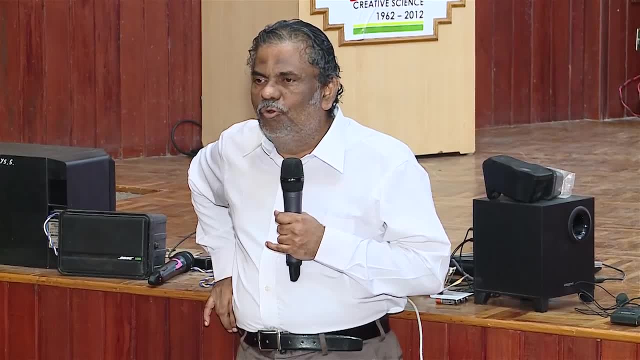 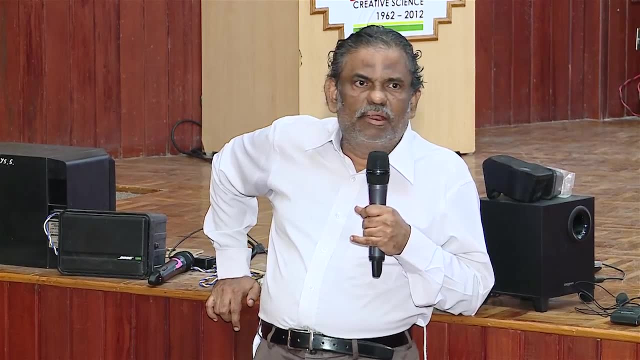 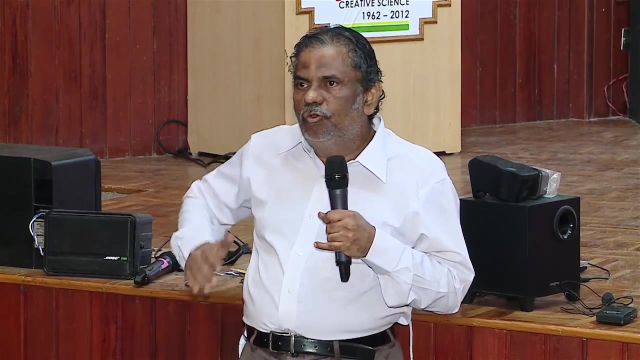 things are done by different group of people whom I really have no idea about, but, on the other hand, the mathematics is being done by something called the national board for higher mathematics, with which I am associated, and therefore I would probably include show all of you to know a little more. 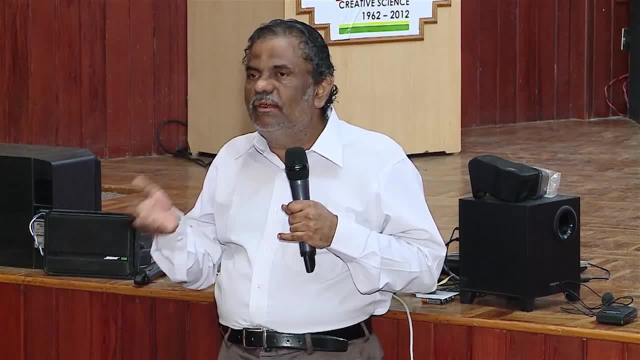 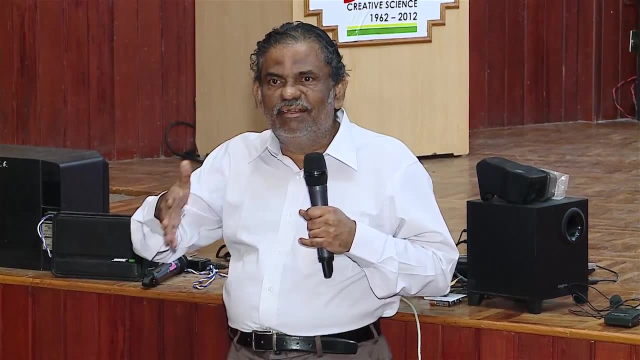 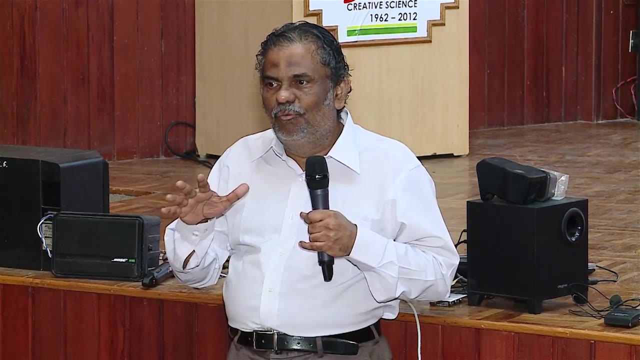 than your syllabus. okay, particularly things which are what one we call as the discrete mathematics and number theory and a certain geometry, because that is the only subjects in which a person in the plus-two level can be actually tested. what? and therefore the whole program would be essentially in those areas, only the discrete mathematics, number theory and some. 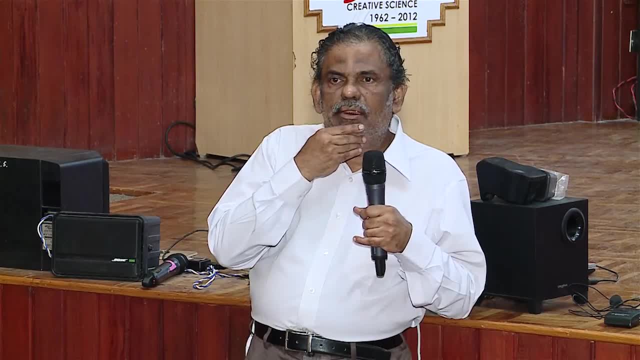 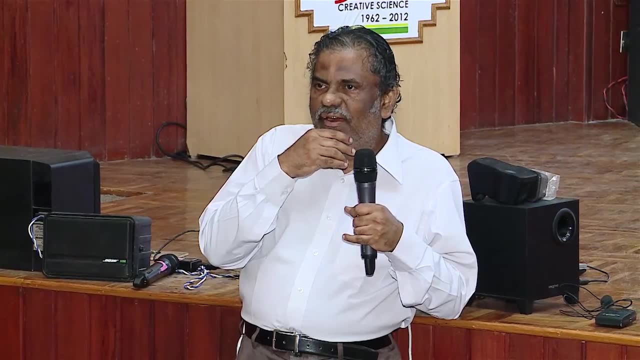 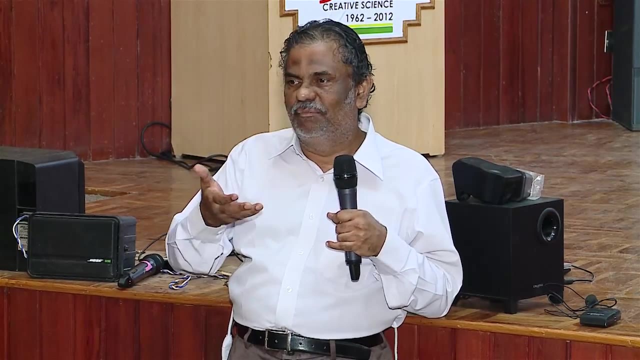 geometry, equivalent geometry, and if you can train your students, then you see, if you do in initial training and if they qualify, then the later for the later purposes, of course we have enough resource people to train them first of all when they cross the first stage, then we have a big 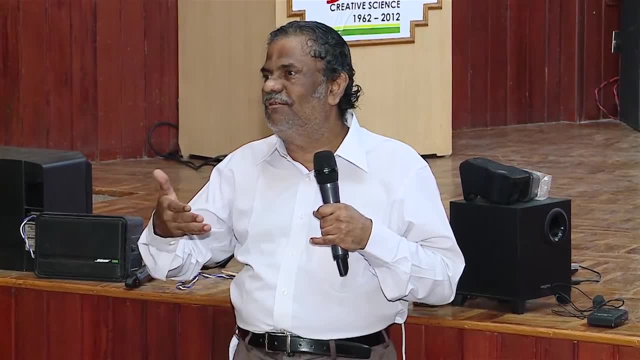 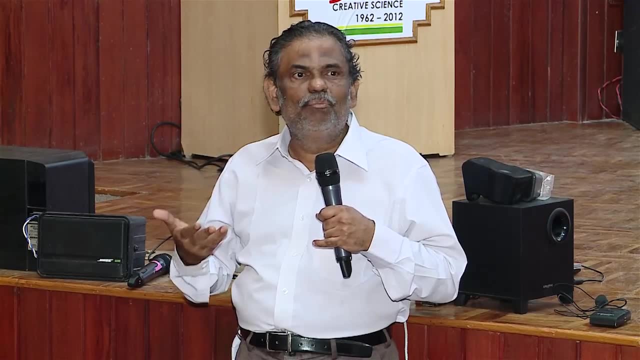 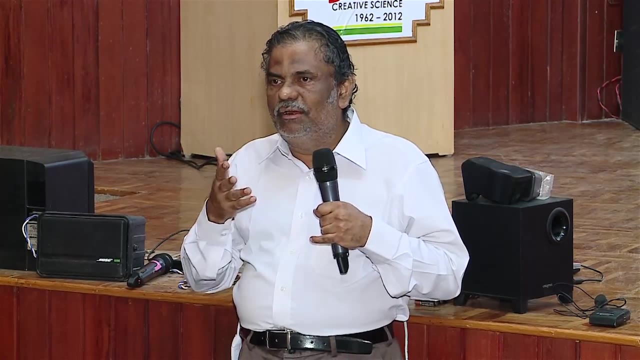 group of people to train them in the second stage to third stage. we have a big group of people from third stage to fourth stage and so on, so forth. the only question is, from the first stage is second stage and if some of you can take some time off from your teaching and identify. 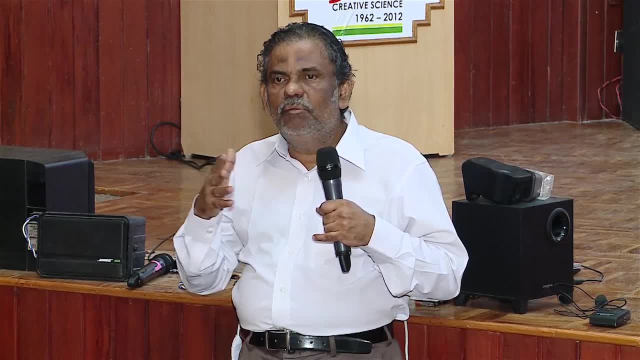 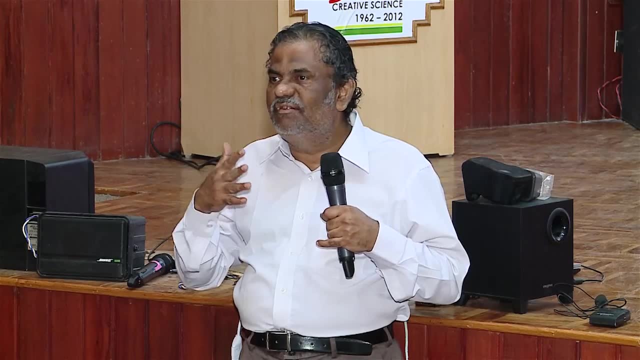 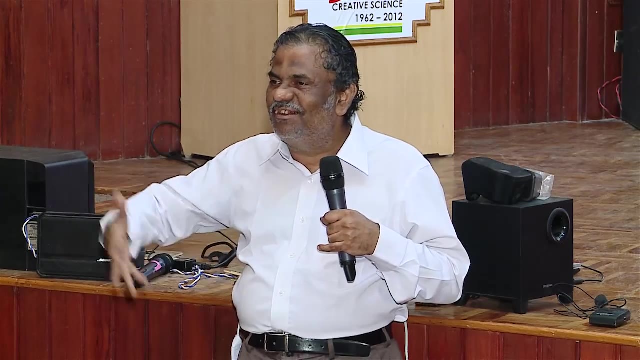 good students and teach them so that they would be able to do the olympiad program at least in the first level and come up to the second level. that would actually give you a certain visibility to your department in your school and you can also write all your cv of your school etc that you know the olympiad level they have gone, and so on, so forth. 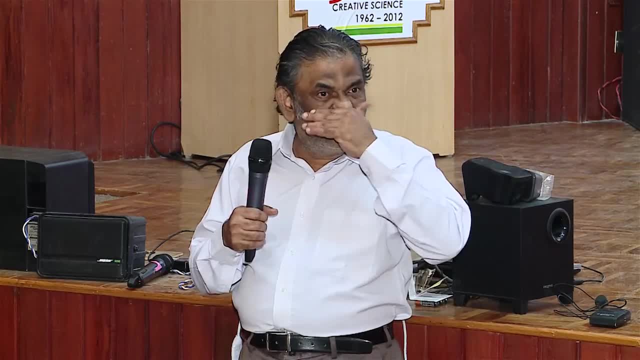 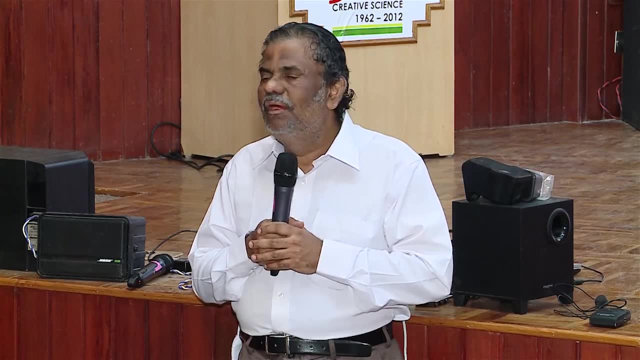 and in that particular condition, we are actually trying to get some books on the olympiad and i think there is a small section of the olympiad problems that at least would be useful for you and therefore i will definitely request you to spend some time than the olympia things and the 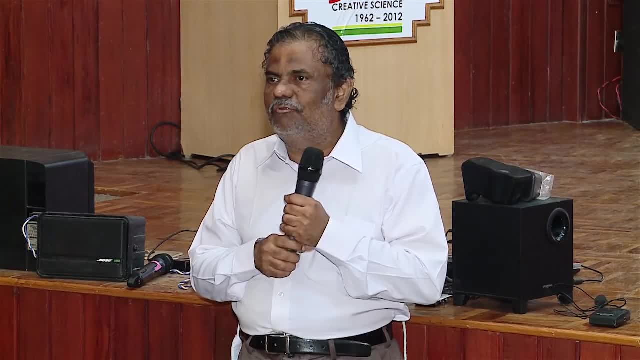 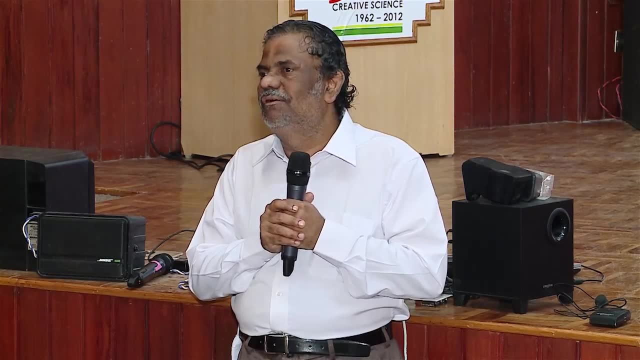 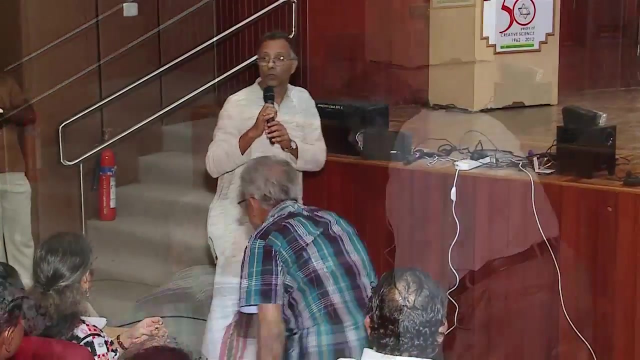 discrete mass and the number theory etc. which you are learning here would definitely be of useful to you to be able to train those children. okay, with that request, welcome you once again. thank you, before i hand over the hand it over to the next speaker who will introduce himself. 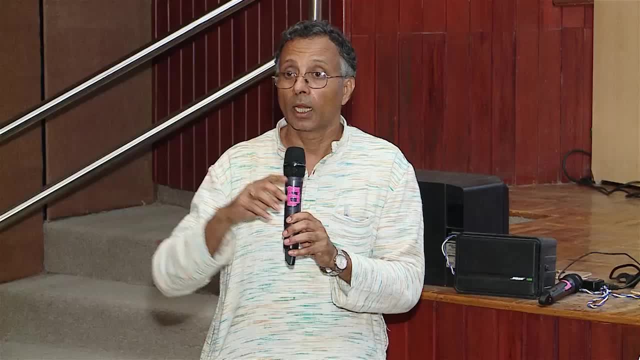 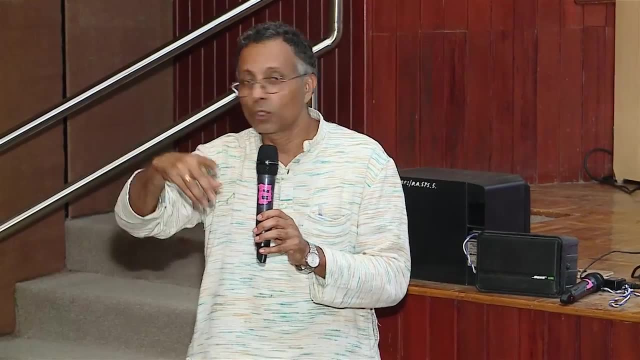 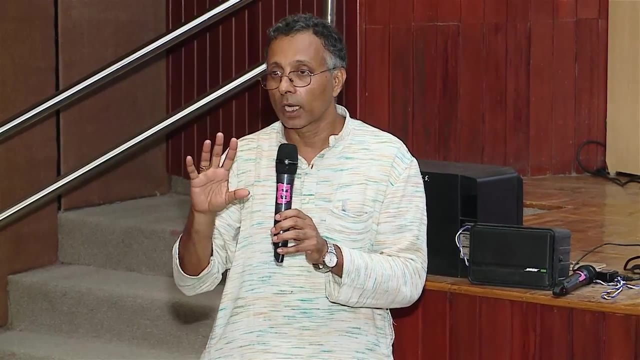 i'll have two announcements. one is that lunch is on the other side of the road, so follow you know. there is, i'm sure, some people who know where it is, so follow them across the road, okay, and then, if you want, the photographs will be put up on the net, if that is good enough. 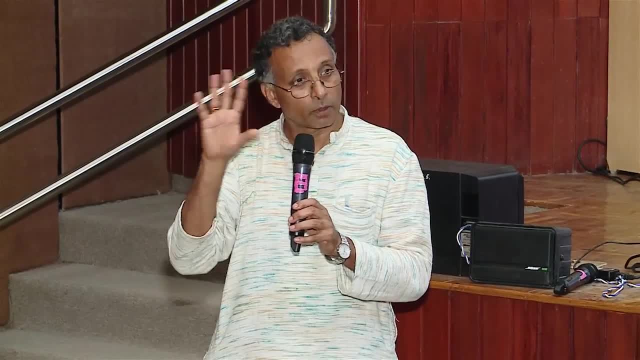 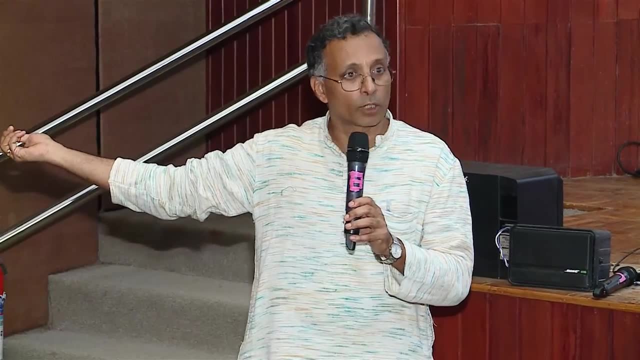 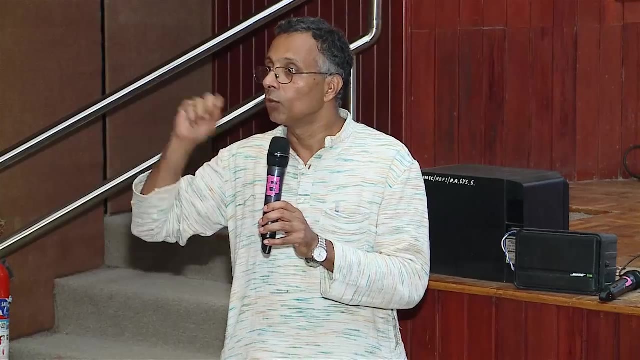 that's fine, you can always access it. it will be available from the web page permanently. but if you want a hard copy, you may sign up for it with somebody outside. okay, there will be people this afternoon or also tomorrow morning with at the registration desk. if you want a hard copy, you can. 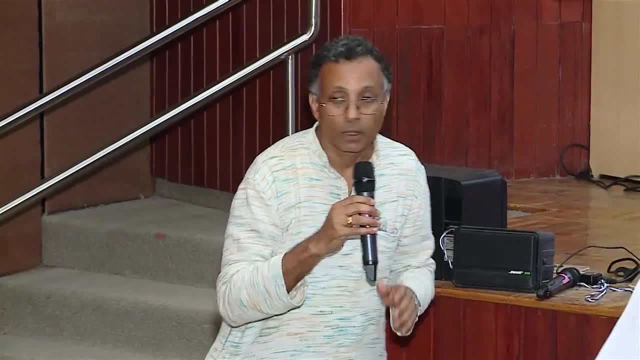 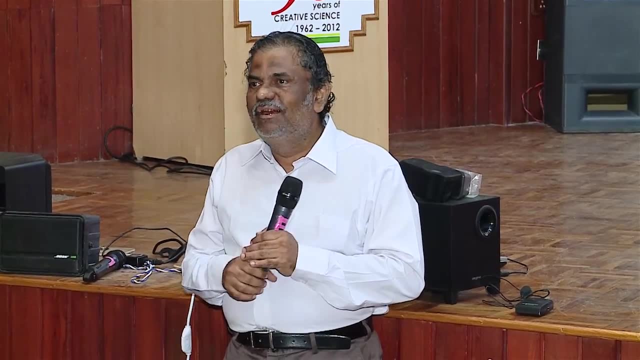 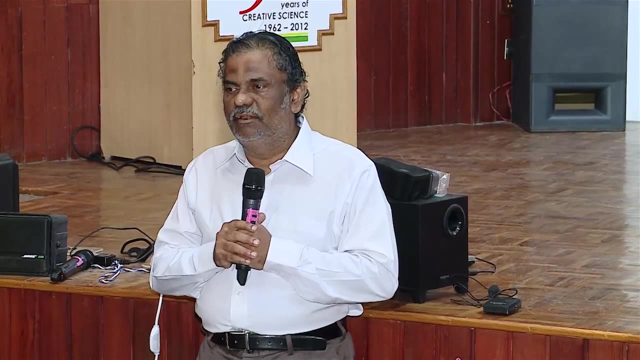 give them your name. with this i hand over the announcement i forgot, particularly since the majority of the teachers whom i see are women. let me just point out that so far for this olympiad program we have been choosing six people and settings for olympia and from this year onwards, the we have decided also to send. 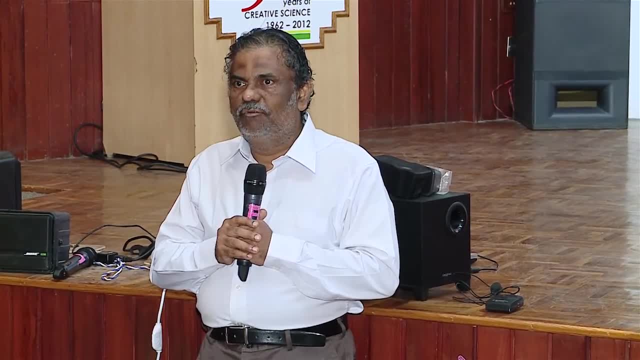 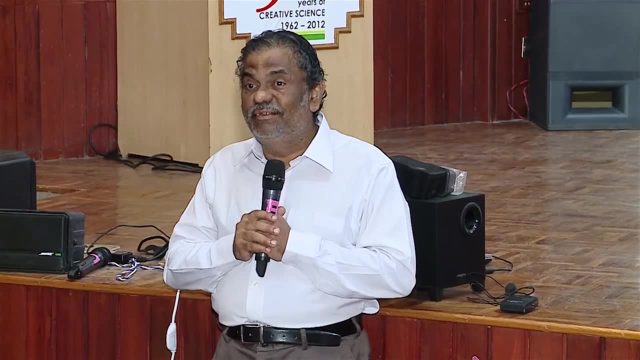 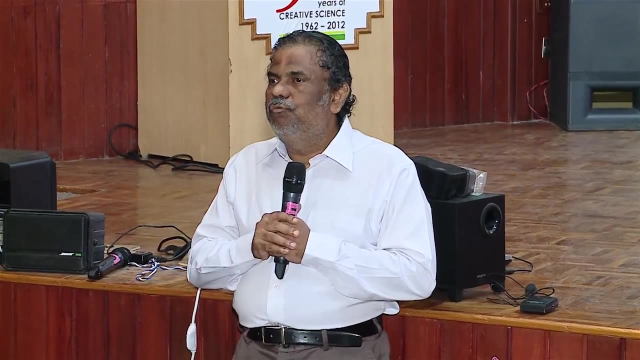 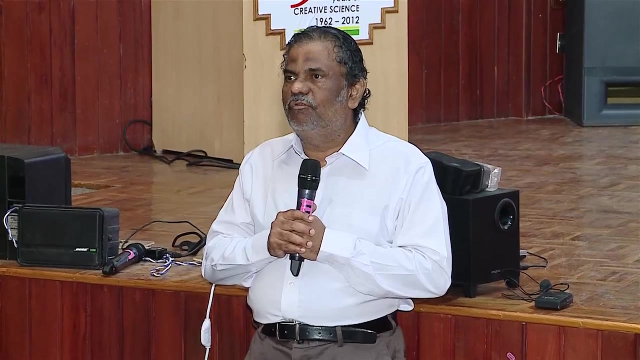 women's students for the women's olympiad program and therefore particularly those who are in women's schools, etc. should take some special effort, because this is something we're is starting this year and it will very nice if- and I should also say that in the last four, five years, the last six out of the last six- ninety percent of 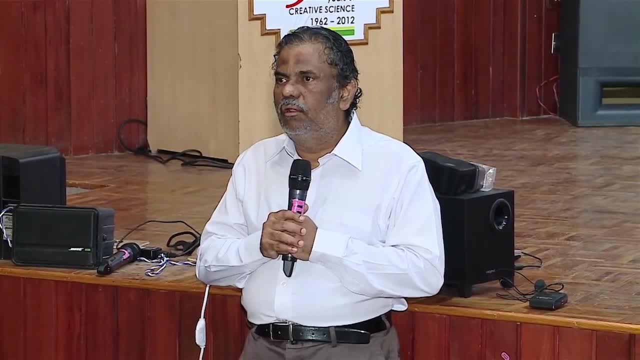 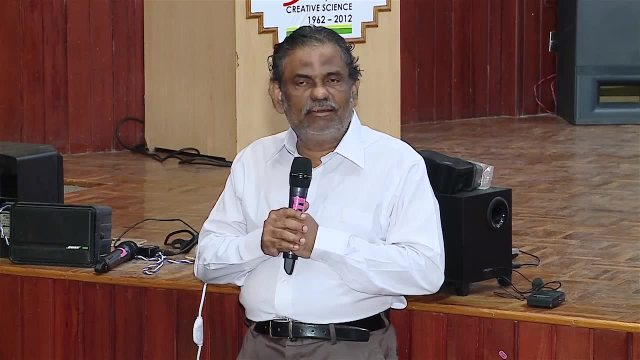 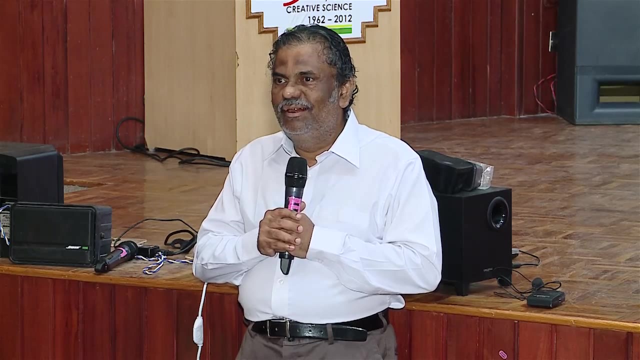 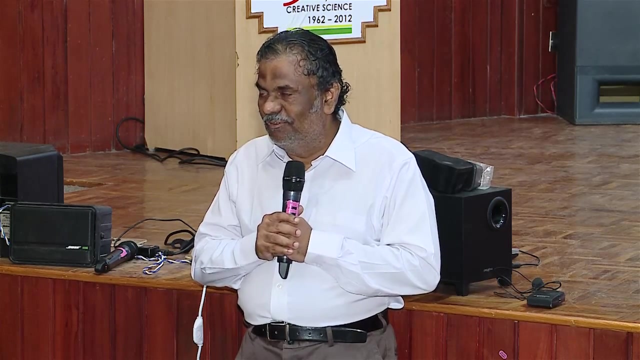 the students do come either from Bengal or from Pune and from no other part of the country. okay, and that for people who has coming from this romanians land should be somewhat ashamed and it is now in your hands to correct it. okay, and at least those girls will pair programs also starting this year, and please take. 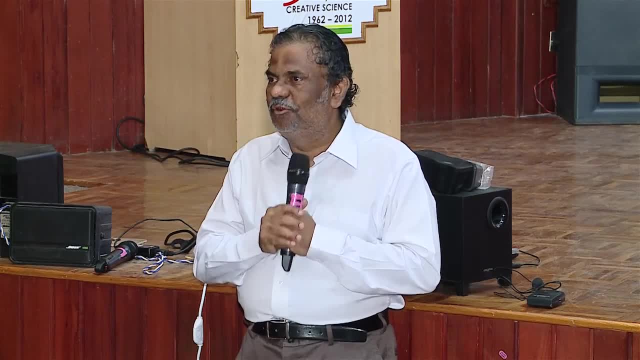 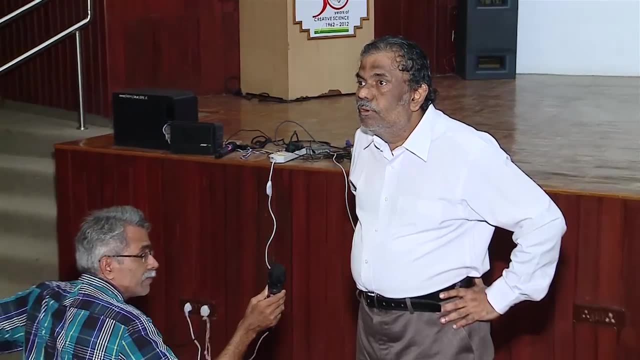 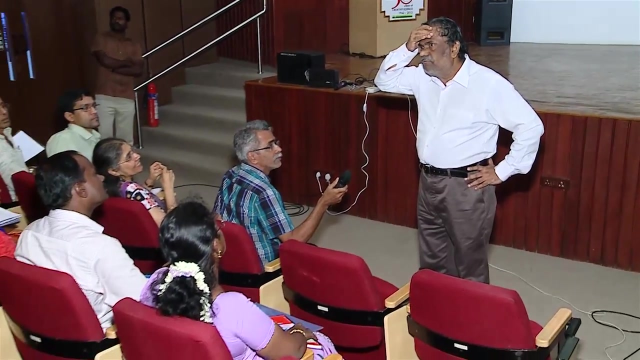 some efforts to train some of your good students to attend the only paid program. preliminary is: I have no idea at all. there's a person by name Ranganathan who retired from Vivekananda college. do you know him? otherwise I will try to get you the information. there should not be a. 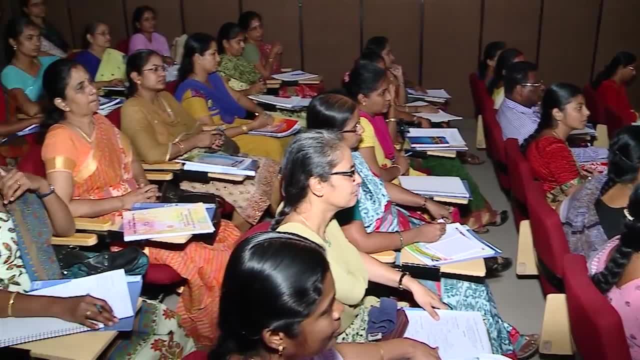 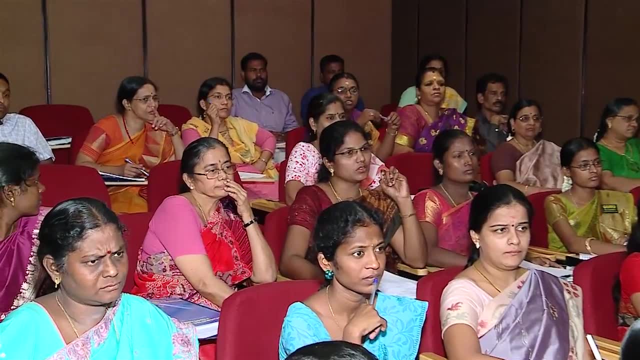 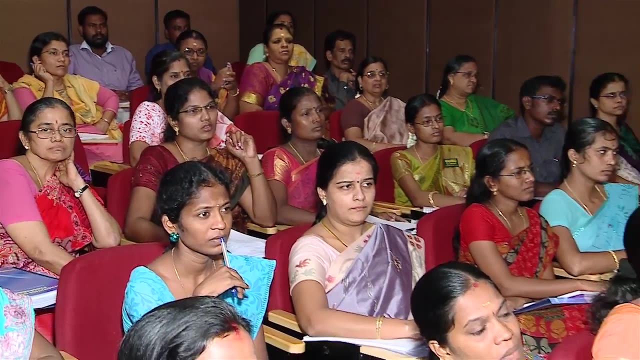 problem. yeah, yeah, yeah, the day, the day of day is the one which it does the first original. no, no, no, no, no, there's no different exam. that's only one exam and the national board for hand mathematics conducts exam from the second stage onwards. the first stage are: 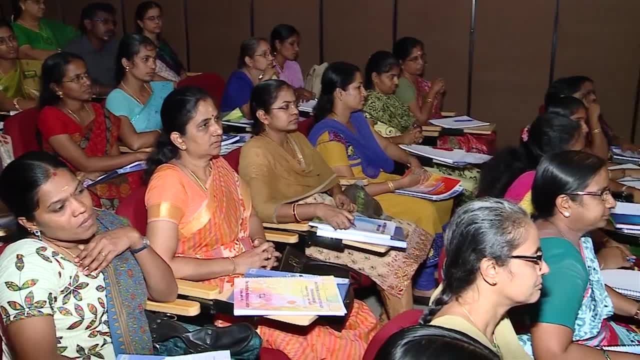 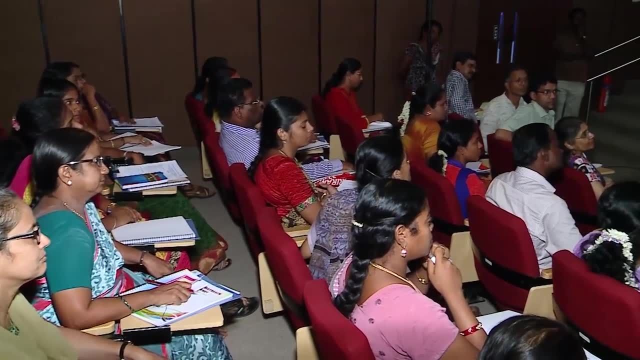 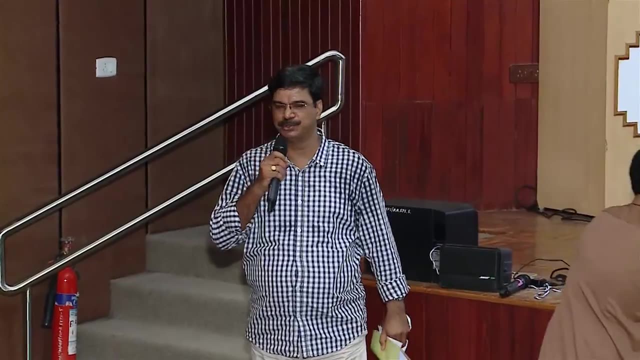 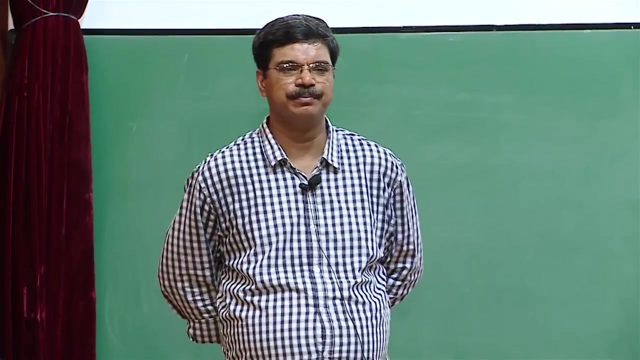 given to the local authorities and the. as far as familiarity is concerned, it is done by IMTA. from the second stage onwards, the national board will take over. hello, good morning everyone. I am case renew us. I work in number theory in this in shoot, so I will be delivering two talks. okay, so I will. so many of you. 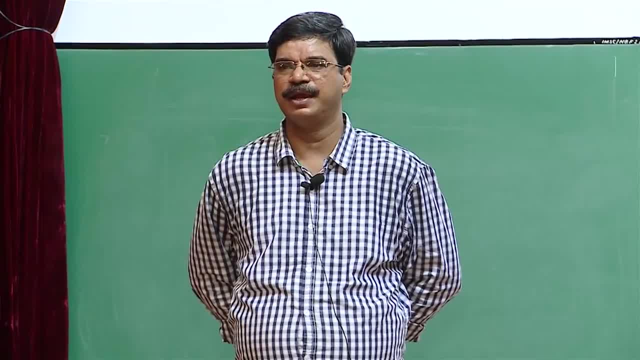 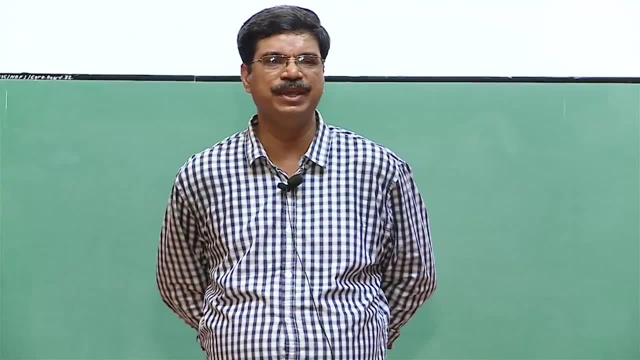 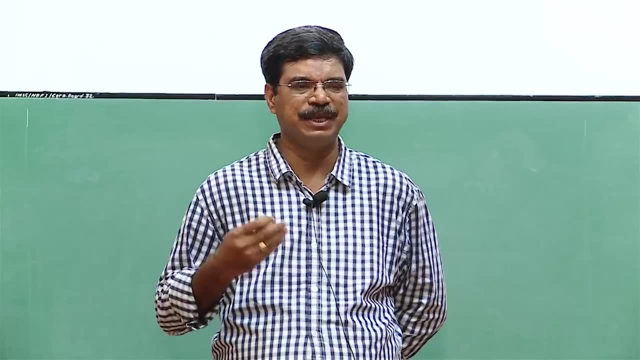 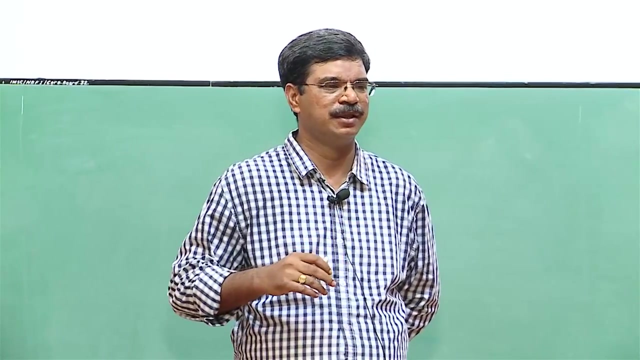 have come previous time also and see, as has been told here in the morning, that one of the aims that we look forward is: you know, the students have many queries like: what do mathematicians do, what is done in research? because it's very difficult to say to students, you know, physicists work, one can find out biologist. 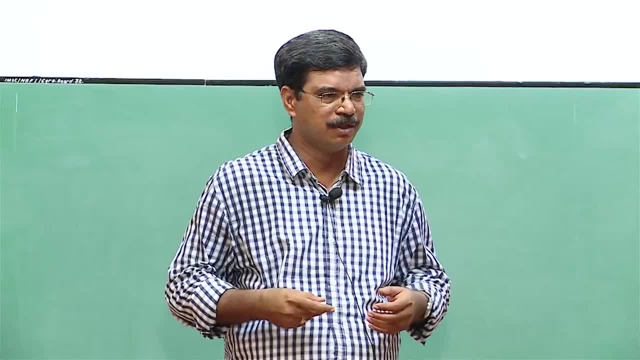 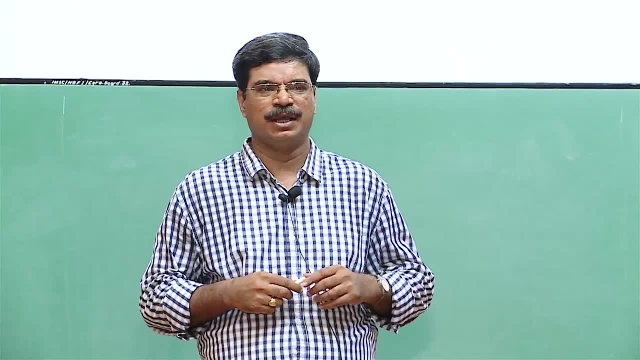 one can find out science. one can find out the calculus, one can find out the knows what they do. it's- because it's very visible- geologist. but what does a mathematician do? what is the research that is done in mathematics? that is one of the problems and the second. 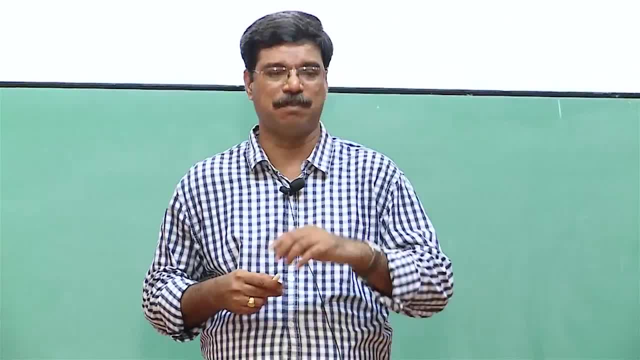 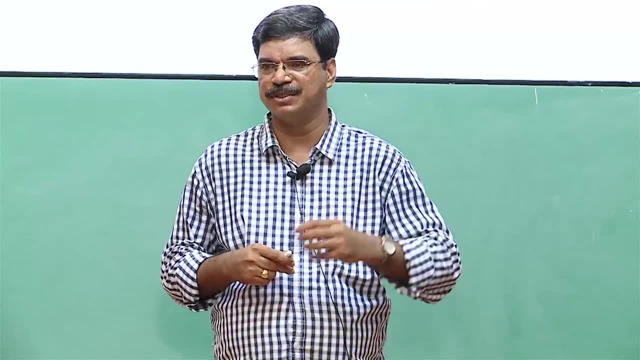 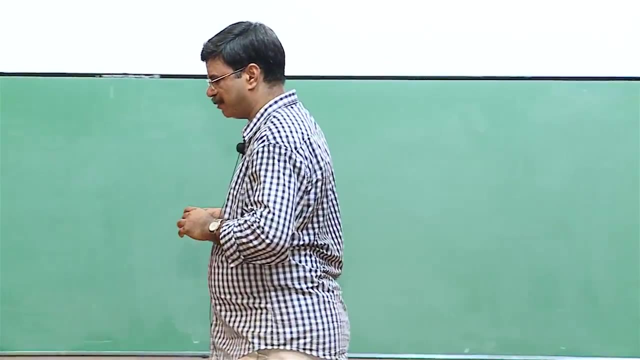 problem which is more often asked is: where is it applied? okay, chemists can easily say that you know we make medicines or something like that, but mathematicians, where is the mathematics applied? so I think we will address some of the questions as we go along, but most 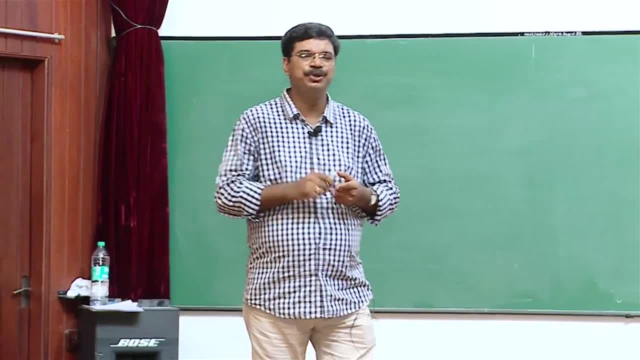 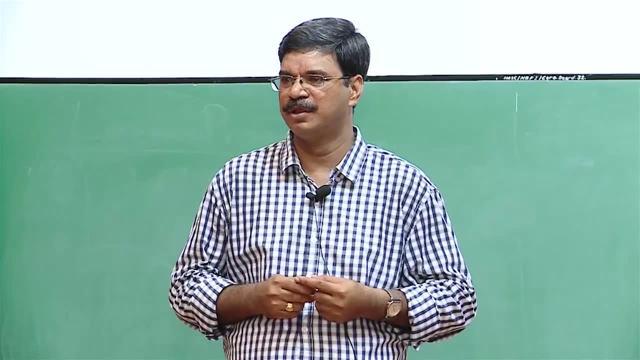 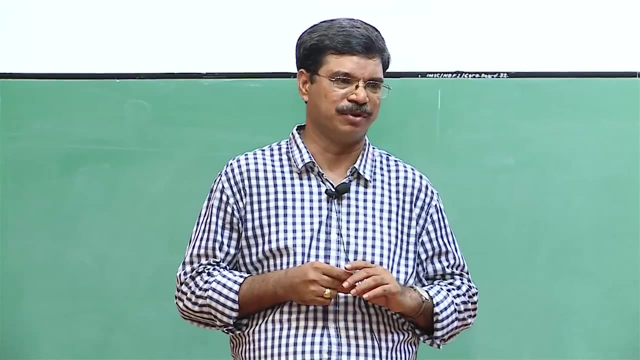 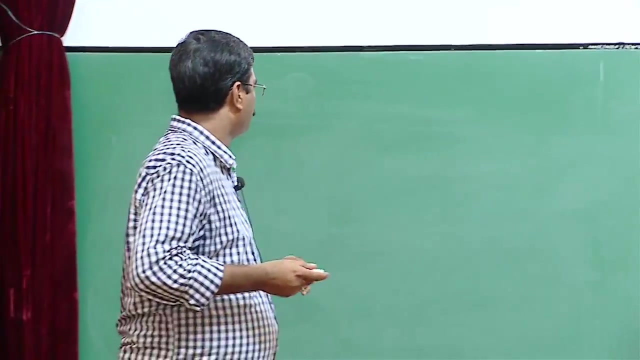 important thing is the beauty of mathematics. okay, the student should be told that mathematics is indeed beautiful, and for that all of us should first get convinced that it is indeed beautiful. okay, so we will see some of the ideas, very basic ideas. okay, so number theory starts with. okay, in my lecture, all numbers are integers. okay, when I say n, 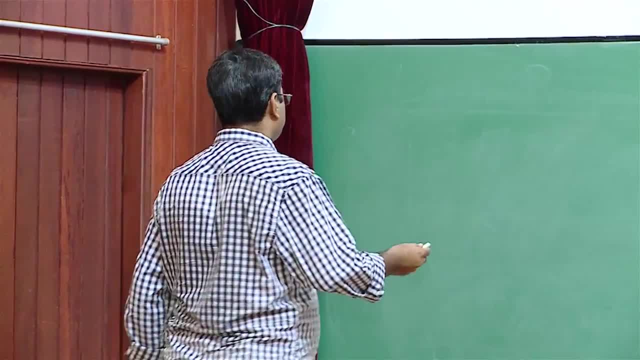 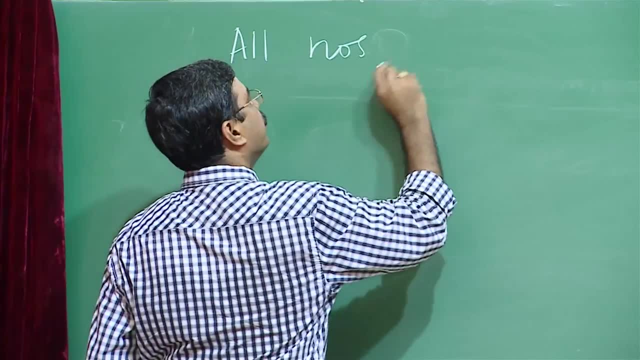 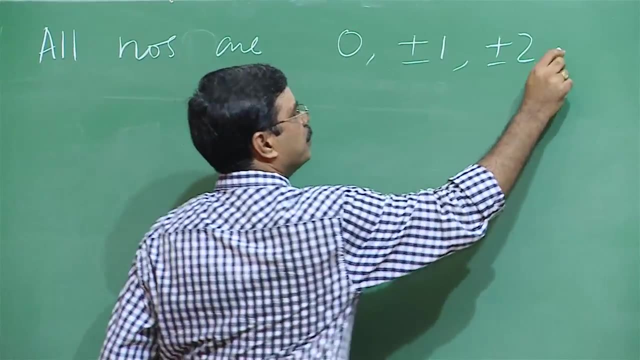 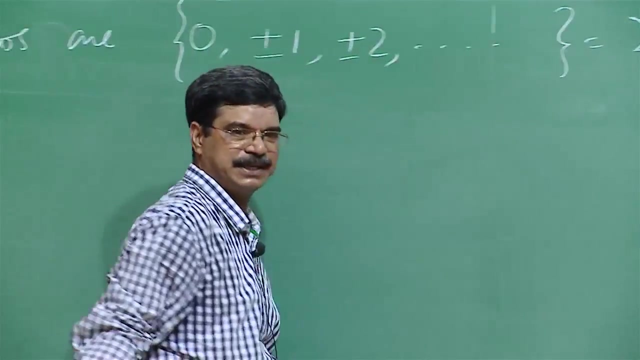 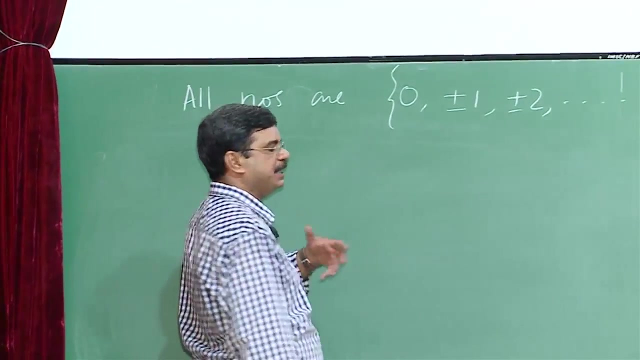 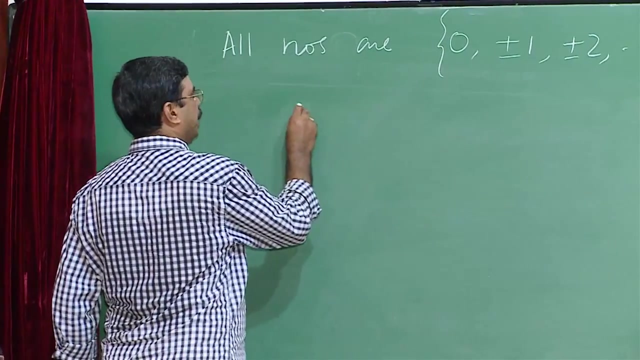 is a number, I mean an integer. okay, so all numbers are, are like: okay, and this, we denote it as set z, okay, set of integers in my talk. okay. and when we say that an integer a divides another integer b, we write it as so: a divides another integer b. 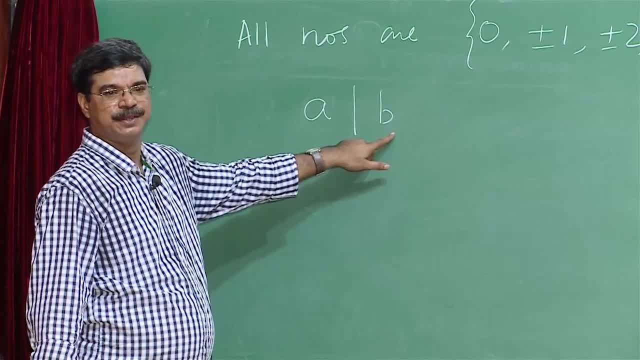 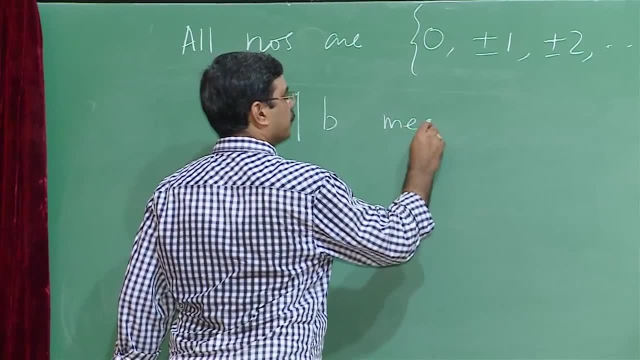 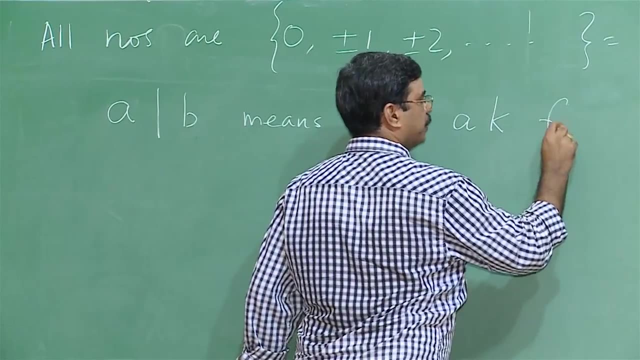 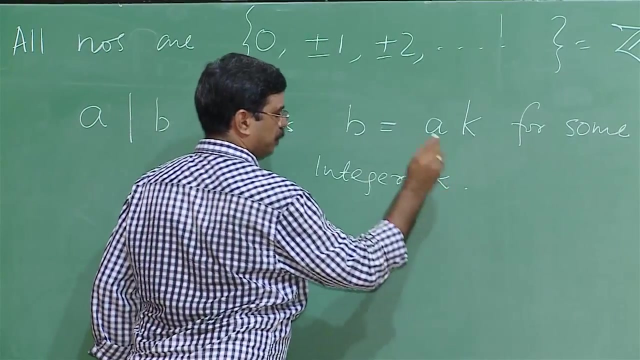 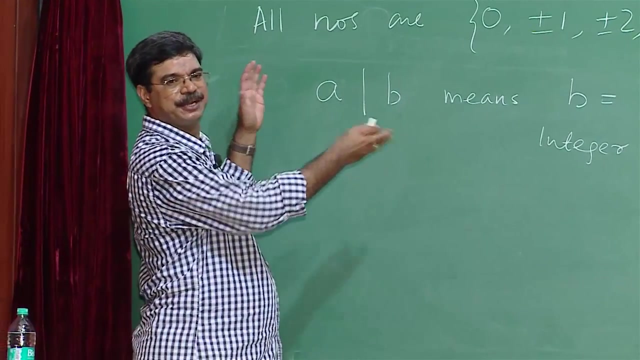 what is the meaning of this? b is a integral multiple of a. okay, that's important. okay, so that's it, Thank you. this means b is some a times k for some integer. okay, and many properties are very clear from this. for example, a divides b and b divides c. 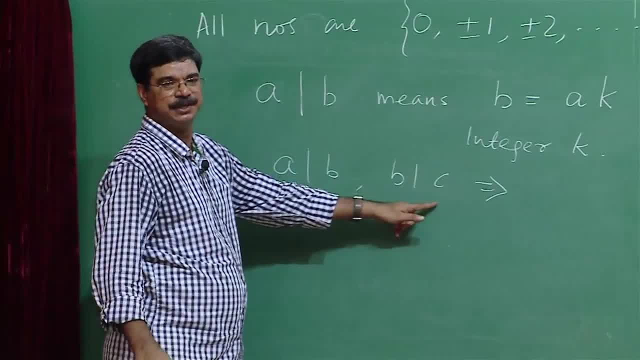 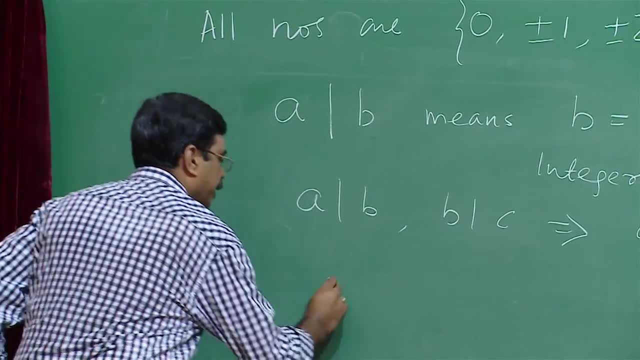 this will imply that a divides b and b divides c. this will imply that a divides b and b divides c. this will imply that a will divide c- okay, this is very clear. and similarly, a divides. suppose a divides b and a divides c, and then a will divide b plus c, a will divide b minus c. 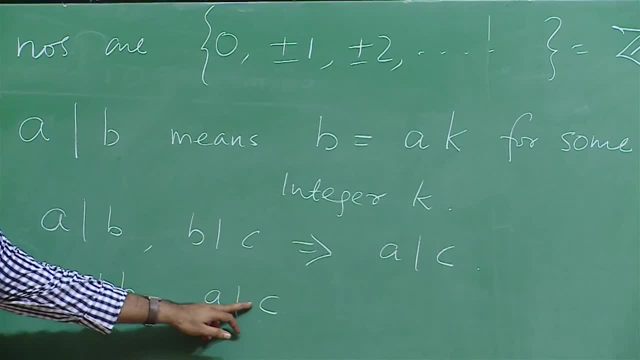 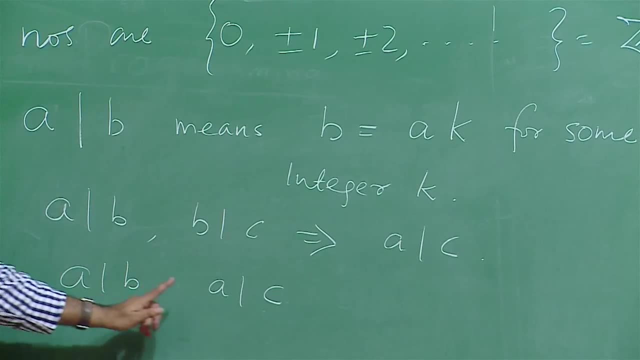 that whole will divide b plus c, a will divide b minus c. a will divide an integral multiple of b, yes, and a will divide an integral multiple of c. therefore we can say that now you have noted also that that angle. ok, so here, if a is so, what I will do here, I will define an integral multiple of b and b. you multiply it with this integral between them. 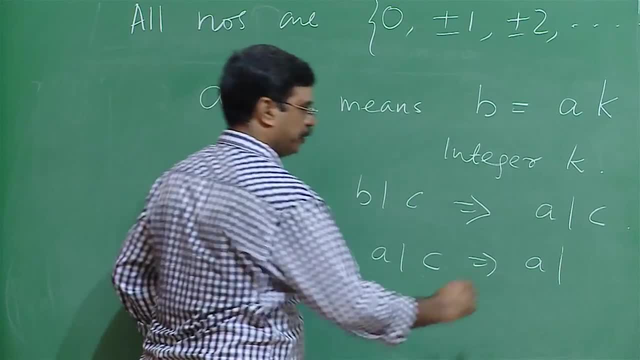 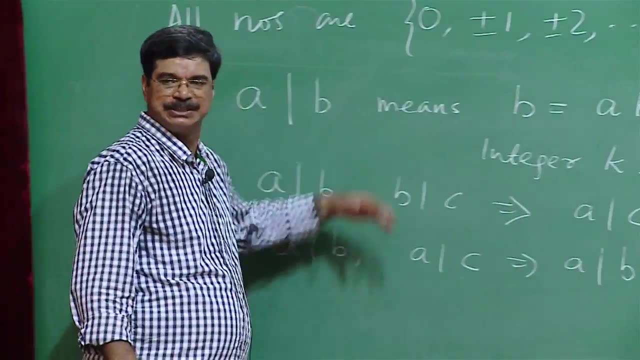 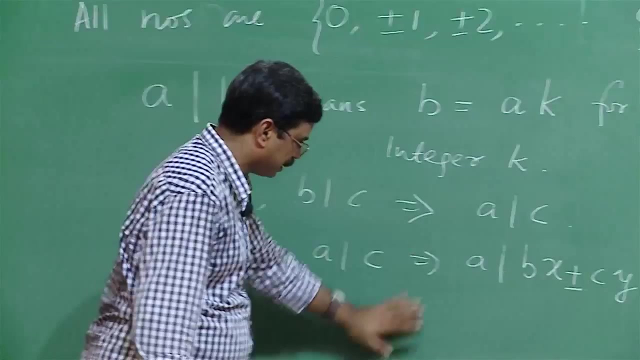 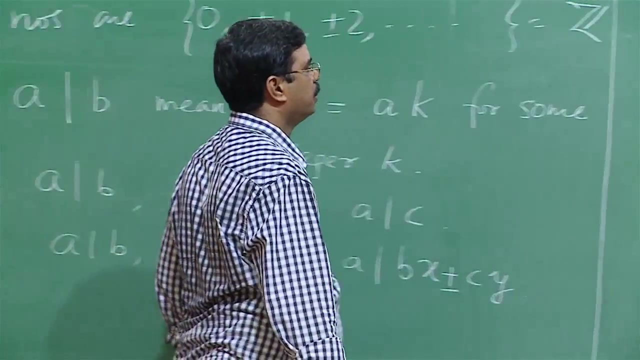 this implies a will divide b times some integer x, plus c times, some integer y. So these things follow from the definitions. ok, Many things. one can write down very beautiful things. And this definition, the first theorem that one encounters, is what is called popularly. 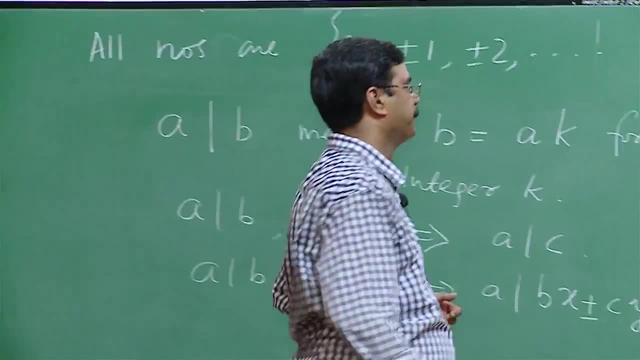 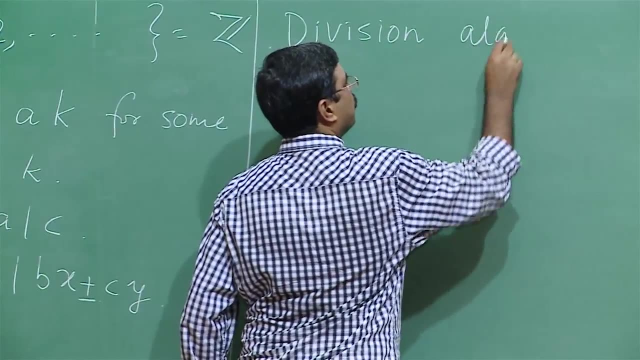 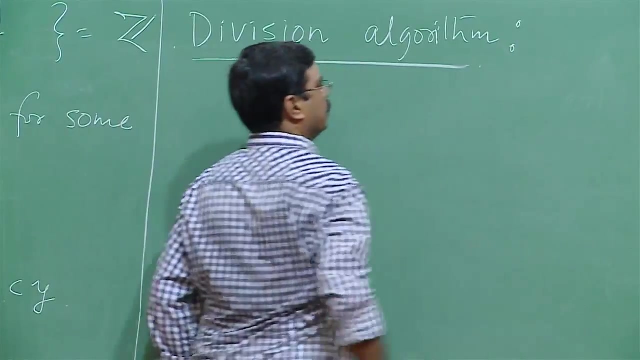 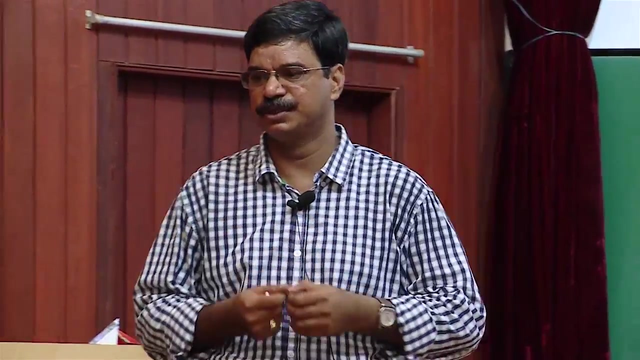 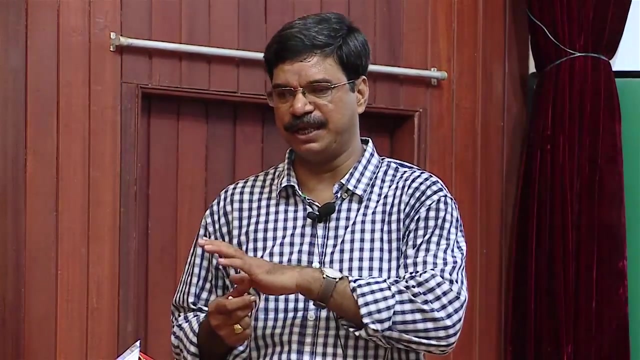 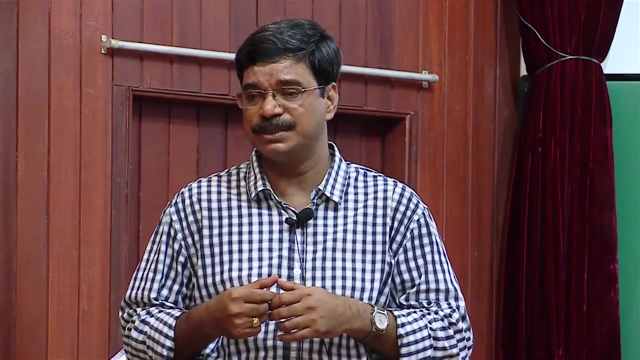 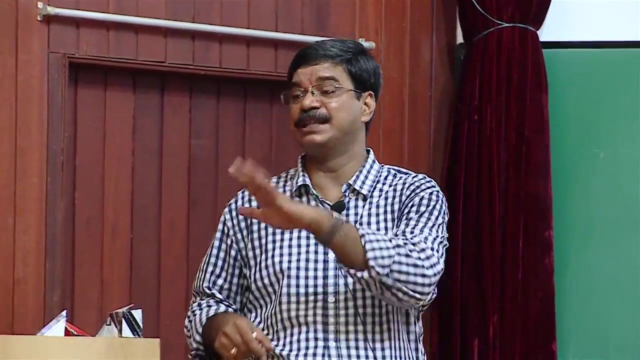 known as division algorithm. ok, What does it say? Given any two numbers, a and b, you divide a by b, you get a quotient and a reminder. But there is nothing great about this statement. What is great about the statement is this: q and r. if you impose some conditions, then 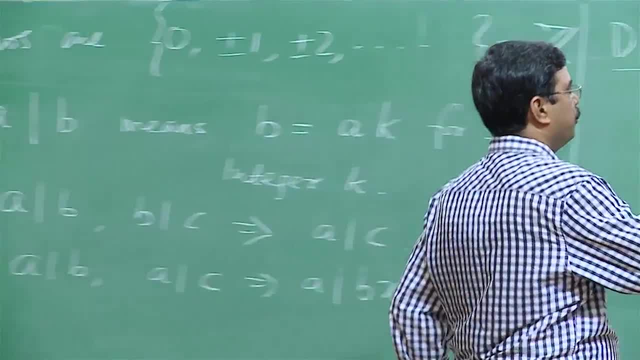 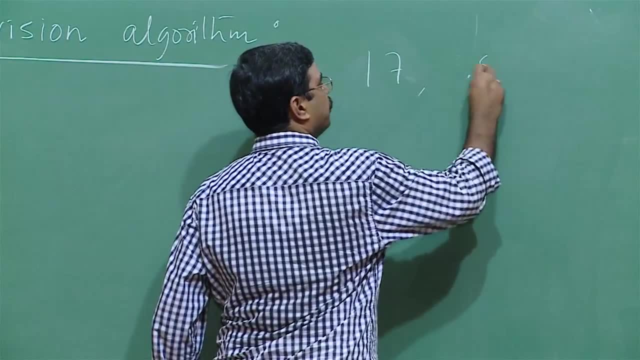 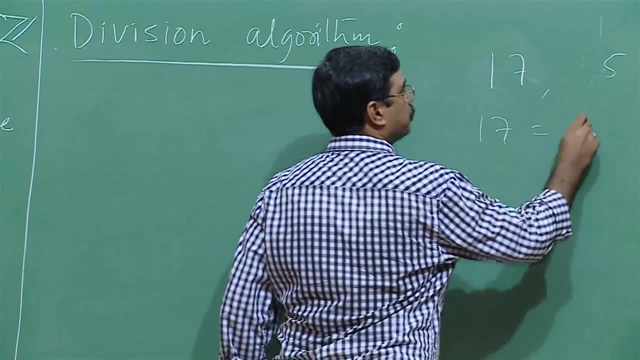 they are unique, For example, 17. 7.. If you are given 18, 17. Ok, What kind of integer are you able to give it? glue? So glue is you can write only an set of categories one on one. 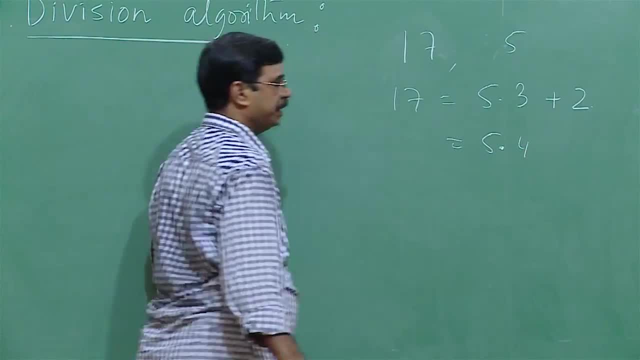 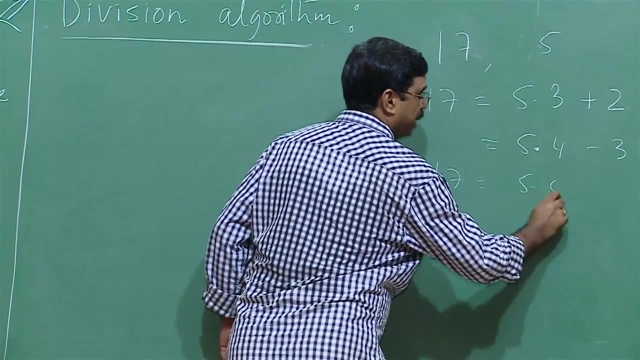 Right, So if a和all is a, then it is. look, it is like that you are going through some problem. Ok, powers converted all the values. 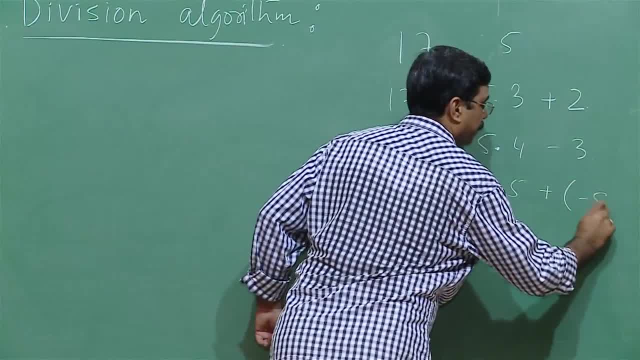 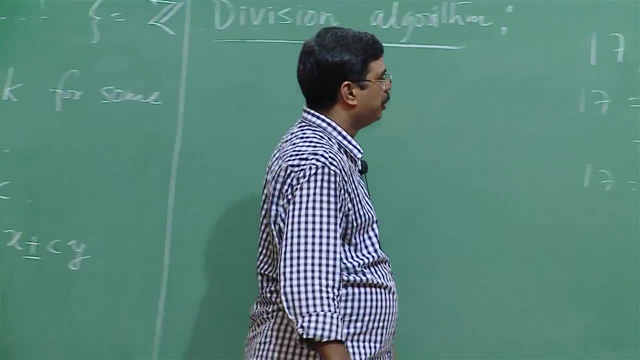 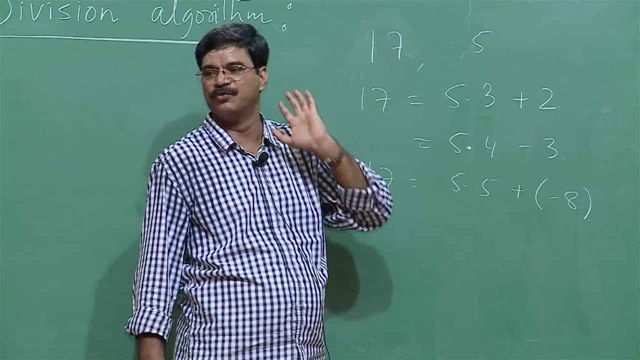 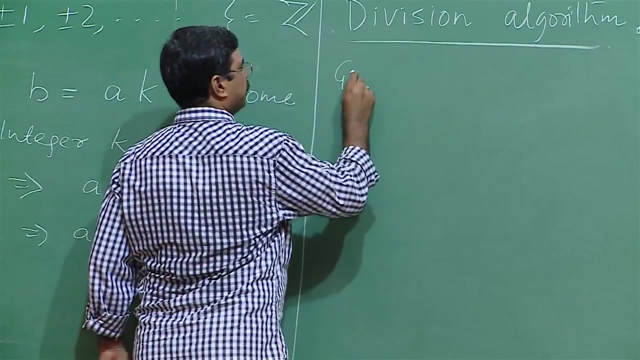 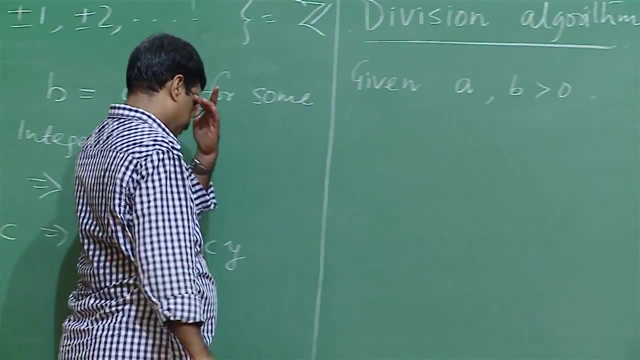 minus 8. there are infinitely many ways of writing, but division algorithm says that if you restrict the remainder less than the divisor, then there is only one way of writing it. So this is the only one way. Therefore, let us state it: given A and B, let us say B positive. 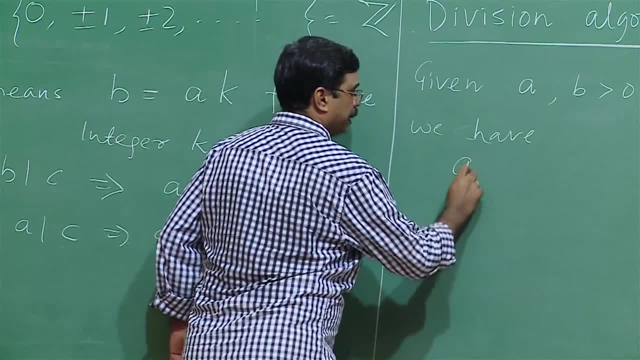 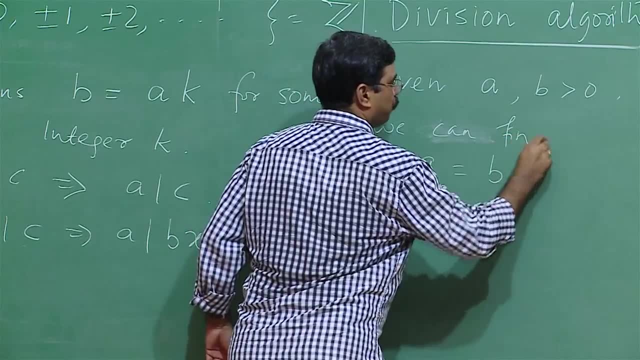 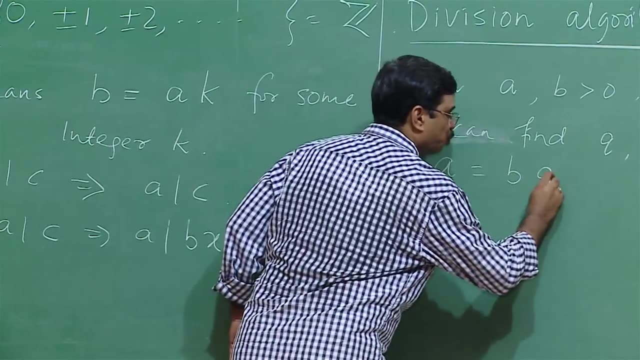 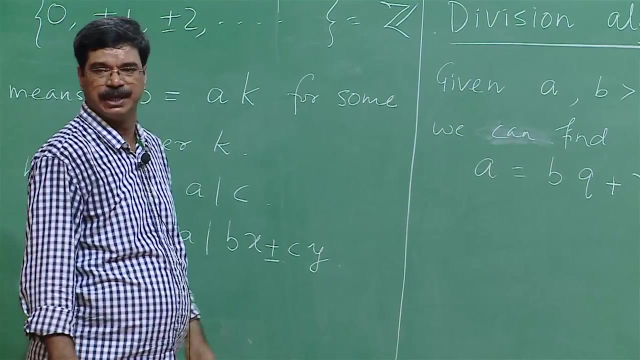 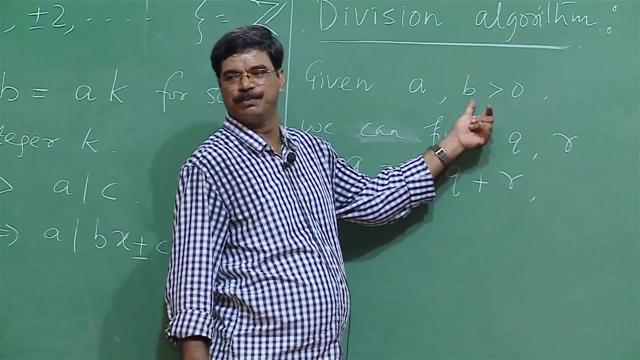 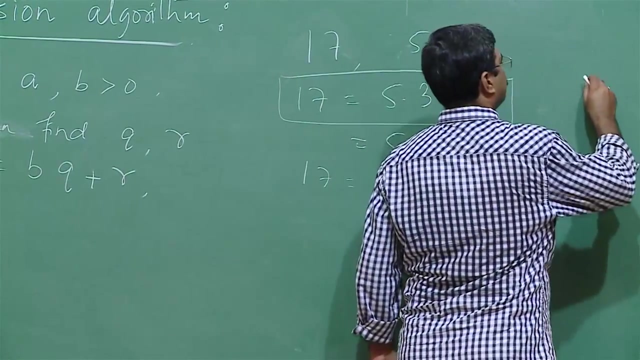 we have. A is equal to. that means we can find, we can find Q and R. integer, yes, says that A is equal to B times Q plus R. yes, B is equal to A Q plus R. see, I mean it is not necessary that B should be less than see, because if I have to divide, you know. 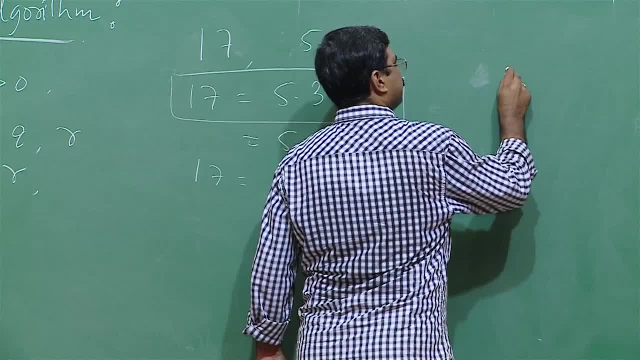 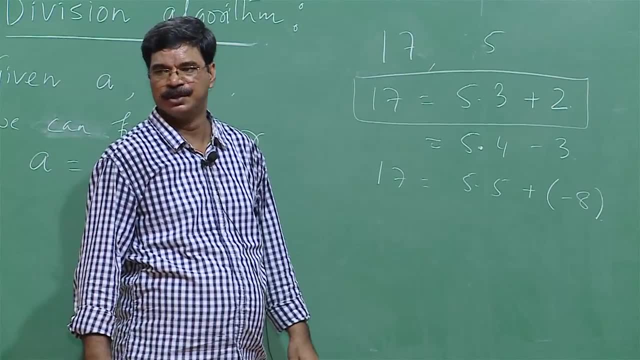 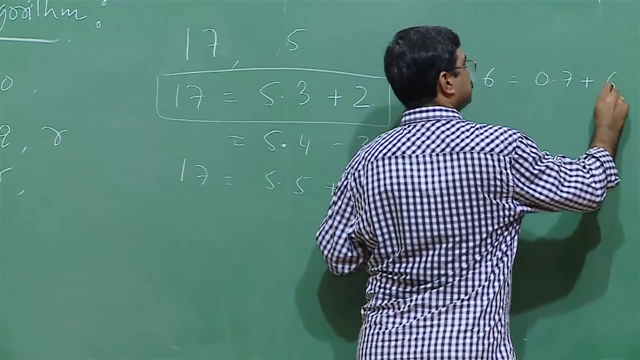 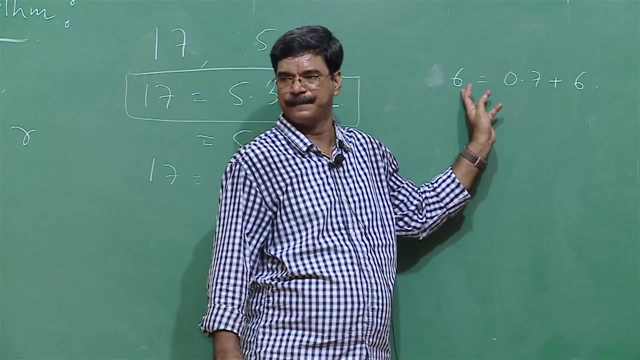 see, for example: Suppose I divide 6 by 7, how will I write? 6 is equal to 0 times 7 plus 6.. So 6 is always less than 7. I am dividing it by 7.. So we are not bothered right now, for simplicity. 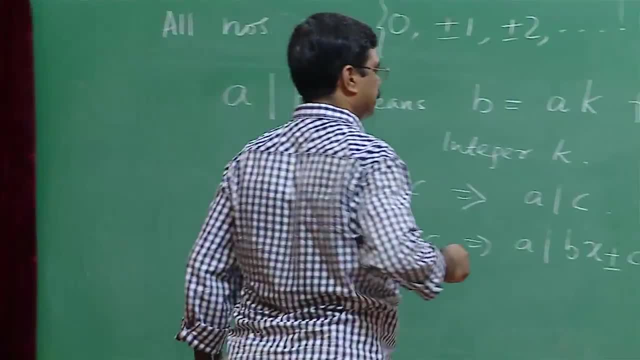 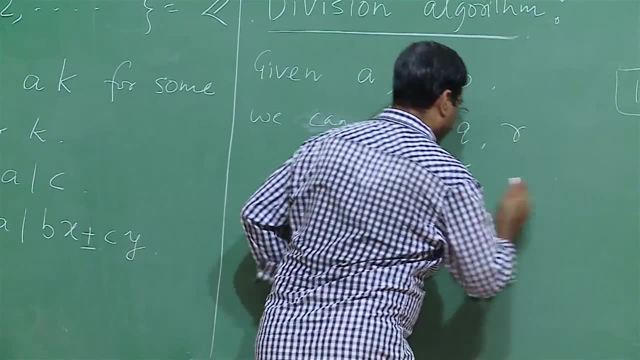 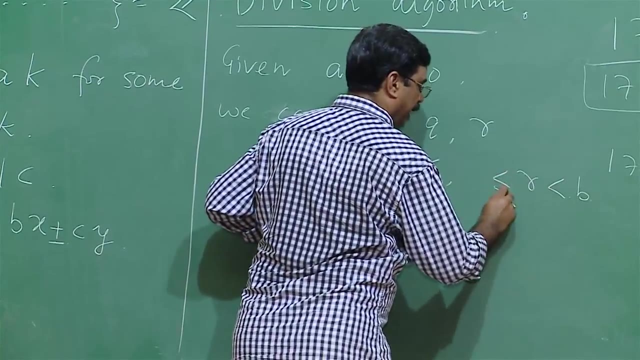 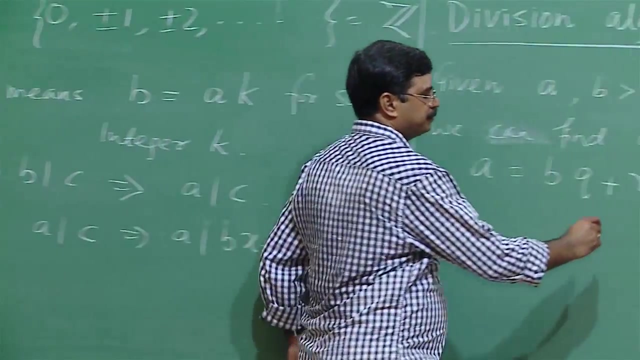 we are only taking. So we are only taking the positive integers with, otherwise we have to put a mod, absolute value. So this R will be less than the divisor B and R may be. it may be equal to 0. also, What is important is the expression 1.. 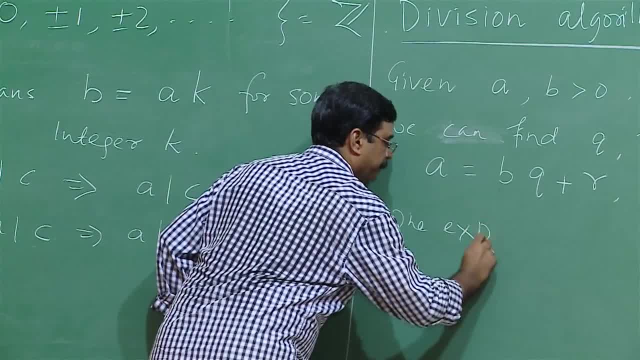 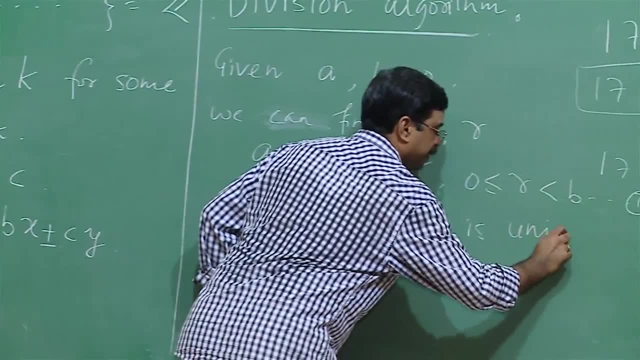 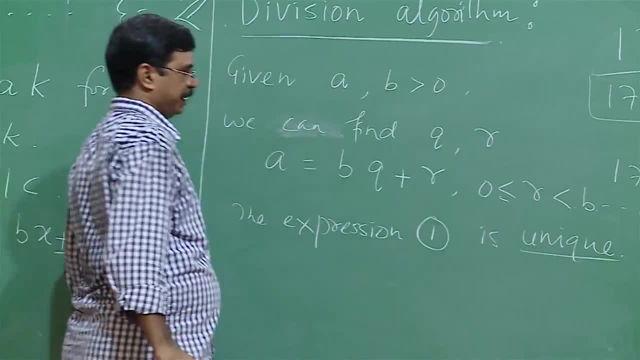 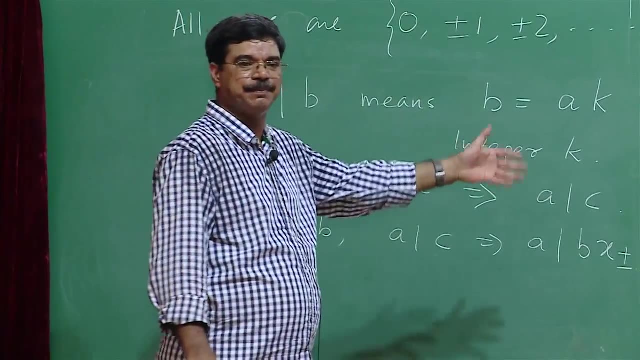 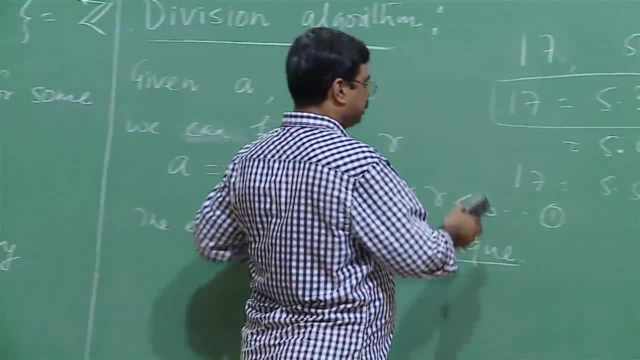 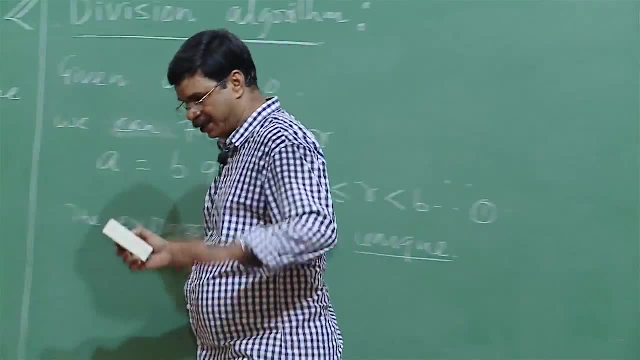 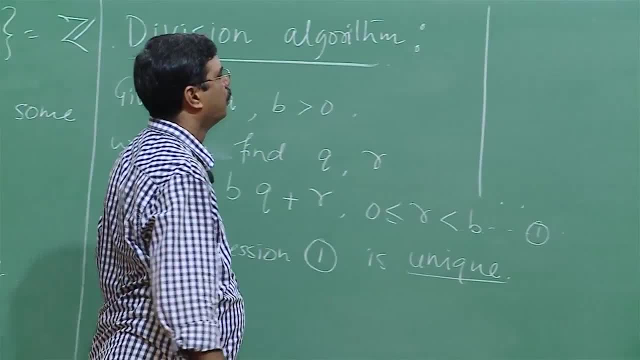 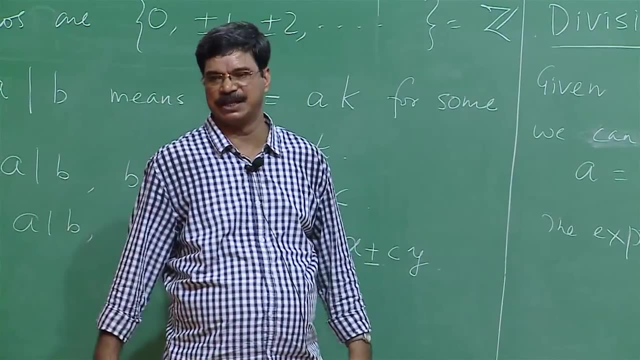 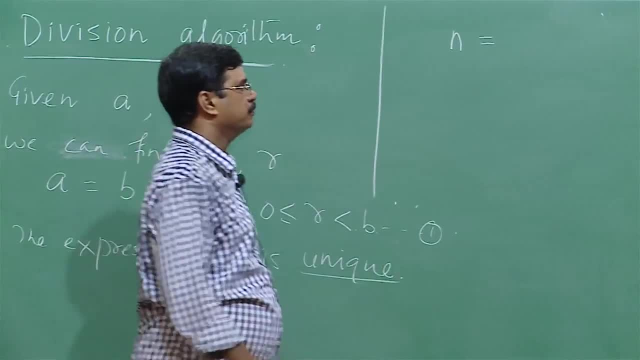 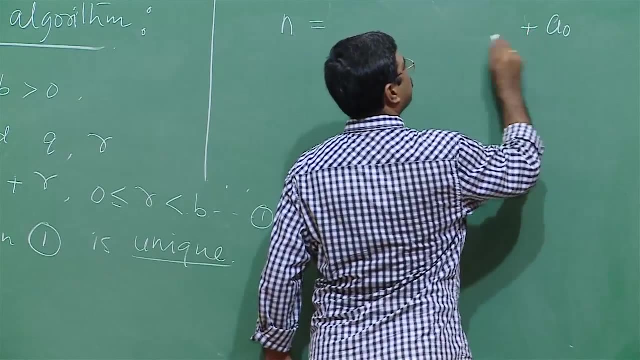 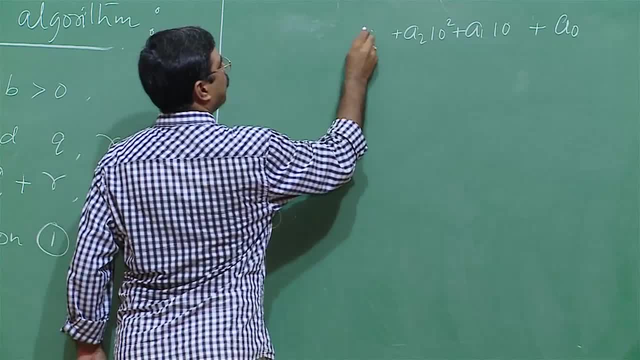 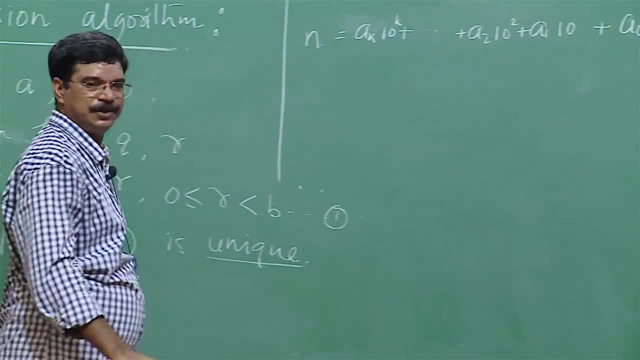 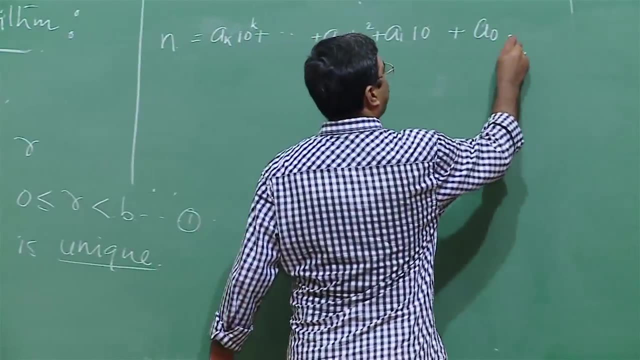 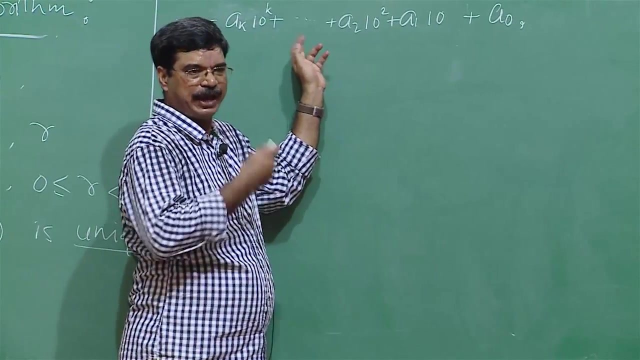 1. 1. 1. 1. 1.. a k 10 to the power k. This is usually how we write decimal expansion to the base 10. and what is this? a, 0, a, 1, all these things there, the digits of n, this k plus 1 digits. 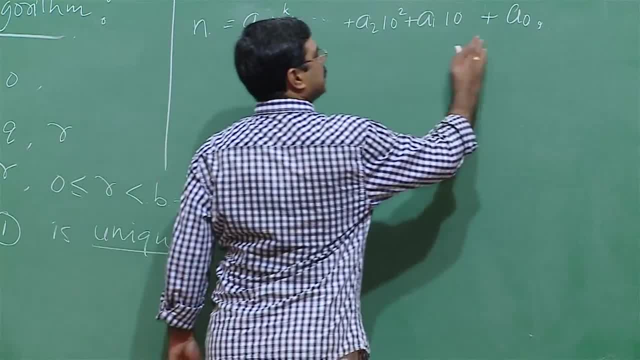 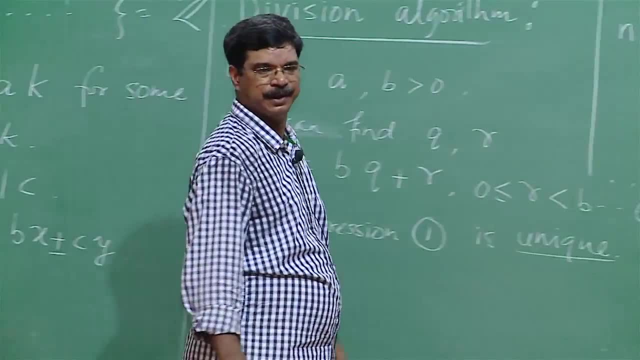 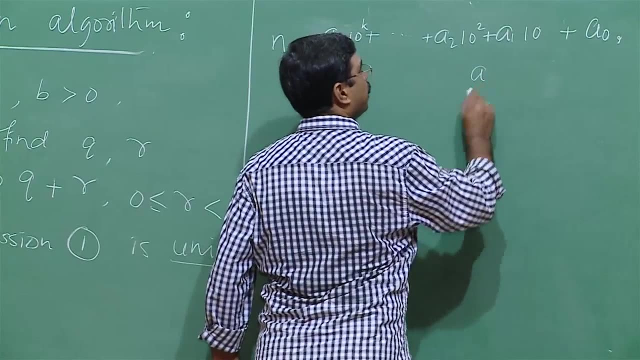 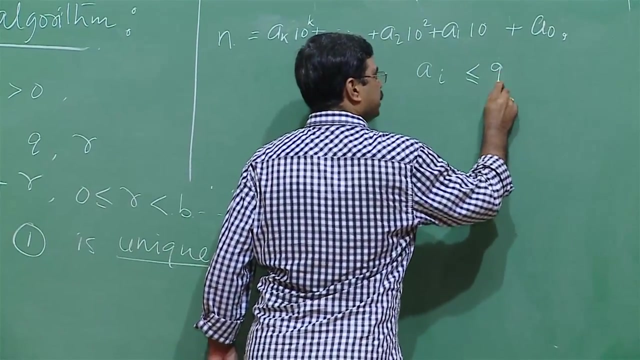 are there, ok? And what is the condition that is imposed on a? 0, a, 1, a, 2, a, k? They must be not necessarily greater than 0. some of them can be 0. Not only non-negative, all these a i's. they are less than or equal to 9, bigger than or. 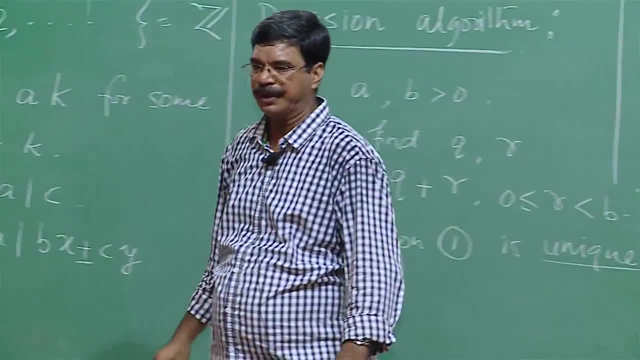 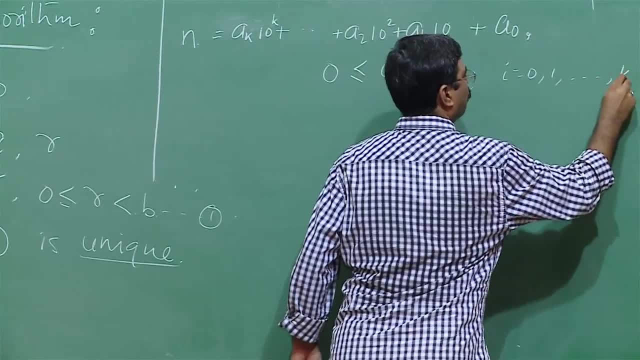 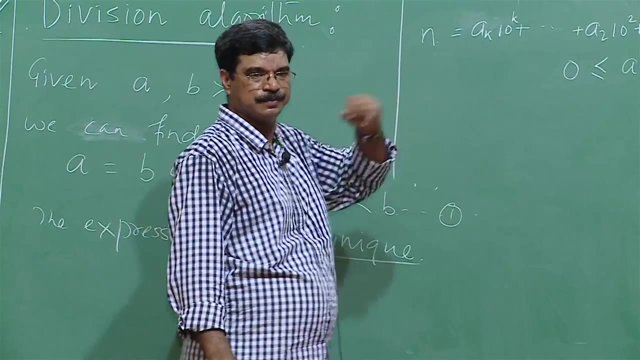 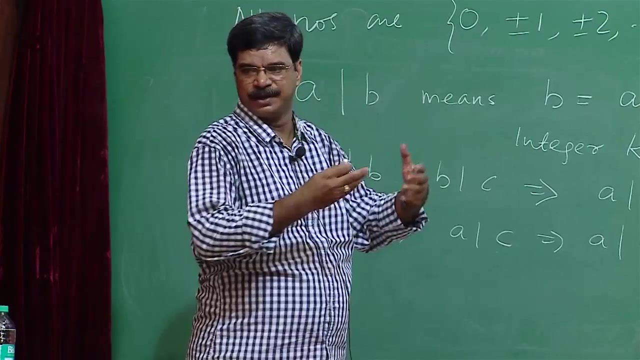 equal to 0.. Ok, Right, For i is equal to 0. 1 up to k. Where did we get this expression Right? this from here? we are given n to find its units rigid. we first divided by 10. So we get units rigid. 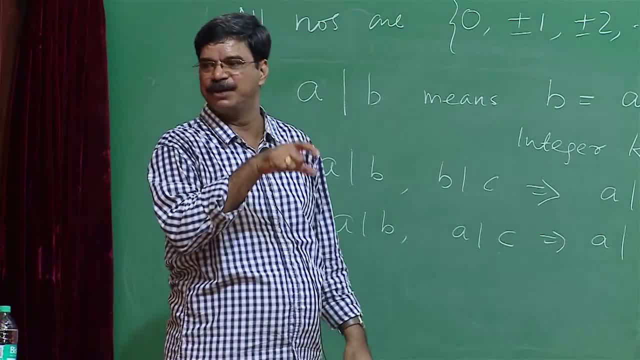 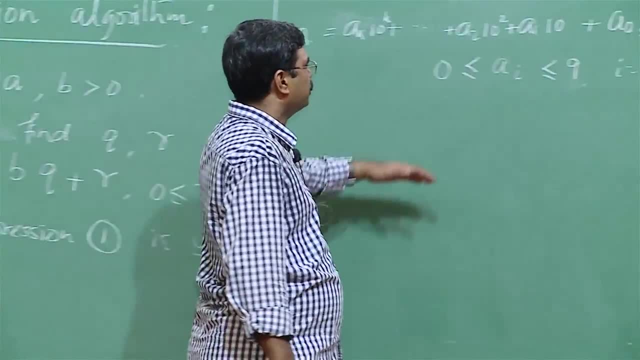 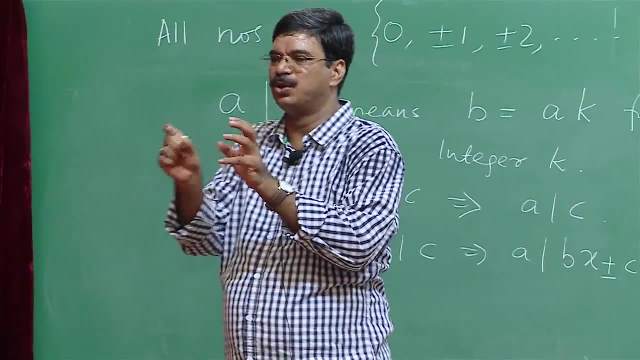 a 0. Then, whatever is there, We divide it by 10 again to get the hundreds, second digit, 10th digit. ok, So this has to be. you know, I mean usually what happens. we present them as an individual, isolated pieces. we must correlate the things, ok. 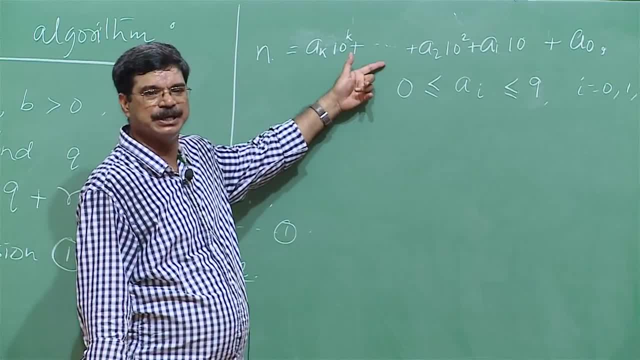 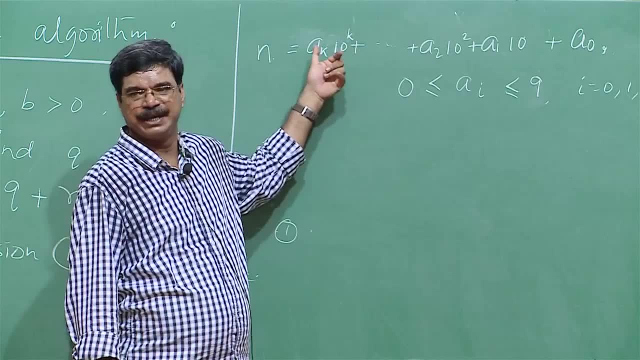 Therefore, and it is not necessary that the base should be 10 only. for example, if you are working with computers, Computers understand binary digits. Ok, Binary digits, So we can take it to be 2 base 2. then all the numbers are as a 0's and 1's, a sequence. 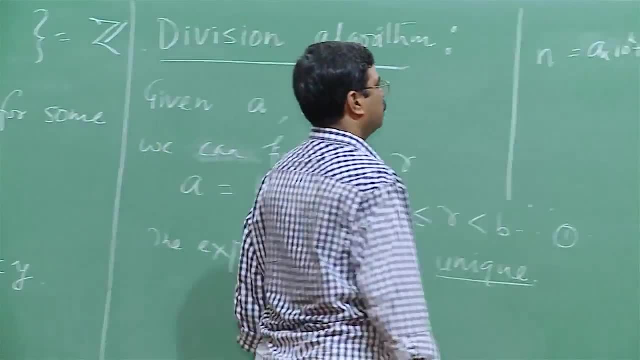 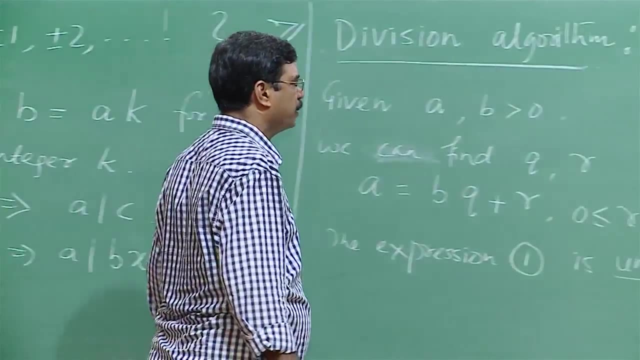 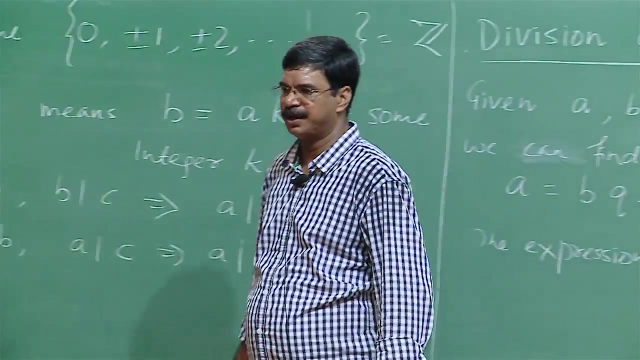 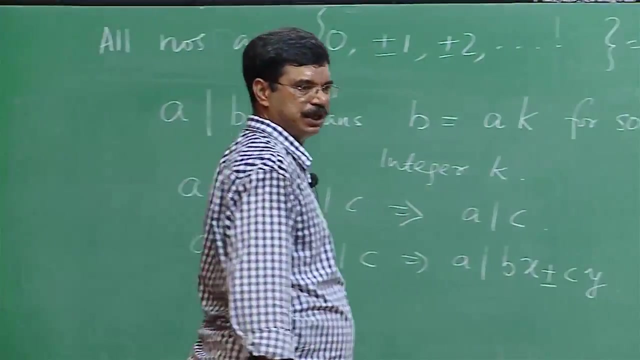 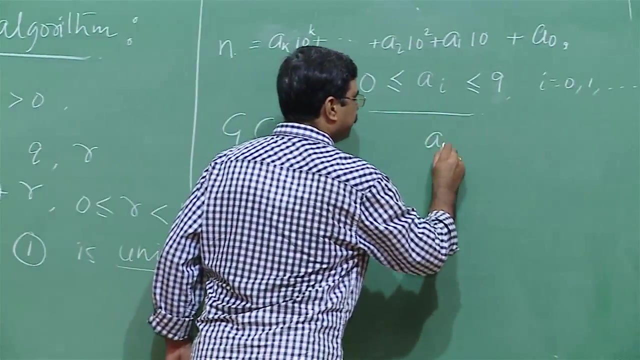 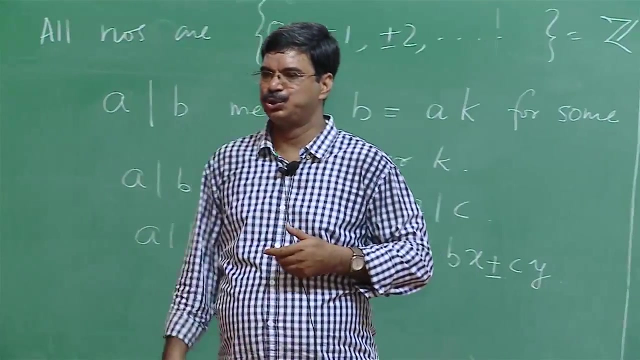 of 0's and 1's. Ok, So this is one of the things. Another concept, important thing is the concept of greatest common divisor, given two numbers. There is a, There is a GCD and which is unique, ok, A and B. look at all the common divisors of A and B. choose the one which is the largest. 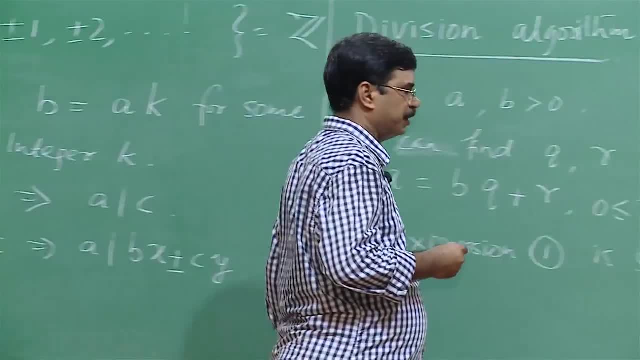 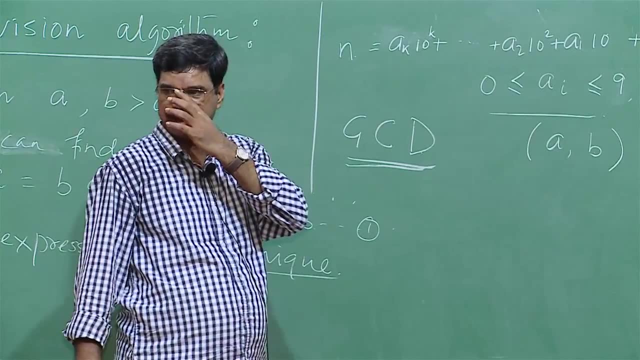 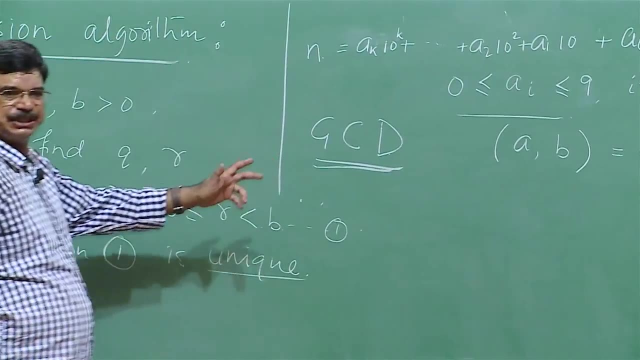 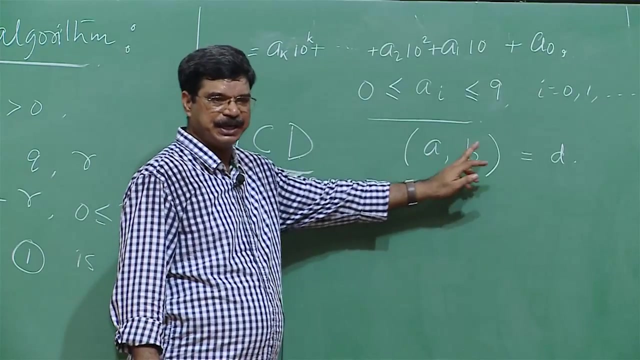 that is the GCD of A and B positive divisor and we represent, denote. this is the symbol to denote The GCD. ok, suppose we can say that when we say D, D is the GCD of A and B, we mean that D divides A and D divides B, because D is a common divisor and D is largest, such that 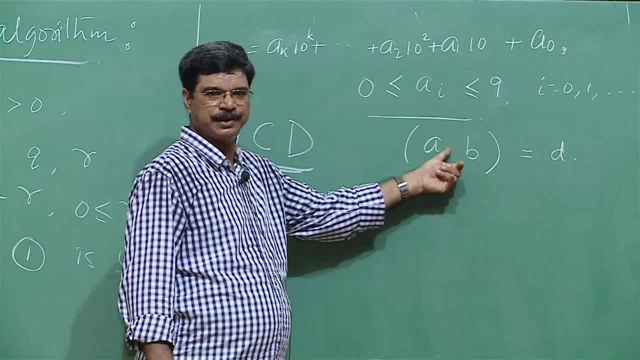 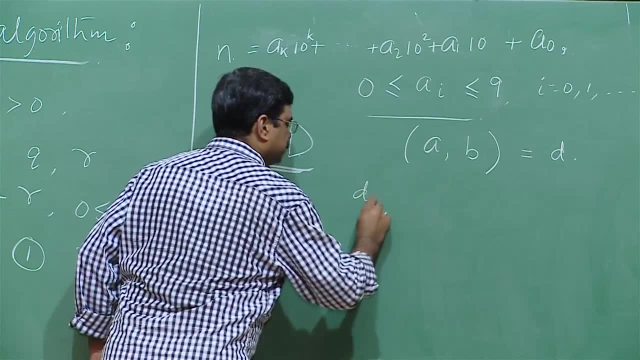 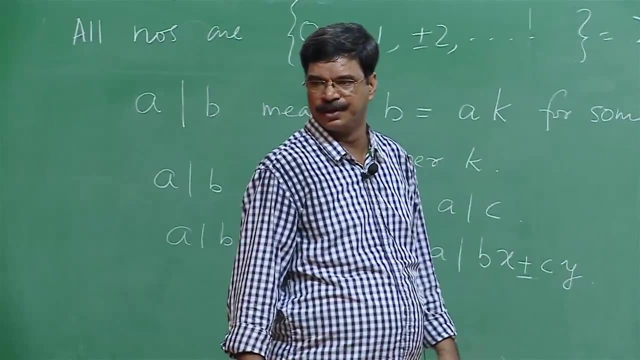 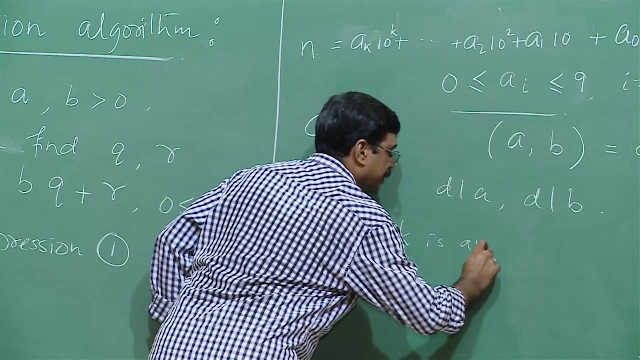 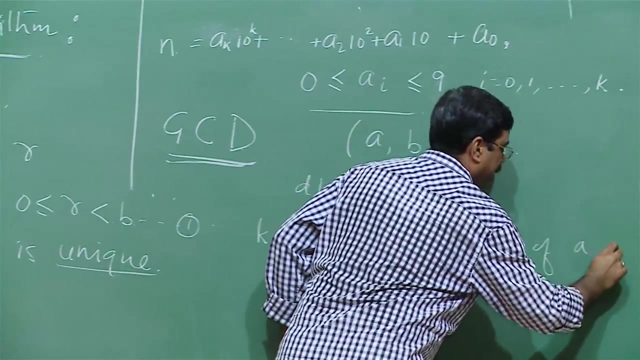 means if you take any other divisor of A and B, ok, Then D is divides that, For D divides A, D divides B. So d is first a common divisor, Ok. And if K is any other divisor Of A, Of A and B, 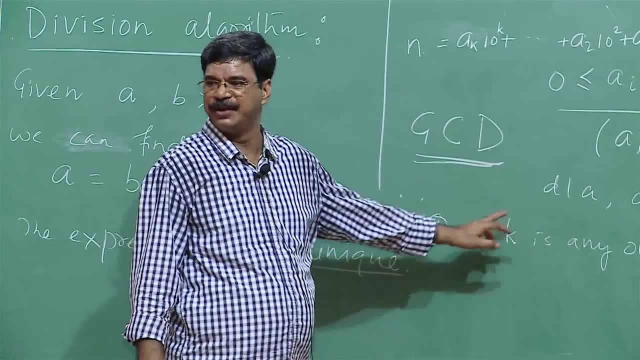 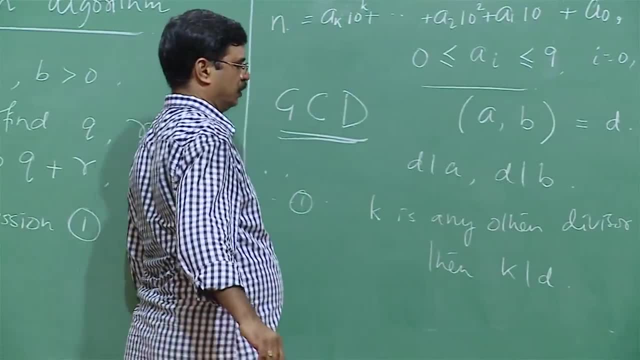 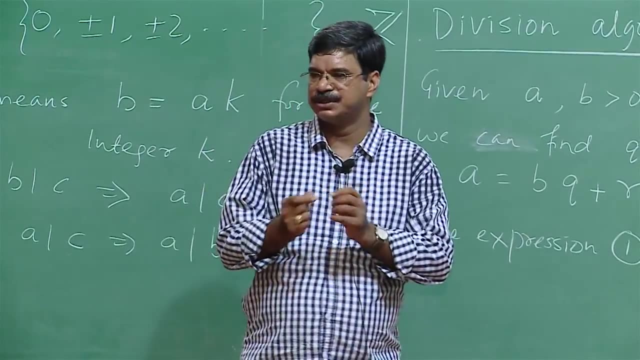 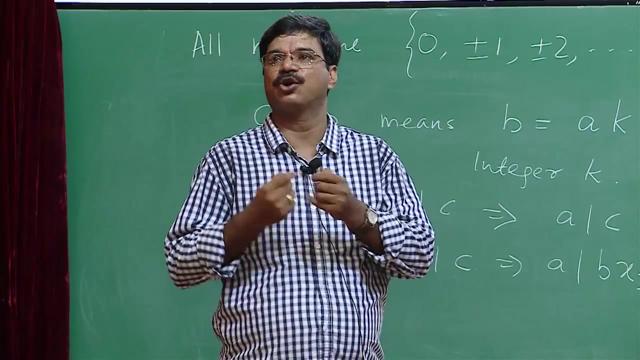 Then K will. can divide a common divisor. Ok, k will divide d. How to find For small numbers we can find the. we can factorize the number a and look at the factors of b. look at what are the common factors of a and b and choose. 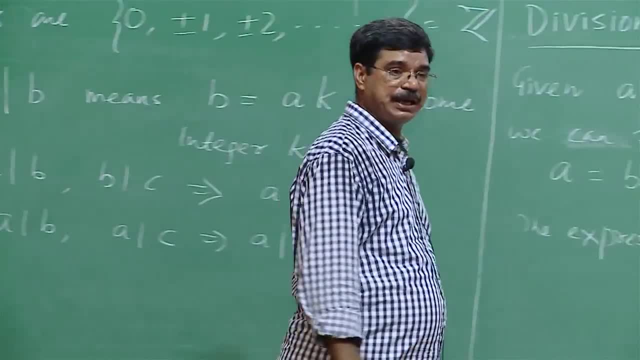 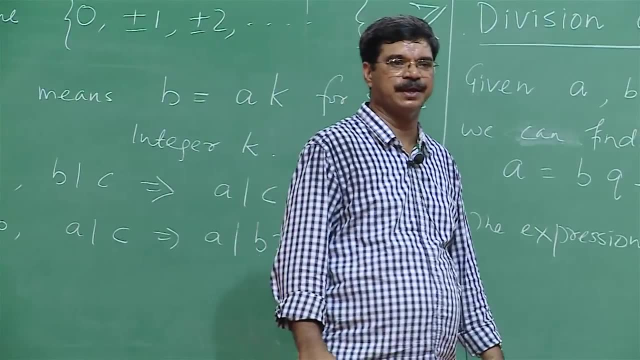 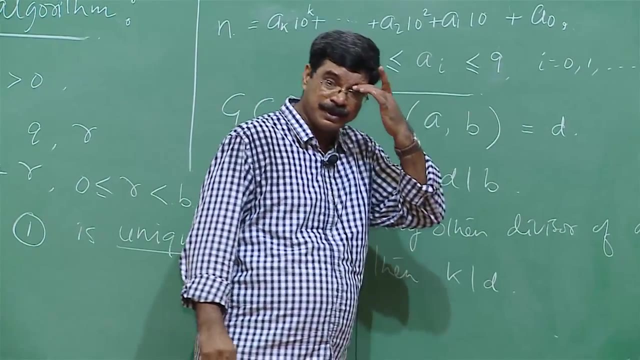 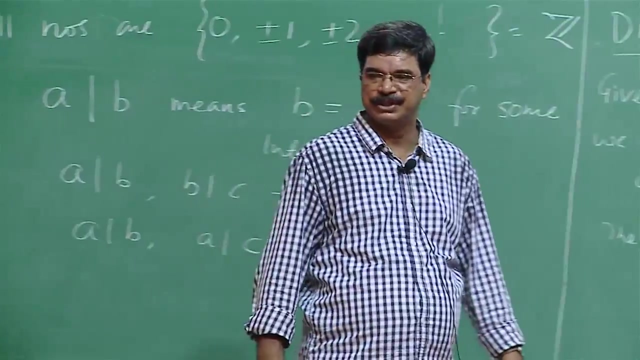 the one which is the largest, But if the numbers are very large, factoring takes time. Factoring is not so easy. Therefore, what to do at that time? And here again, the Greeks have told us how to find the GCD. It is one of the most novel ideas. 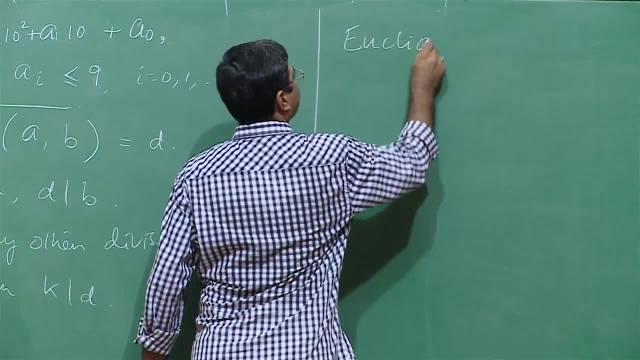 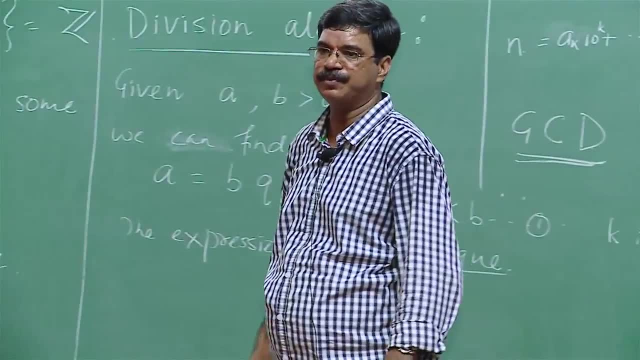 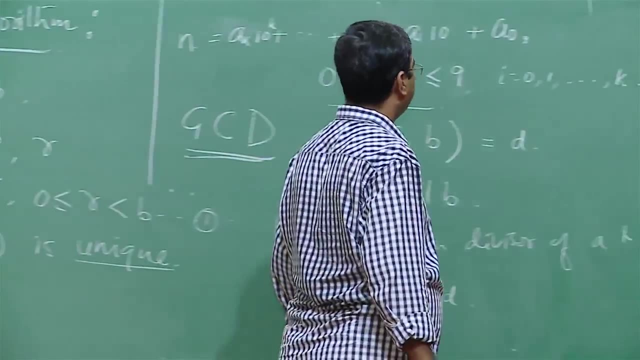 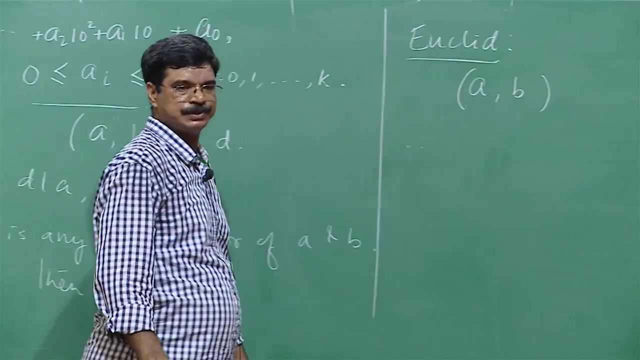 Euclid around 300 BC. he gave us a method, algorithm, Euclid's algorithm- how to find the GCD of two numbers- however they are large- in a very easy way And his method can be written as a and b. The GCD of a and b is same, as suppose a is bigger than b there. 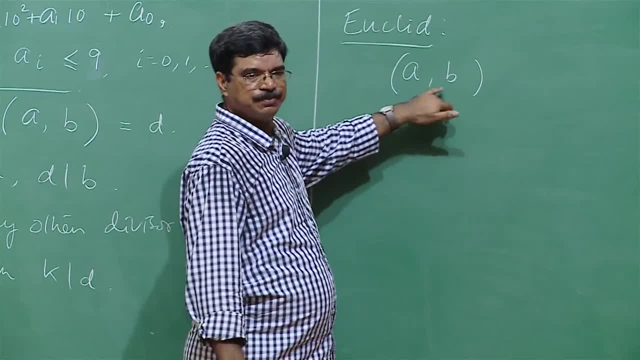 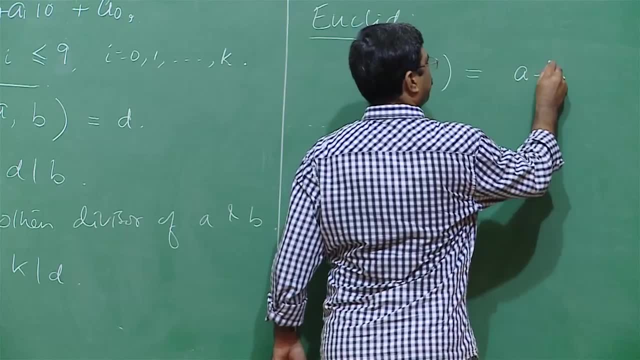 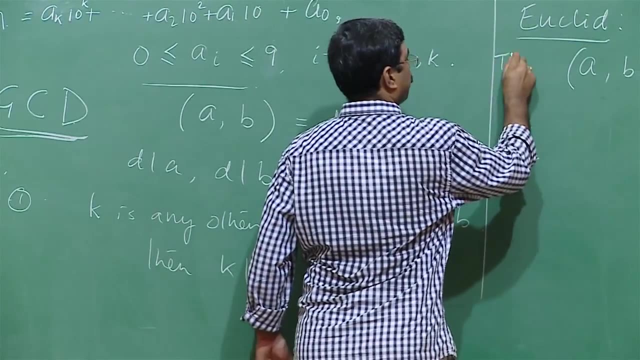 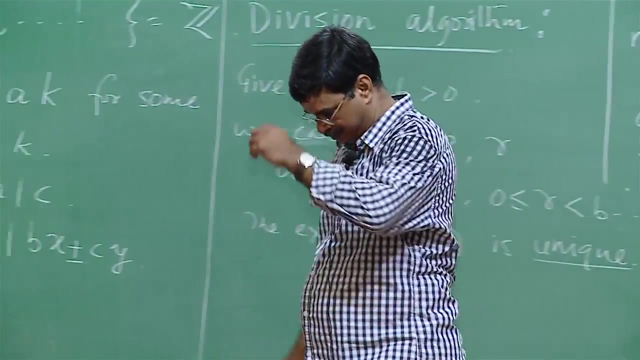 are two numbers So different, a is bigger than b, then the GCD of a and b is same as the GCD of a minus b and b. So this is- you can call it as a theorem And in mathematics you know- proof. 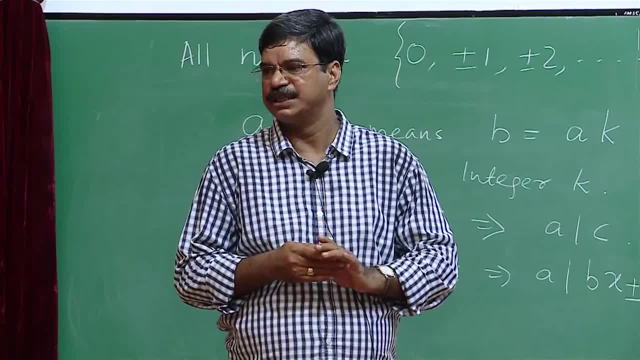 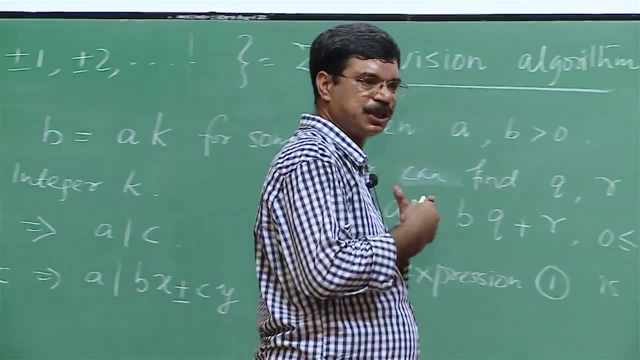 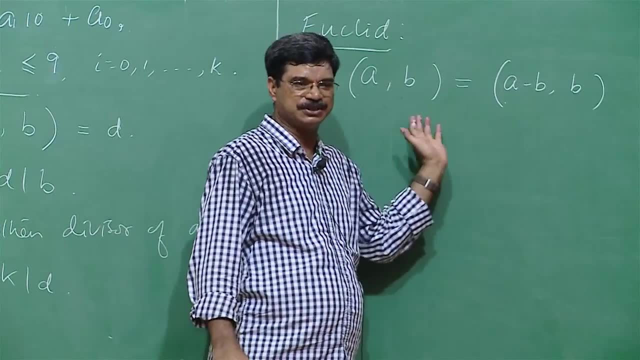 unless you prove a statement, it cannot be called as a theorem. Okay, Near examples do not prove a statement. Okay, They are just illustrations. So sometimes it is nice to show students what a proof means, how to prove such simple statements. Okay, Here is a positive. 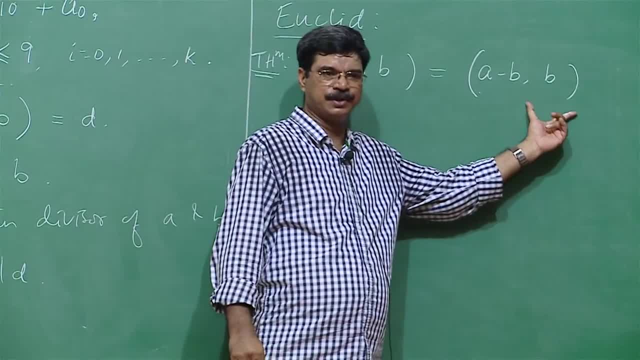 number here is a positive number. You have to show that they are equal. Okay, So take this if… P L 1.. Okay, P L 2.. P L 2.. P L 3.. 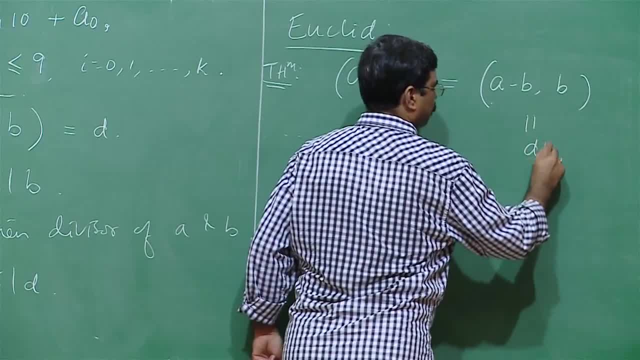 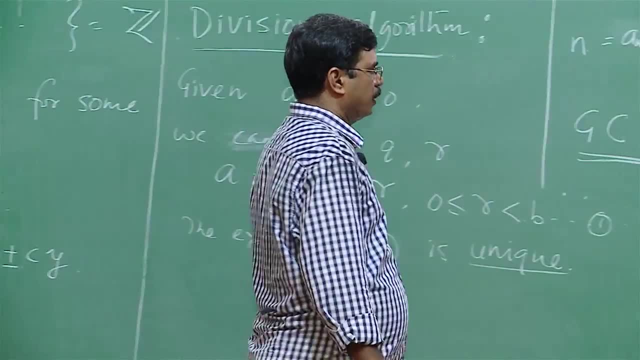 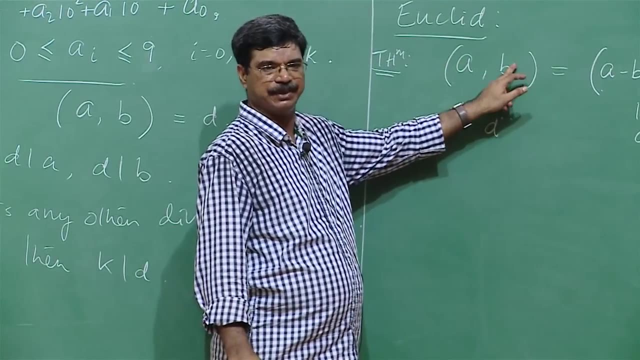 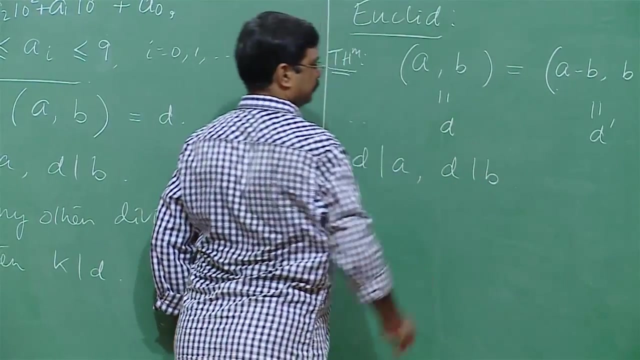 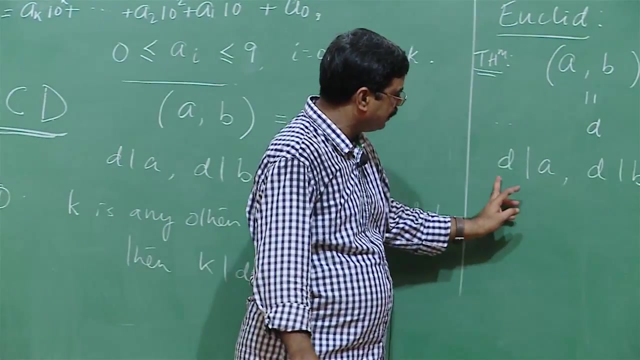 P L 4. equal to D. and suppose this is equal to D prime, Since D is the GCD of A and B. D divides A, D divides B by definition. So D divides A, D divides B. Now, D divides A and D divides. 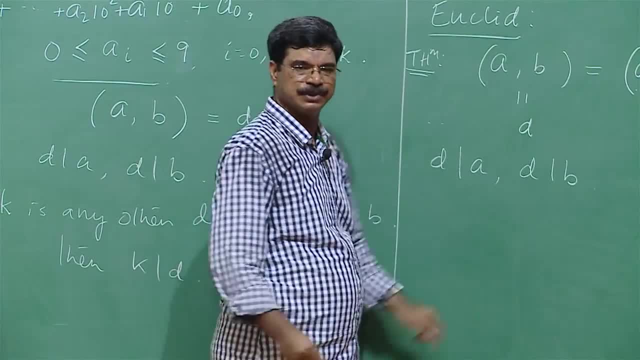 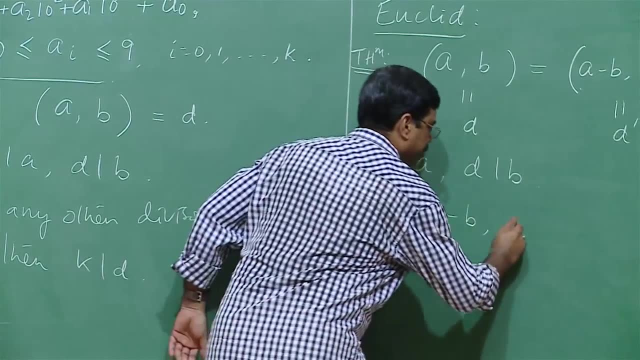 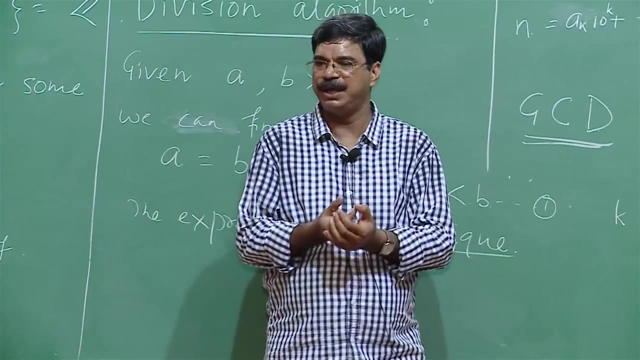 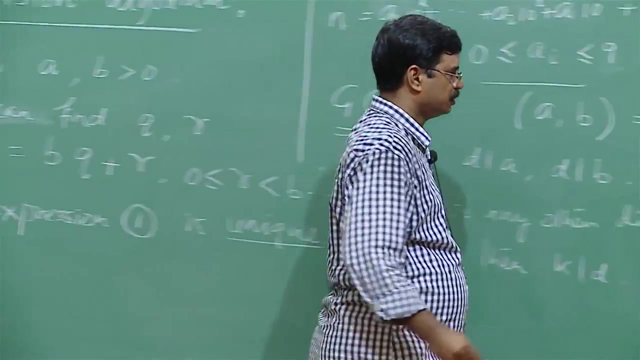 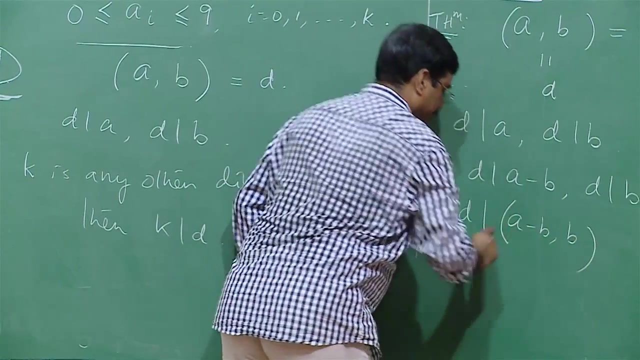 B means D divides A minus B. So this implies D divides A minus B and this statement is: D divides B. Now, if D divides A minus B and D divides B, D will divide the GCD of A minus B and B, right? So therefore D divides the GCD of A minus B and B, because D is a common divisor. It. 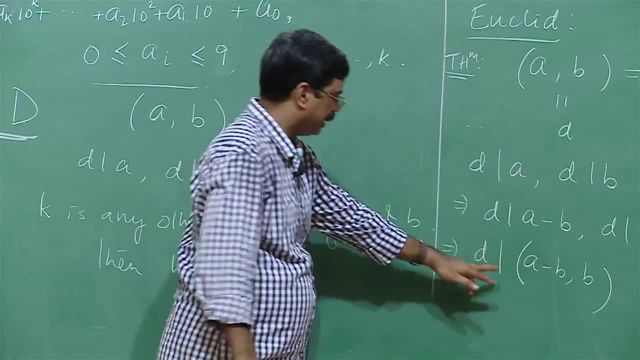 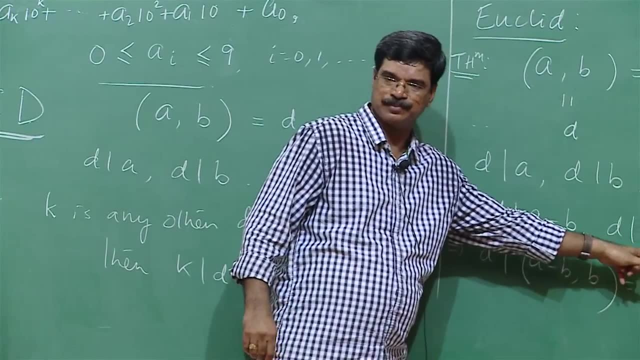 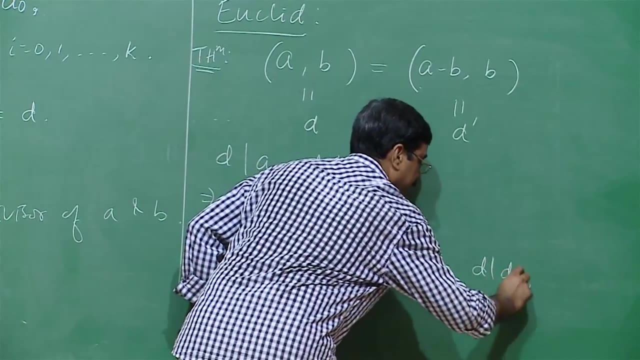 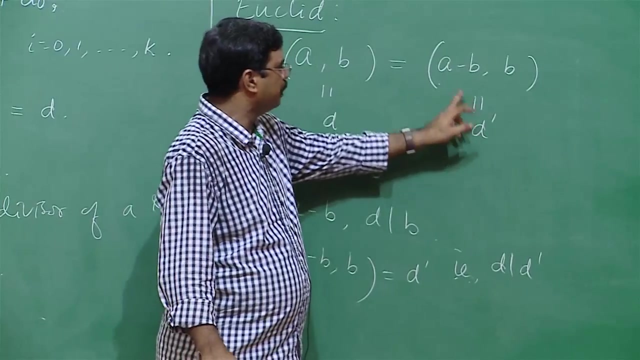 will divide the greatest common divisor And this is nothing but D prime. So D divides D prime. So this we have got. that is IE, that is D divides D prime. Now flip the argument. D prime divides A minus B. because it is a common divisor. GCD means it is first of all, it is a common. 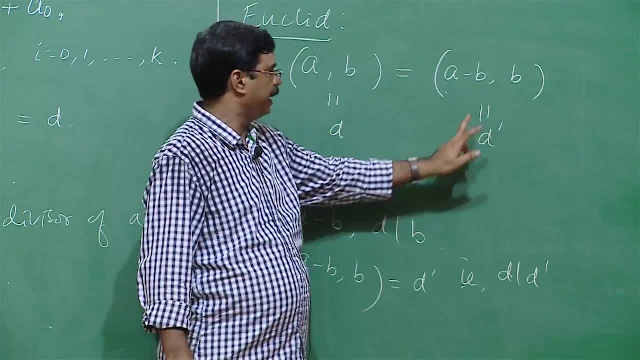 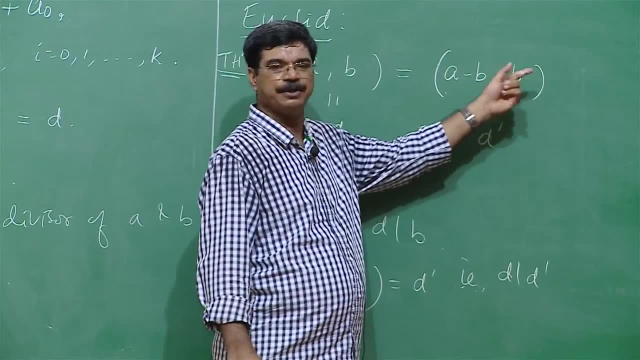 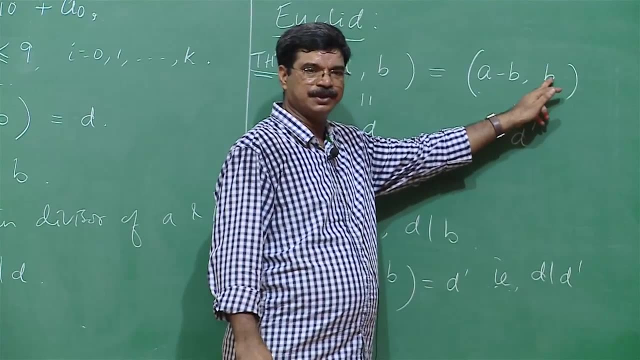 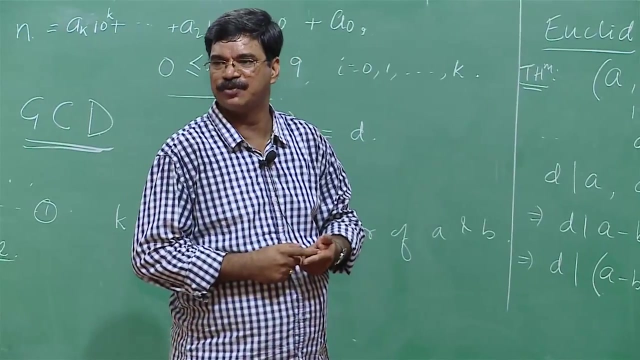 divisor. So D prime divides A minus B and D prime divides B. Therefore, D prime will divide the sum of these two numbers, A minus B plus B, which is A. So D prime divides A and D prime divides B. Therefore, D prime is a common divisor of A and B. And since it is a common divisor of A and B, therefore, 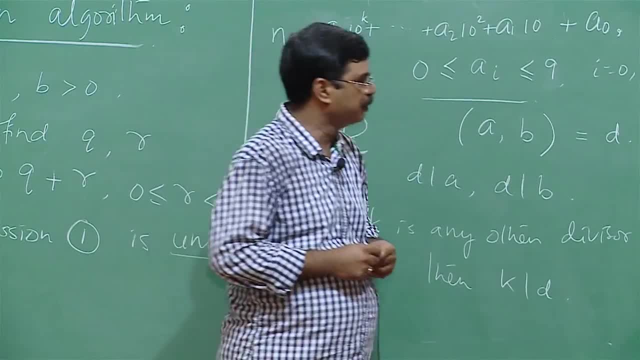 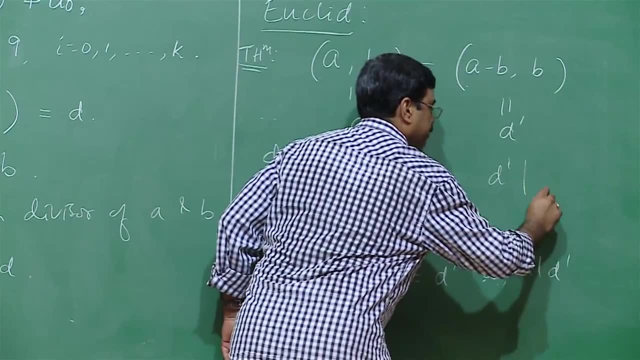 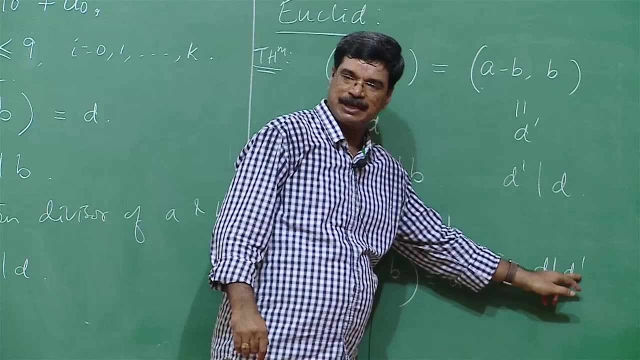 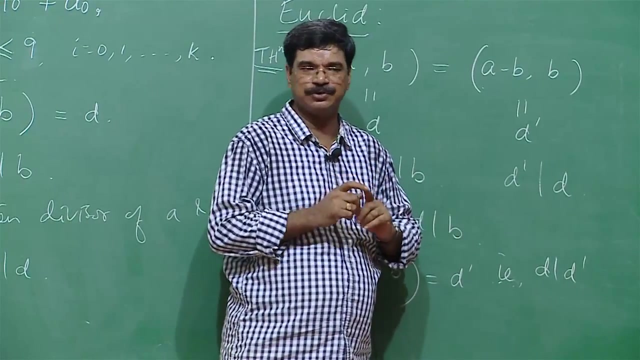 it will divide the greatest common divisor of A and B. Therefore D prime will divide D. ok, So D prime divides D, D prime divides D and D divides D prime. That means D is equal to Plus minus D prime. Right, But since both are positive, they must be equal because we are dealing with integers. 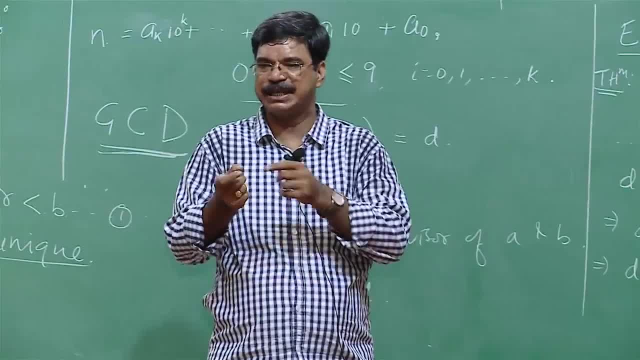 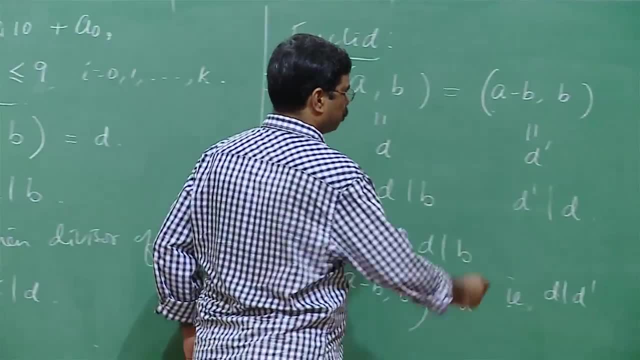 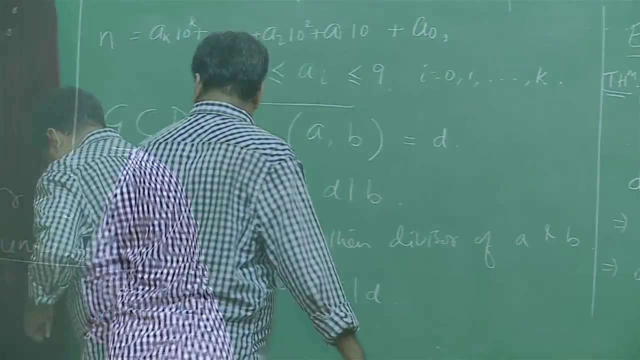 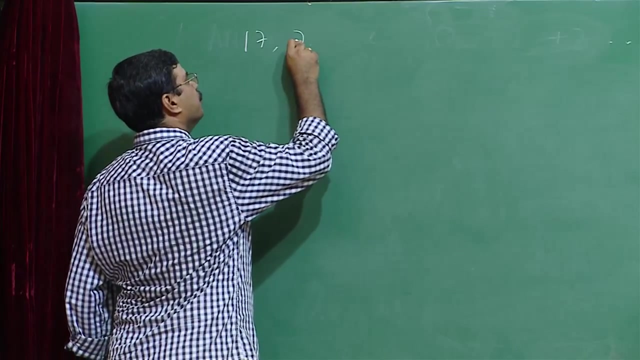 only One integer divides another, the another one divides. this means they can be plus, minus, But since we are dealing with positive integers only, so they must be equal. Therefore, this shows that D, A, B, D is equal to D. okay, So let us take an example, let us our famous 17, and let us say 7.. So 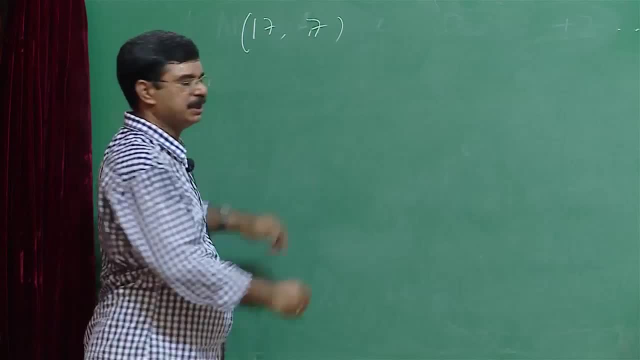 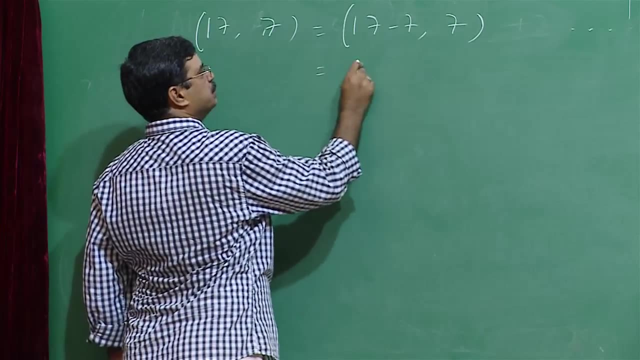 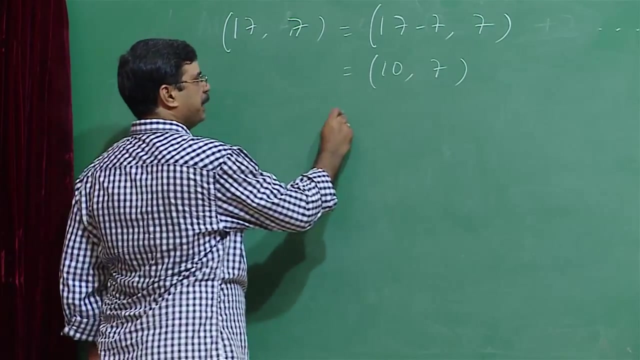 what does it say? 17 and 7? GCD of these two numbers is same as 17 minus 7 and 7.. So this is 10 and 7. we can still subtract one more time, So this is same as 10 minus 7 and 7. 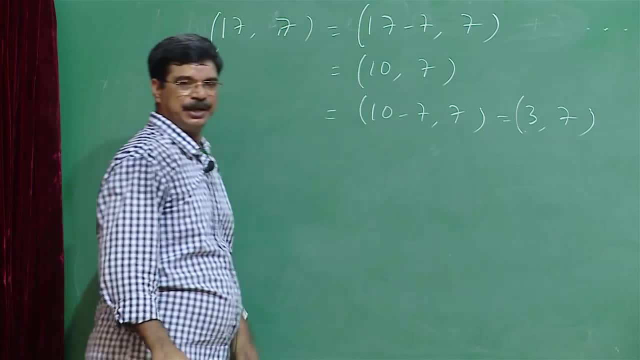 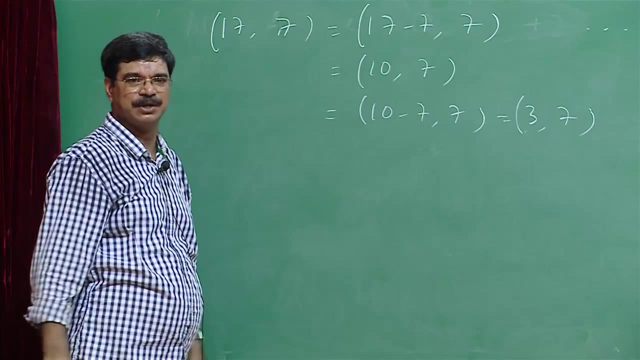 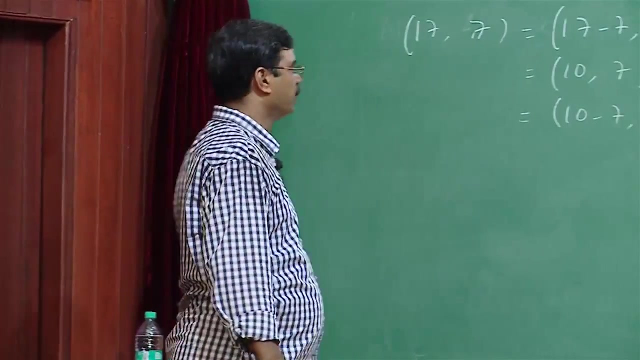 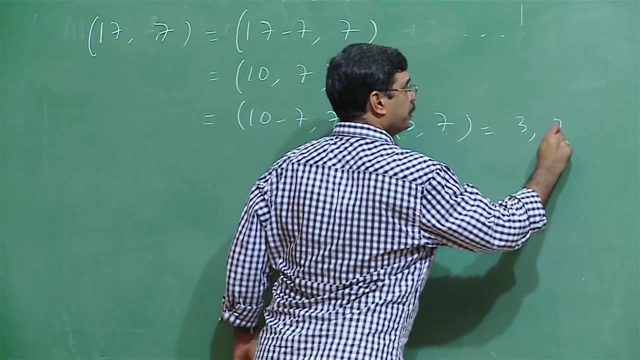 which is 3, 7, but I mean, this is just an example. we can take large numbers. subtraction is easy rather than factorization. So we can subtract two numbers quite efficiently, quite easily, whereas factoring numbers is very difficult. okay, So 3 and 7. if you want, you can further do it: 3, 7 minus 3, which is 3 and 4 further you. 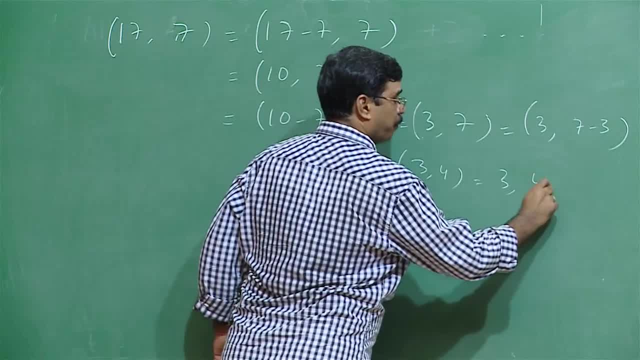 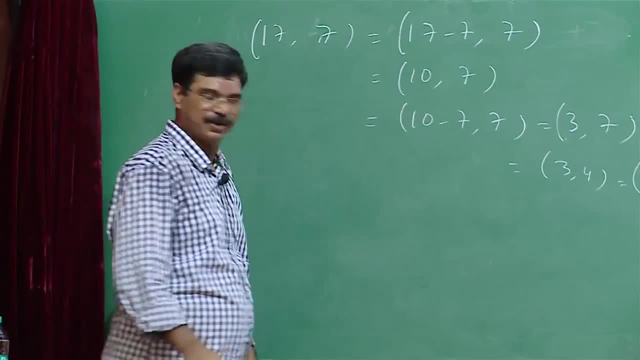 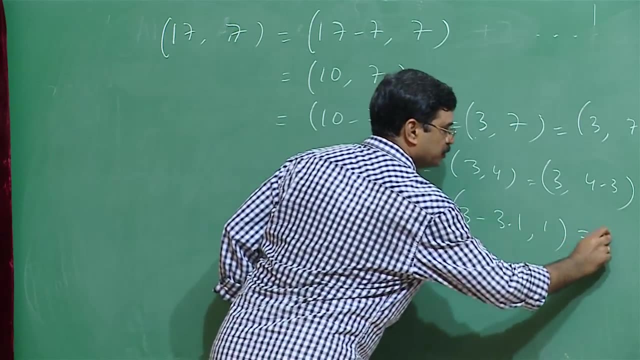 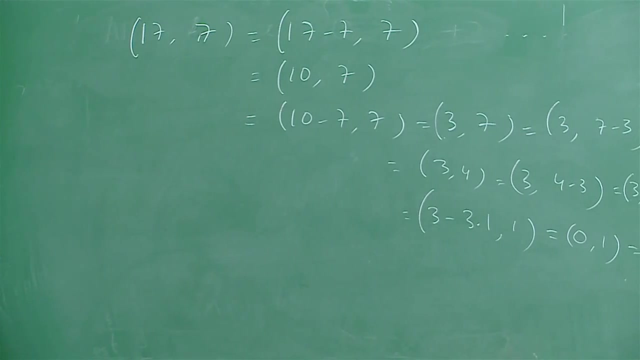 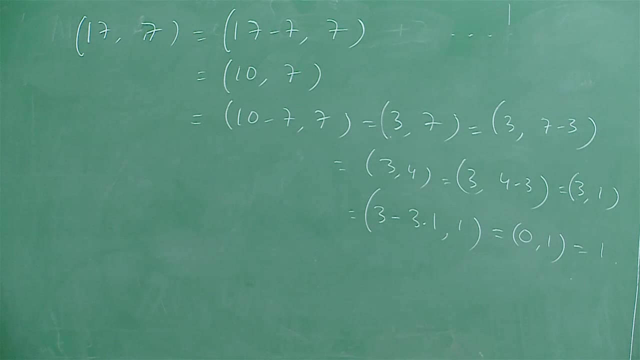 can do it: 3, 4 minus 3, which is 3 and 1. if you want, you can further do it, okay. So this is 3 minus 3 times 1 and 1, this is 0.. Okay, Where is division algorithm coming here? Please think about for a minute. where is division? 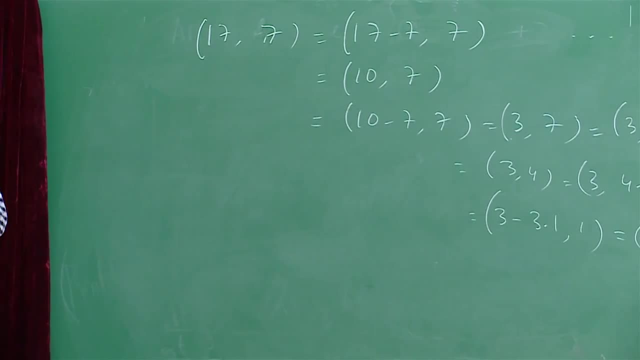 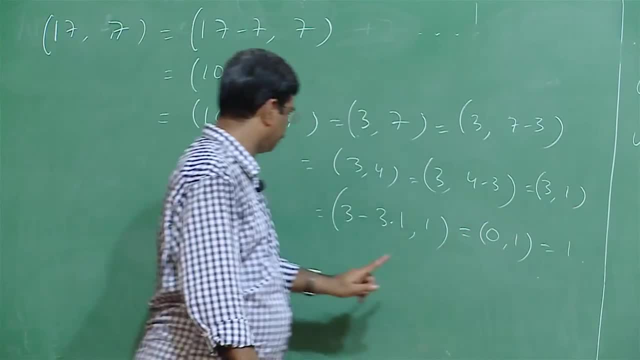 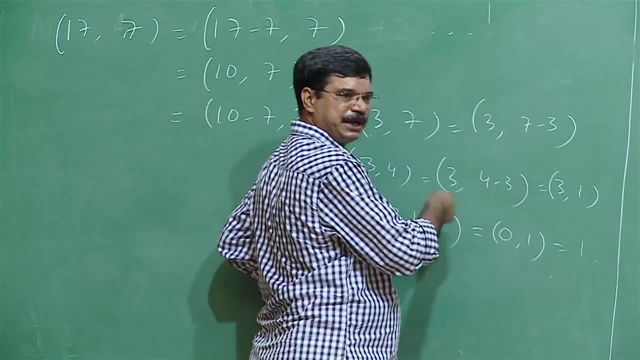 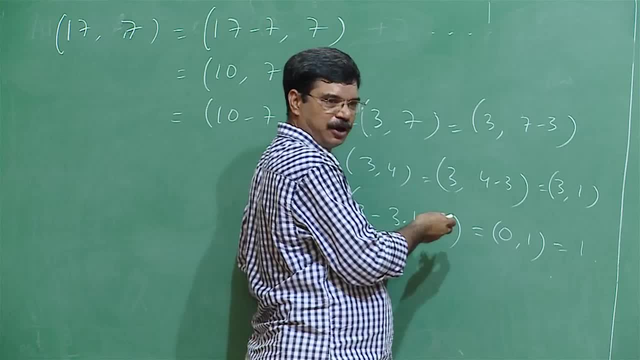 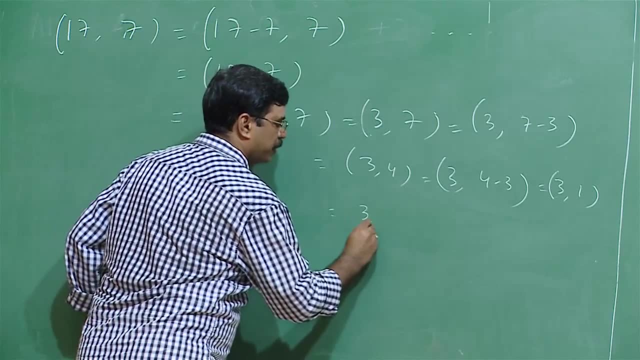 comma 1, again 3.. So 2, 1 I have got. if you want, I can do it like this- 3 comma 1 right here. So 3 minus 1 comma 1, which is 2, 1. 1. 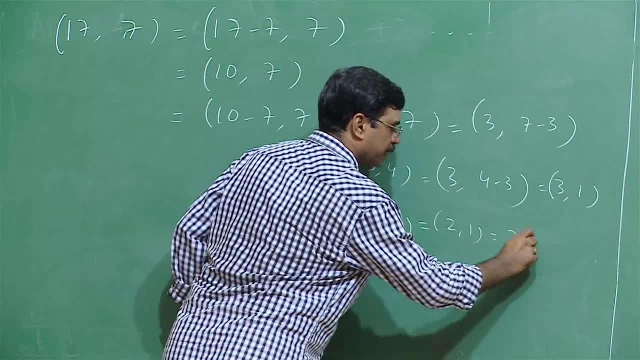 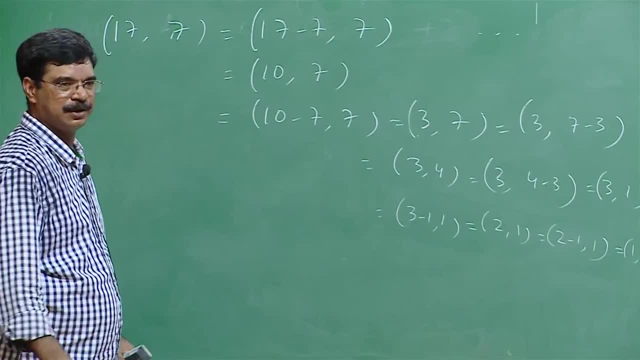 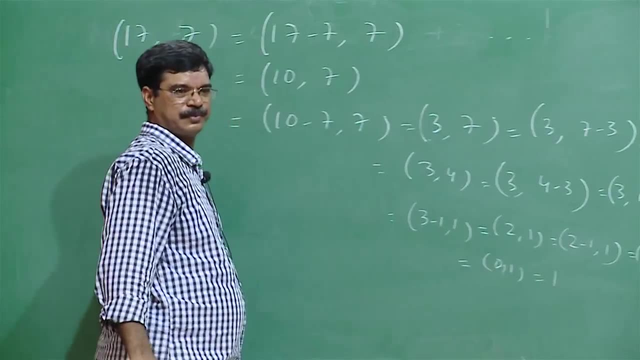 1. Again 2 minus 1.. 1. 2 minus 1 comma 1, which is 1 comma 1. I can subtract one more time: 0, 1. Okay, or you can say 0 comma 1, 1.. 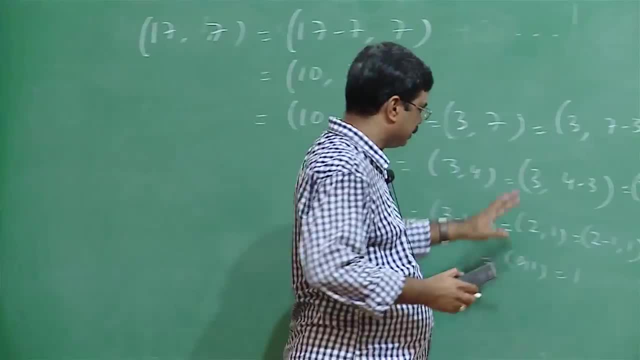 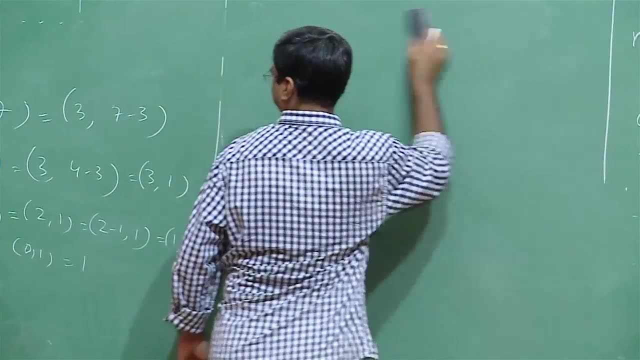 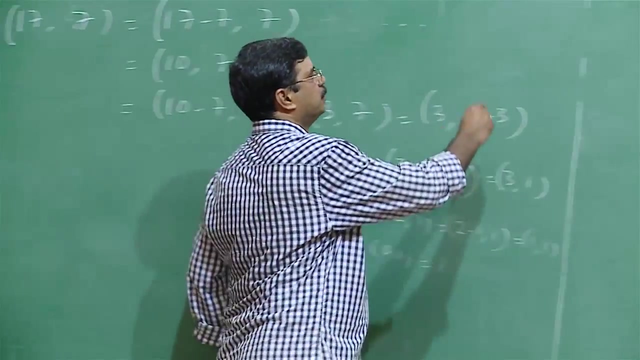 Okay, So you see this division algorithm we are. what we are doing is division algorithm precisely: Yes, Yes, Yes, Yes, Yes. So 17, we are dividing it by 7.. 17.. 17 is 7 into. 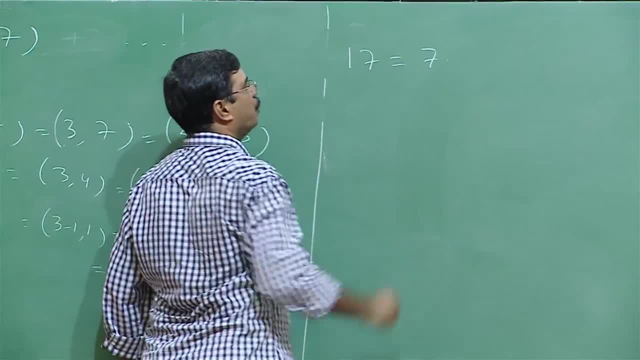 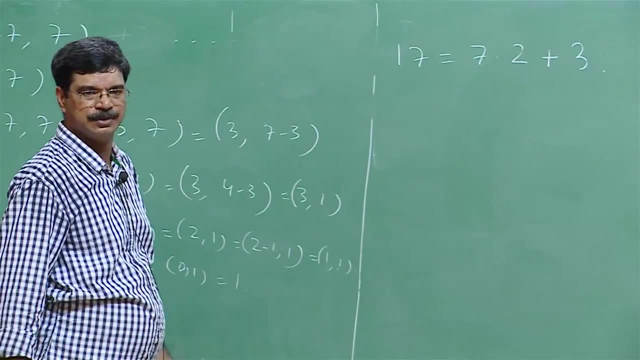 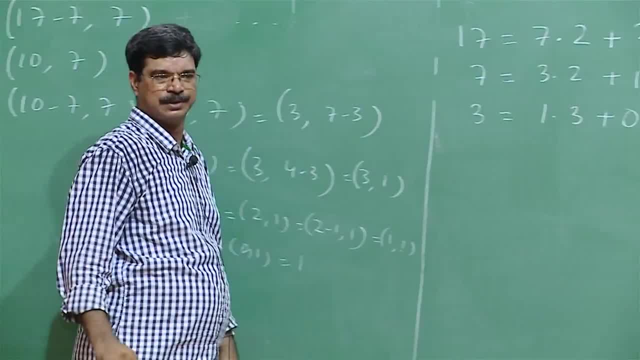 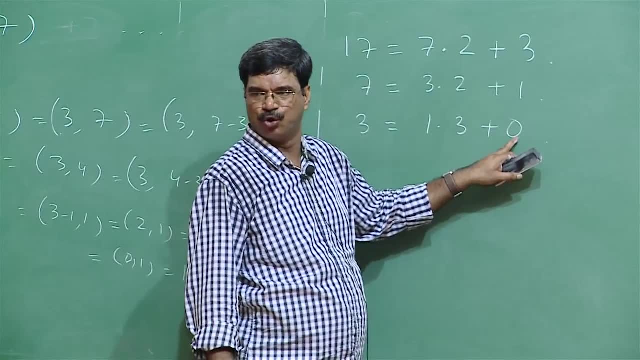 2., 2., 2., 2., 2., 0.. 0.. 1. 0. 3. 1. 3 is equal to…. 2., 2., 2., 3. 3 is equal to this one times 3 plus 0.. 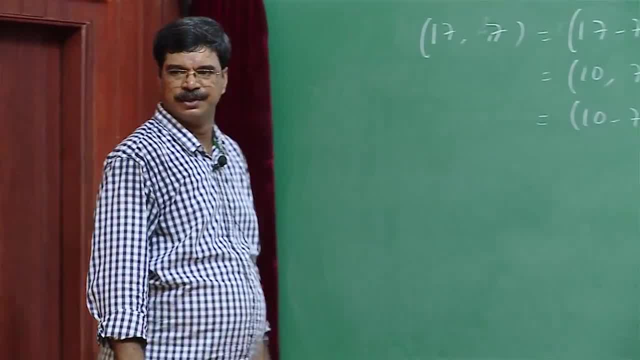 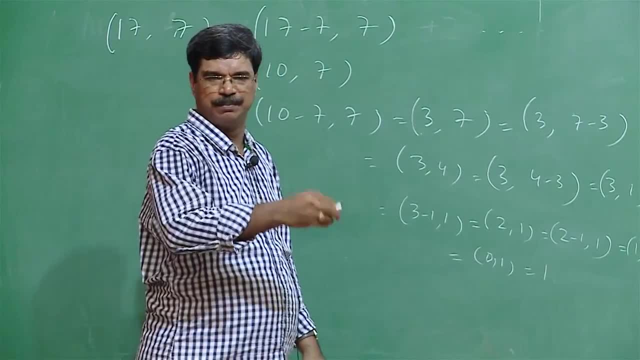 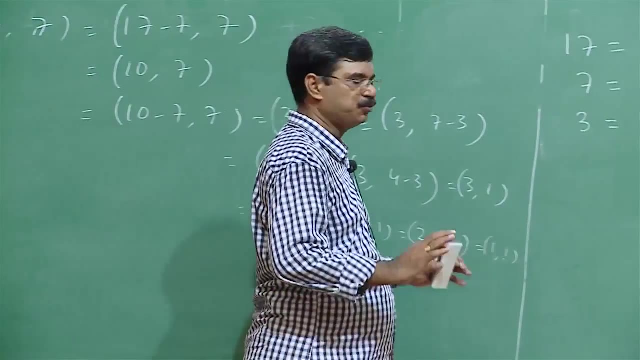 This is what, precisely, we have done. You can write it in symbols a, b, so a is equal to b1, q plus r1 and b. divide r1 by r1. keep doing that. that is what is called Euclid's algorithm to find the GCD of two numbers. 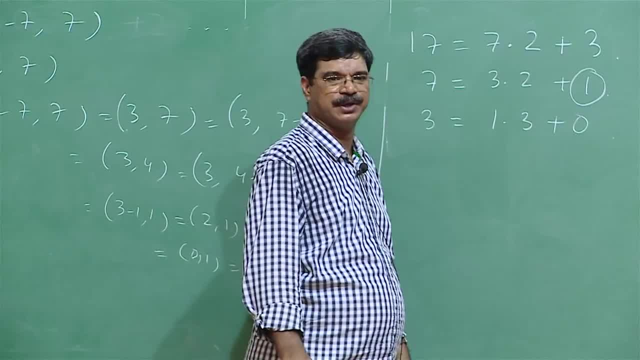 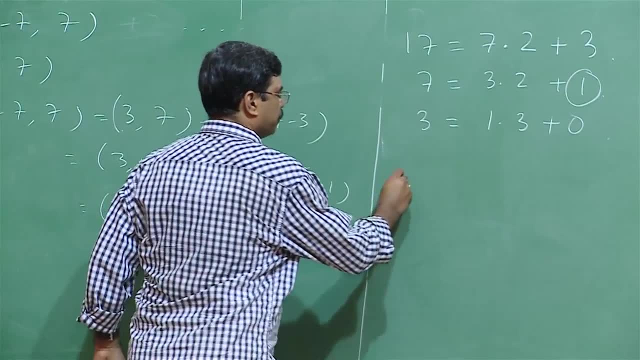 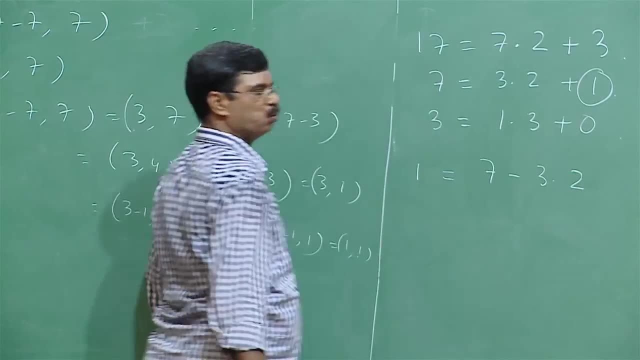 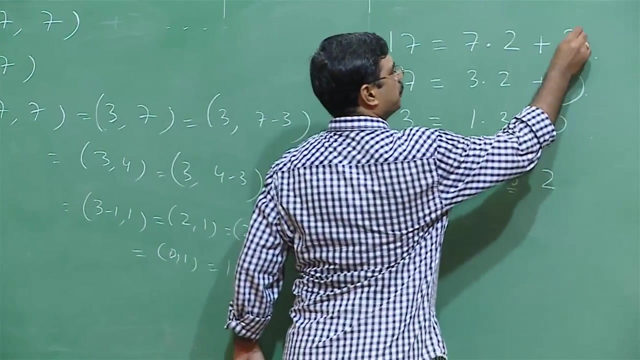 As a byproduct, we get something else. For example here: 1. 1, which is the GCD of two numbers. so 1 is nothing but 7 minus 3 times 2.. We are working backwards, okay. Now this 3 is coming from here, okay. 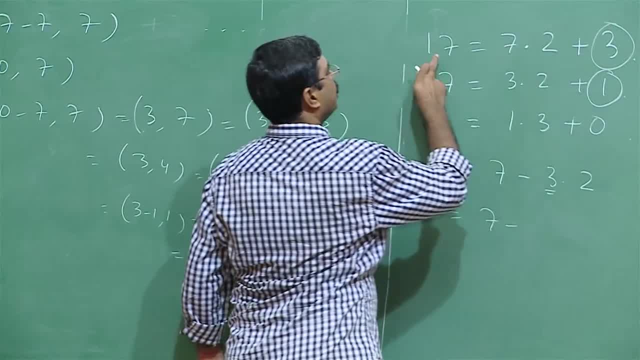 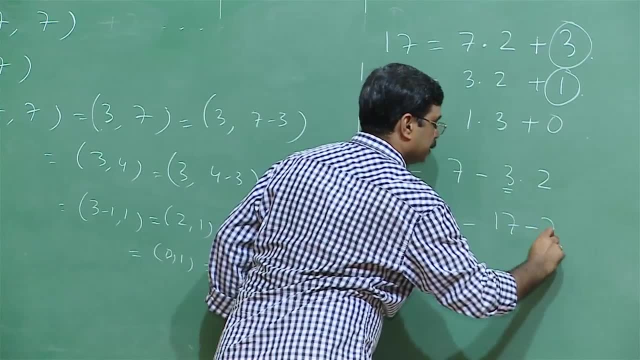 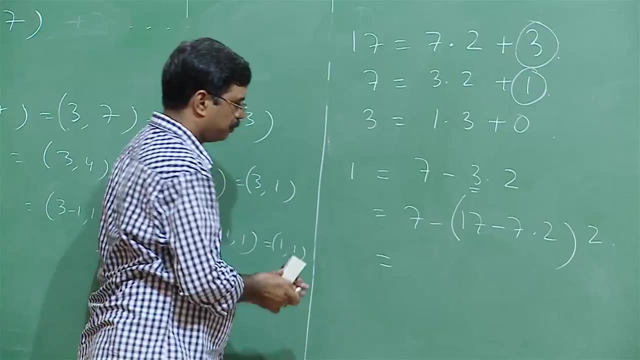 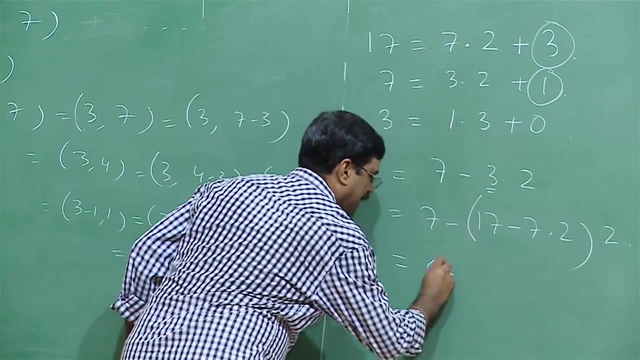 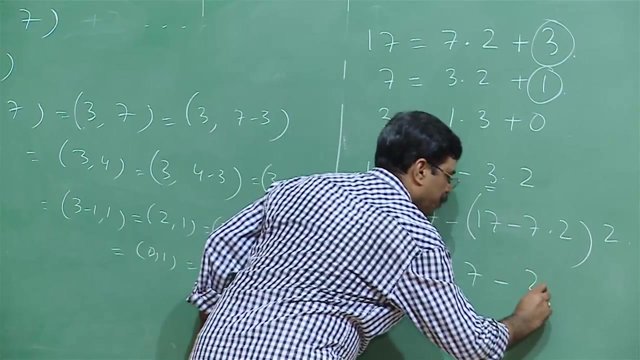 So this is 7 minus 3, is 17 minus 7 times 2.. 17 minus 7 times 2 times 2.. So this is how much 1 times 7, 4 times 7.. So this is 5 times 7 minus 2 times 17, 2 times 17.. 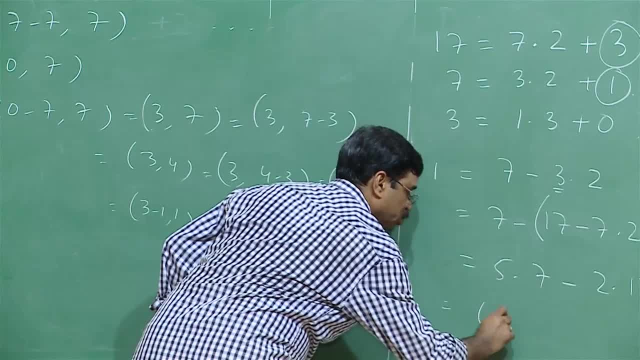 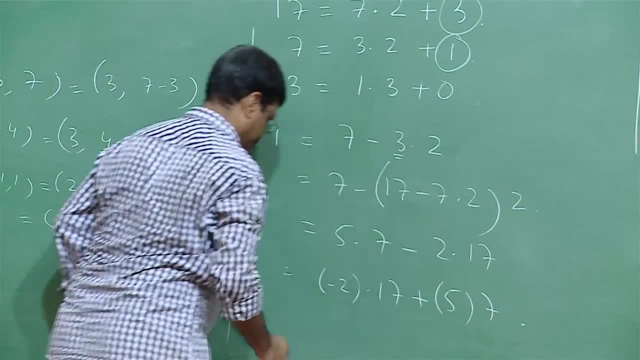 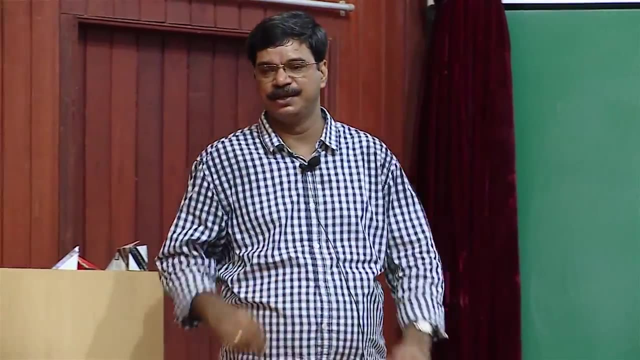 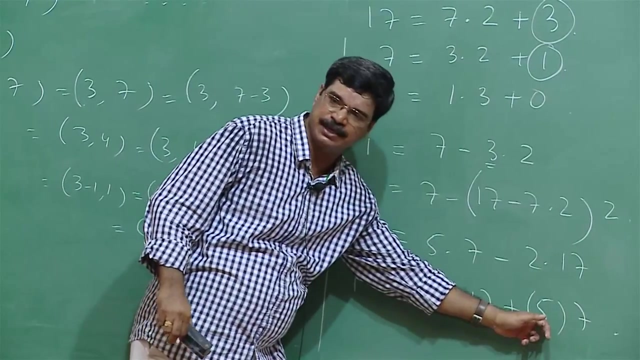 Okay, This is same as writing minus 2 times 17, plus 5 times 7, which is equal to 1.. So what did we get? GCD. given any two numbers we are able to find out integers x and y, such that the GCD is: 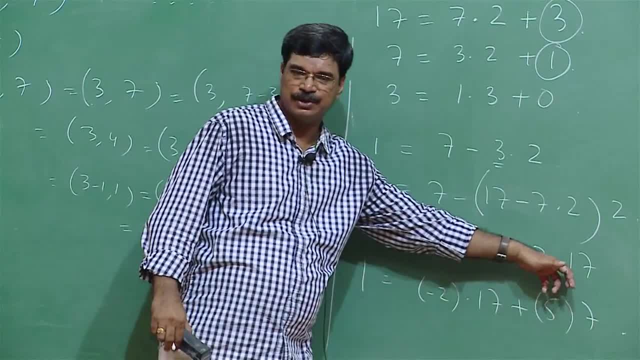 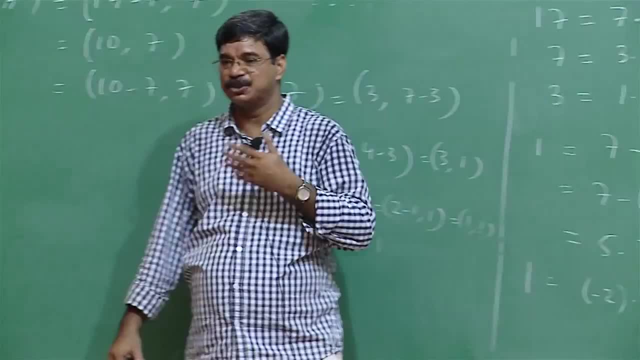 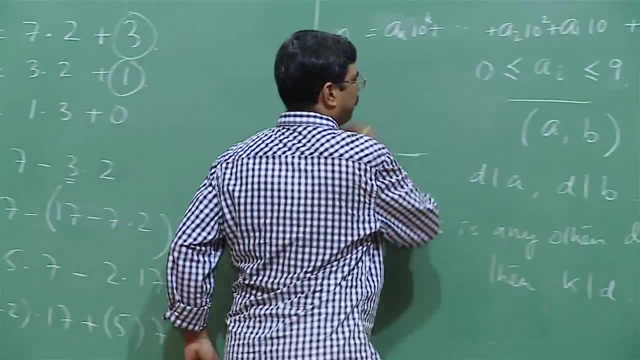 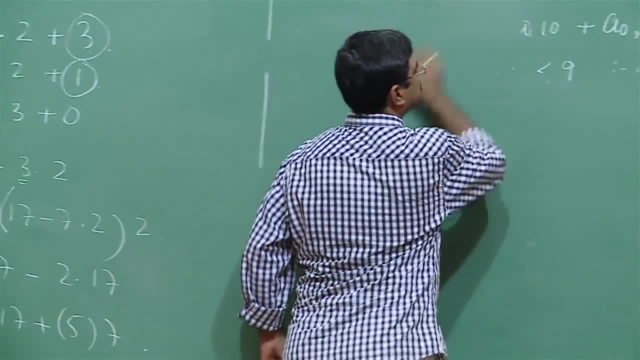 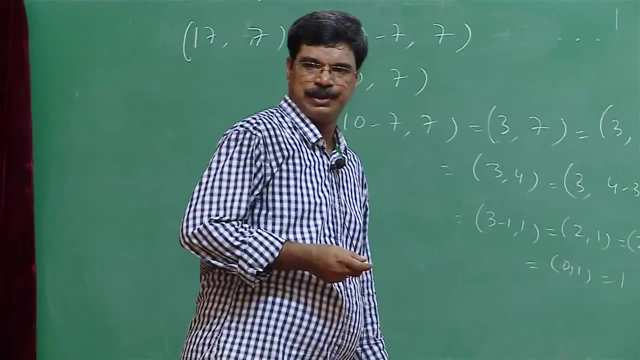 b. Okay, So very important and very beautiful thing. See how many things the Greeks have left to us. Yes, GCD of negative integers or GCD of positive integers? Yeah, So GCD. what is GCD of negative integers? GCD of, let us say, minus 4 and 12.. 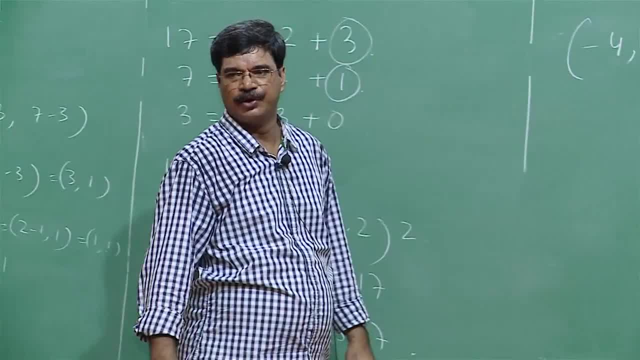 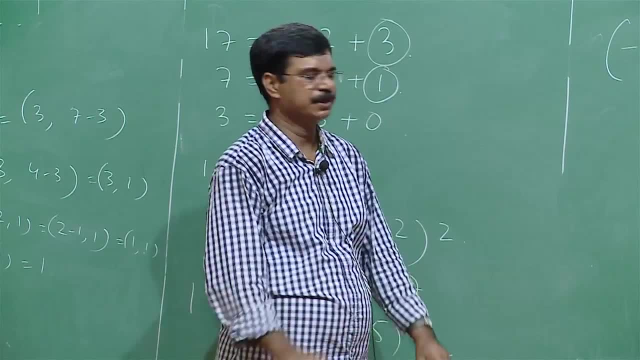 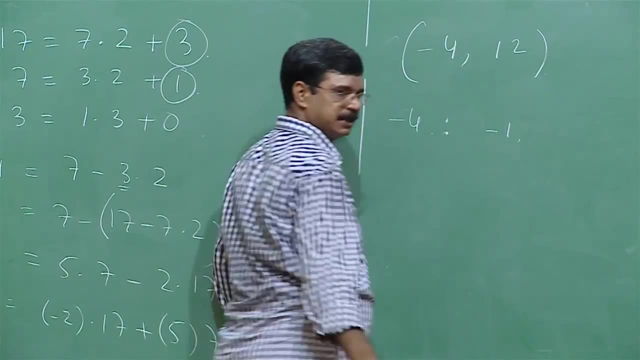 Okay, Something like this: Okay, So when we say GCD, we always mean the positive divisors. Okay, So, minus 4, the factors of divisors of minus 4. you know, you can say that minus 1 is a factor, 1 is a factor. 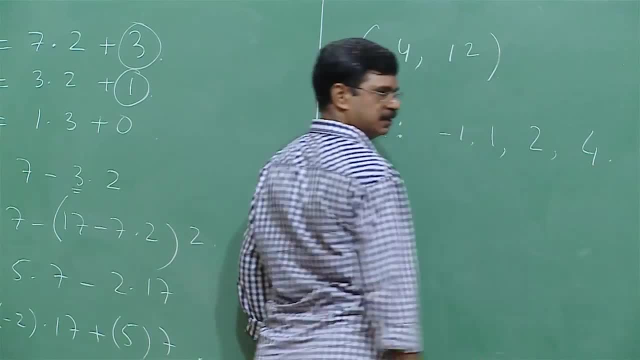 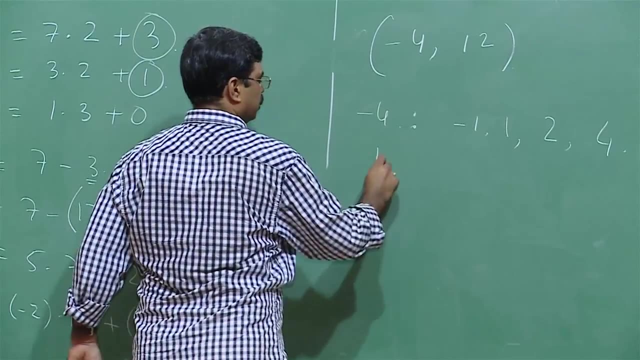 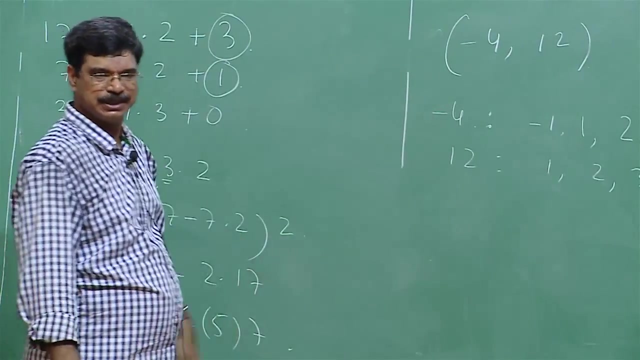 2 is a factor, 4 is a factor. 4 is a factor. We will only look at the positive divisors of this number and for 12,, 1,, 2,, 3,, 4, and therefore, since 4 is the greatest, so we will say that this is 4.. 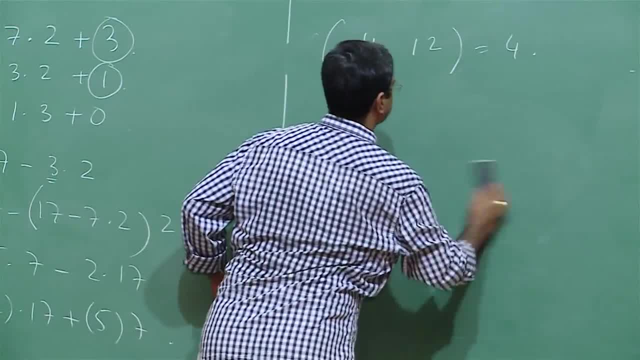 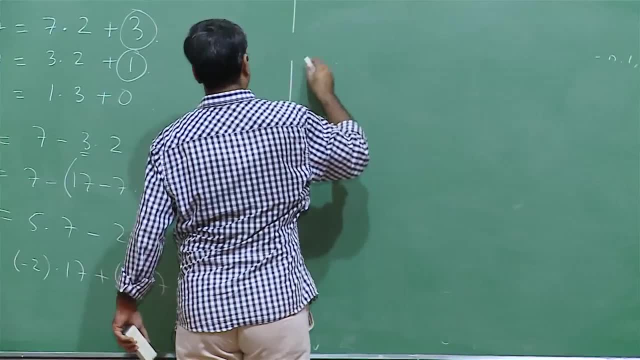 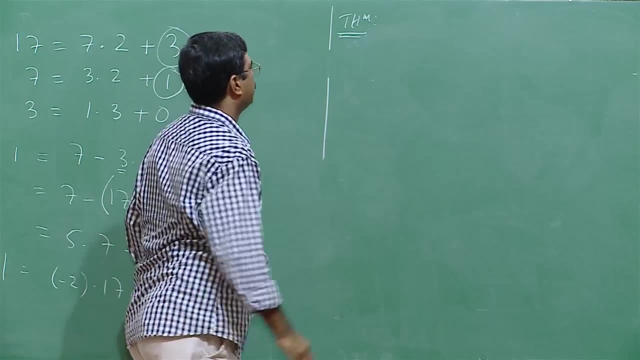 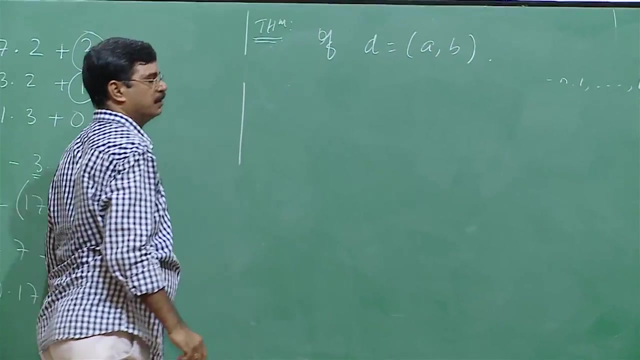 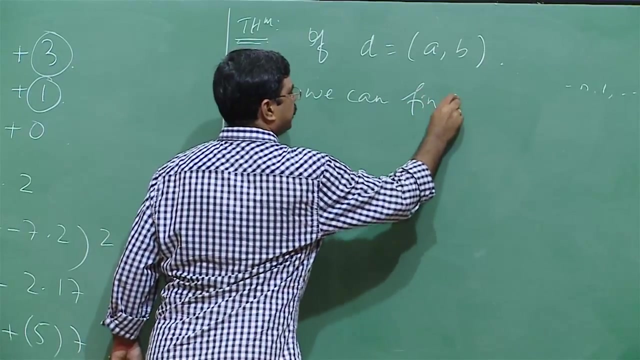 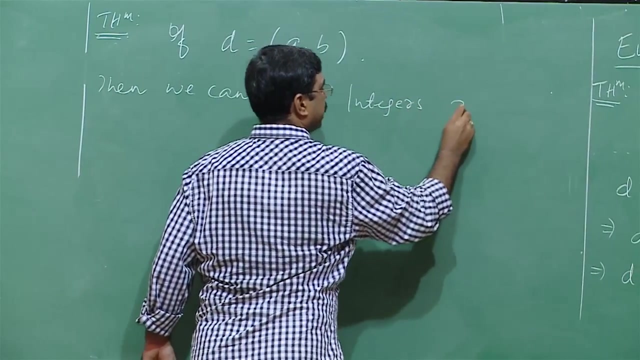 Okay, So, yeah, Yeah, Therefore, Yeah, So we can. We can write it as so. we have a theorem that if D is the GCD of AB, then we can find integers X and Y. Okay, So we can write it as so. we have a theorem that if D is the GCD of AB, then we can find. 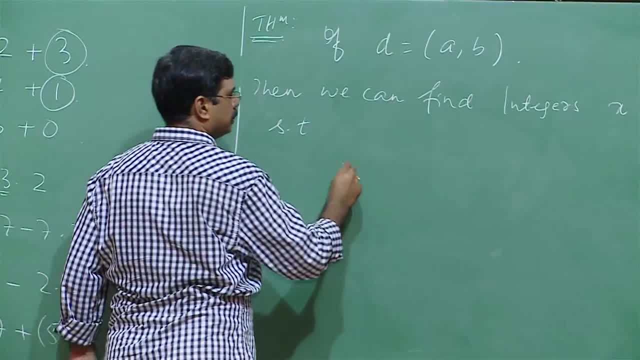 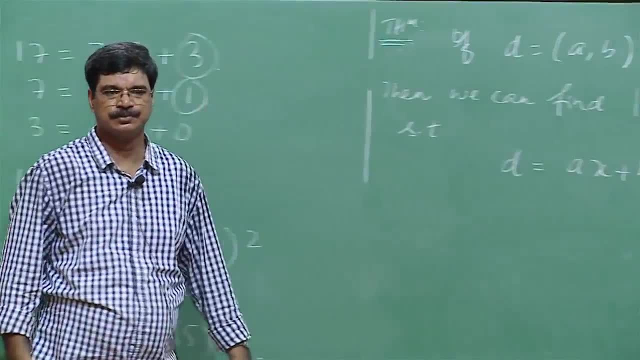 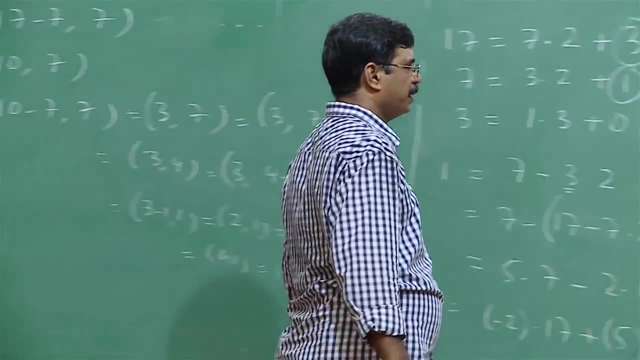 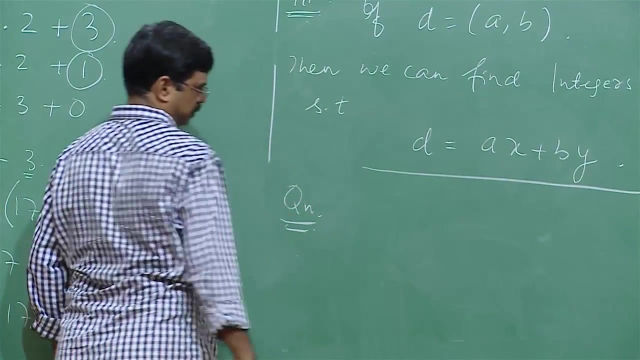 integers X and Y. Okay, Such that D is equal to a times x plus b times y. Yes, Okay, So GCD can always be written as a linear combination of a and b. Now Let me ask you a question. Suppose I give you an equation. 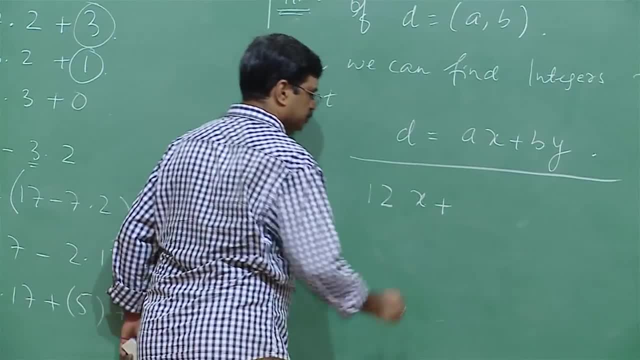 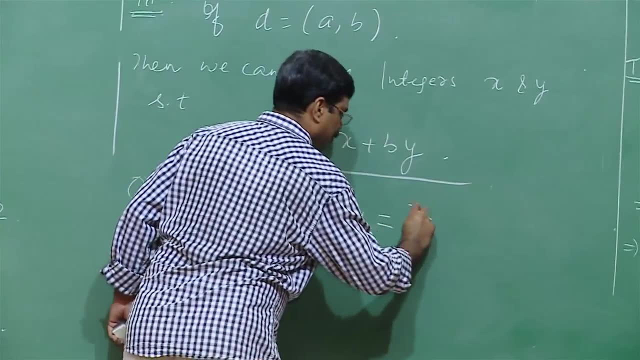 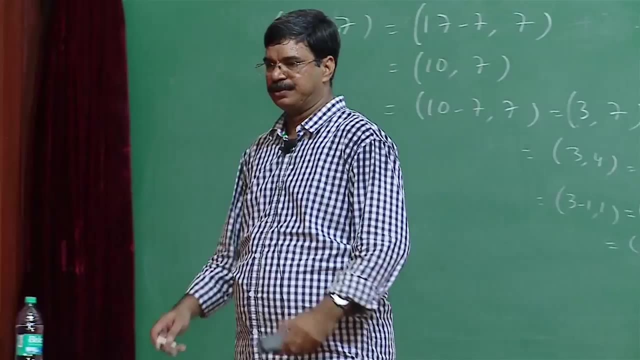 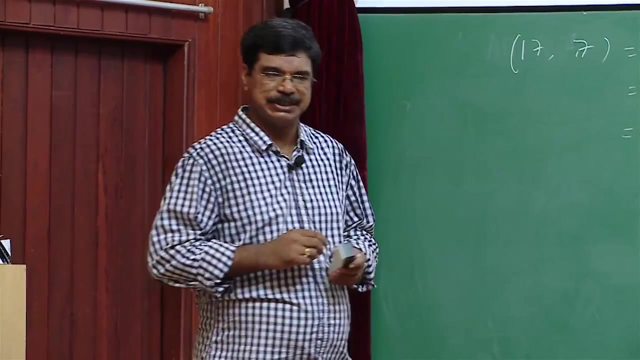 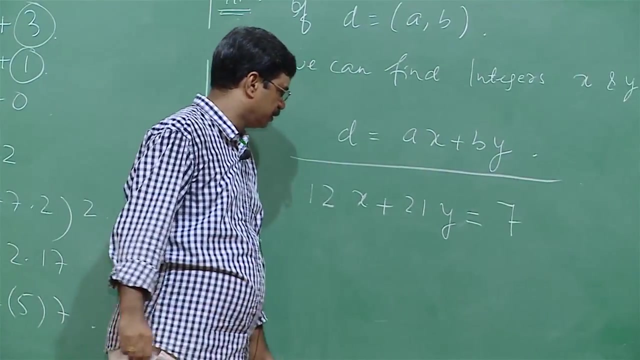 12x, 1x, 21 plus 21y is equal to 7.. Does it have a solution? Can we find any x and y such that this is satisfied? No, I am talking. all my numbers are integers. 1 by 3 does not exist. 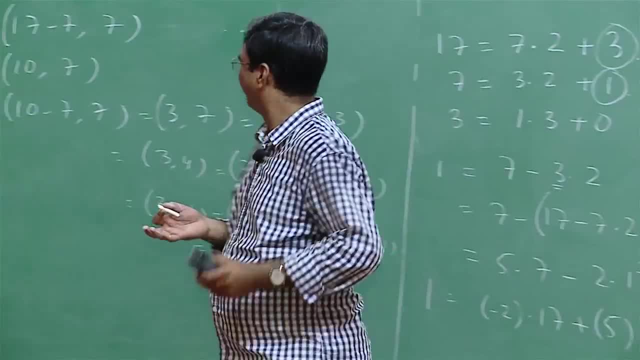 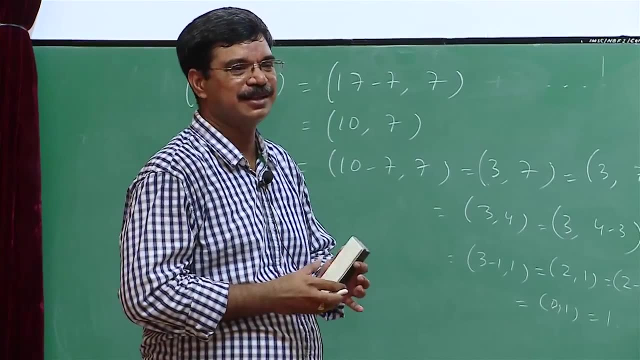 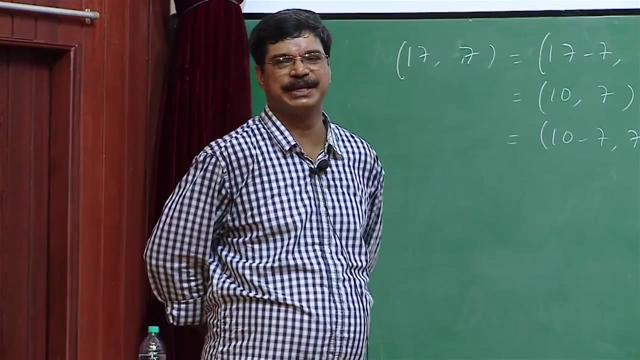 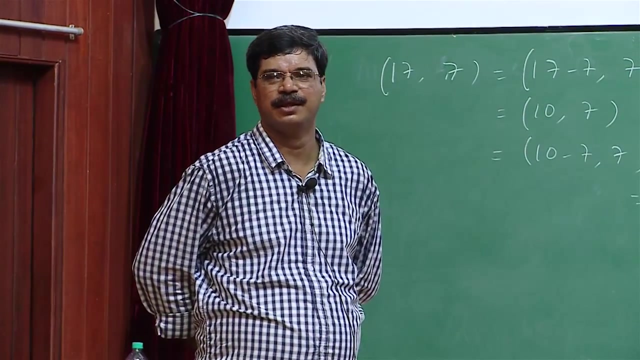 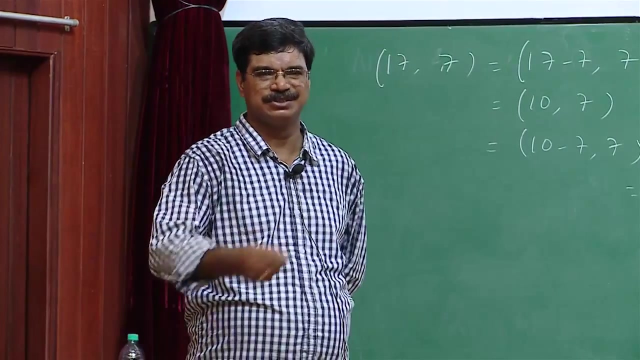 I do not know what is 1 by 3.. I started with that stuff. All the numbers that I know are integers. What is your guess? Infinitely many, Infinitely many. Anyone else? Multiples of No, I just want, since you said infinitely, 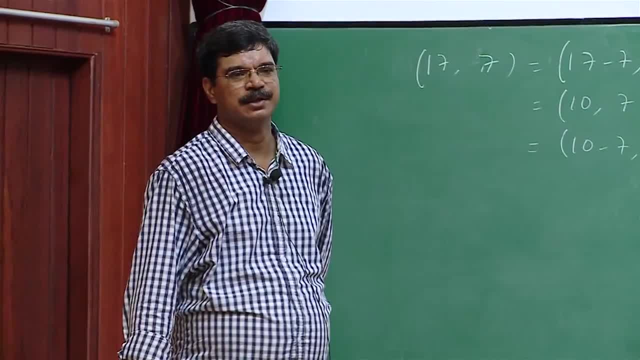 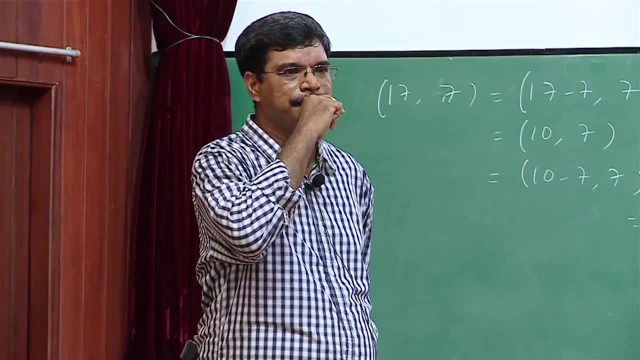 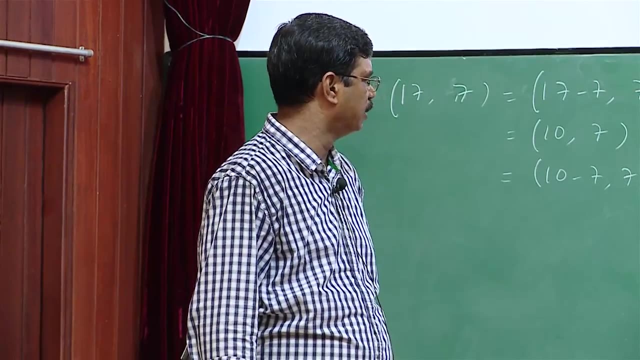 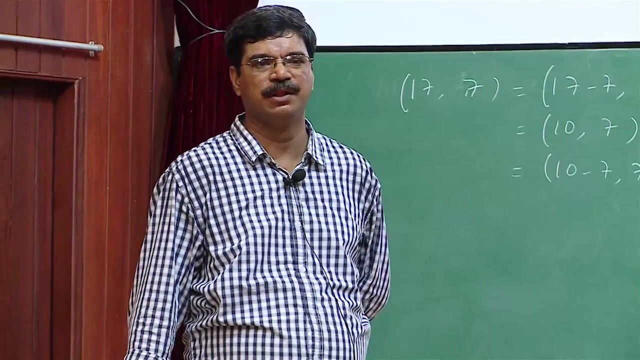 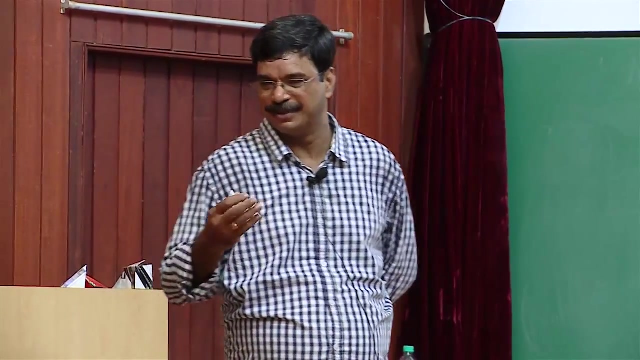 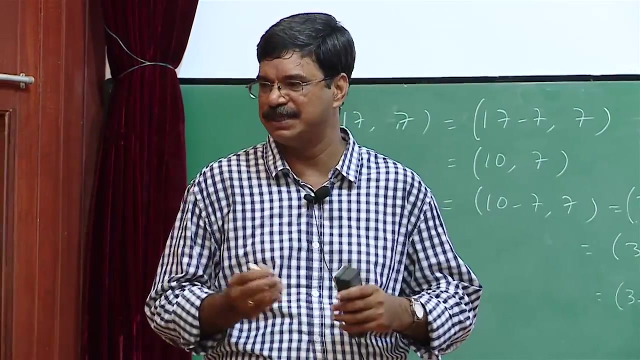 many. I just want one solution. Not possible, Positive or negative, whatever. Negative, Yeah, negative is also allowed. Not possible, The one candidate who says not possible? many are saying infinitely many. Majority rule should, majority should rule. What is I mean? there is one. very few answers, Please. Even if it is wrong, does not matter. 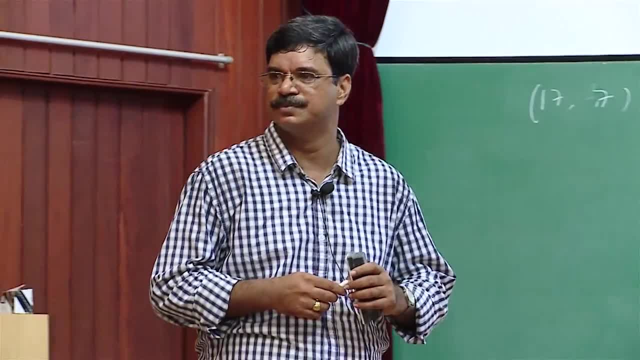 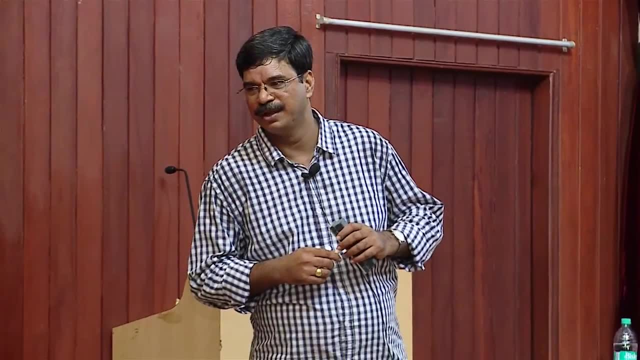 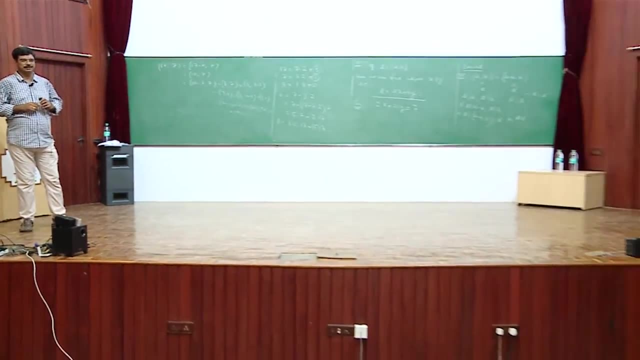 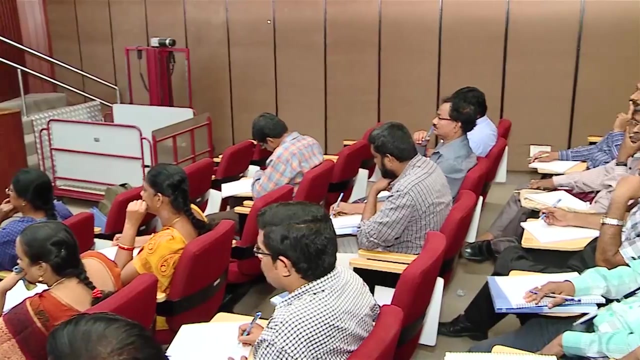 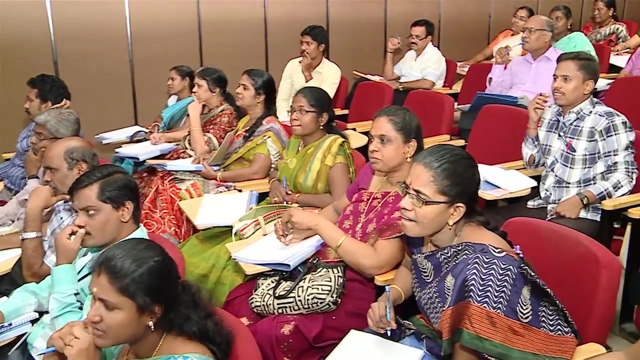 Please tell us, tell me … … … … …. So how to argue this kind of thing? Suppose there is a solution, Suppose there is an x and y. You look at left hand side, Here is 12,, here is 21.. There is a number 3, which 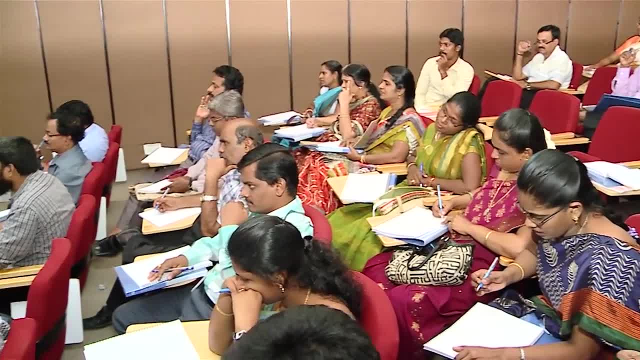 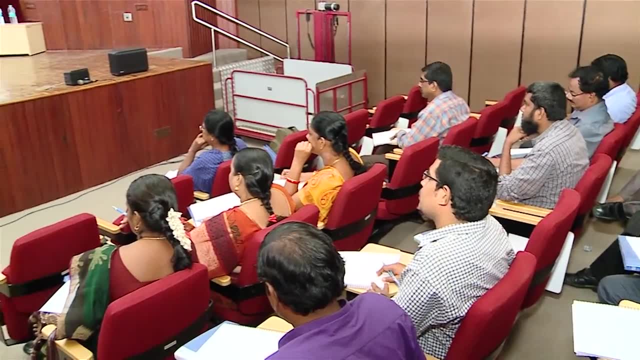 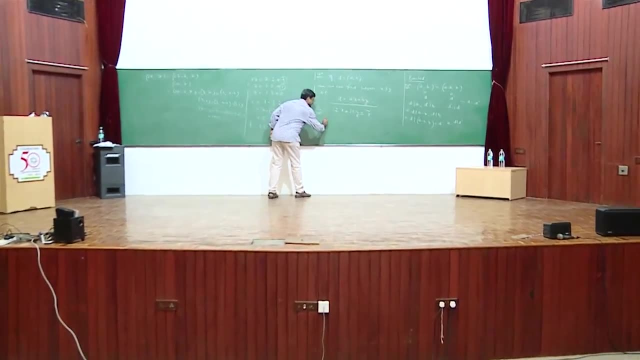 divides 12 and 21.. So, whatever the x and y, the left hand side is a multiple of 3, whereas the right hand side is not a multiple of 3.. So that is all. So LHS is a multiple of. 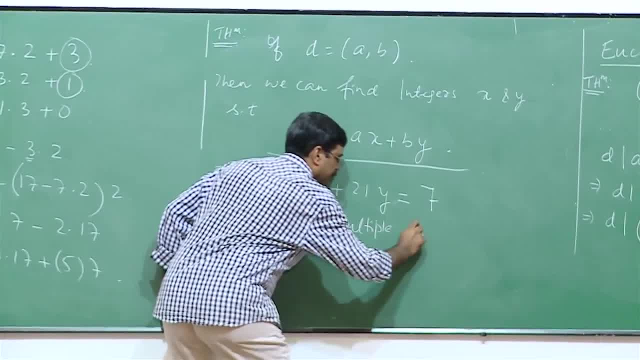 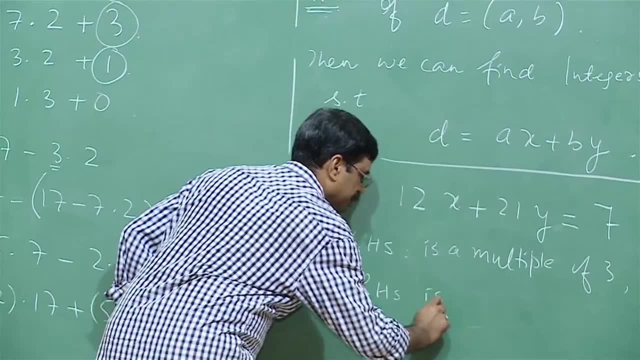 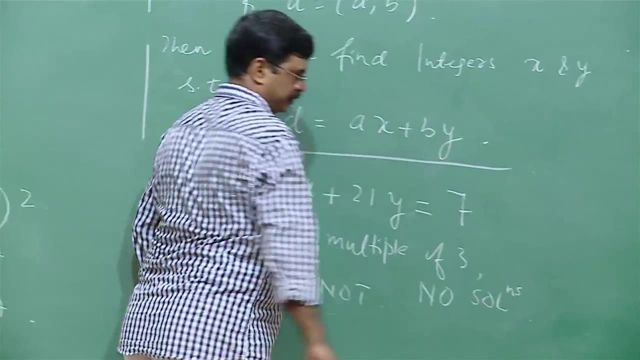 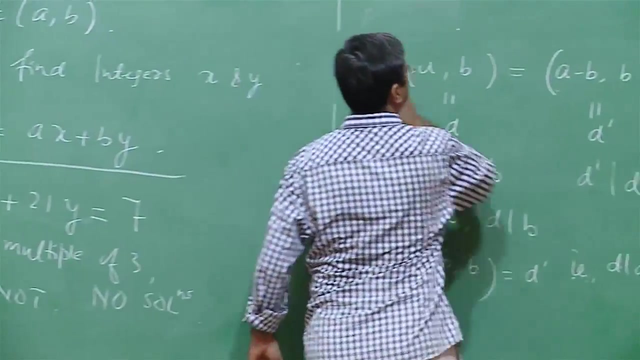 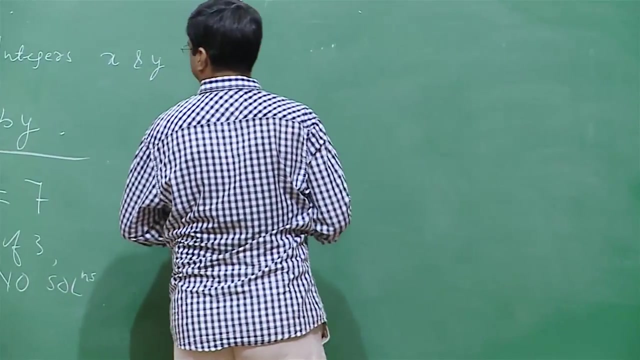 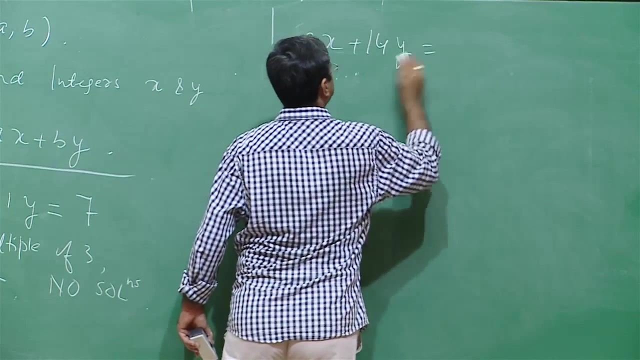 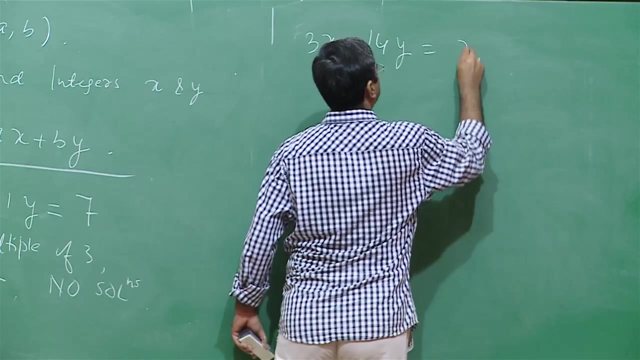 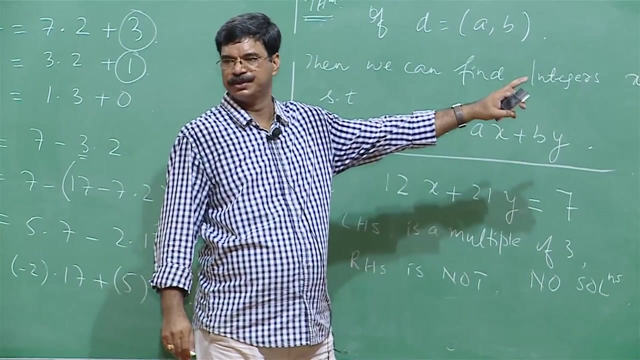 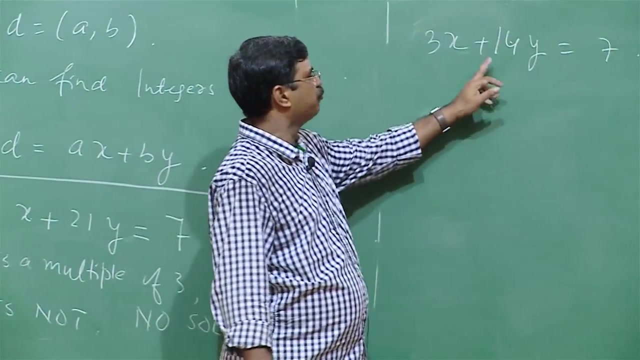 3, whereas RHS is not. Therefore, no solutions. It is very easy to. On the other hand, if I give you, let us say 3x plus 14y, Yes, 3x plus 14y is equal to let us say 7. again, You can find solutions. Why? Because 3 and 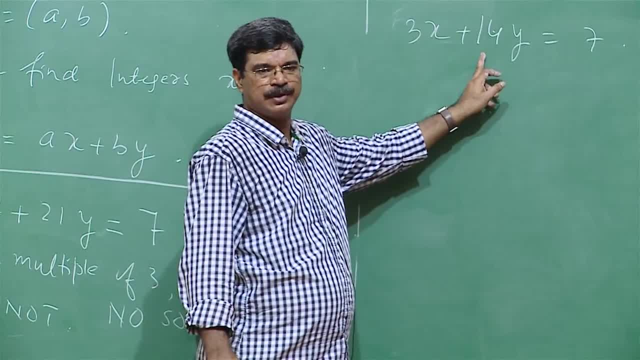 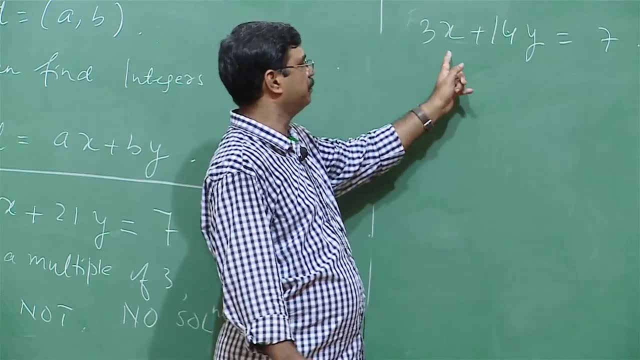 14 are co-prime. Therefore their GCD is 1. And GCD can always be written as a linear combination of x and y, So you can find some y So that this is solvents. So you. 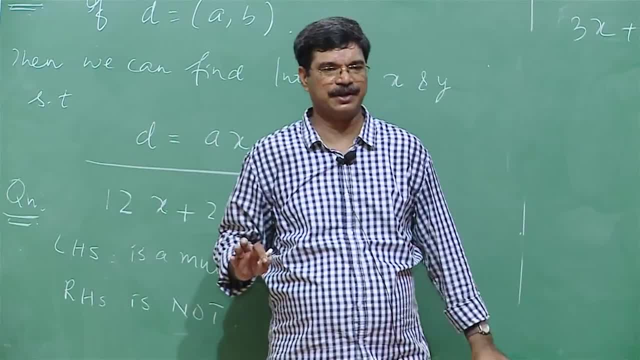 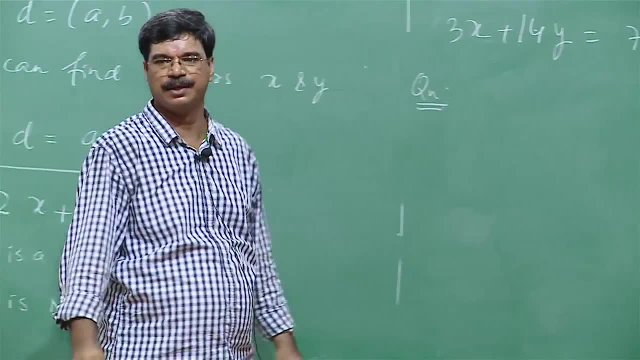 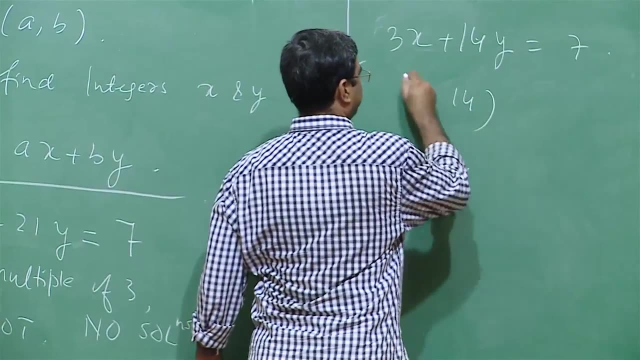 see how all these things are very elementary and they are related. So question: Yes, Ok, So what I am saying? 3 and 14. Co-prime Are co-prime, Co-prime, Co-prime. 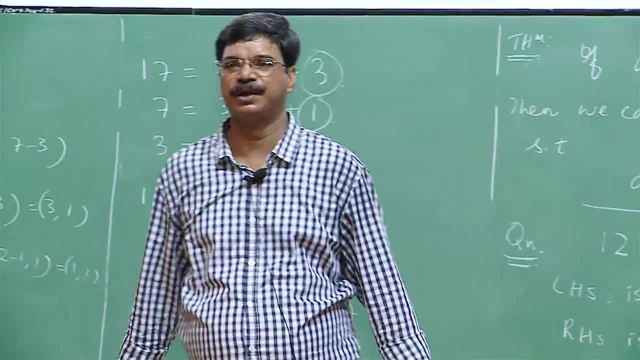 Co-prime. So what about some of these Co-prime, Co-prime? So what about some of these Co-prime, Co-prime, Co-prime? So what about some of these? They are great. 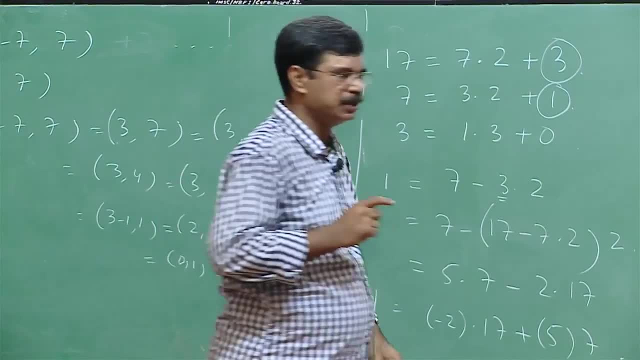 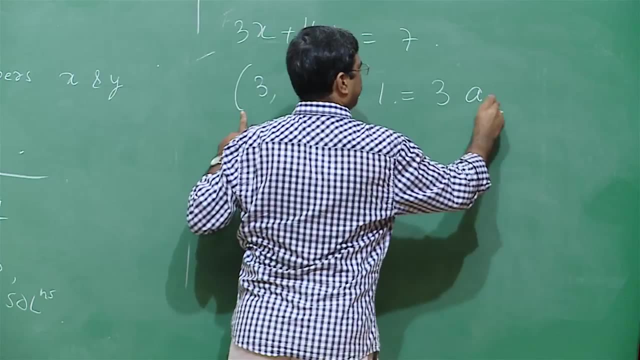 They are great. The GCD is 1.. Ok, And we have seen that the GCD can always be written as an integral multiple of a and b. Therefore, this 1, we can write it as 3 times some a plus 14 times some b, For some we. 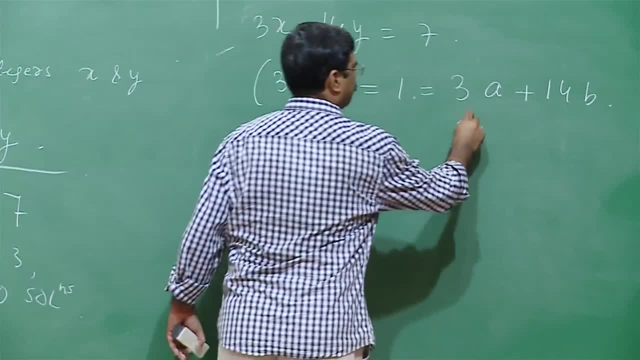 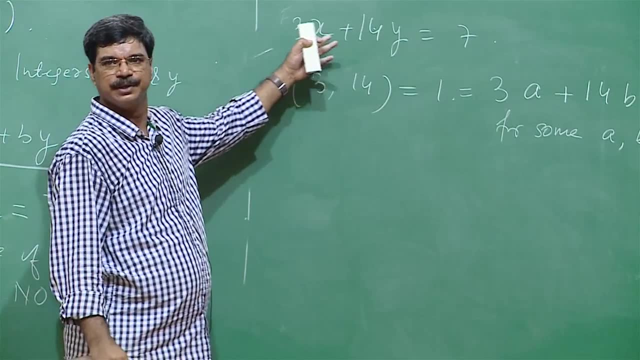 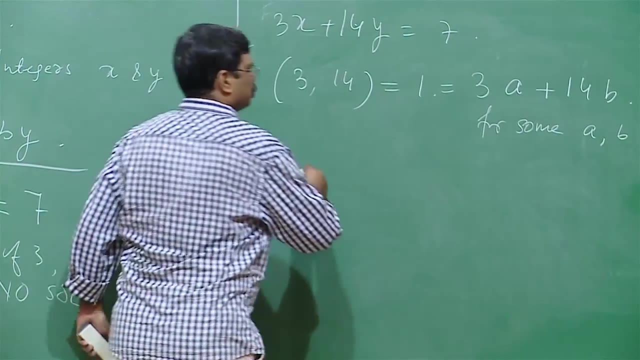 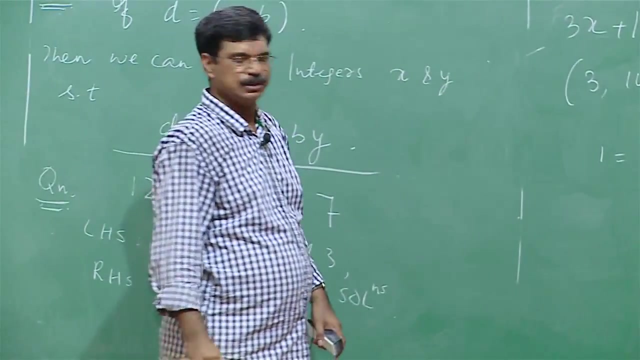 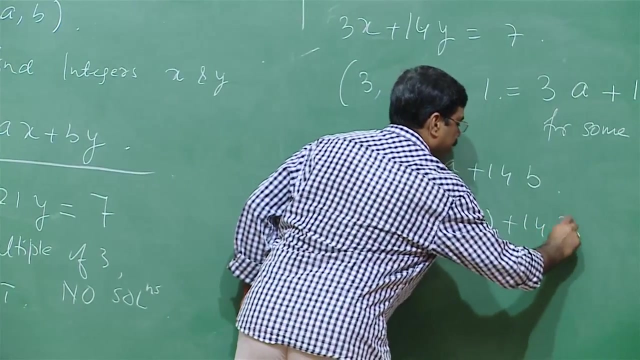 can find out a and b. Ok, Ok, Ok, Ok, But that is what we wanted. okay, so you multiply it by 7 there, so 1 is equal to 3a plus 14b and 7 is equal to 3 into 7 times a plus 14 into 7 times b. so x and y are formed. 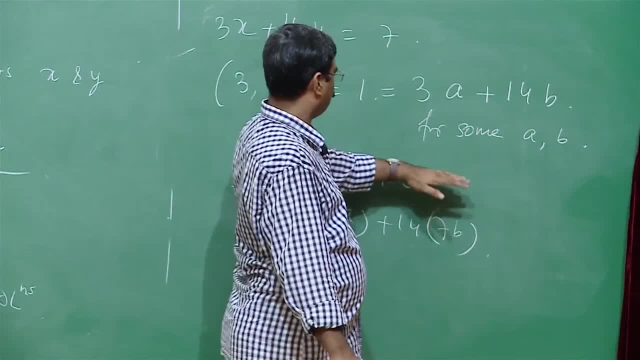 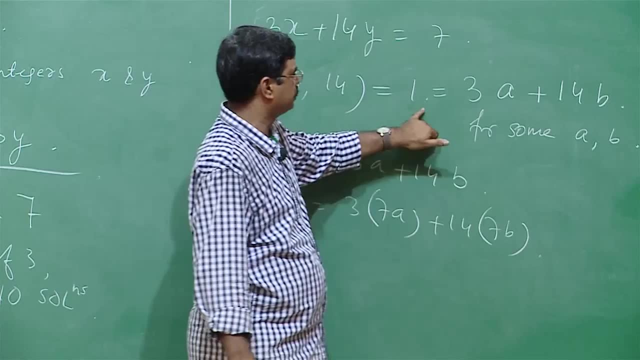 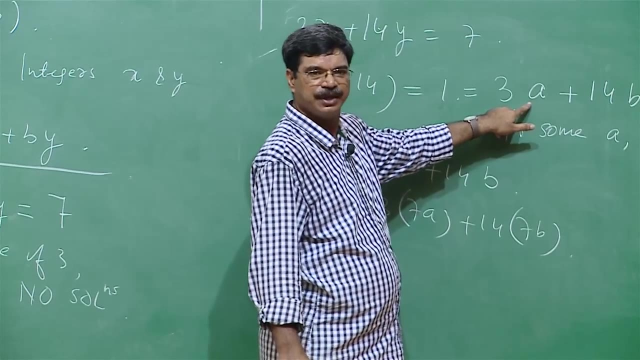 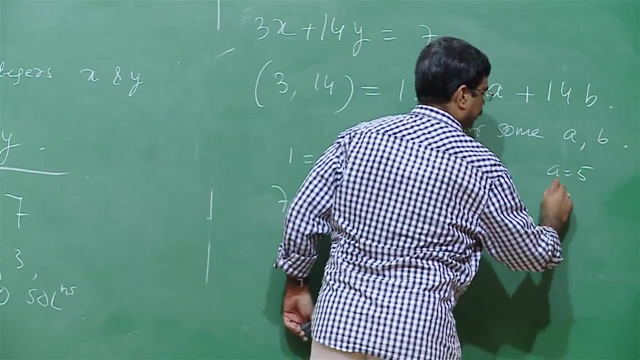 Once you find this a and b, for example, what is a and b here in this equation? can you guess? just say what. what can you say about a and b? See, for example, a is 5 and b is minus 1 is a solution. So a is equal to 5 minus 1 and therefore you put: 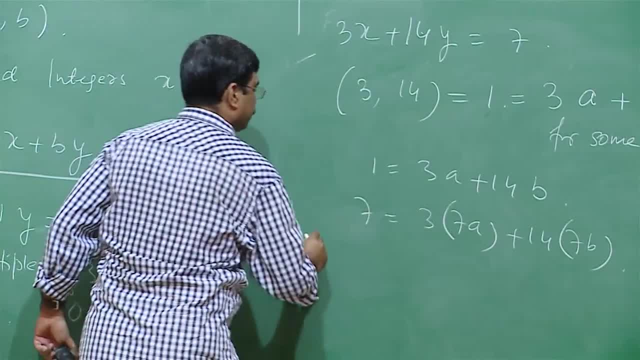 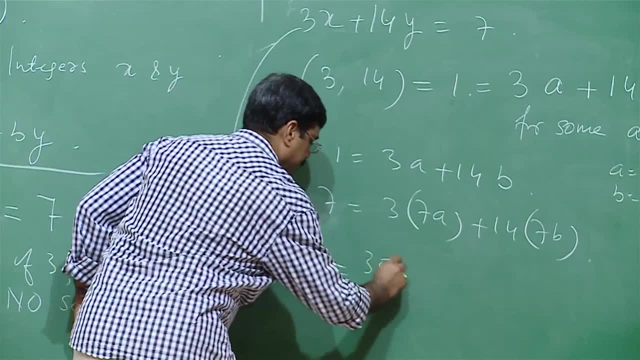 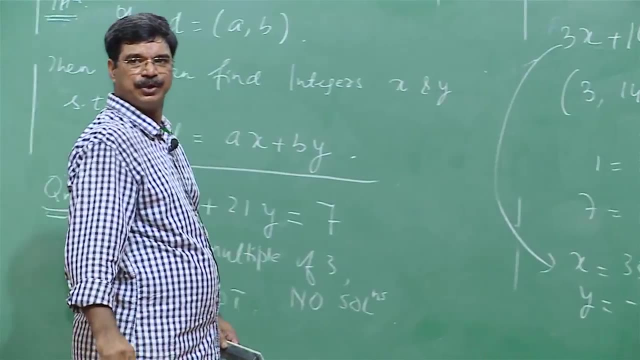 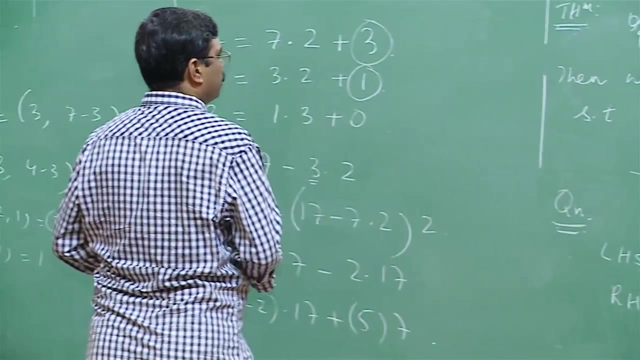 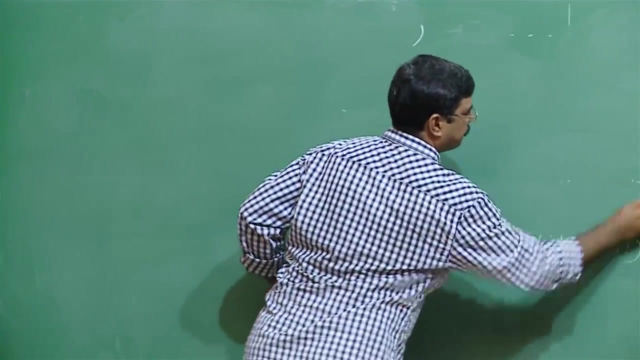 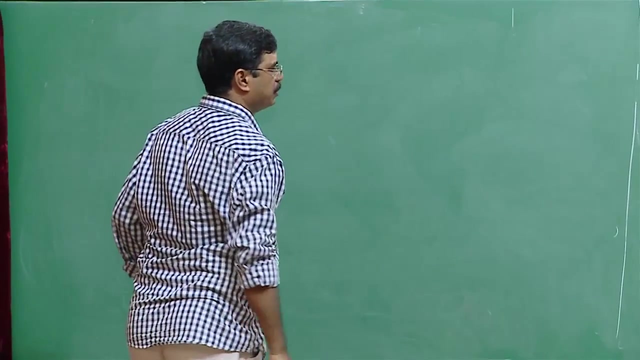 7 times this thing, So x for this equation, x is equal to 5 into 7, 35 and y is equal to minus 7.. We can see that if you multiply and see that that is a solution for that Question that I wanted to give you is. 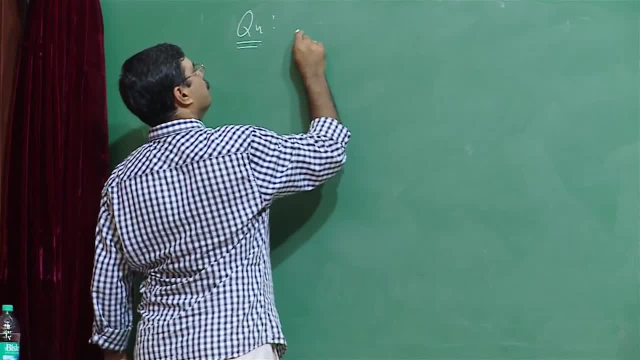 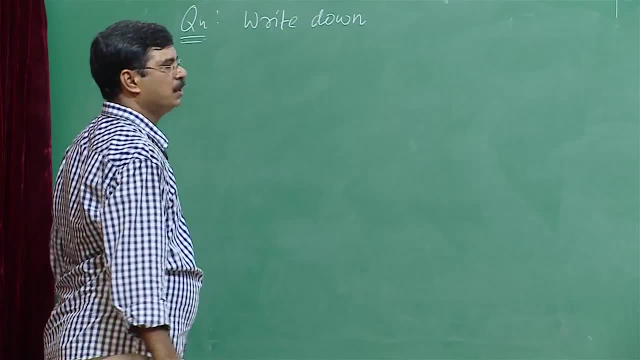 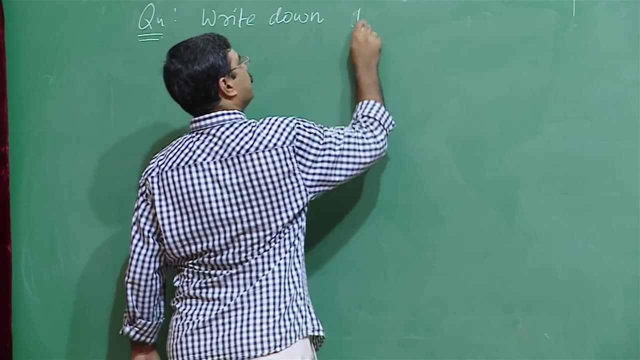 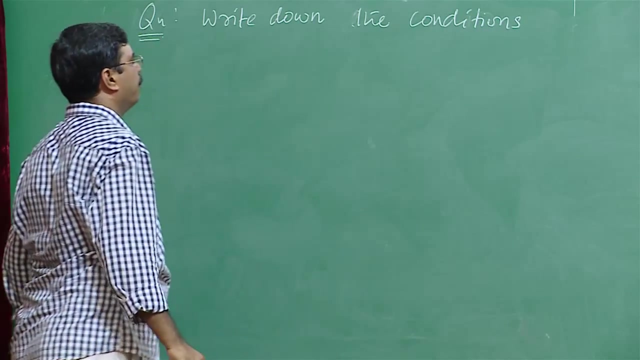 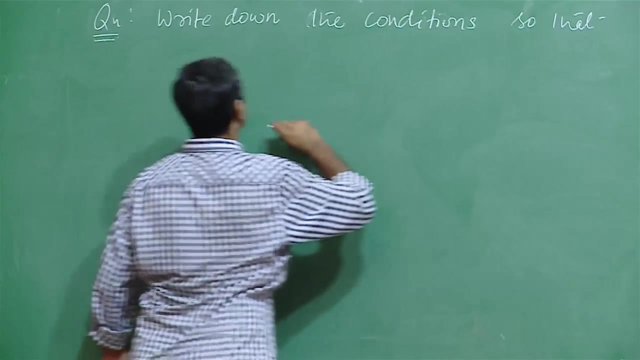 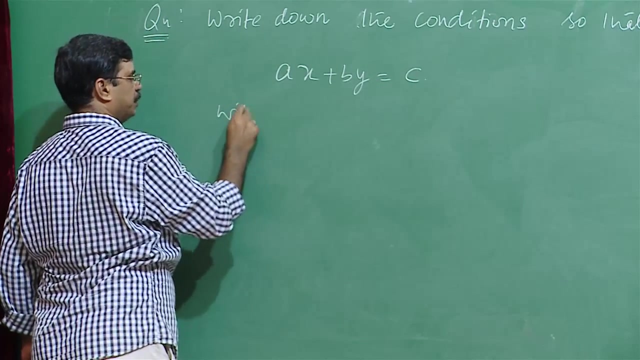 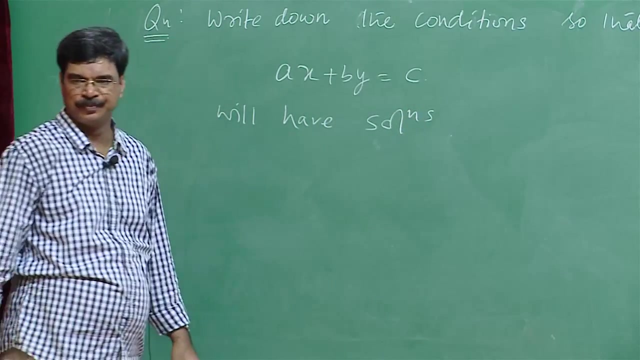 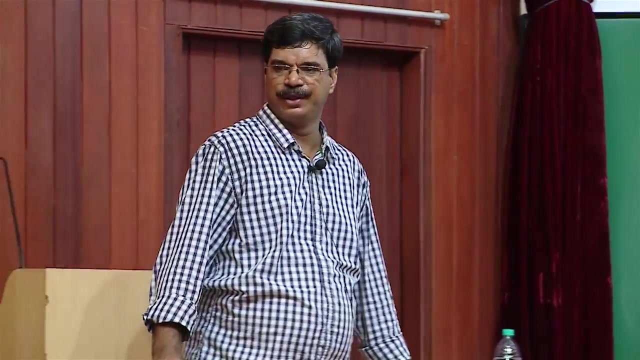 Write down conditions so that A x plus b? y is equal to c will have solutions. You are given an equation: a x plus b? y is equal to c. a, b, c are integers, not 0, and we have to find out under what conditions we 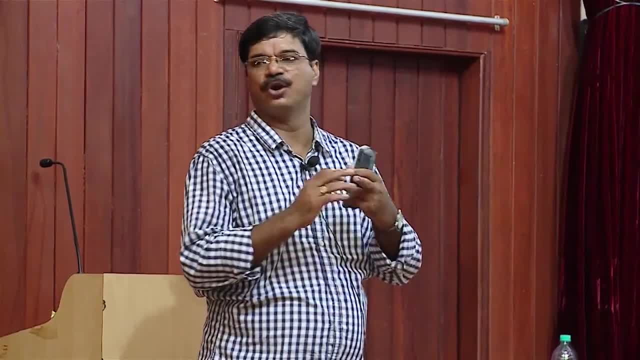 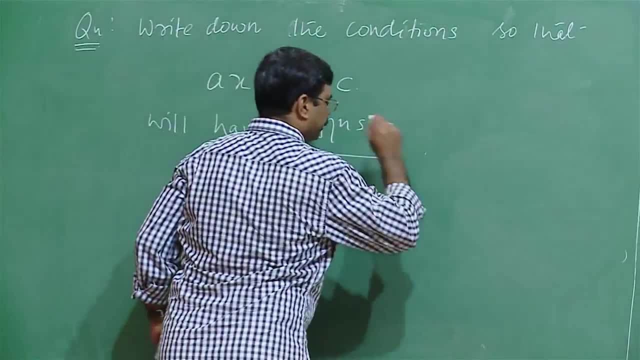 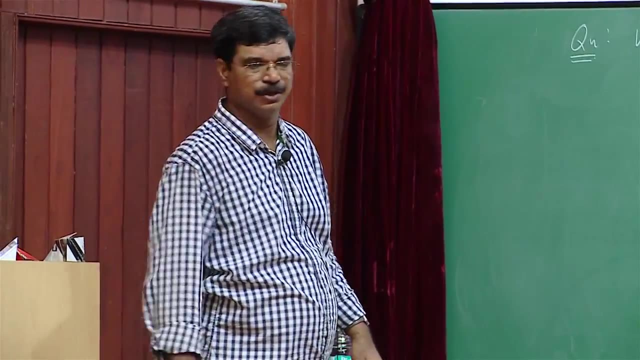 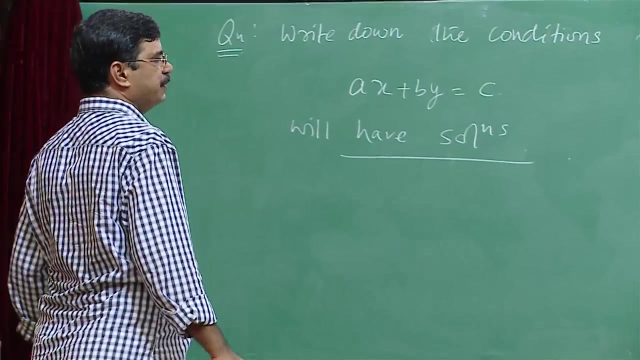 have solutions for this. Under what conditions? it will not have solutions. So discuss the solution of this things. So we will discuss it later. You can discuss among yourselves and you can. we can discuss it later also in the leisure time and tomorrow also. So this is about this things. GCD Now. 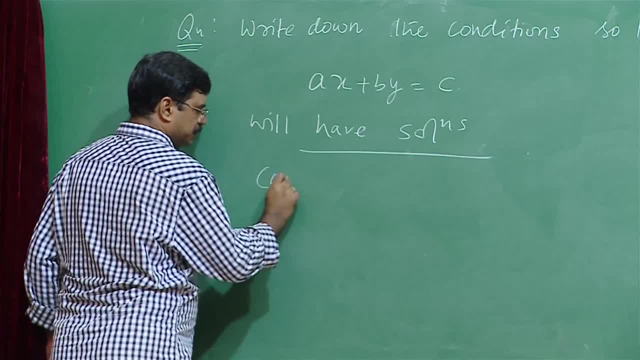 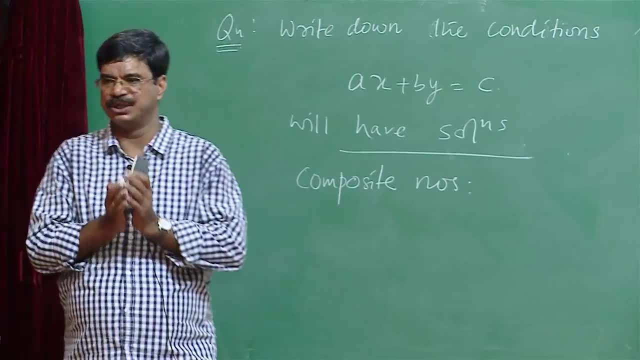 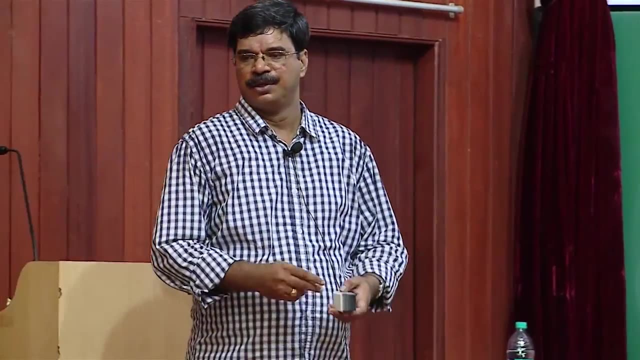 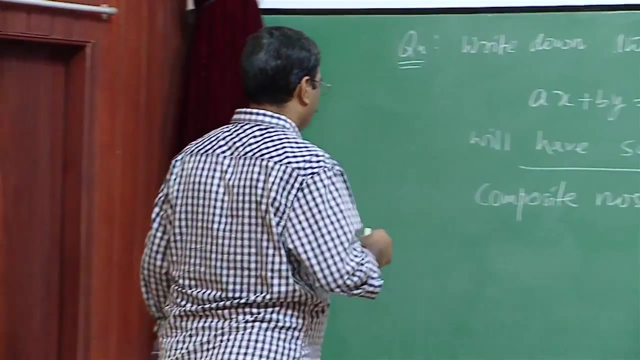 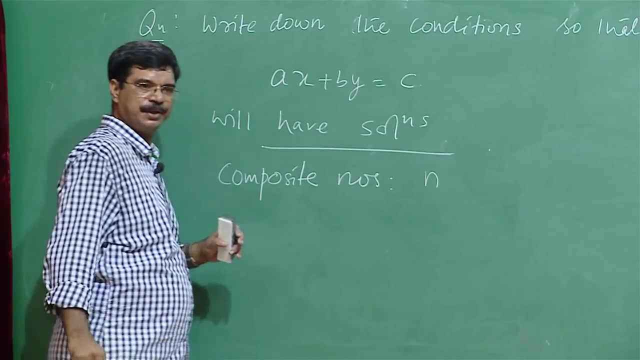 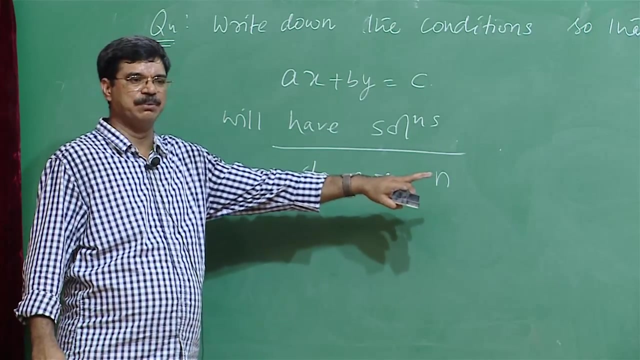 as you know, Composite numbers, for example a number, we say that it is composite if n can be written as product of 2 numbers, a and. 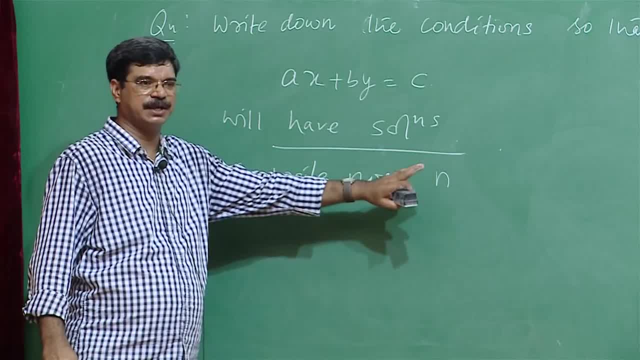 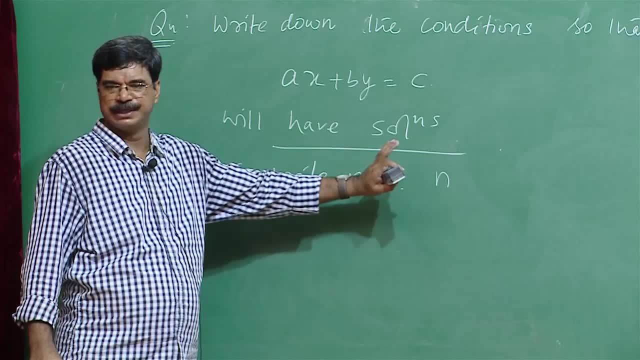 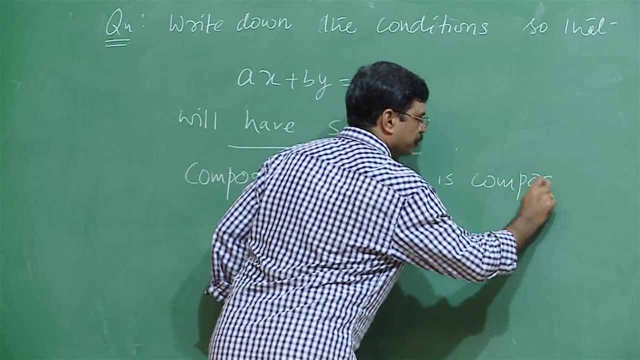 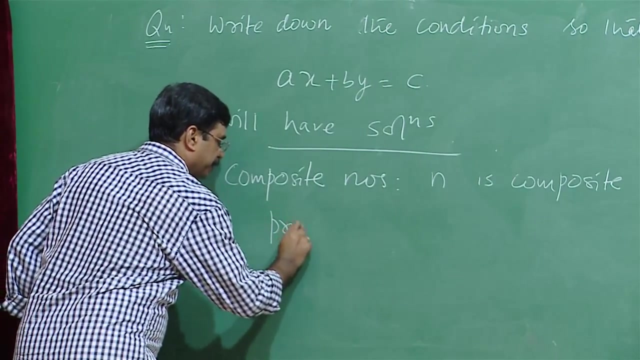 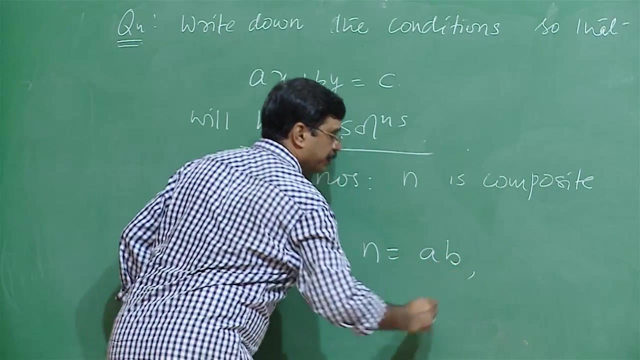 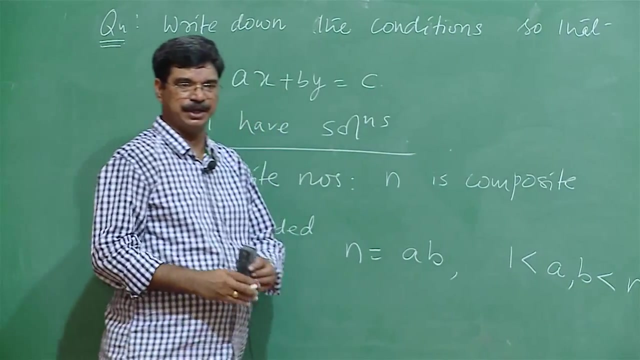 b, with some conditions. a is not equal to 1 and b is not equal to 1. that much will suffice. So n is composite, provided we can write n as a times b. with strict inequality, a and b should- strictly should- lie between one end. 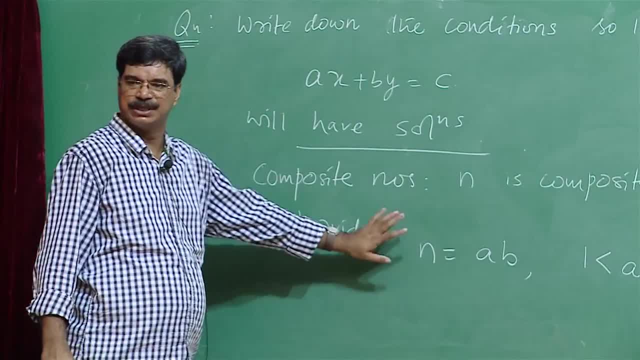 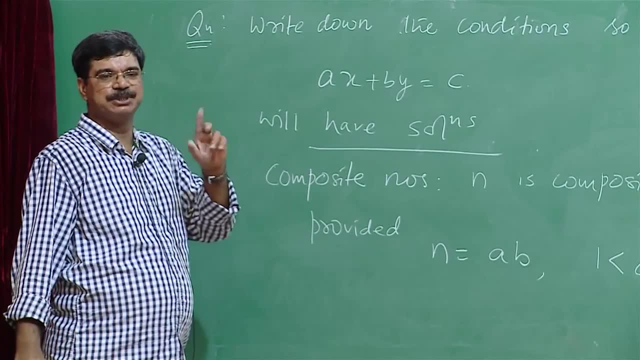 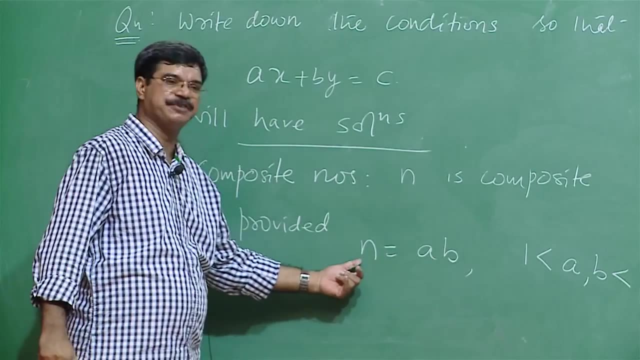 So this is the way of what you have said: more than two factors. it means the same, because only two factors means one end itself, but here are more than you know. one end itself, one end itself is of course a factor of this, but there are other factors, a and b. so which? 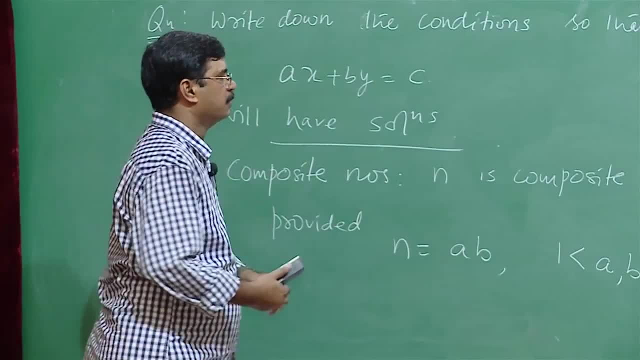 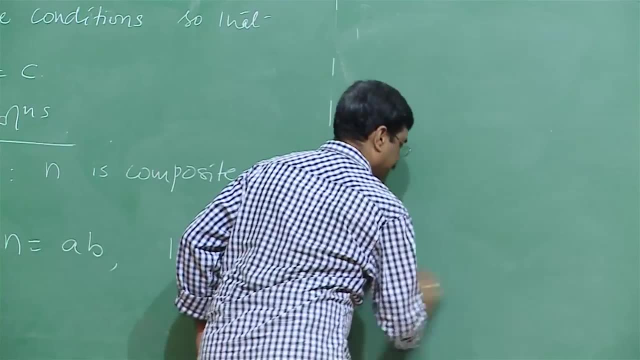 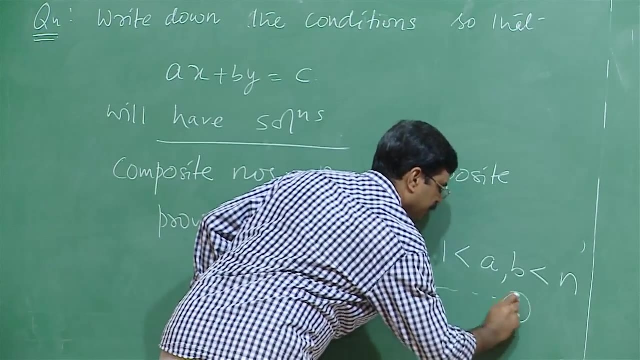 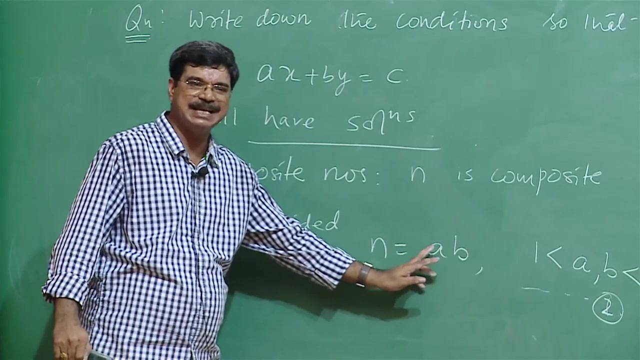 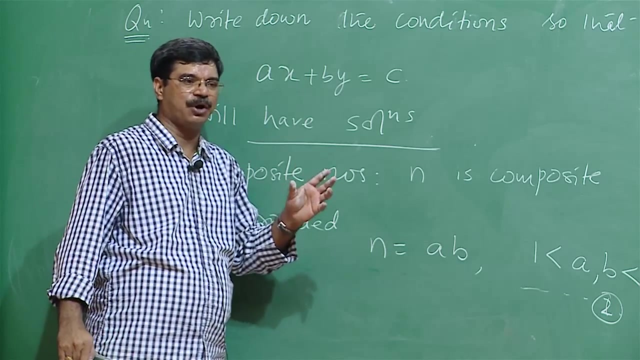 is lying between one and n. Okay, this is number two from here. what can you say about the size of a and b in terms of n? okay, I mean how large can be or how small can be a and b, For example. can a and b? 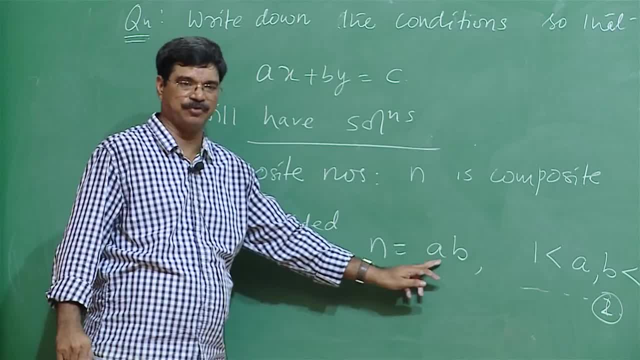 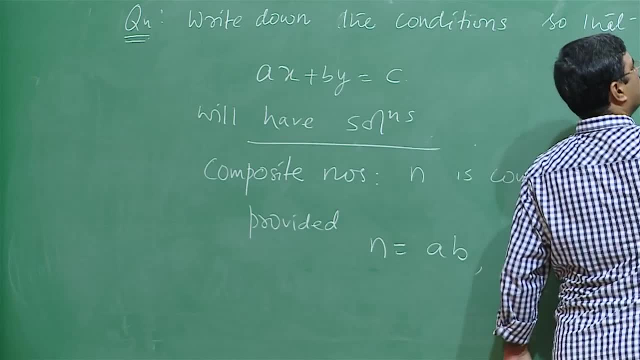 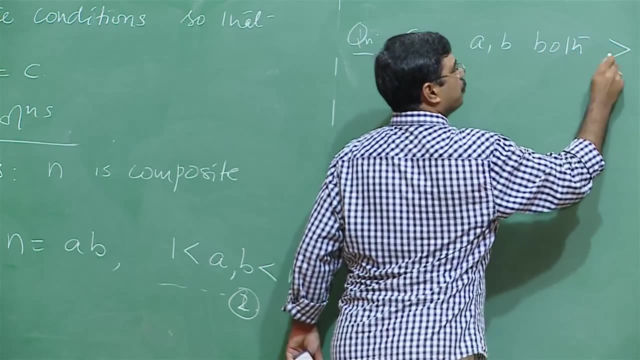 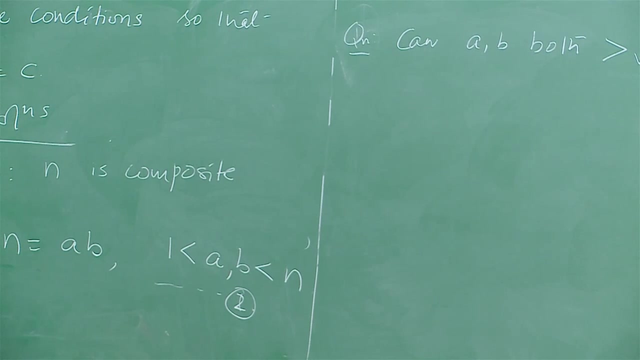 Okay. Can they be both bigger than square root of n? okay? question: Can a and b both? It is not possible, okay, because if it is true, Okay, It is not possible, no, but it is not possible, Okay, Then a is bigger than square root of n. b is bigger than square root of n- their product. 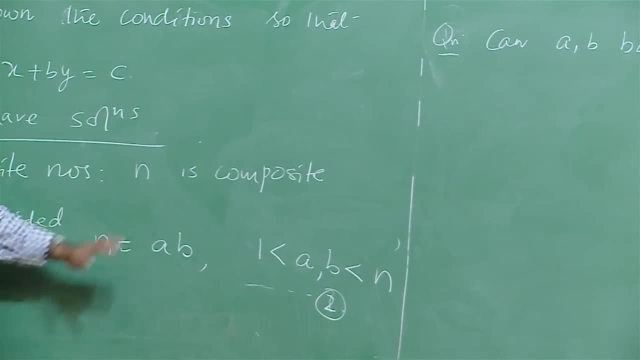 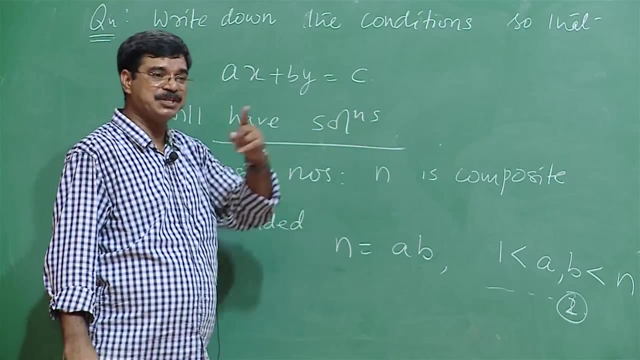 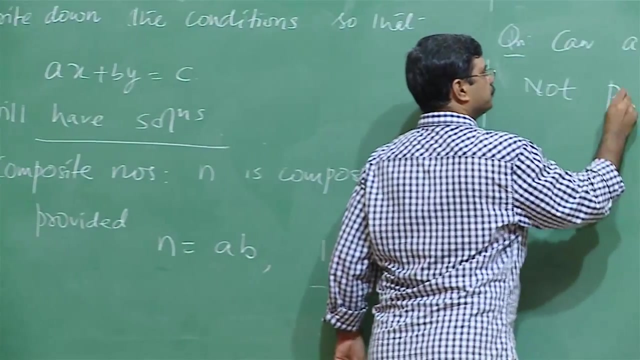 will be bigger than n. therefore, it is not possible. Therefore, what is possible? That one is any greater than One of them must be less than square root of n. okay, that is the conclusion. so it is not possible. And not possible implies the negative union. 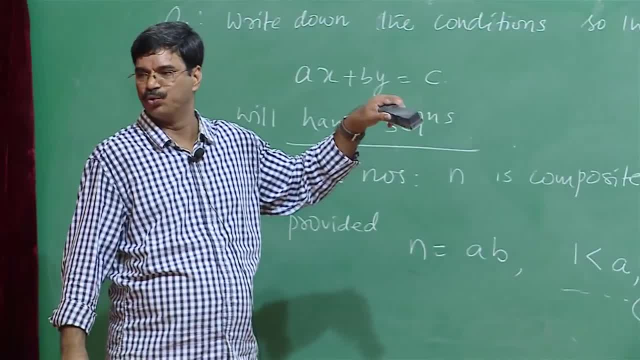 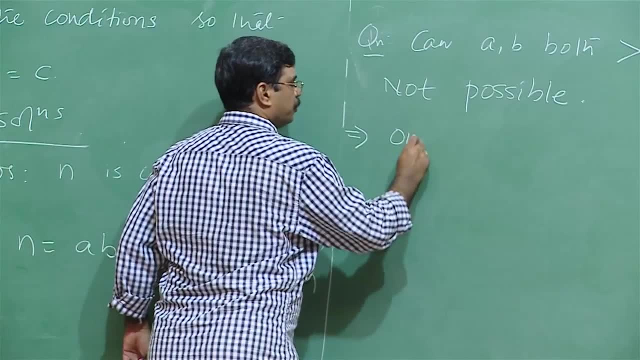 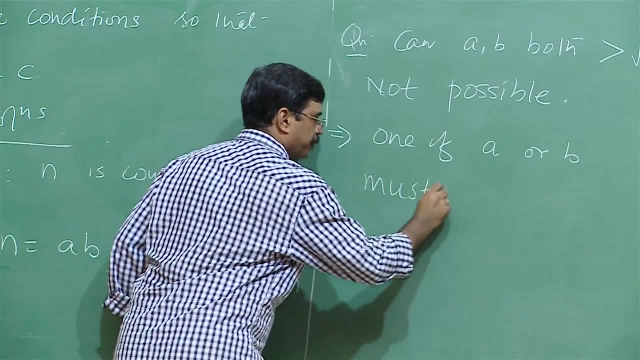 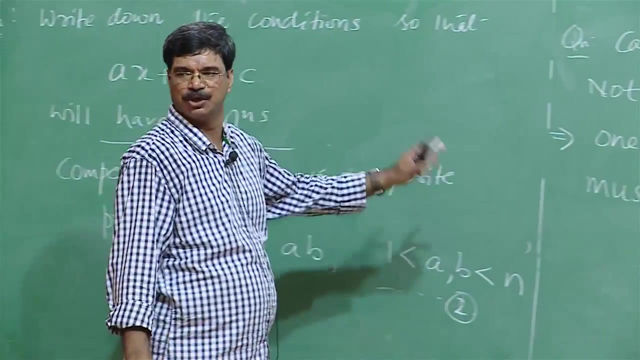 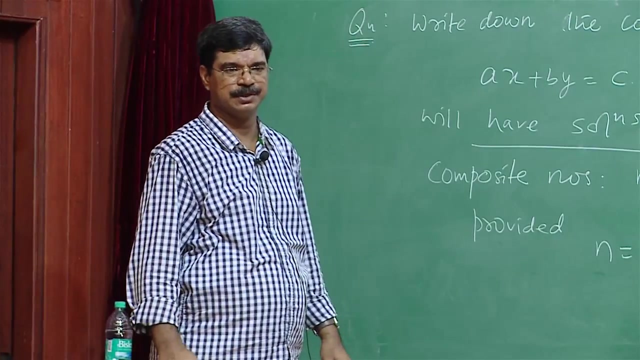 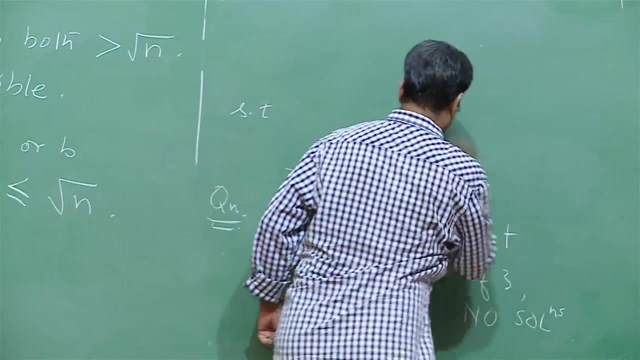 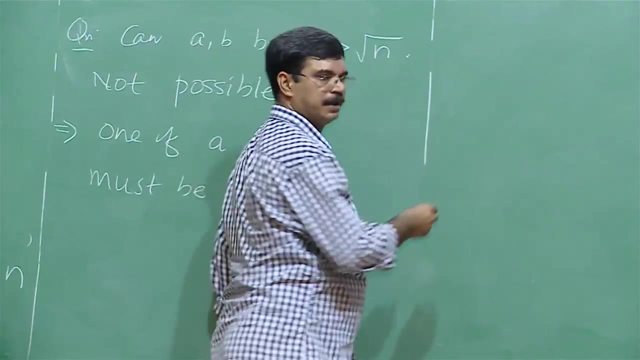 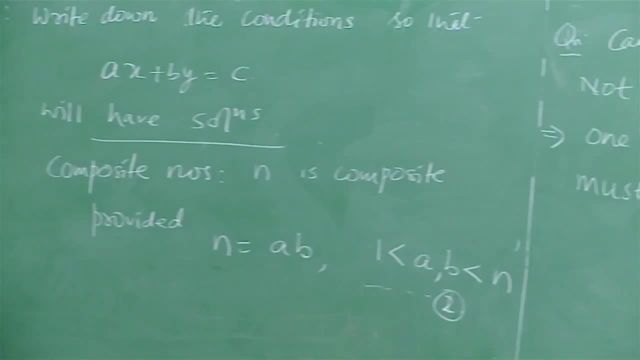 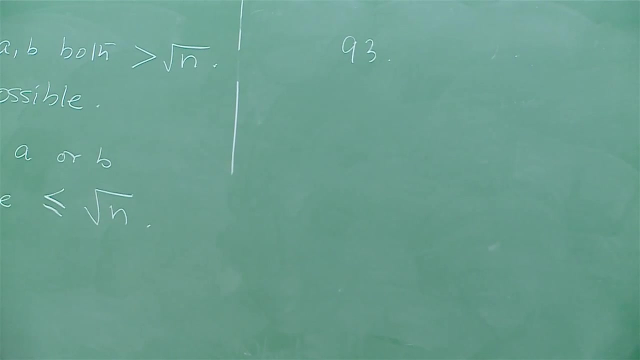 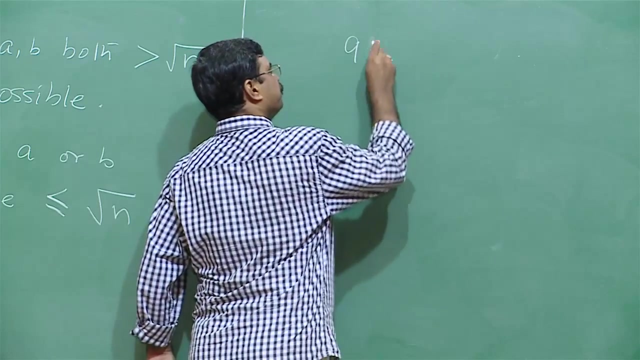 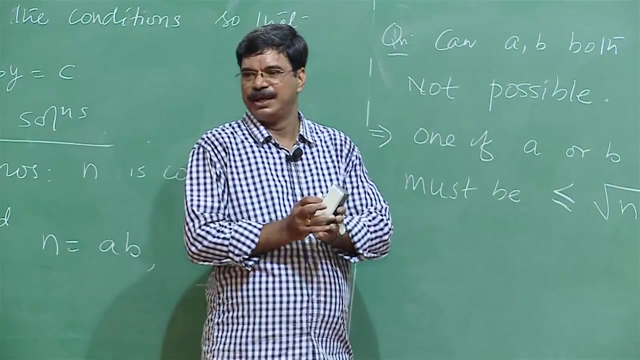 I give you a number 93. Is it prime or not Prime? Not prime, How do we know? Because we divide it 31.. 31 divides it. Suppose I give you 91. Some, that is not, Yeah, but the thing is, here to save time. we are taking small numbers, But supposing we 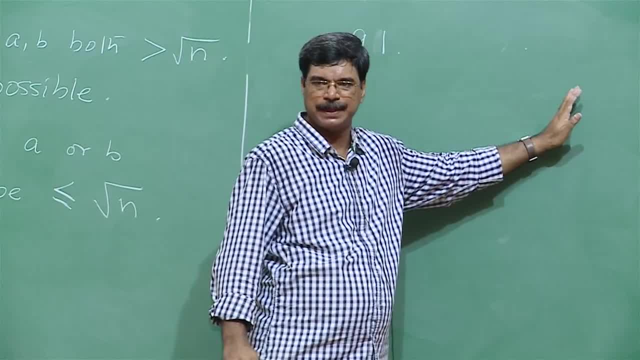 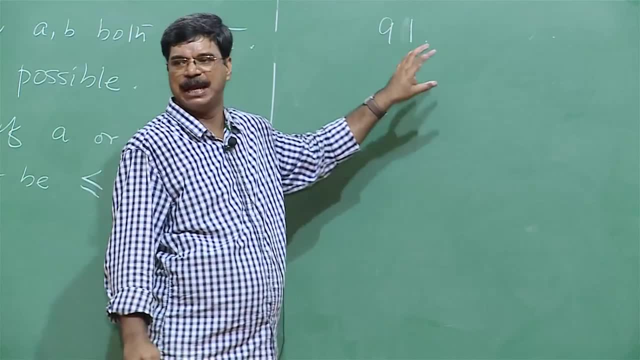 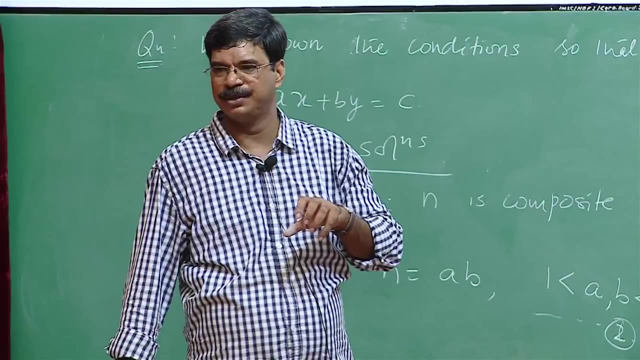 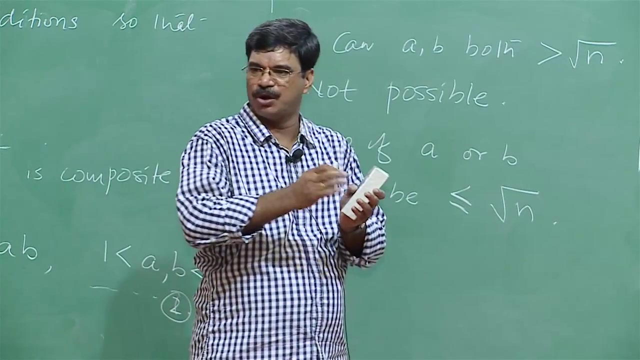 write large numbers and ask the question: Now, when we say that it is prime or not prime, if it is composite, Yeah, It will have a prime number, prime divisor. It will have a divisor which is less than square root of this number. Now, one thing is: every number, a composite number, has lot. 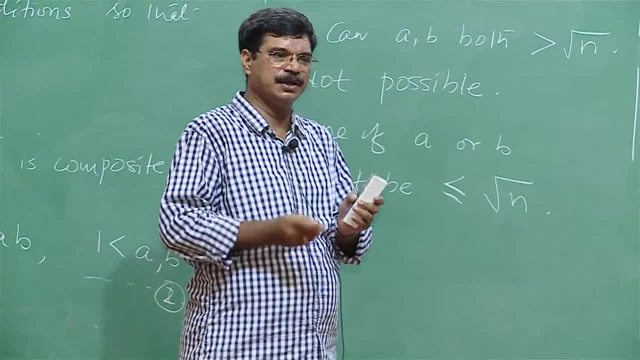 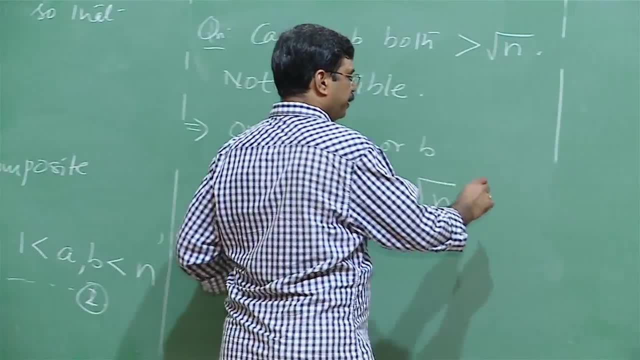 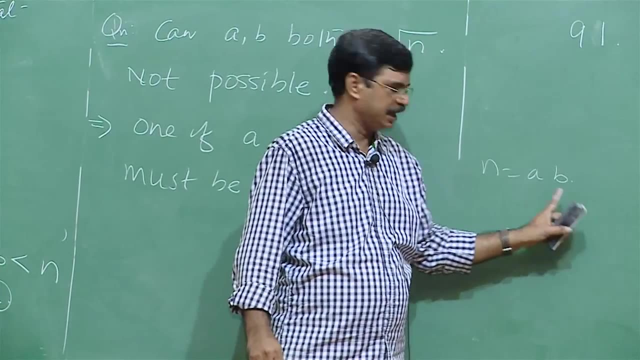 of factors You keep dividing. ultimately, you can write it as a product of primes. N is A and B. Right Yeah, If A and B are both composite, you can further write it as A1, B1,, A1, A2, B1, B2.. So ultimately, 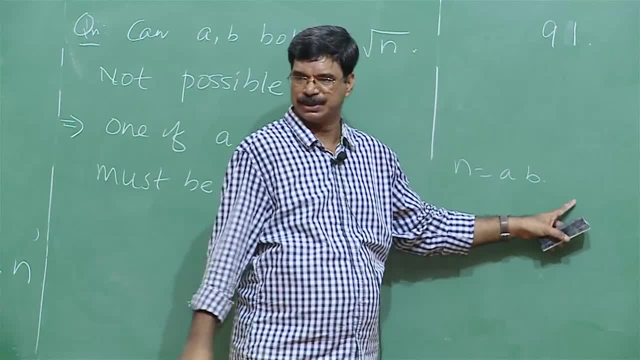 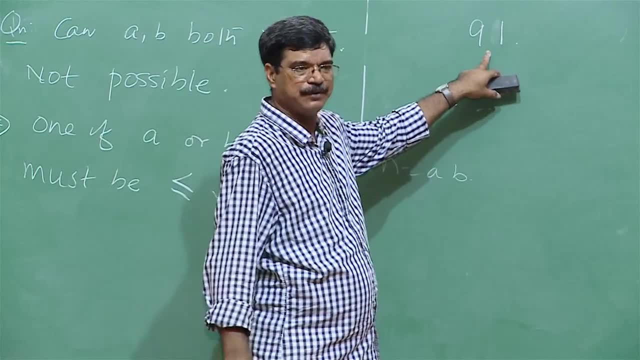 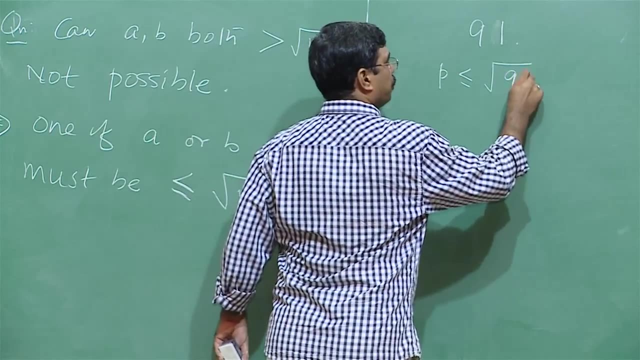 you can arrive at a product of primes. So every number has a prime divisor. Therefore this number will have, if it is composite, it will have a prime divisor, P, which will be less than or equal to square root of 91.. 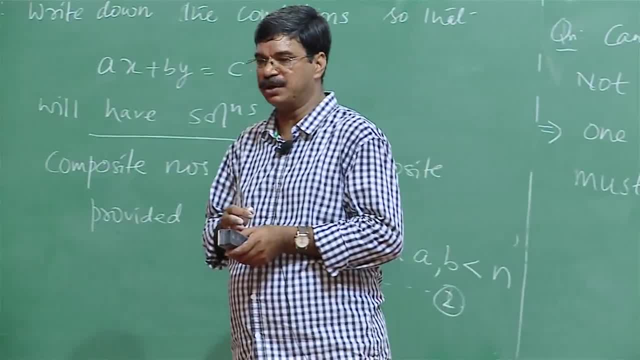 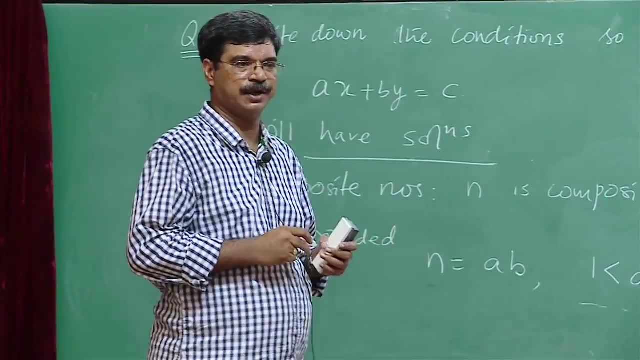 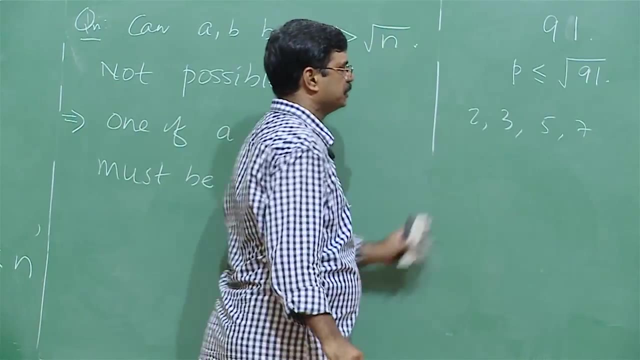 What are all the primes which are less than, Which are less than square root of 91.. What are all the primes which is less than square root of 91? 2,, 3,, 5, 7.. Only few primes: 2,, 3,, 5 and 7.. Because the next prime, 11, square, is 100, more than this. 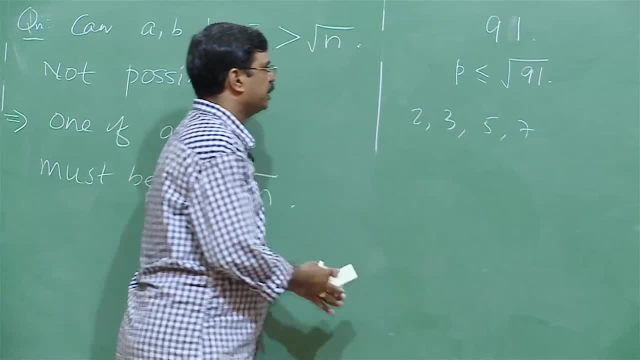 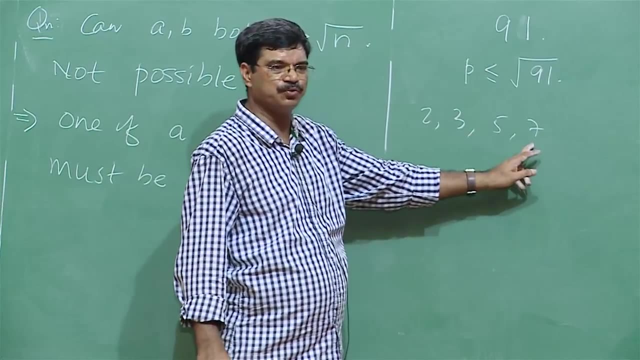 one, 121.. 121.. Therefore, whether this is prime or composite enough to check with this, Yeah, You have to check with this. only this 4 divisors So 2, check 2 divides this. it does not. 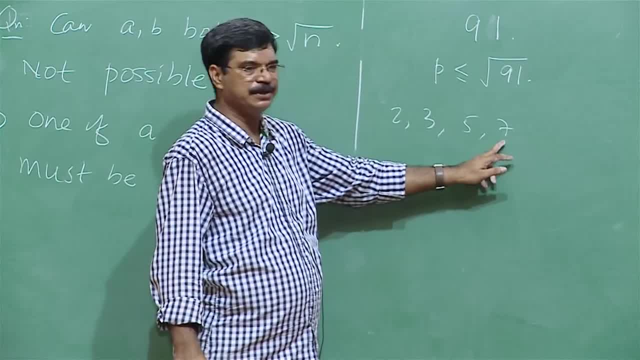 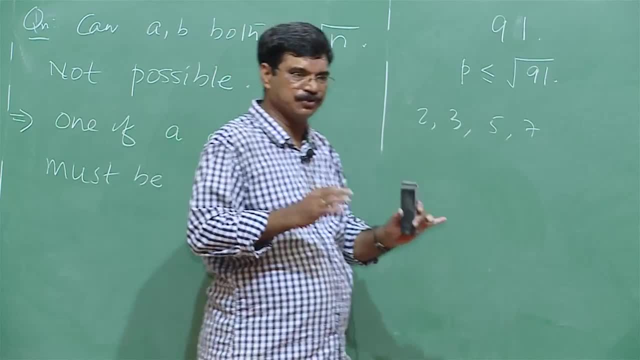 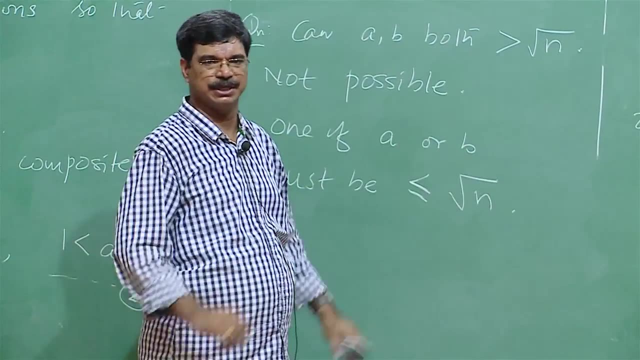 3? Does not 5? No, But 7? Yes, Therefore. So only 4 steps are enough, Rather than you know thinking and looking and all these things. So, even if you are given a large number, this process is very efficient. 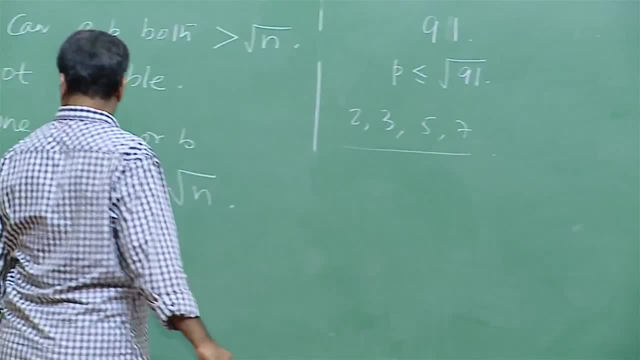 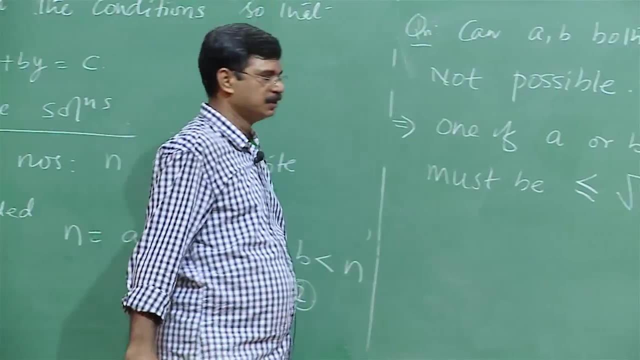 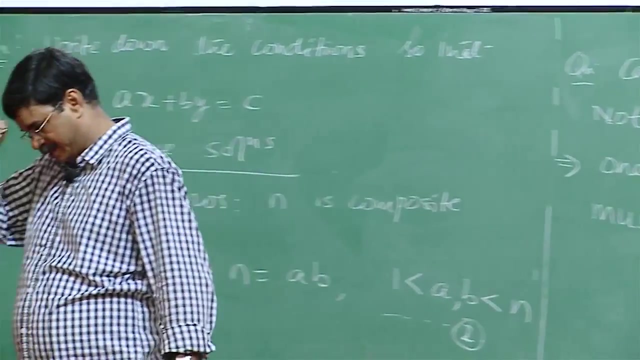 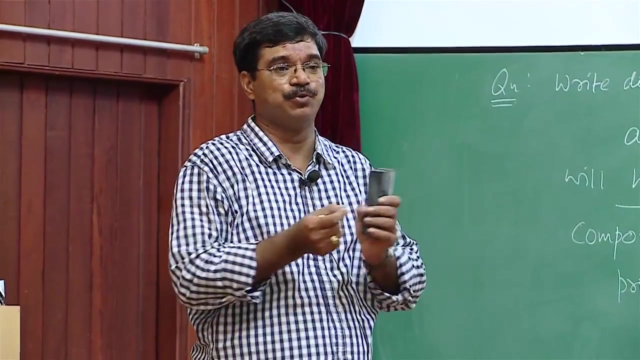 Ok, So this is one of the things It is. it gives you a primality testing In the sense whether a number is prime or not. So what is See? supposing you have a digit which is 400 digits, a number with 400 digits, then this: 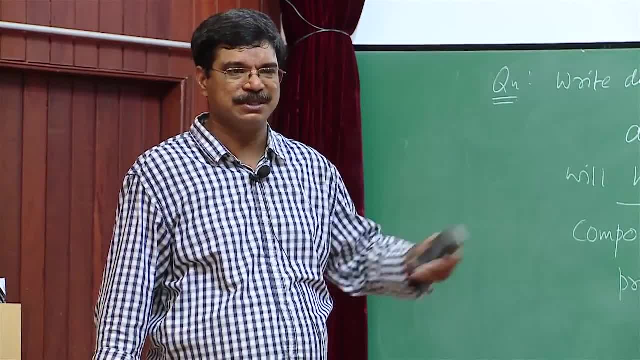 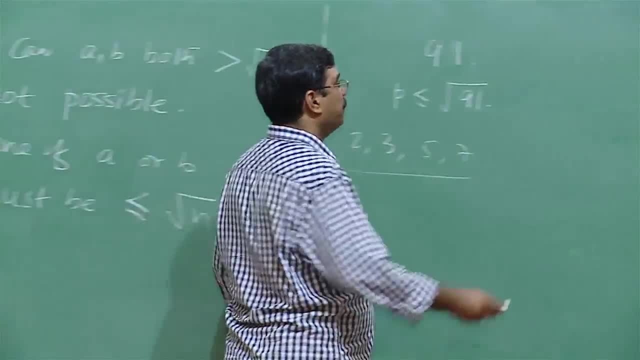 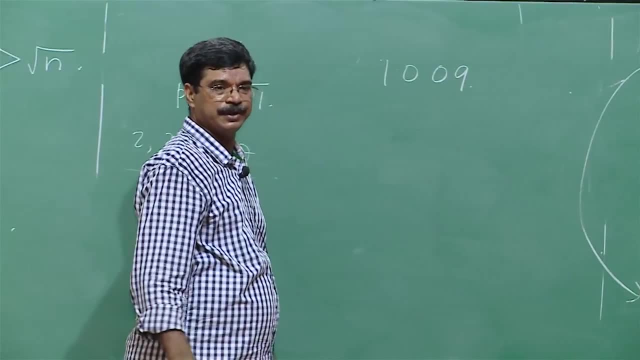 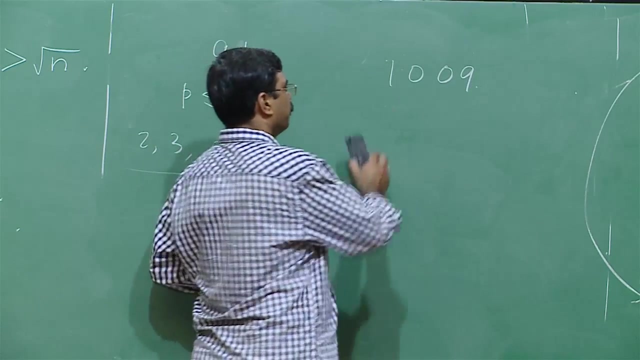 is not efficient. There are other ways, But for small numbers it is quite efficient. Ok, Now I mean even 1009, whether it is prime or not, this method will tell you very efficiently: Ok, Such small numbers we can manipulate, use this method quite easily. 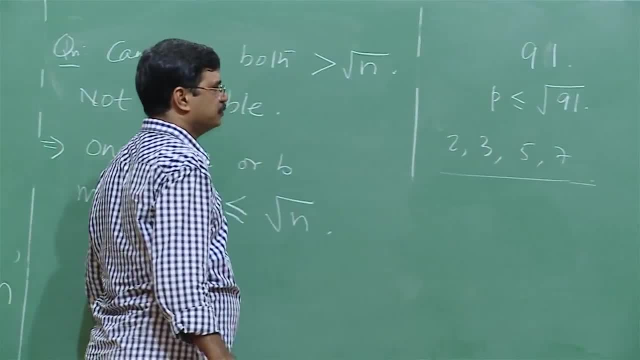 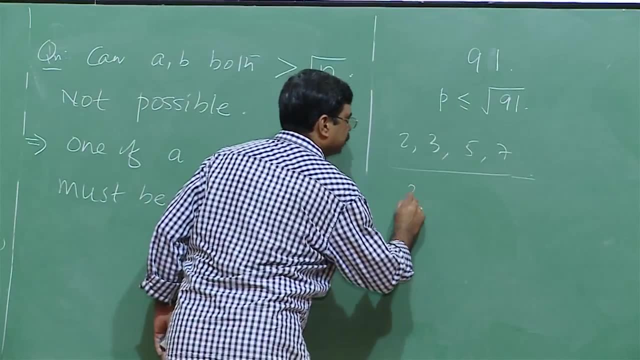 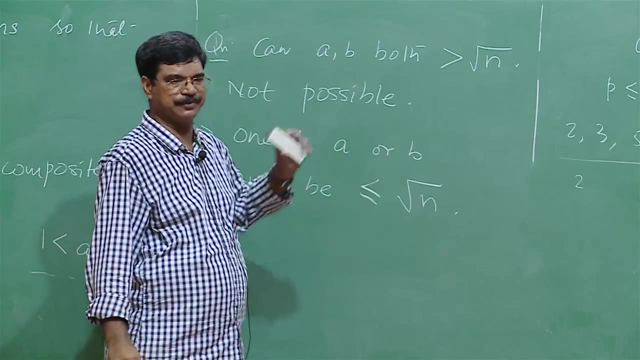 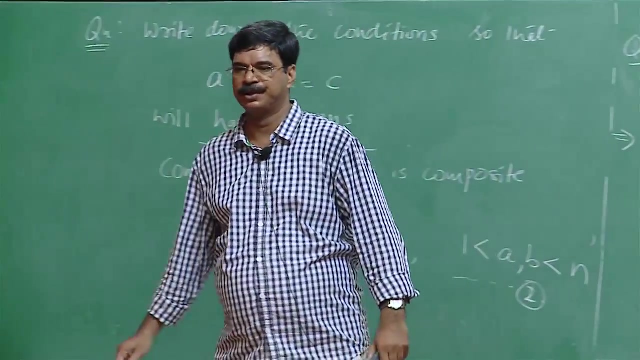 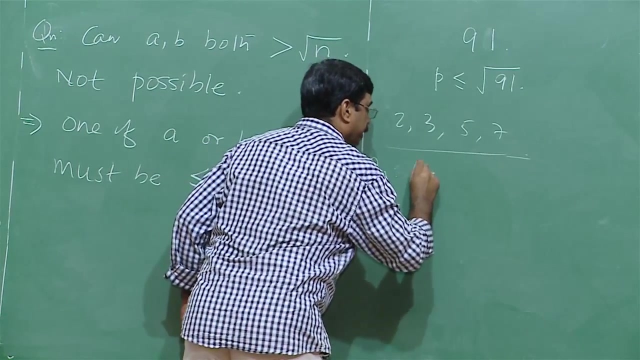 Ok, So this is one thing. A beautiful application of this is: Suppose you have a Suppose you are given only this many primes, all the primes up to square root of 100, so 2,, 3,, 5, 7, with these primes we want to generate more primes. we are given only question find. 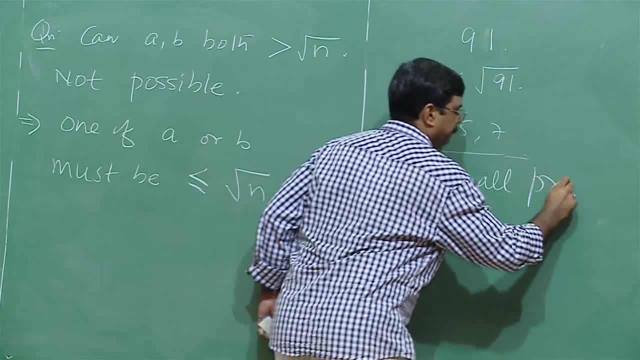 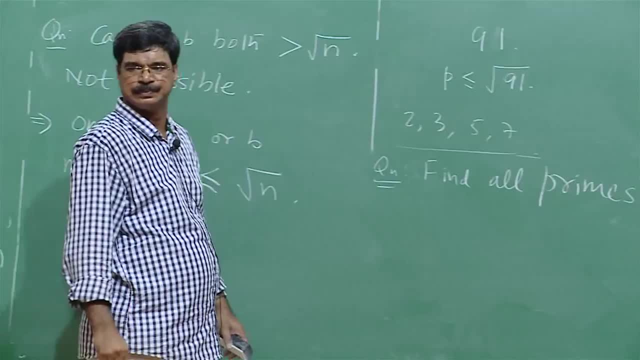 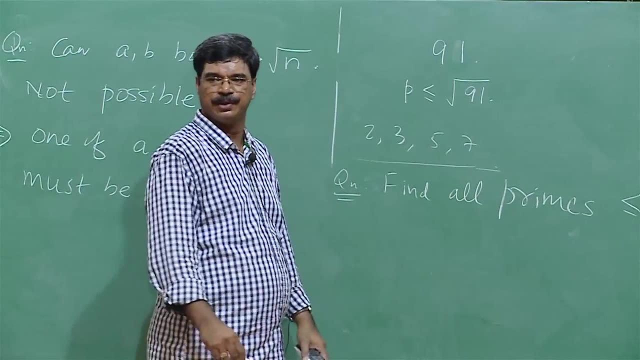 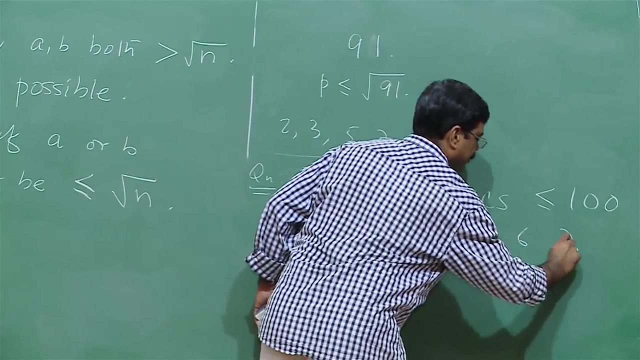 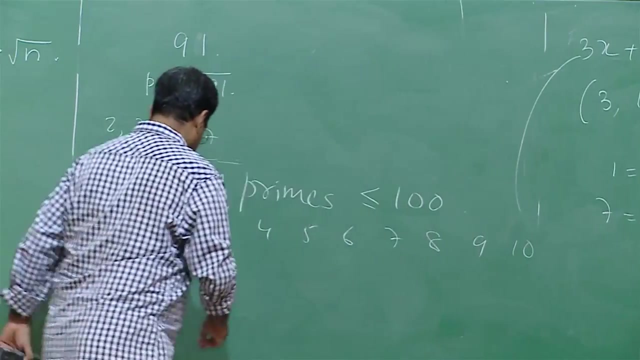 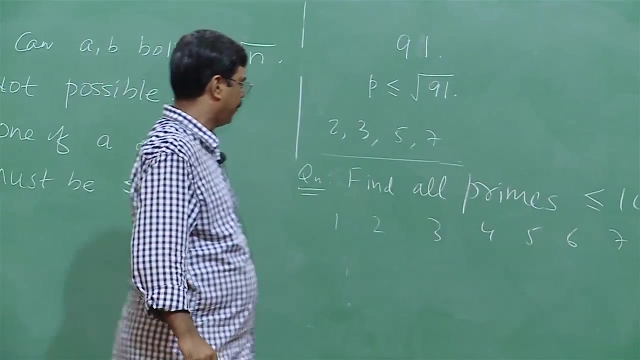 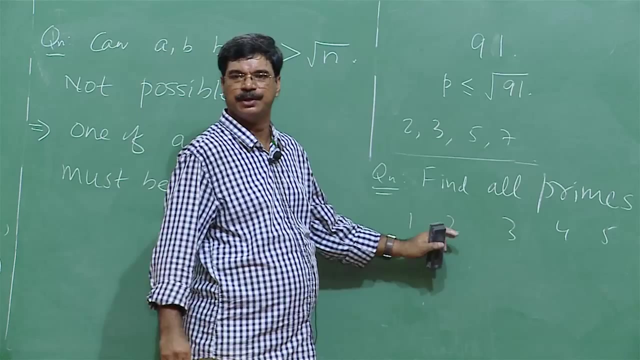 all primes? this is a question. so what we do, we will make a table of numbers, 1 to 100,: 1, 2,, 3,, 4,, 5, 6. And go on like this. so here is 100, and we are given only these primes. now, sorry, first, 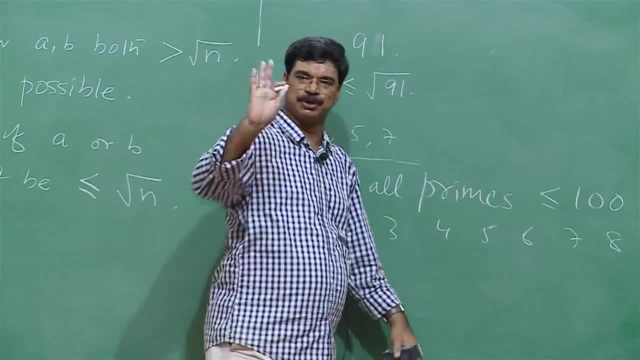 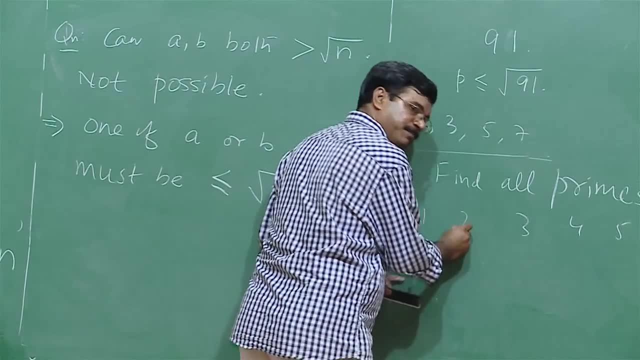 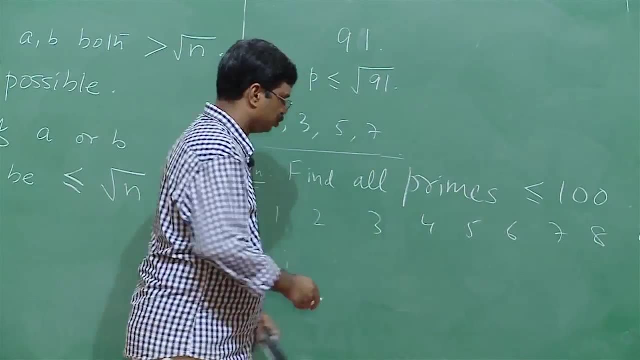 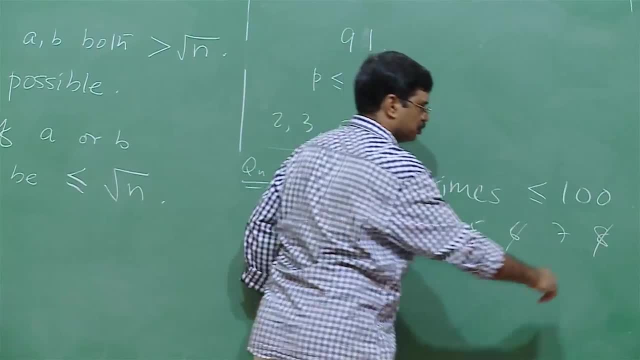 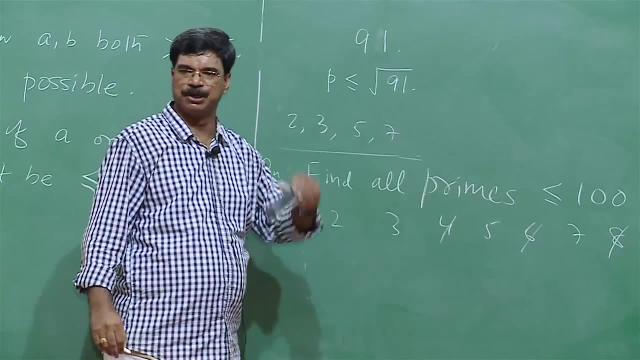 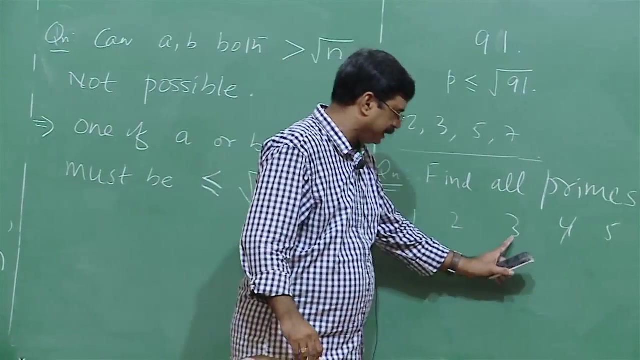 goes away. 6 goes away. 8 goes away. 10 goes away. okay, retain this. 3, remove all the multiples of 3,. so 6,, 9 and so forth goes away. retain this 5, remove all the multiples. 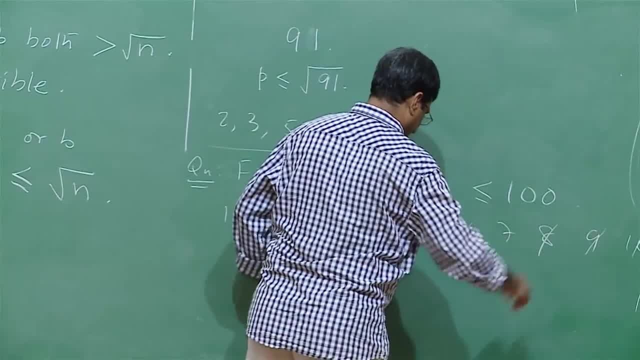 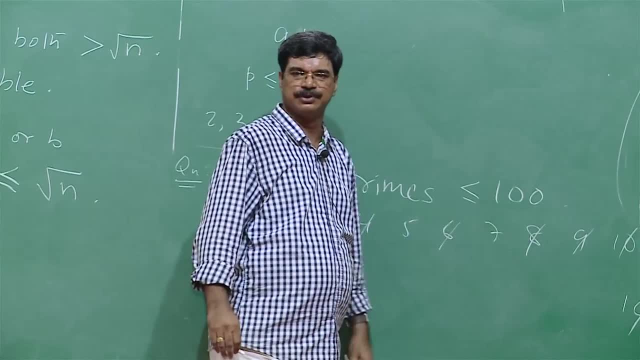 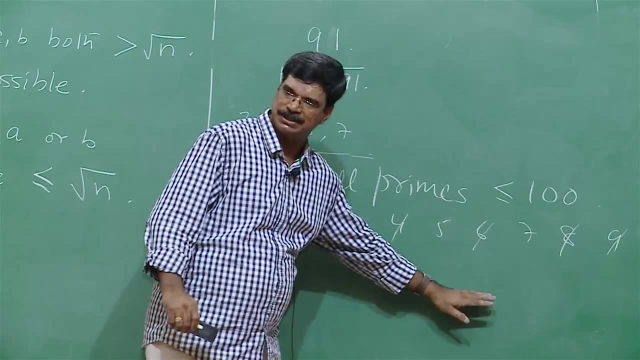 of 5, okay, So 25 and all this 15, all these numbers goes away. retain this 7,, remove all the multiples of 7, that is all we have to do. So many numbers have gone away, but still some numbers are remaining here, okay, and 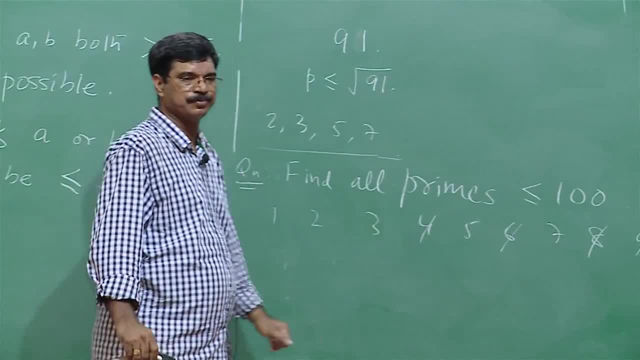 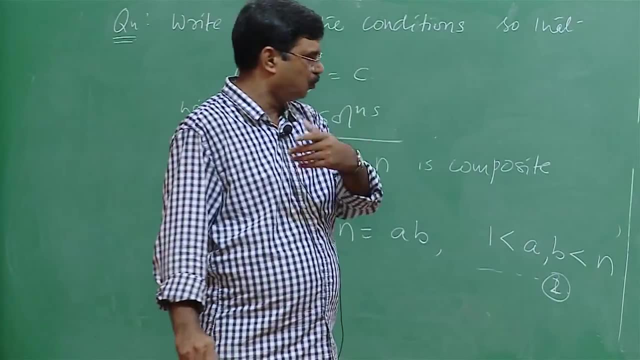 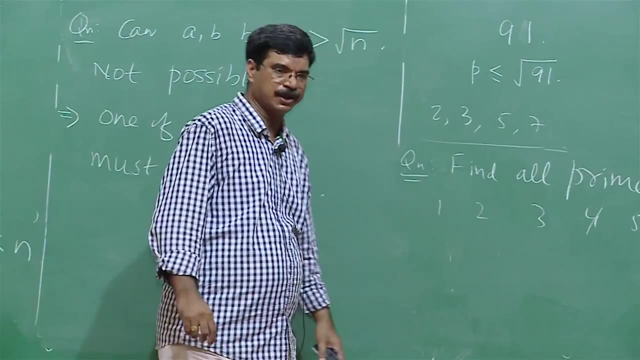 whatever number is remaining- they are all primes, sorry- 7,, 8,, 9,, 10,, 11,, 12,, 13,, 14,, 15,, 16,, 17,, 18,, 19,, 20,, 21,, 22,, 23,, 24,, 25,, 26,, 27,, 28,, 29,, 30,, 31,, 32,, 33,, 33,, 34,, 34,, 35,. 35,, 36,, 37,, 38,, 38,, 39,, 40,, 42,, 43,, 44,, 45,, 46,, 47,, 48,, 49,, 50,, 52,, 52,, 53,, 54,, 55,, 56,, 57,. 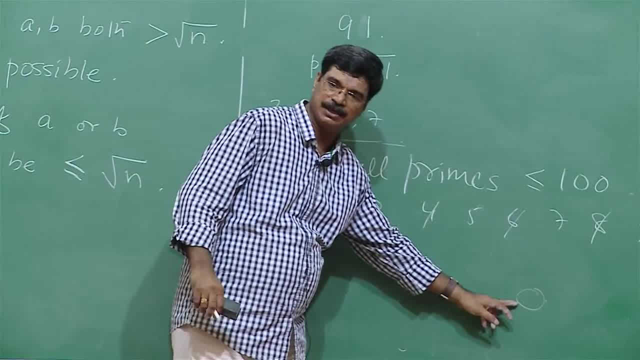 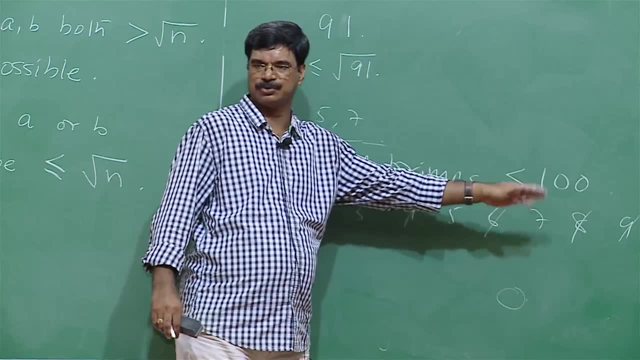 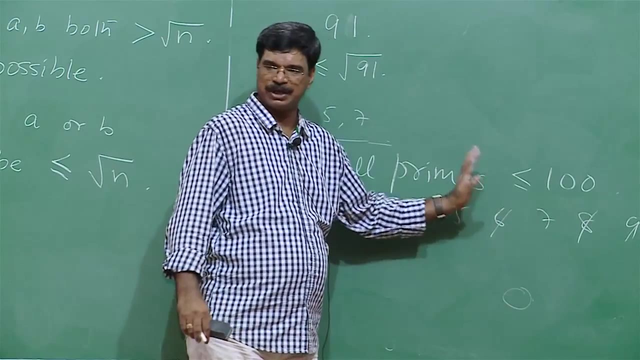 then it will have a prime divisor less than square root of this. but we have removed all the multiples of you know those numbers, so no composite number can remain unchecked, therefore, whatever is remaining. so we have got all the primes up to 100, now, if you want, 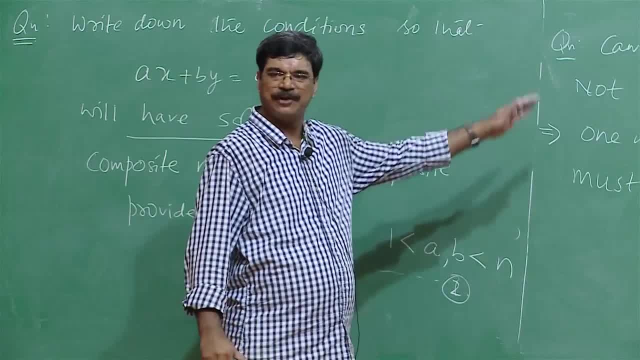 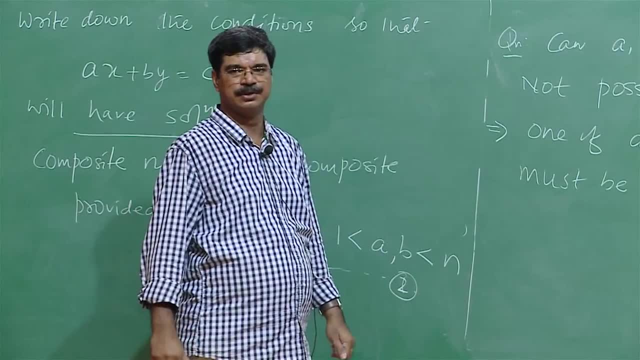 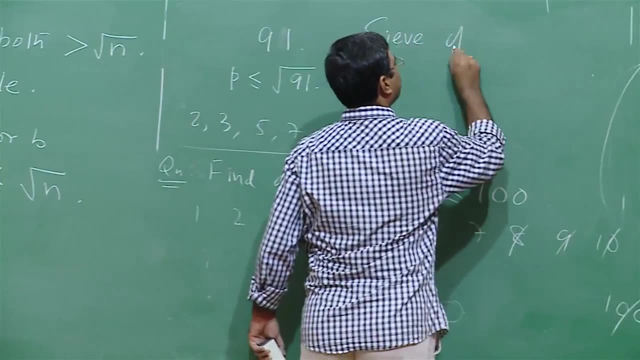 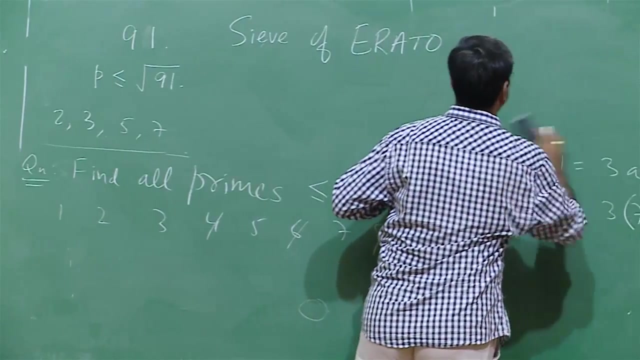 1000 or 10000. you have primes up to 100, make a table up to 10000 and keep doing that. okay, So this was given to us by CEO of Eratosthenes Eratosthenes, Eratosthenes, Eratosthenes. 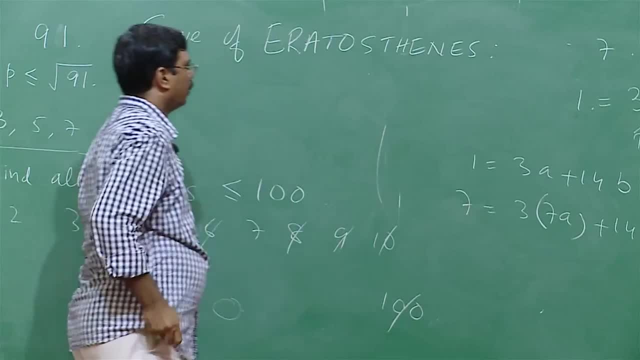 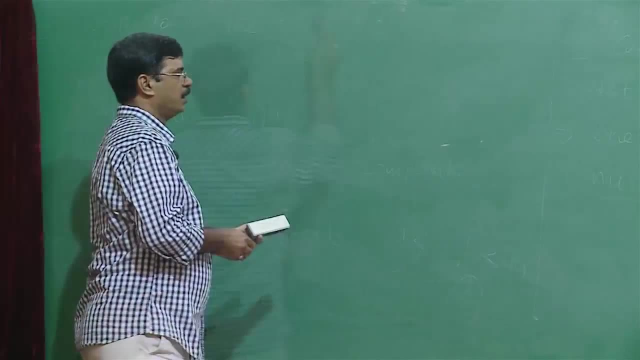 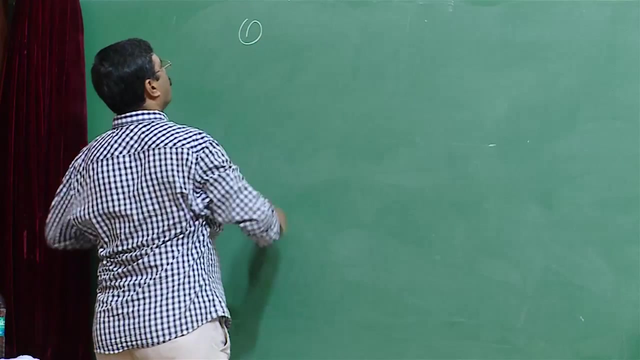 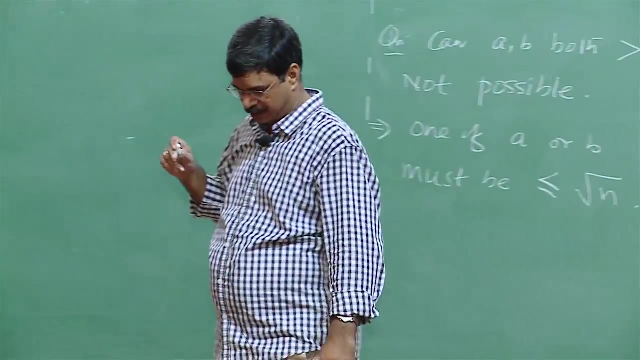 Eratosthenes, Eratosthenes. Okay, these are some of the important things. okay, Your now? the next concept is: yeah, yeah, another thing. let me, since I am talking about primes, how many primes are there? Total number of primes. total number of primes: infinite. 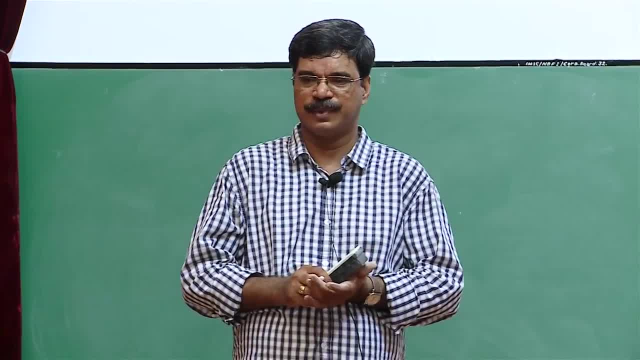 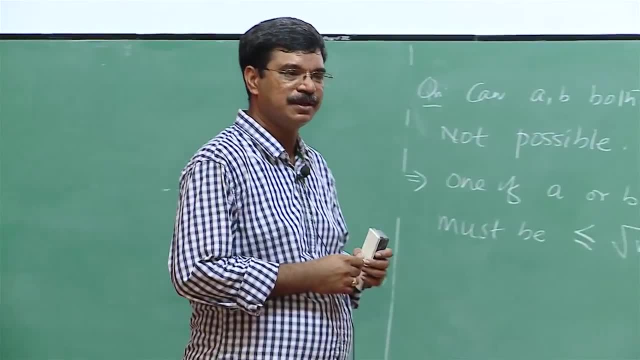 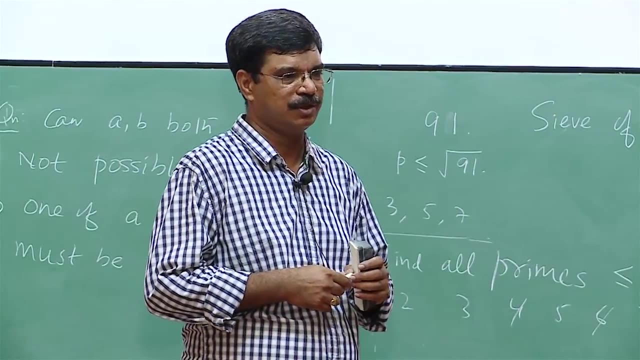 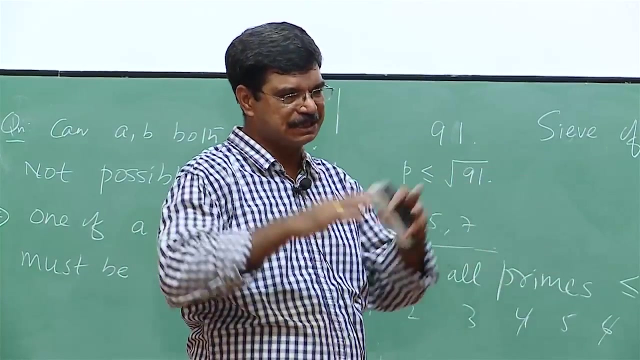 And how do we know that Numbers, No, numbers- are more than primes? no, No, no, no. that is, see, the set of numbers is much larger set than the set of primes. but if larger set is infinite does not mean that the smaller set is infinite. 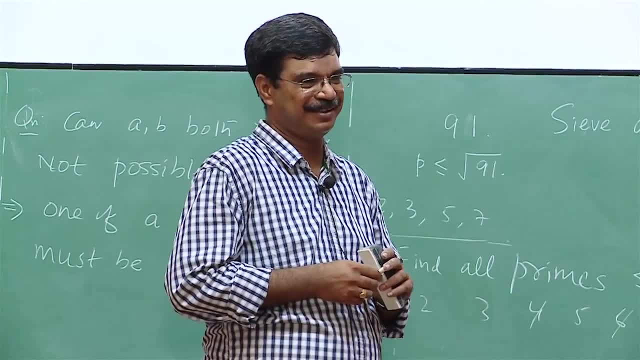 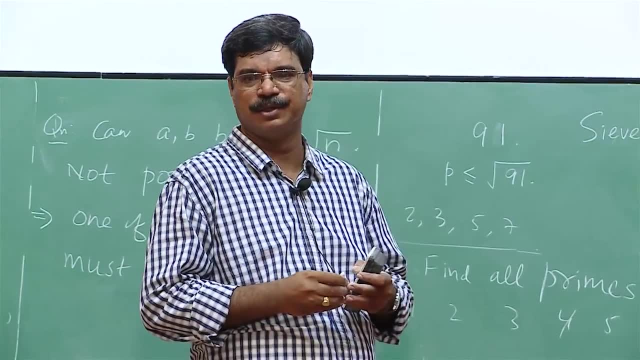 No, no. so how do we, you know? how do we know? I mean, can we simply prove, Taking One to one, correspondence between Between the multiples of two and the all the numbers set? So what is the set of numbers? 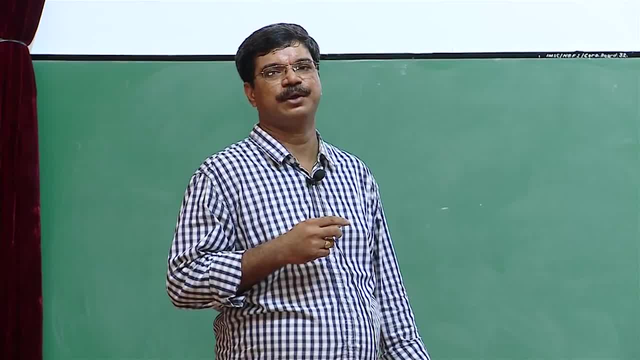 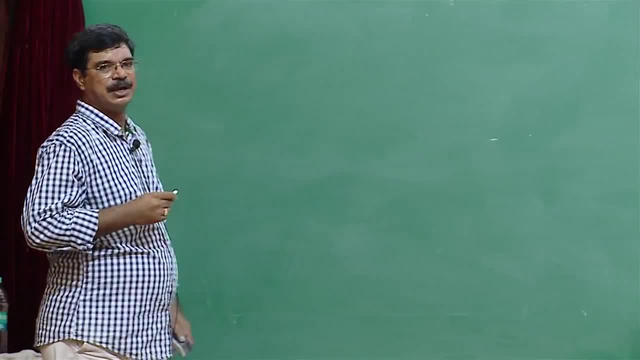 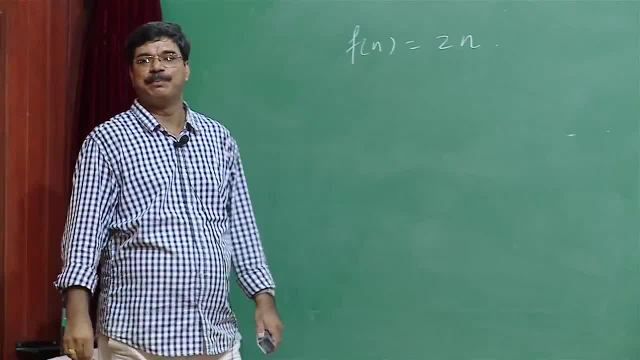 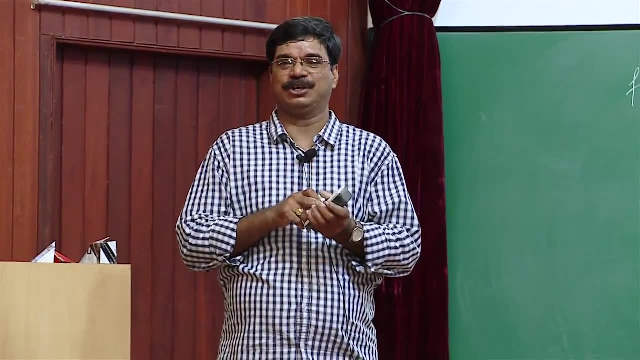 Which I have taken a subset. So f of n is 2 n Yeah, but you have shown the one to one correspondence with an infinite set. Infinite, Therefore it is infinite. but can you show an one to one in correspondence between: primes and integers. We cannot, because we do not know where is the next prime lies. primes do not follow any regular pattern. Yes, k factorial plus 1 need not be a prime number. it may be a composite number. It may be a composite number. yeah, it is not divisible by all primes up to k. 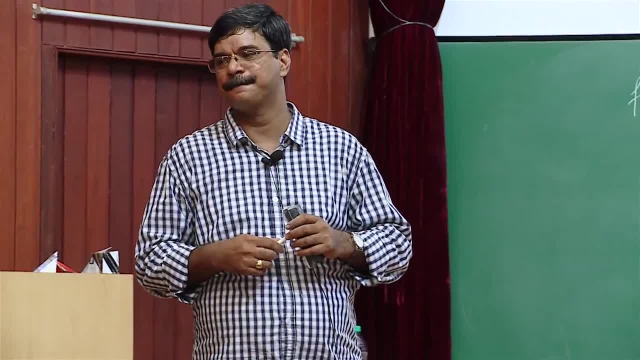 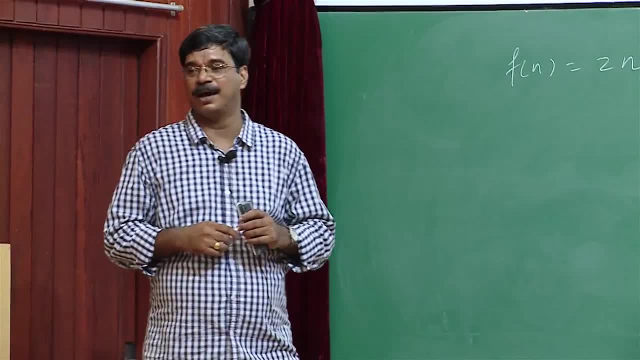 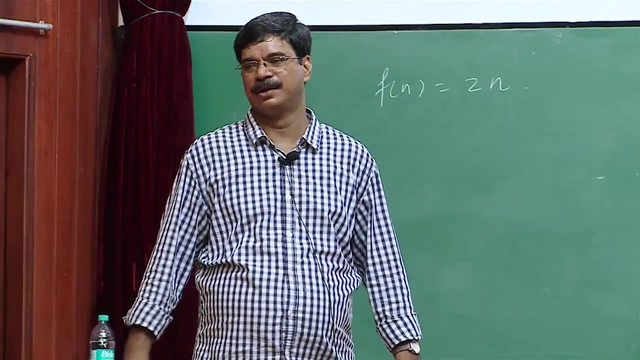 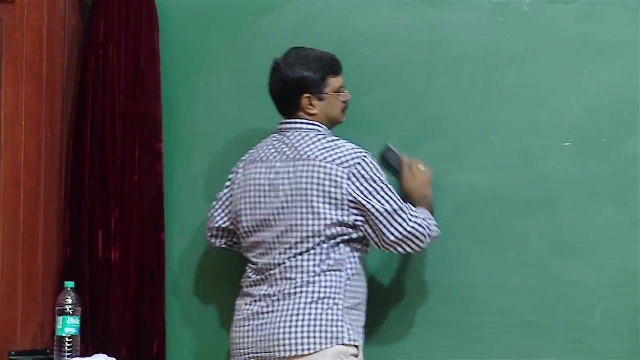 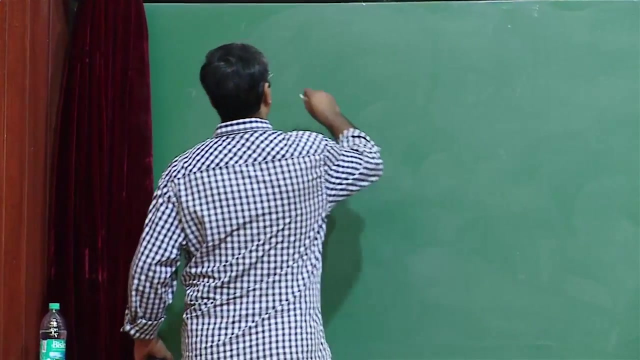 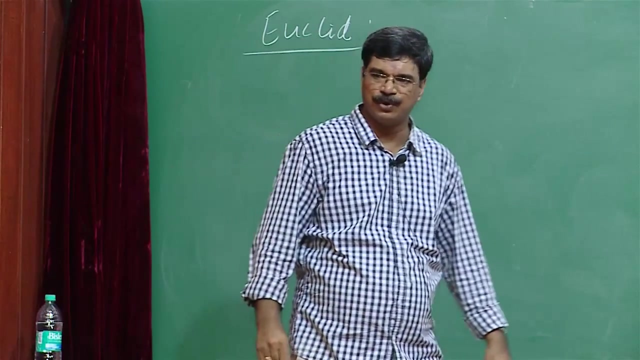 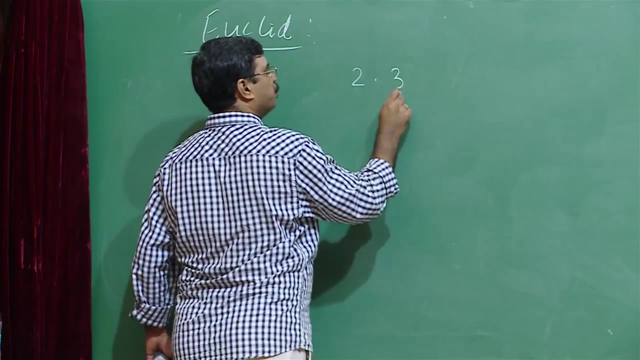 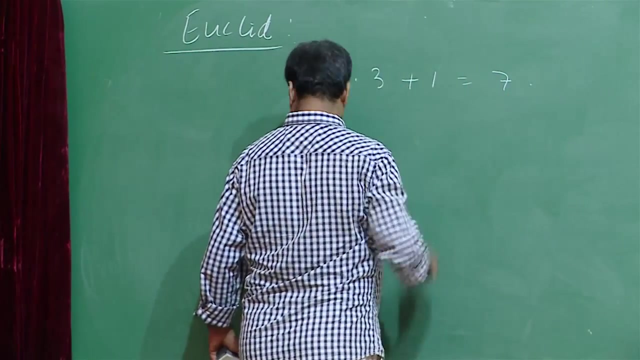 So there is some assumption here, suppose: ok, so right, so again, again, this goes to Greeks. ok, So what is the argument? Yeah, I am explaining your argument. What Euclid, again he did, was you look at the number 2 into 3 plus 1. ok, this is 7.. 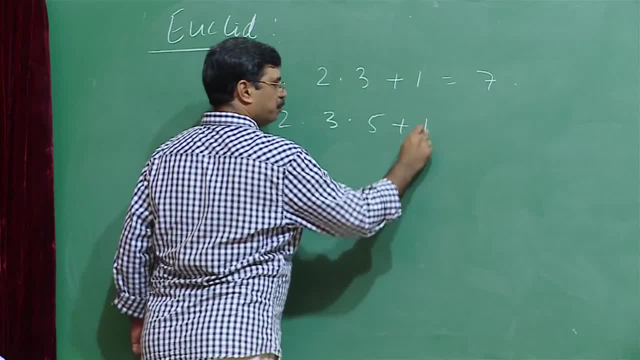 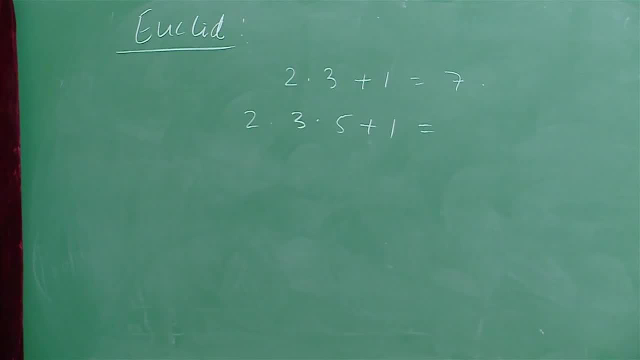 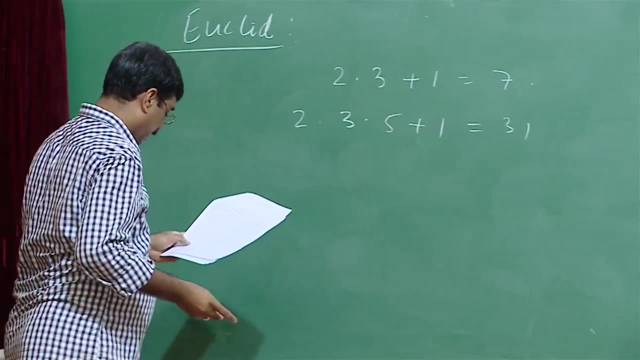 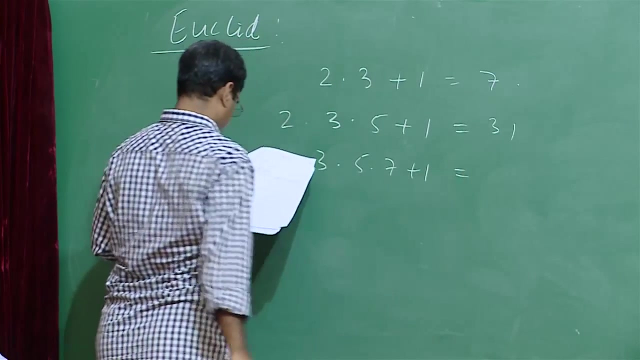 Now 2, 3, 5, ok, So let me write it down to save time. This is 31, and then 2 plus 2 into 3, plus into 5, into 7 plus 1, this is 211, 2 into 3, 5,. 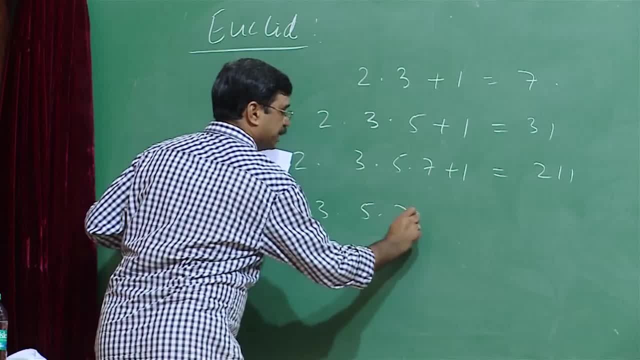 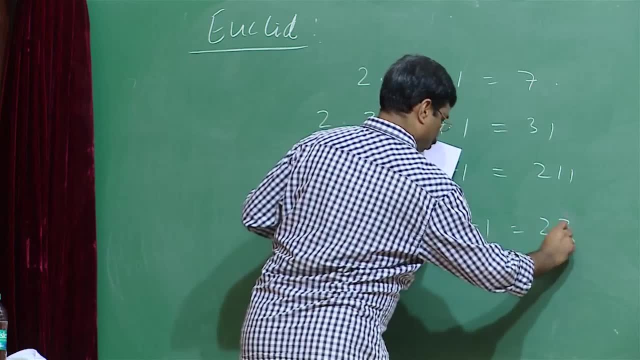 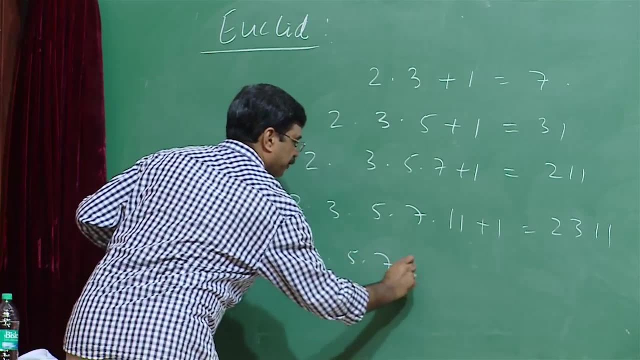 7. Ok, Ok, Next prime is 11 plus 1, 2,, 3, 1, 1,. take one more prime: 2,, 3,, 5,, 7,, 11,, 13 plus 1,. 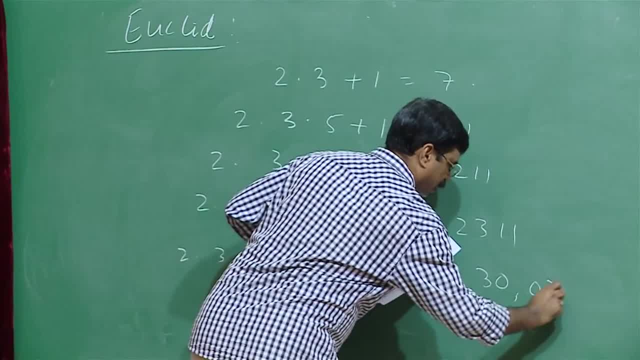 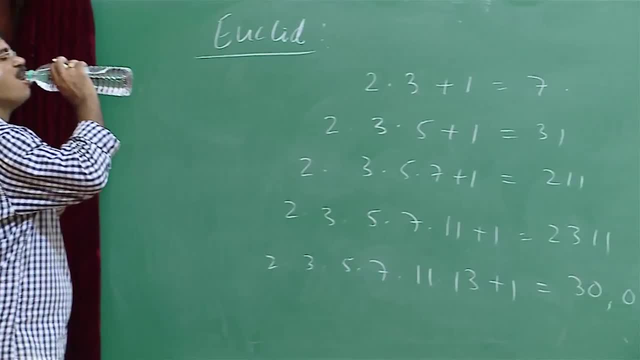 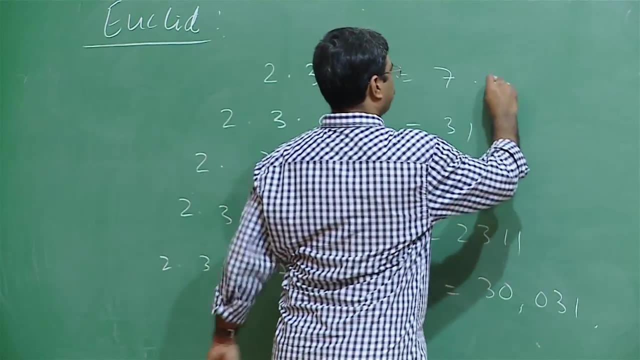 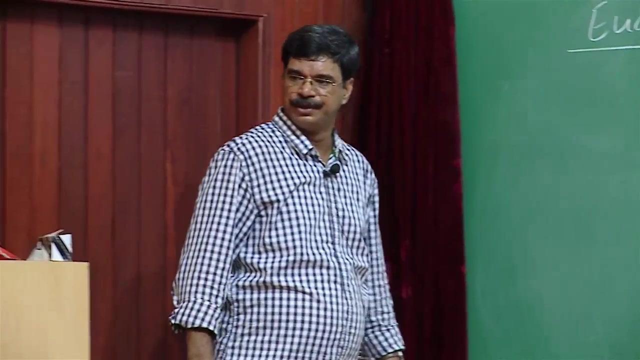 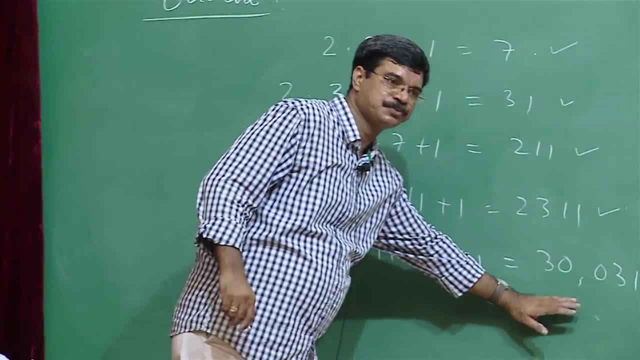 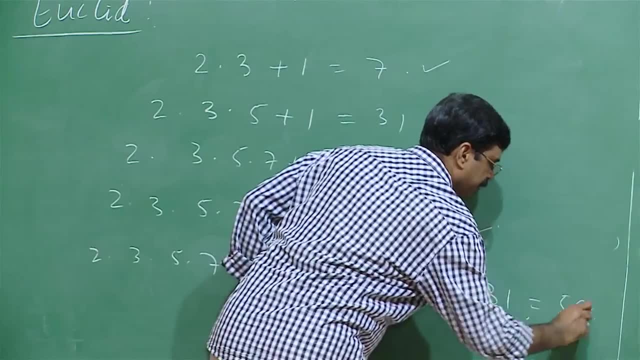 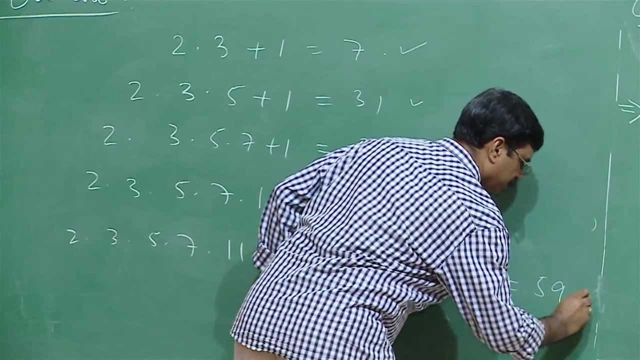 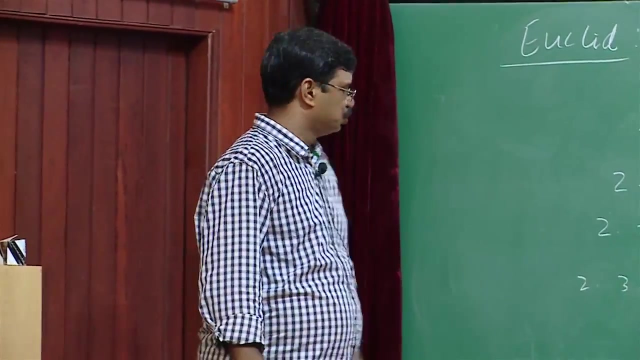 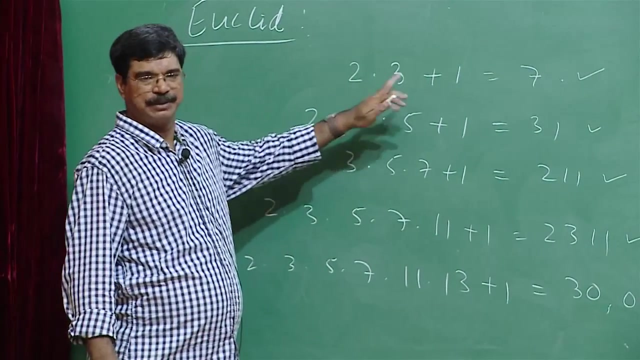 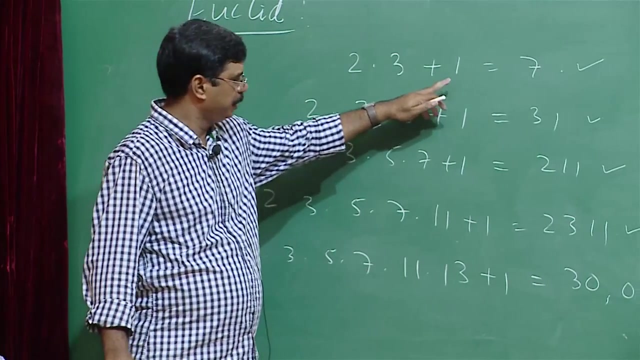 Ok, But this is not a prime number. ok, You can show that this is a multiple of 59 times 509, I suppose 509.. Ok, Ok, 509.. So what was the argument of Euclid? You look at all the primes, Add 1 to it. In all: 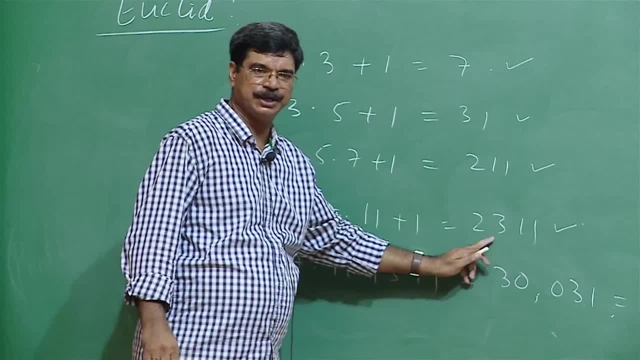 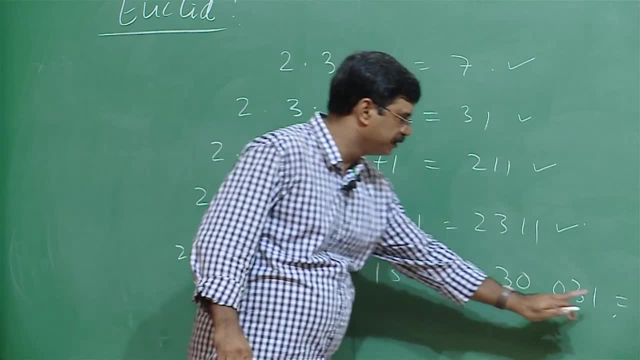 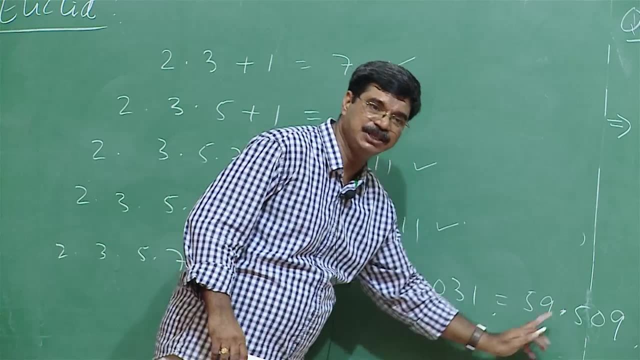 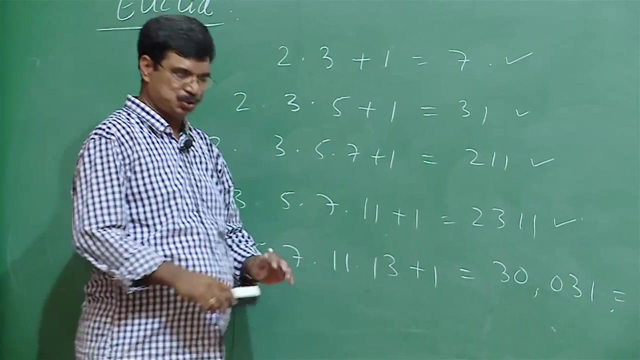 these cases you got a new prime. In this case you got a number which is composite, but it is a product of two numbers. This is a prime, this is a prime, and these primes are bigger than 30. So the Euclid's argument is: 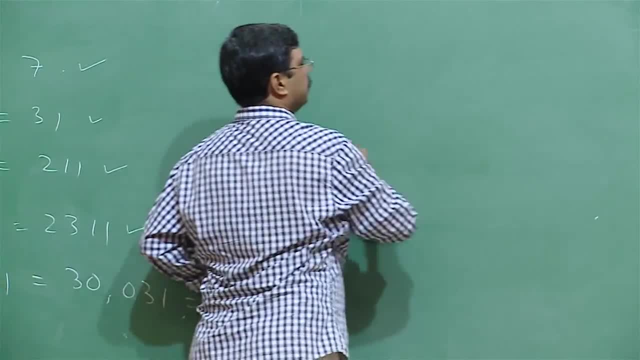 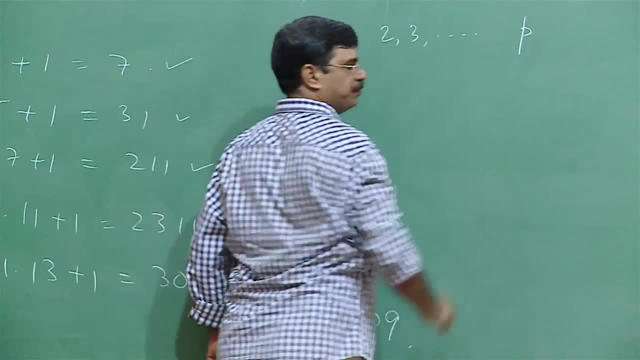 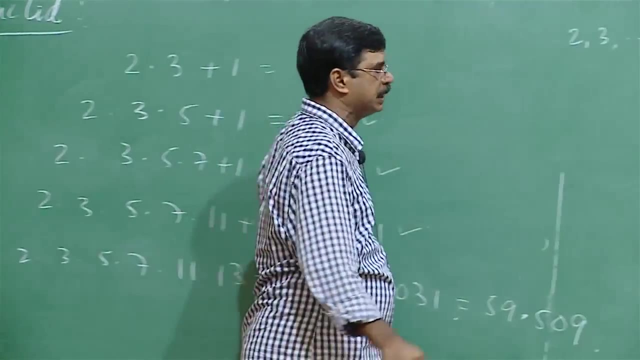 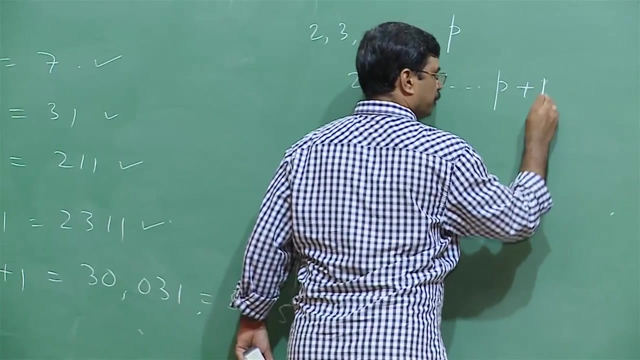 Given a set of primes, let us say 2, 3, up to p. you are given a set of primes, p prime. P is the up to p primes you are given. You form the number 2,, 3,, 5, up to p plus 1.. Call. 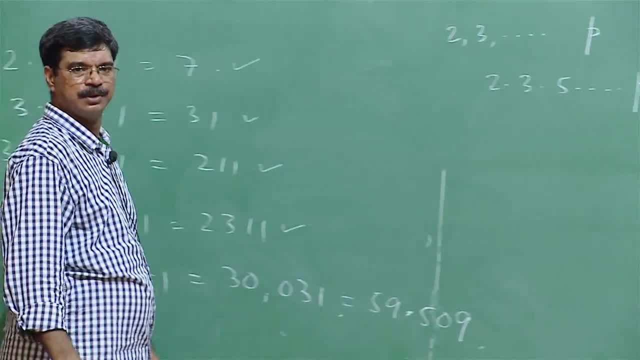 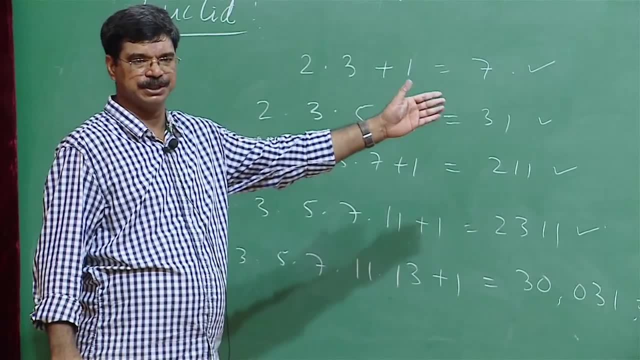 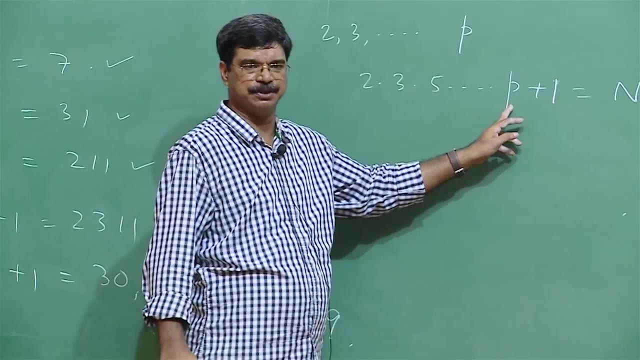 this as n. Two possibilities for Euclid: Either it is prime or composite. If it is prime, certainly it is larger than p, much larger than p, because it is the product of all this plus 1.. But one, but supposing it, 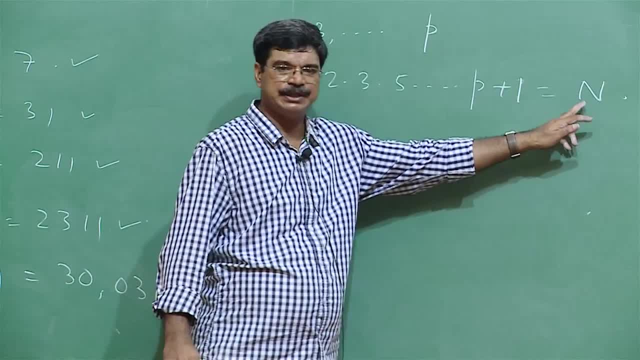 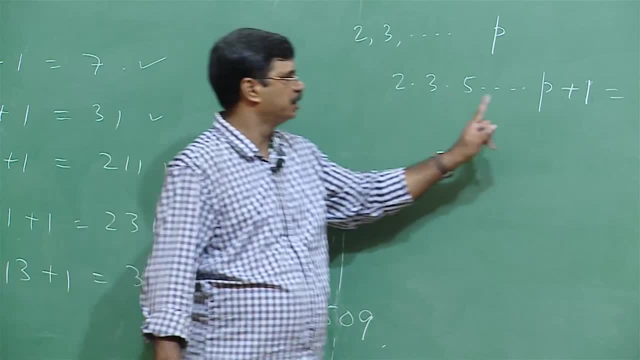 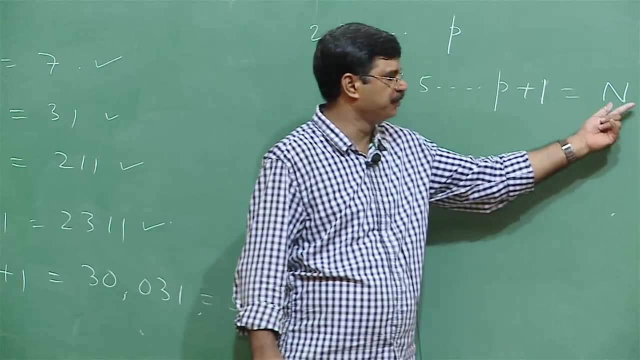 is composite, then it is not divisible by 2.. It is not divisible by 3. Because n cannot be divisible by 2.. Because … because this number is divisible by 2.. If n were divisible by 2,, then this number minus. 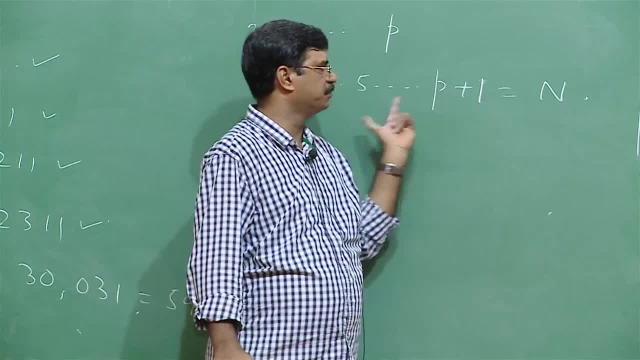 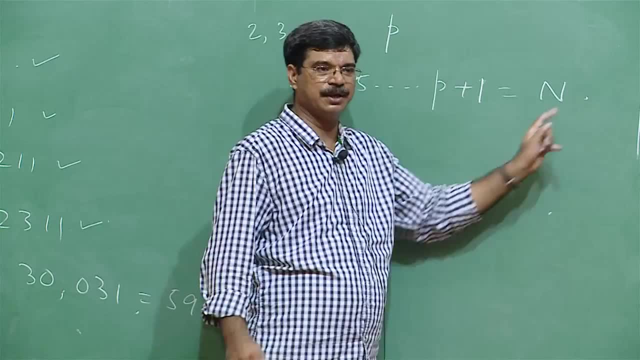 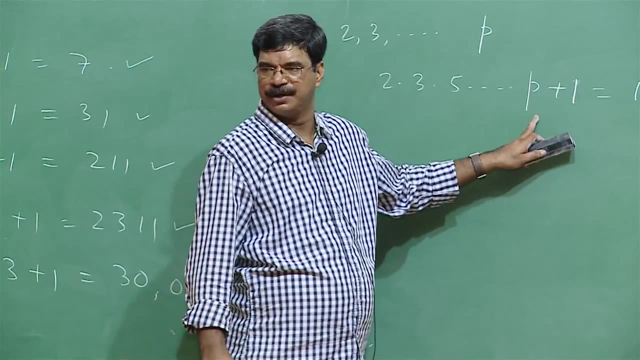 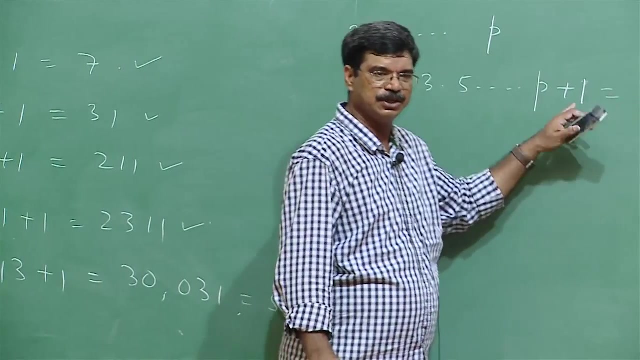 n will be divisible by 2, but this number minus n is 1.. Therefore, n is 2 does not divide n. 3 does not divide n. by the same reasoning, p also does not divide n. If p divides this, p divides n and p divides this, then p will divide the difference and the 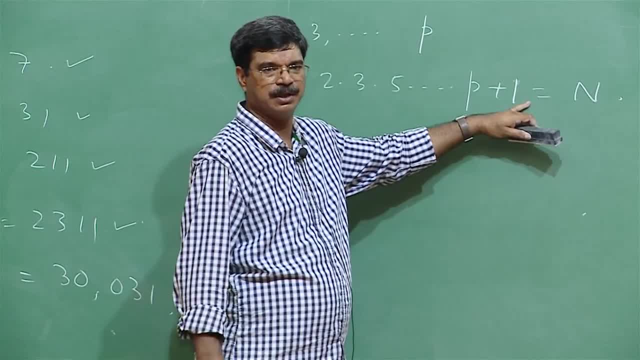 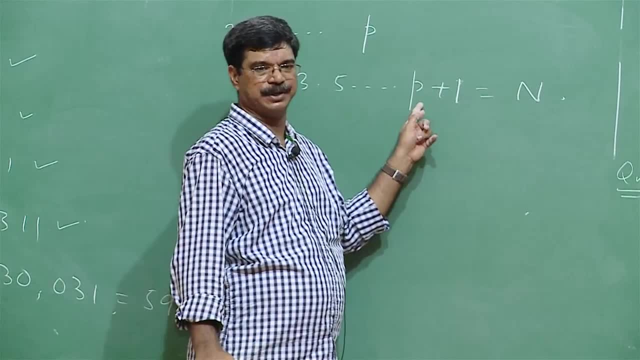 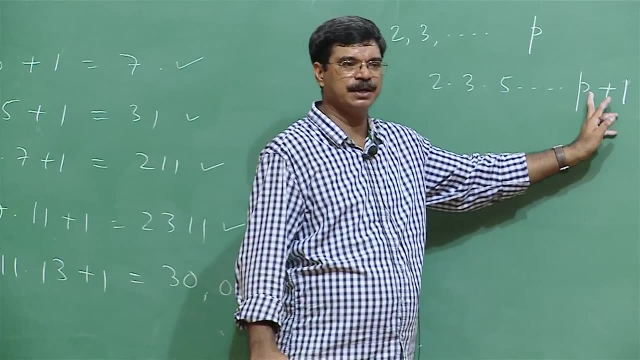 difference is 1.. Therefore, p will divide 1,, which is not possible. Therefore, n has a prime factor which is bigger than p. In either case, we have exhibited a prime which is bigger than these primes. So one more prime. So therefore it shows that there 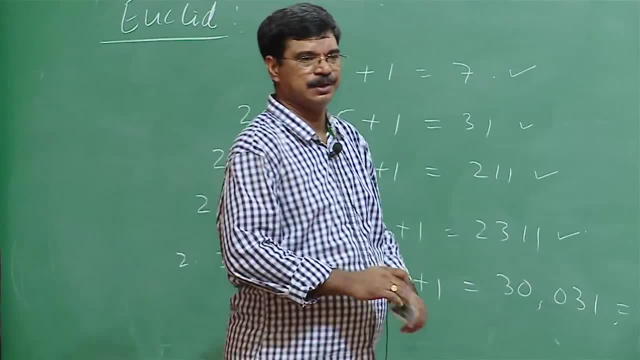 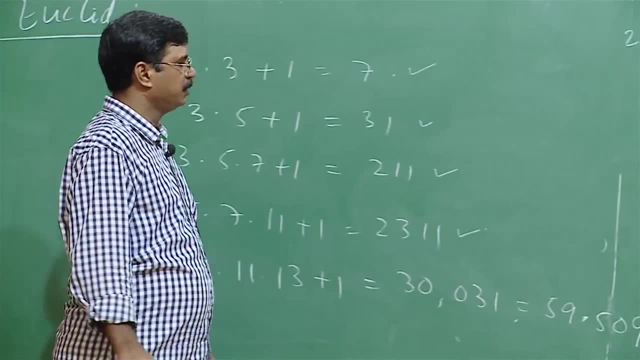 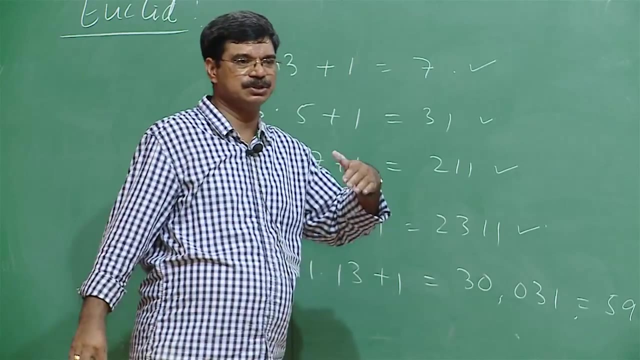 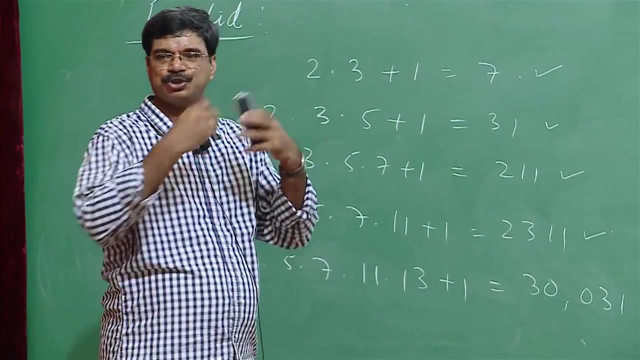 are inferences. So this is the brilliant idea of Euclid, And this is so simple and elegant that it has percolated to us from civilizations to civilizations. the novelty of this idea. What is the most natural way of showing that something is infinite? You look at the next element. 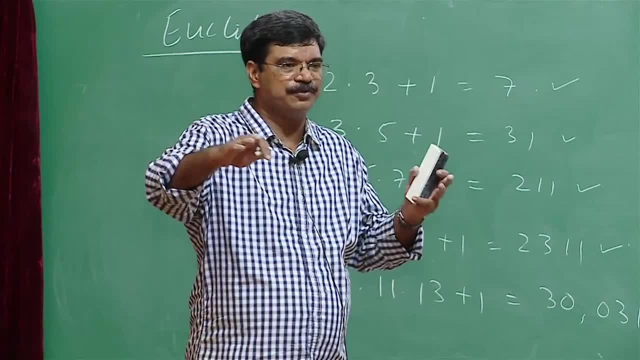 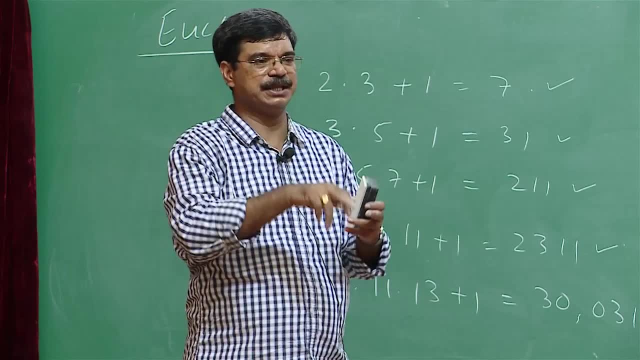 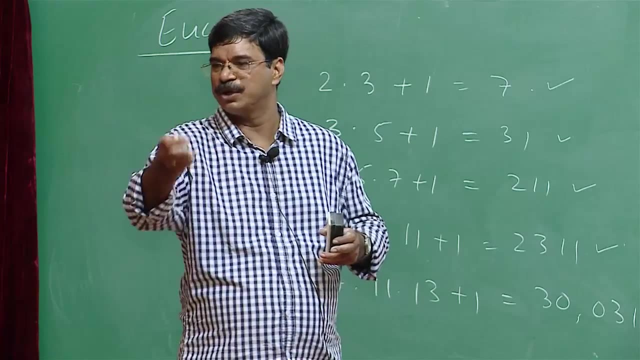 Number of natural numbers is infinite. So you take n be the largest, add 1 to it. That is again a natural number which is bigger than n. Therefore there is a contradiction. that n is the largest natural number. So you look for the next one. But Euclid did. 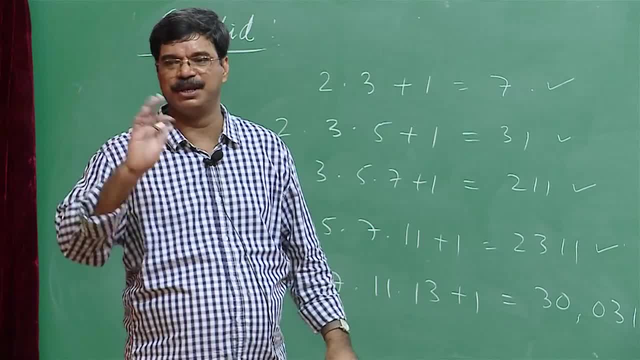 not look for the next prime. That is a brilliant thing, He said: let me not look for the next prime because I do not know where is the next prime. I look for a prime which will not be the next prime. I will look for the next prime. So I looked for a prime which is greater. 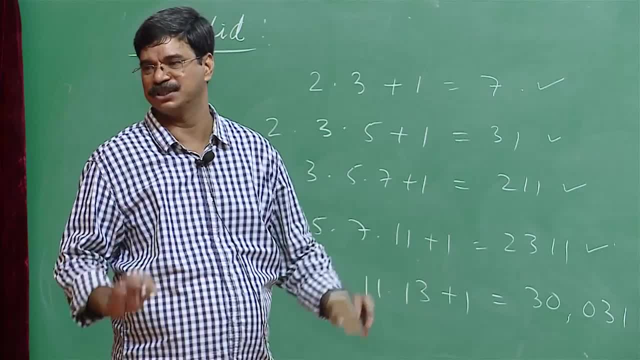 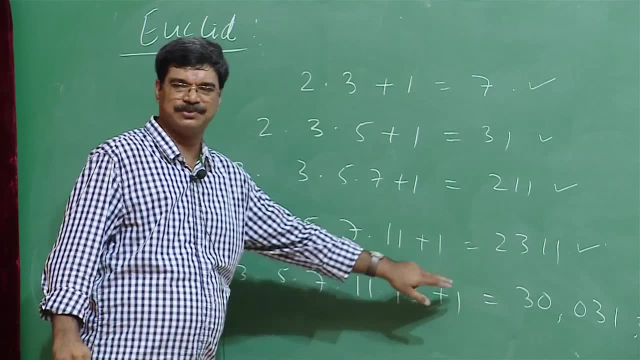 than n. I am defying to me that the number of natural numbers are not infinite, because I'm not prime which is bigger than the given prime, and he was successful Here. the next prime after 13 would be 17. he didn't bother about that. you know, I want a. 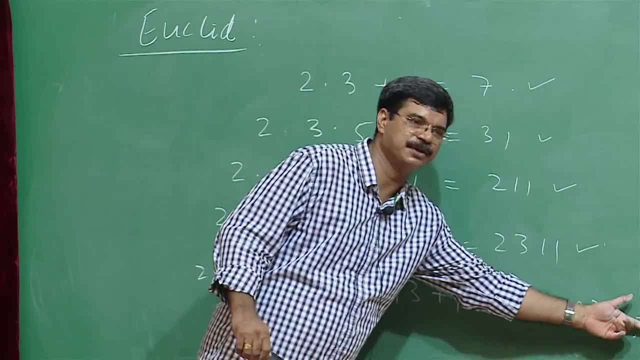 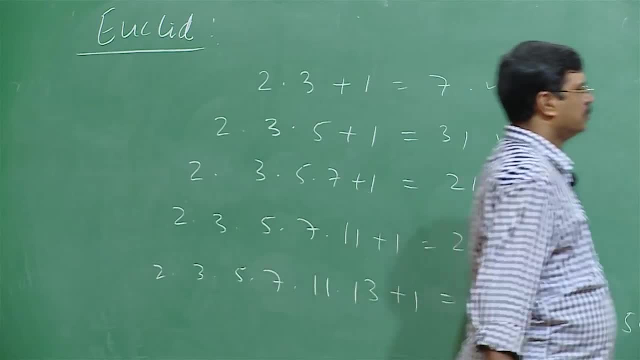 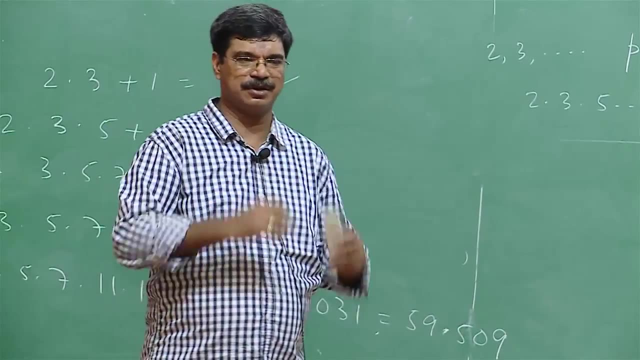 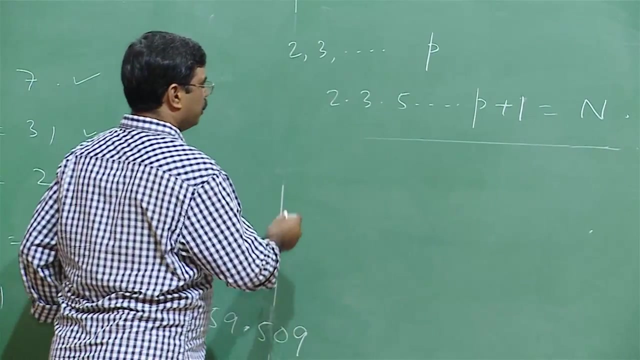 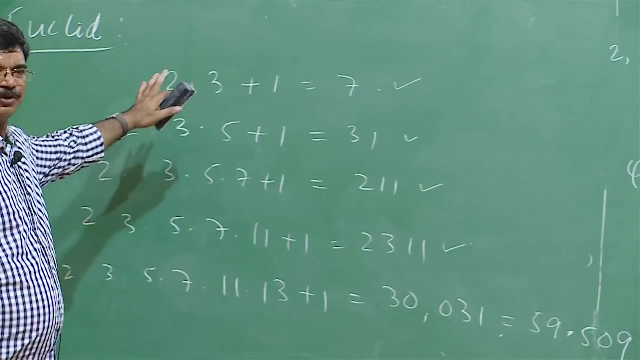 prime which is bigger than 13, which is 59, that's it and that you know. that's the brilliancy. okay, so it such ideas can come only if you have some feeling for the subject. okay, fine, There is a beautiful function, so there are. therefore, there are infinitely many primes. 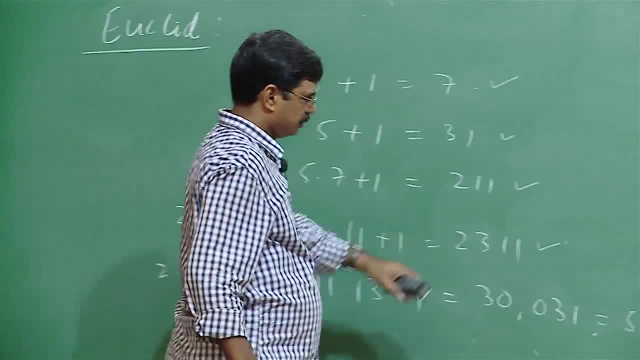 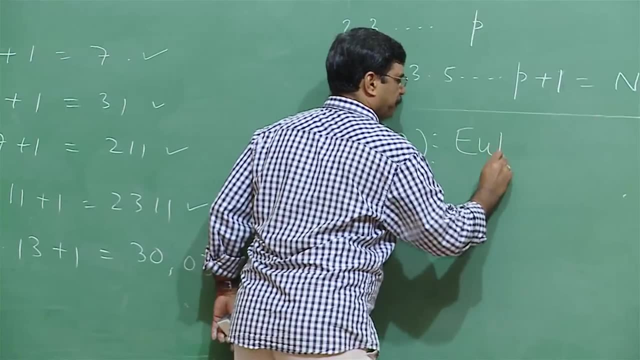 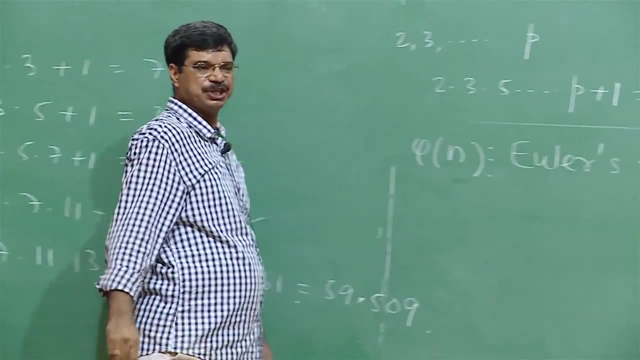 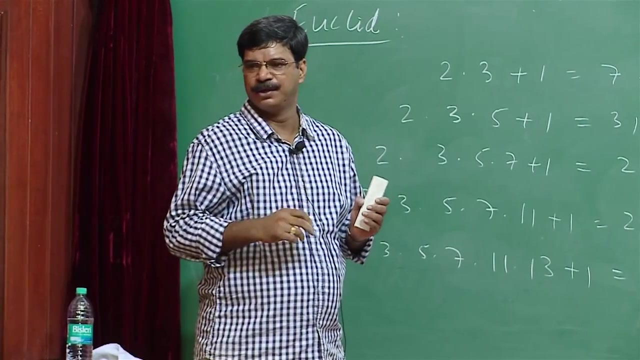 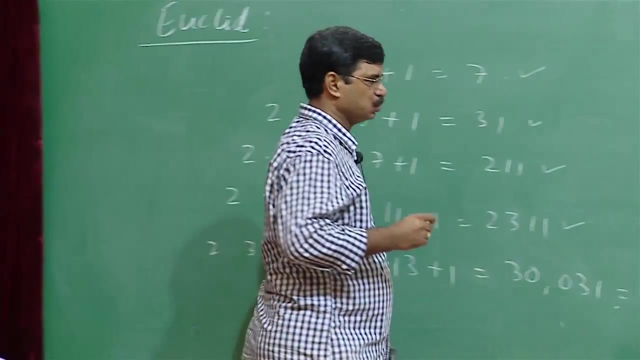 I will not go into details of that. This is a very Nice function. this is called Euler's torsion. Euler's torsion function: it counts the number of integers from 1 to n which are relatively prime to n. okay, So this is number of. 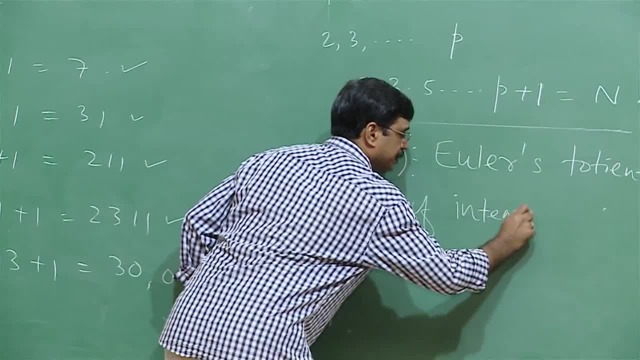 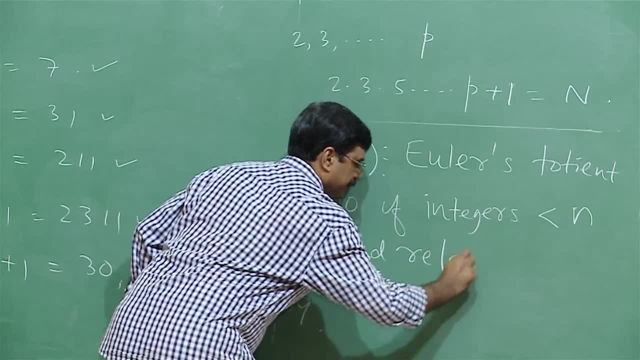 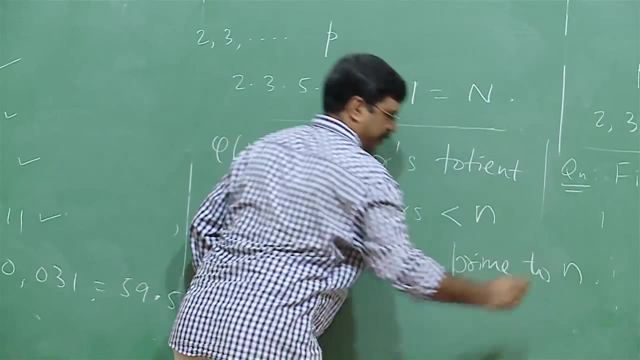 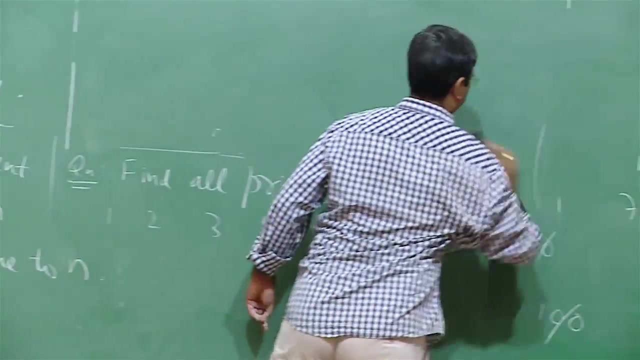 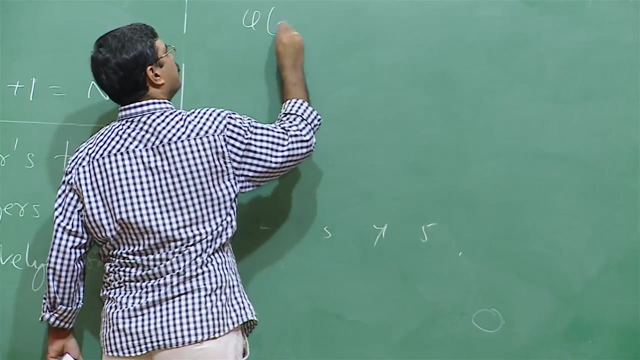 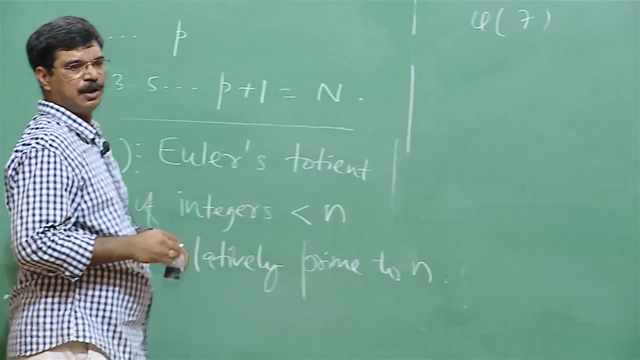 Integers: Integers less than n And Relatively Prime to n. For example, what is This? 5 of 7,? what is 5 of 7? All the numbers less than 7 which are relatively prime to 7, not. 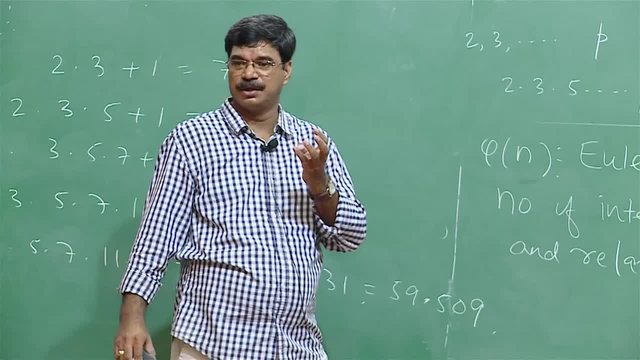 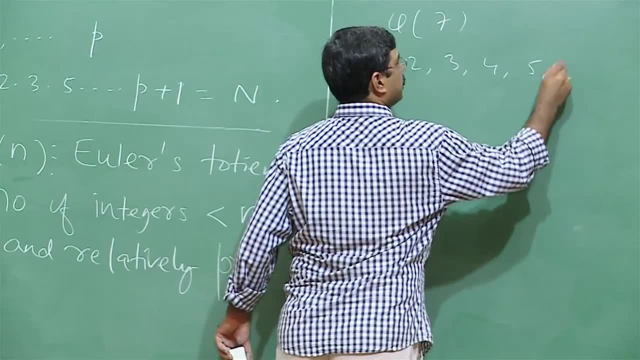 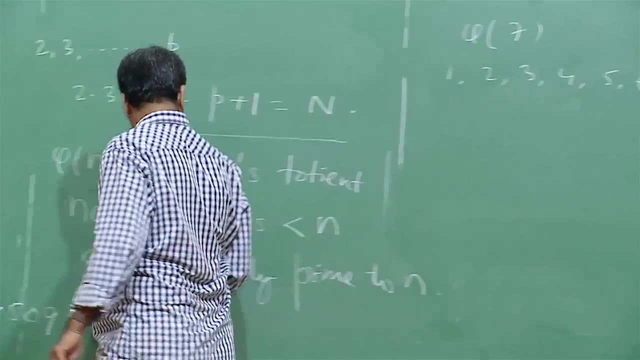 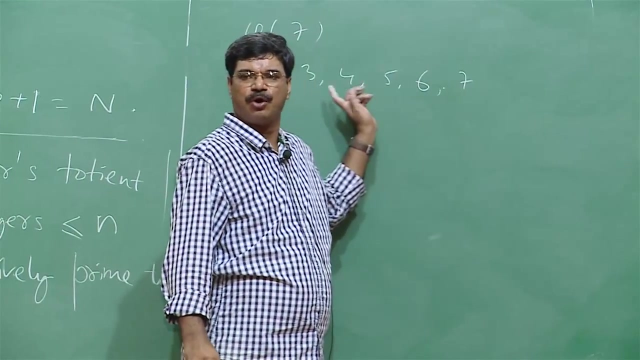 3,. answer is what See, I have to look at 1,, 2,, 3,, 4,, 5, 6, and let me write 7. also, let me write it less than or equal to, it doesn't matter. Of these numbers I want to look at. 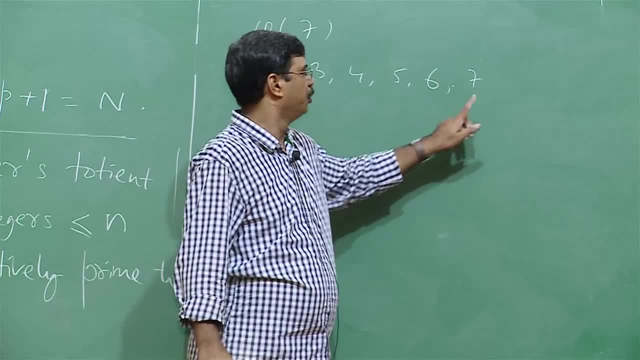 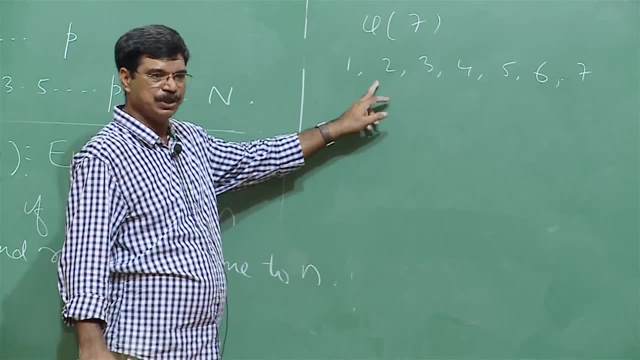 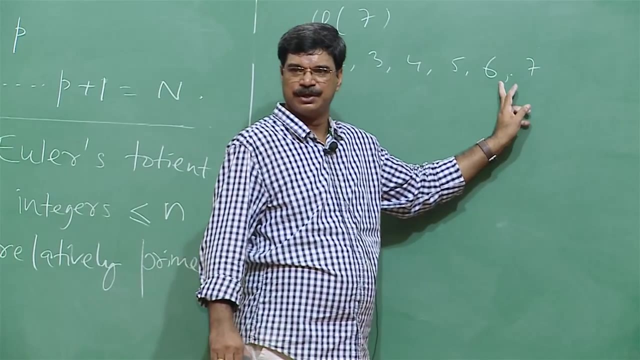 all those numbers which do not have any common factor with 7.. That means the only common factor should be 1, so 1 is a number, 2 is doesn't have any common factor, 3 doesn't have, 4 doesn't have, 5 doesn't have, 6 doesn't have. therefore, 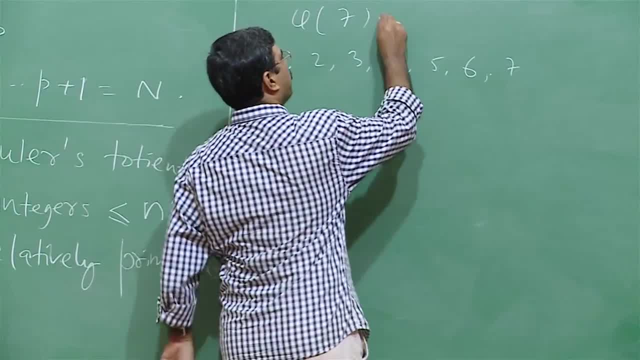 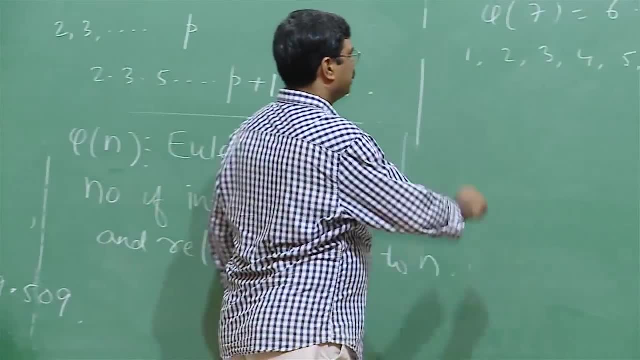 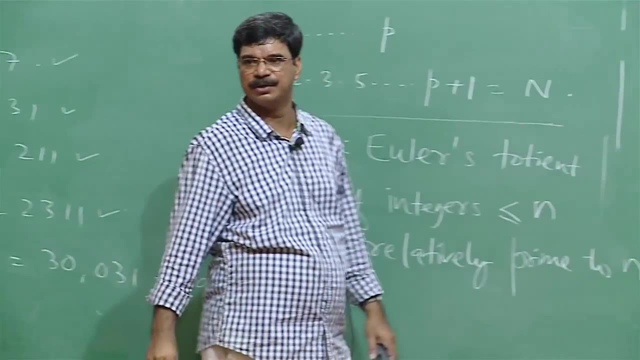 the total number is 6, okay, Given any prime pi of p, Okay. Okay Is p minus 1, because 1, 2, 3, up to p minus 1,, all the numbers, because p is a prime they. 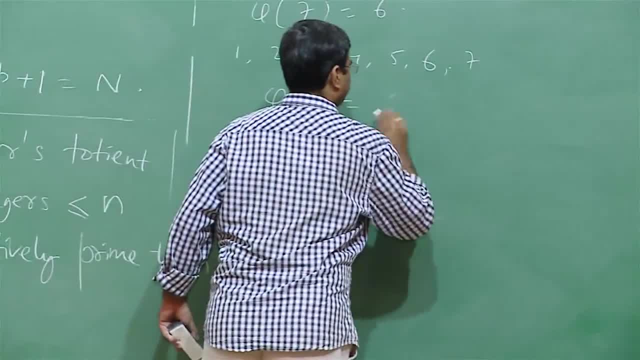 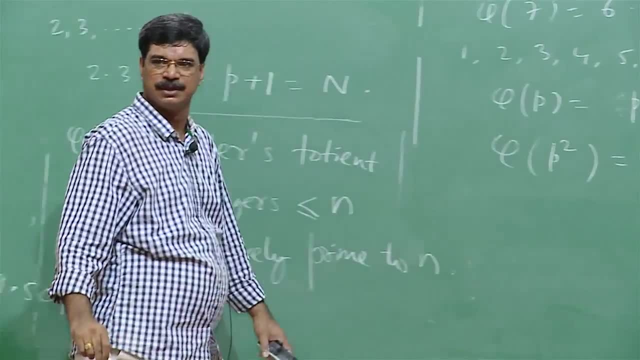 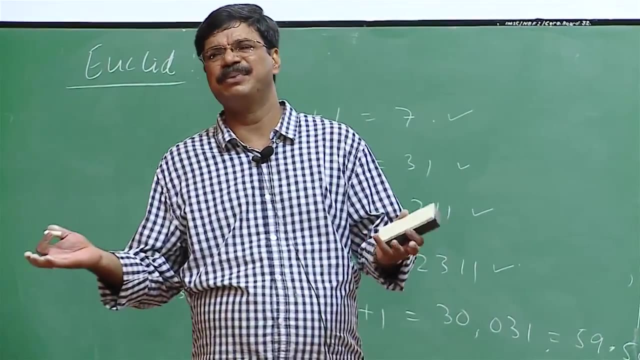 will not have any common factor, so it is p minus 1.. What can you say about phi of p square, Sir? Yes, Why do we take the number which is less than or equal to n? It doesn't make difference, We do not have to take that. 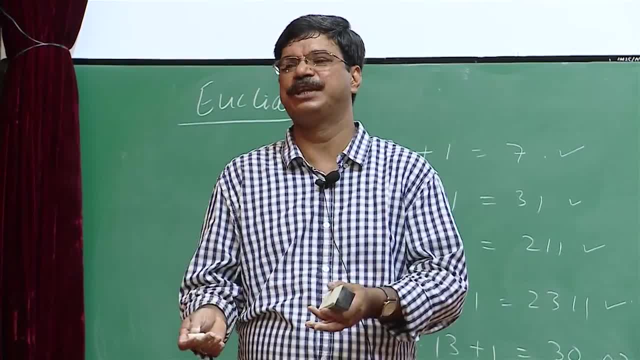 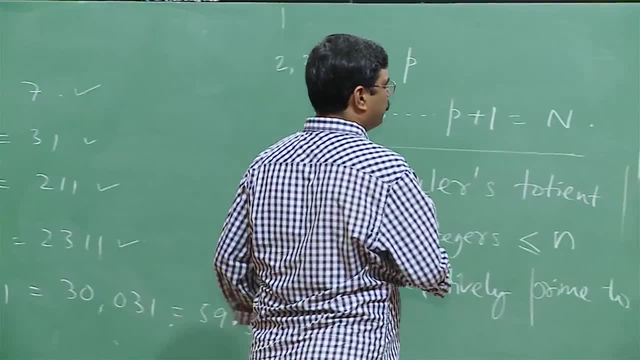 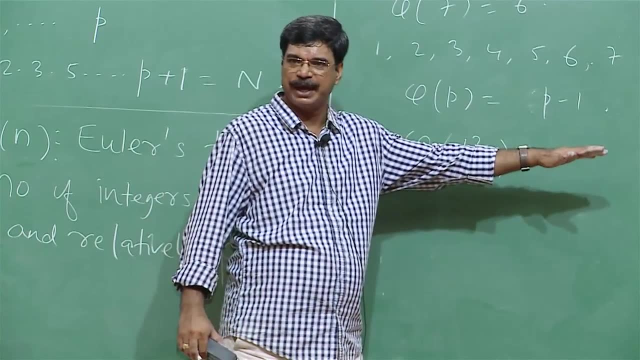 Yeah, That is not Yeah. So even if you take less than or equal to, it doesn't make any difference, that's all Okay. So phi of p square, for example. so 1,, 2,, 3, up to p square, how many numbers are there? 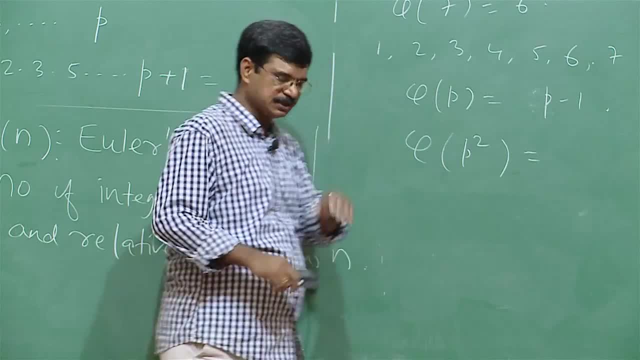 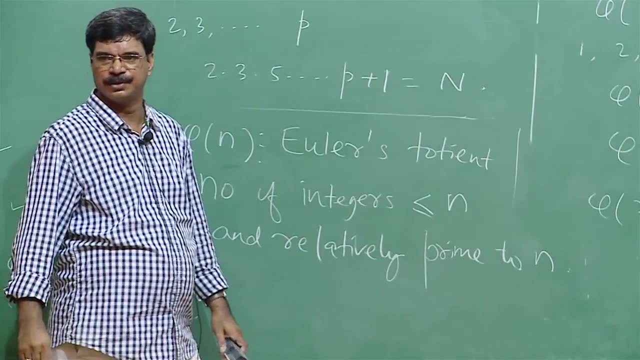 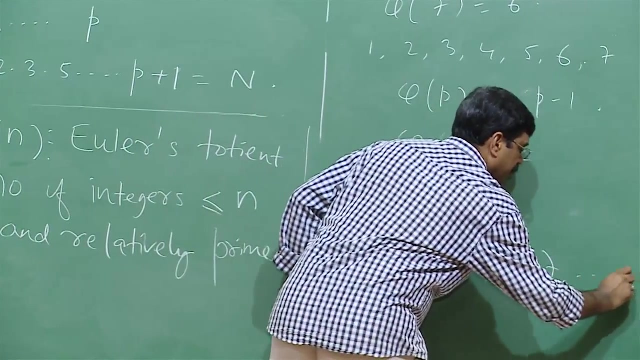 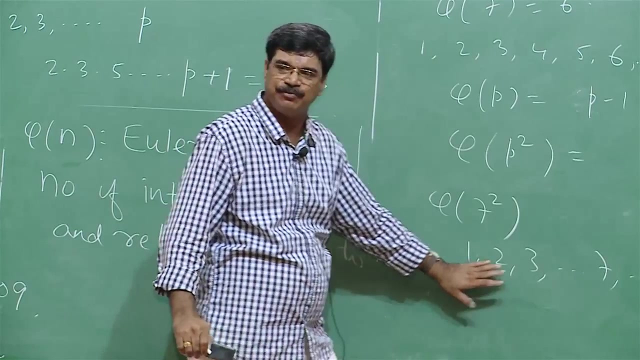 which are relatively prime to p square. Okay, For example, phi of 7, square 41. There are 49 numbers: 1,, 2, 3, there is 7, up to 49.. Of this, how many are there which are which do not have any common factor with 49?? 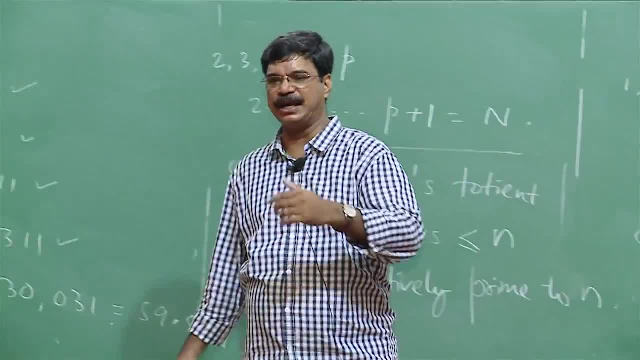 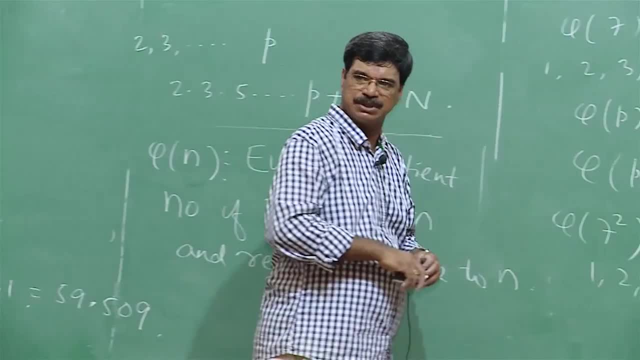 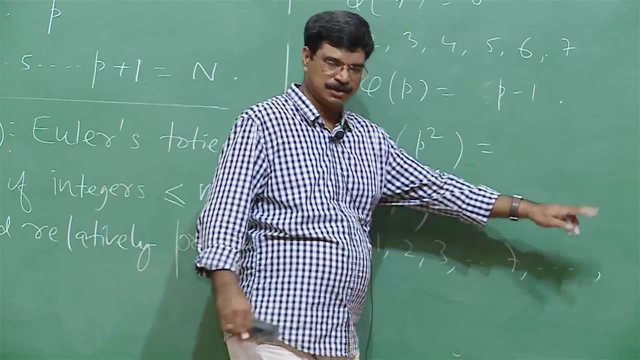 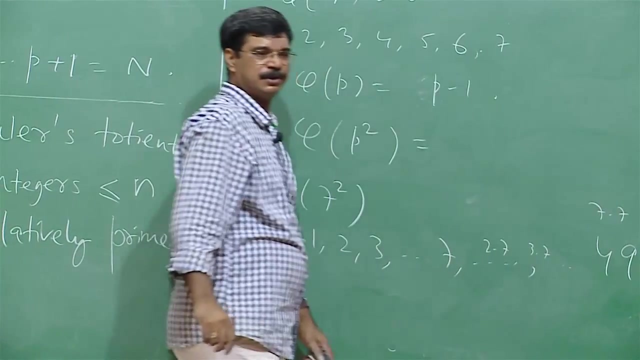 So easiest thing will be: first find out how many are there which have something common with 49. Okay, And then remove those numbers: 7.. 7 has 14 has 14 has So 7.. 2 times 7, 3 times 7 and this is 7 times 7.. 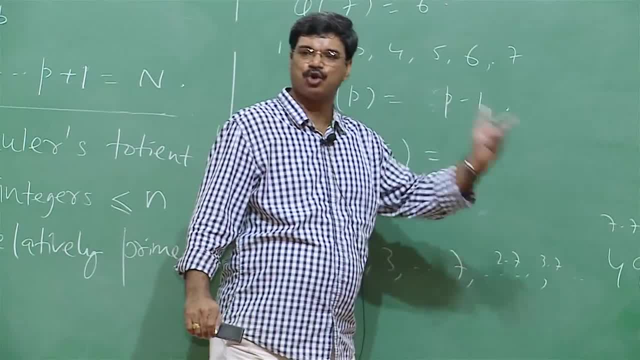 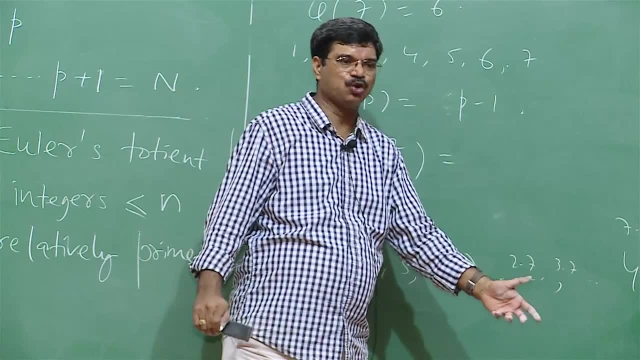 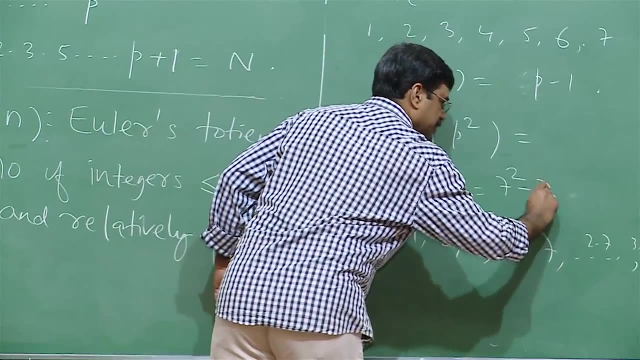 So there are 7 numbers which are not co-prime to 49.. Therefore, total number of numbers minus the numbers which are not co-prime will give you the total number of co-prime numbers. So this is 7 square minus 7, okay. Therefore, in general, you can show that this is p square. 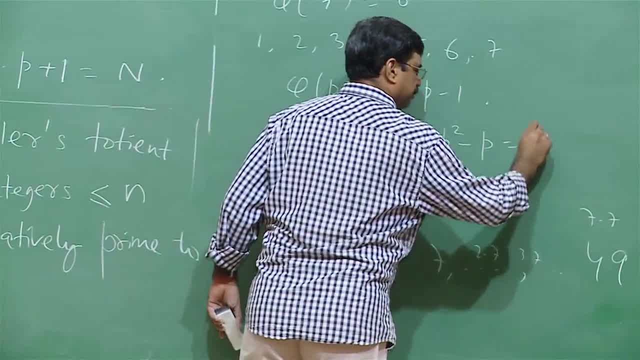 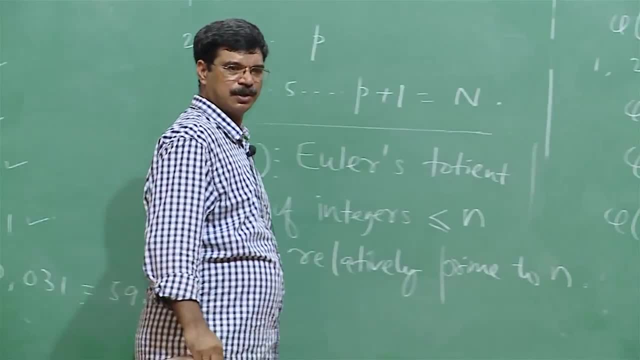 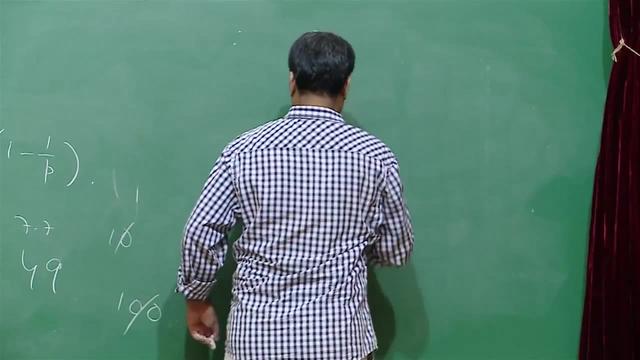 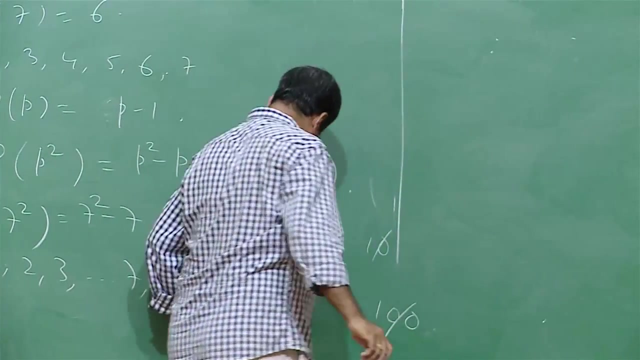 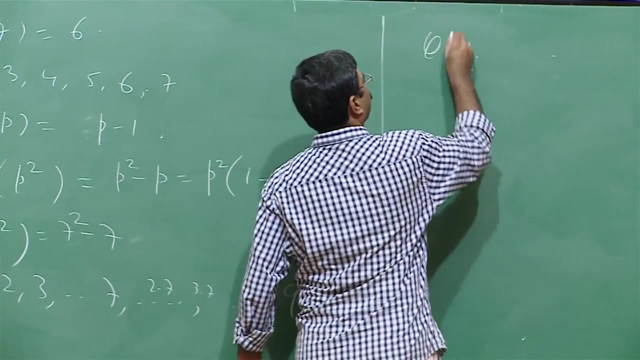 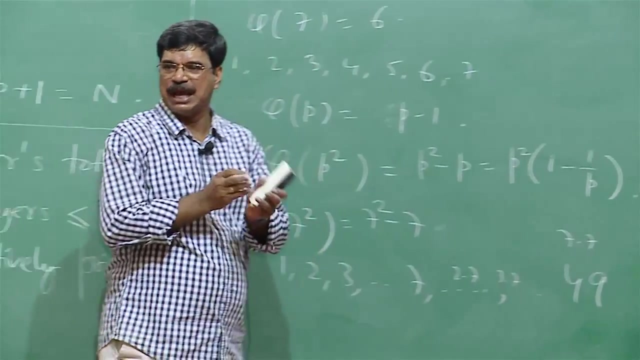 minus p. Sometimes you can write it as p square 1 minus 1 by p. okay, I will just take few more minutes because I have started late also. okay, Now another thing: phi of p- q. let us have suppose phi of p q, 2 primes, p and q are primes. okay, For example, phi of let. 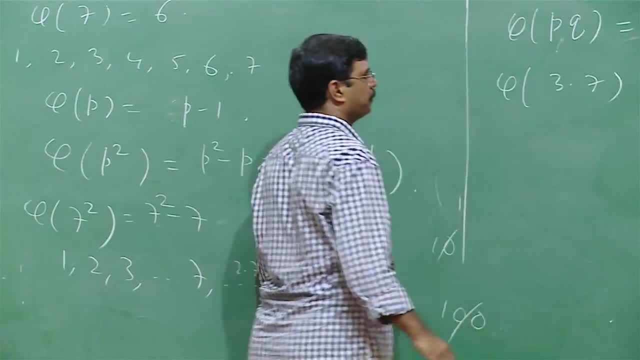 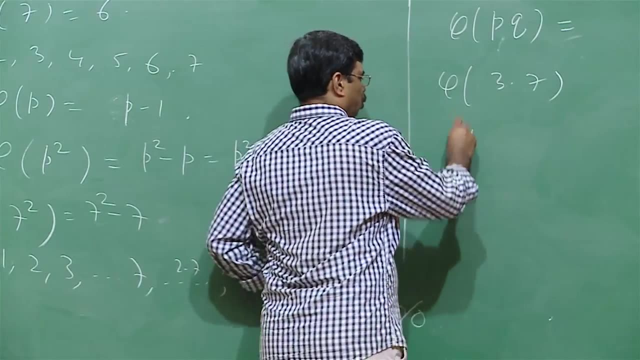 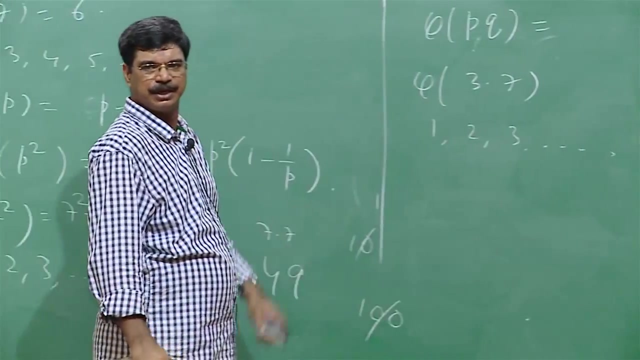 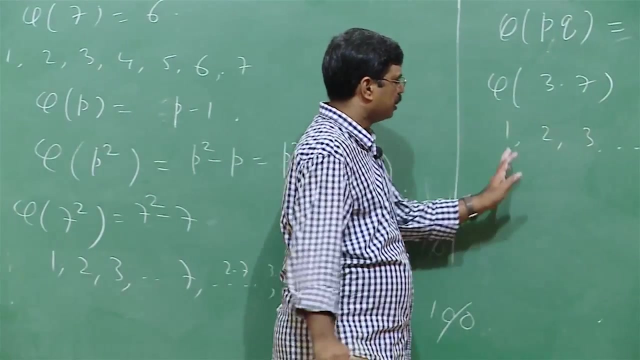 us say 3 into 7.. This is into, not point 3 into 7.. So 1,, 2,, 3, up to 3 into 7.. From here, first remove all the numbers which are not co-prime. okay, The numbers which are not co-prime are should. 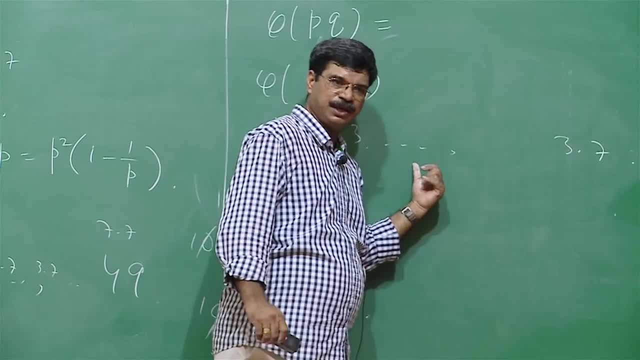 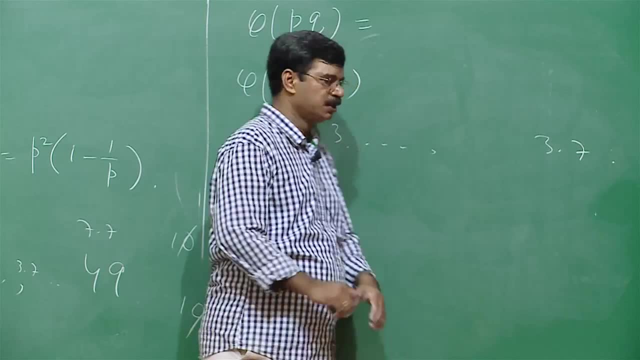 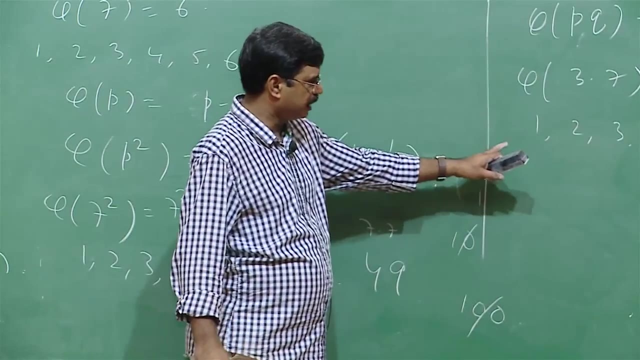 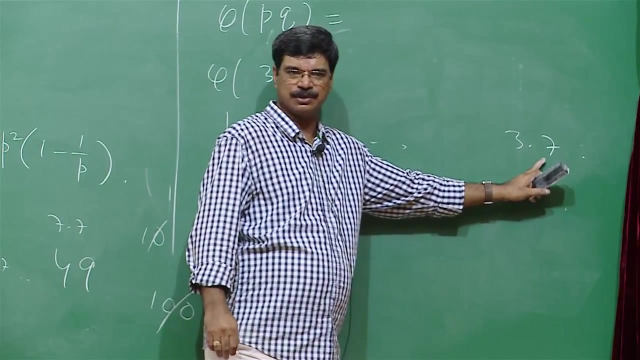 have a common factor: 3 or 7,. okay, Those are the only numbers which are not co-prime. So how many numbers are there which have multiples? 3? 3 is there? 2 times 3 is there? 3 times 3 is there? 7 times 3 is there? 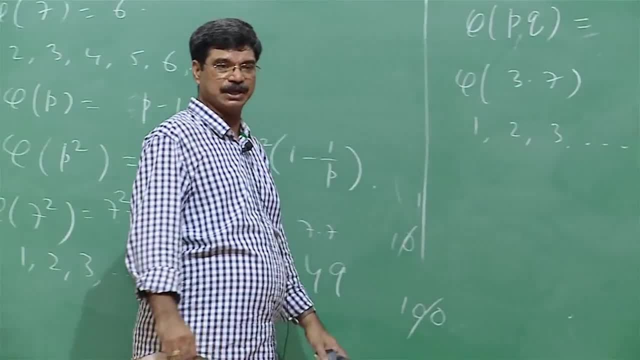 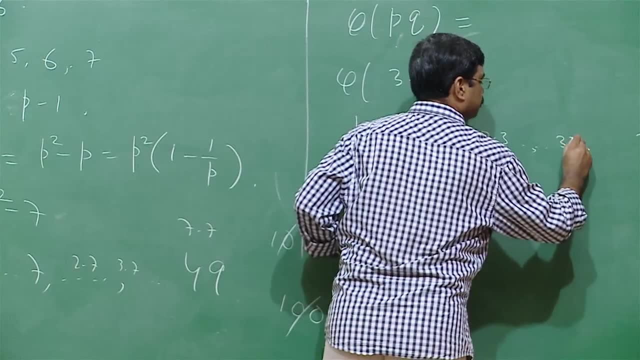 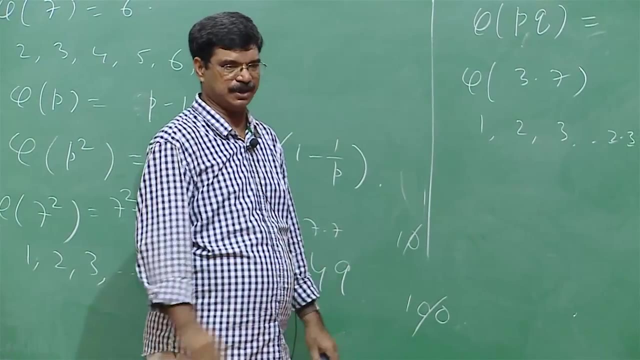 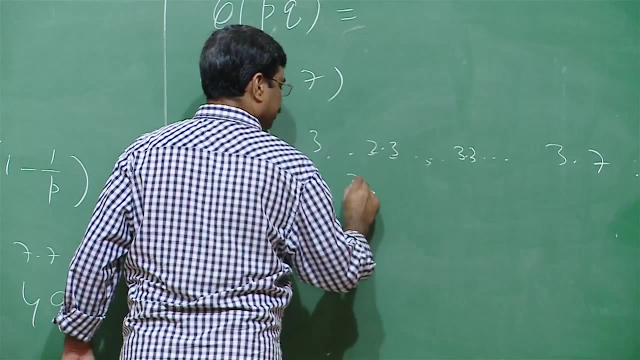 So you remove all of them, not 11 of them, 7 of them all. So 3, 2 times 3, 3 times 3, 7.. 1. 3 times 7, and then you remove those which are multiples of 7, okay, So 7 is there. 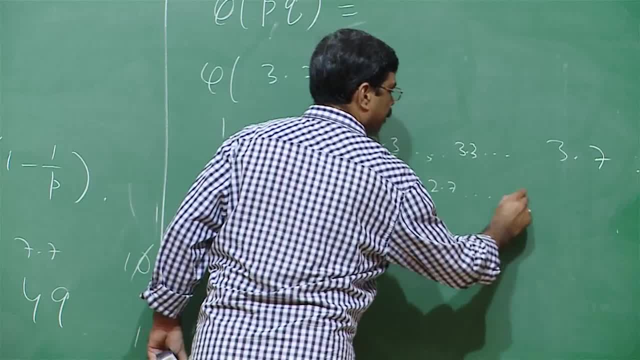 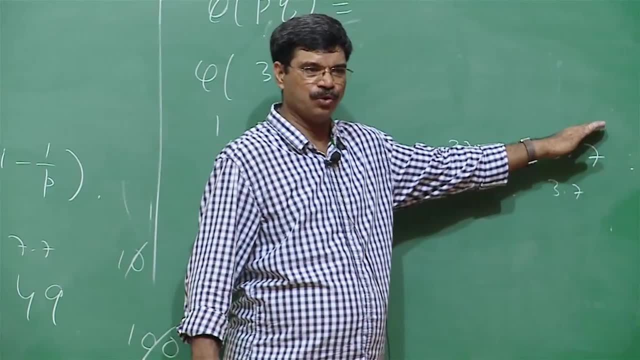 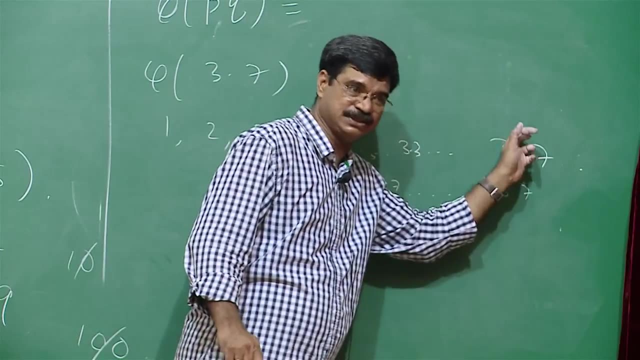 1 times 7,, 2 times 7,, 3 times 7.. But you see we have removed 3 times 7 in the first go. We cannot remove it again. So we have to add this one Once, because while removing this, we are removing twice. So add this. So therefore, 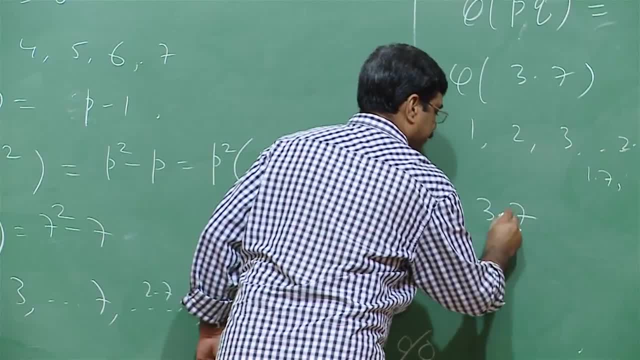 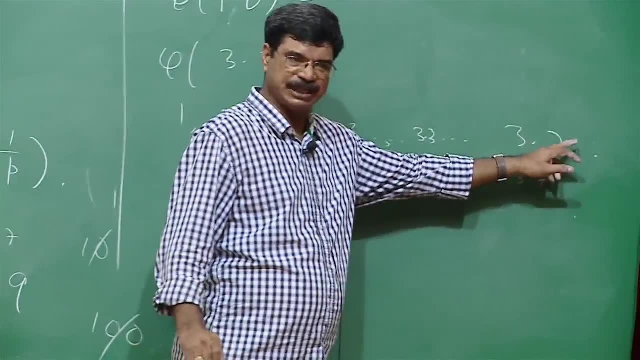 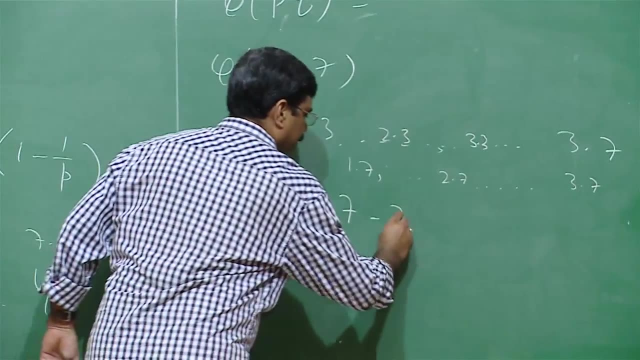 what we are doing. total number is 3, 3 into 7.. These many numbers are there minus the multiples of 3 or 7.. The multiples of 7 are 3 and since we have removed this number twice, we have added 1.. Okay. 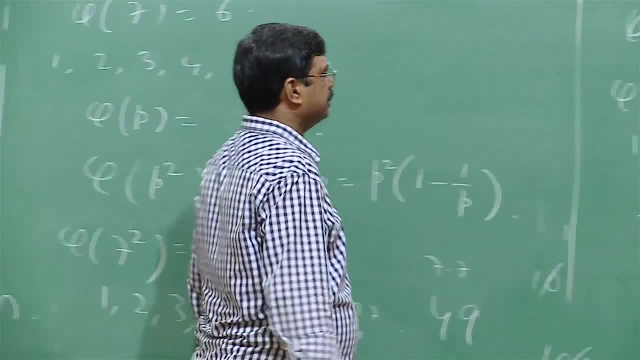 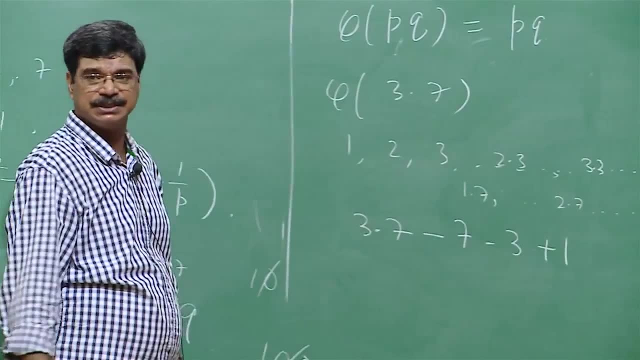 1., 2., 3., 4., 5., 6., 7., 7., 8., 9. 10.. If we remove this, what will we get? 5. 0., 6.. 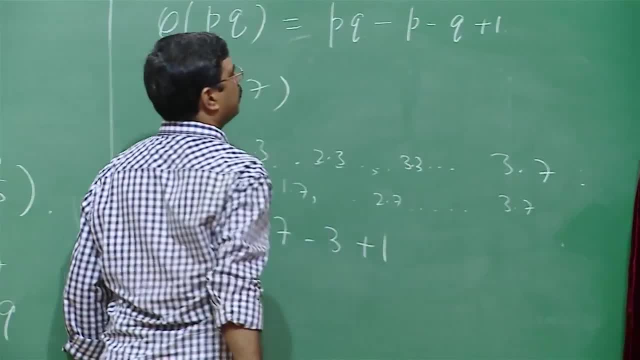 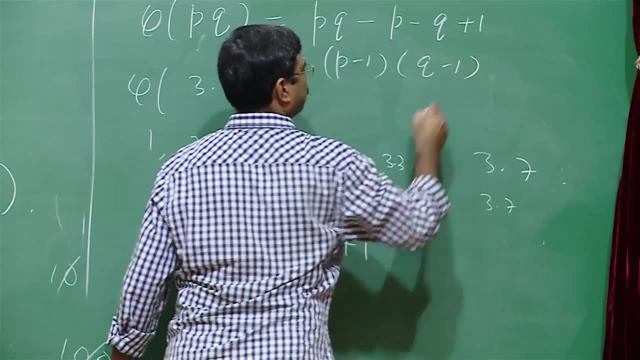 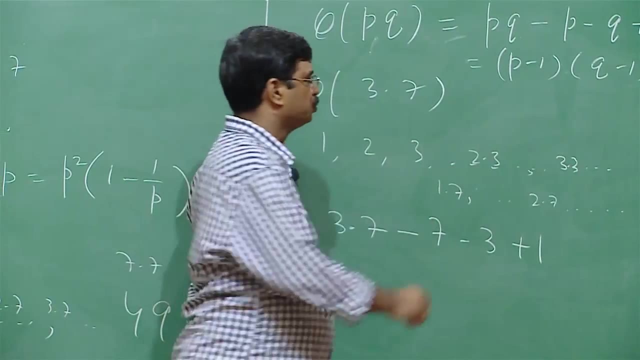 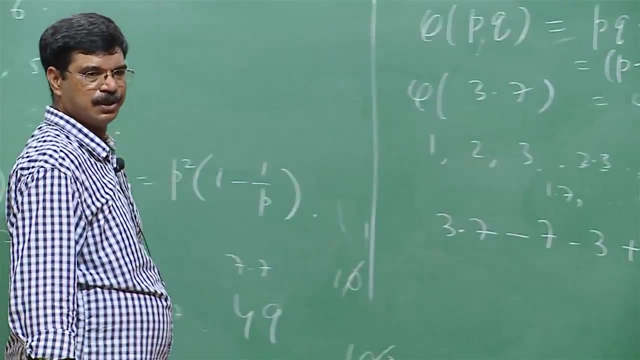 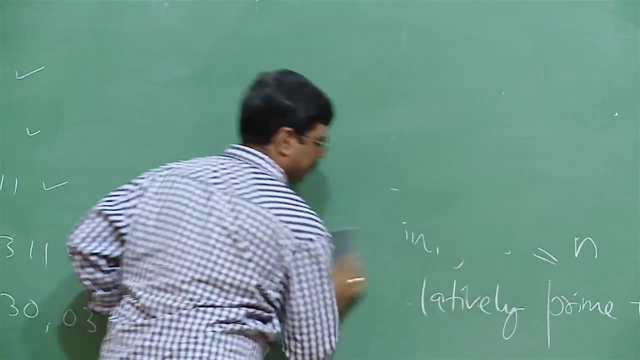 5., 8., 9., 11., 9., 12., 13., 11., 14., 15., 16., 17., 18., 19., 20., 21.. is phi of q. So this is phi of p, phi of q. ok, In general, 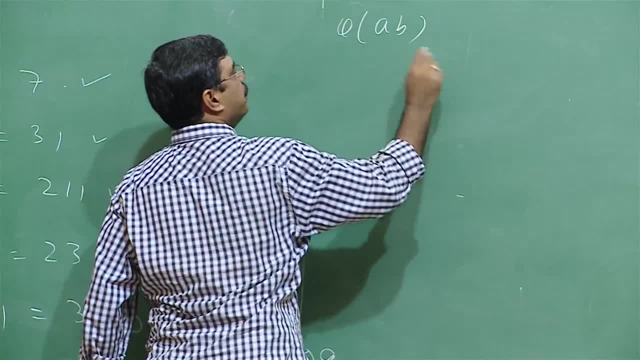 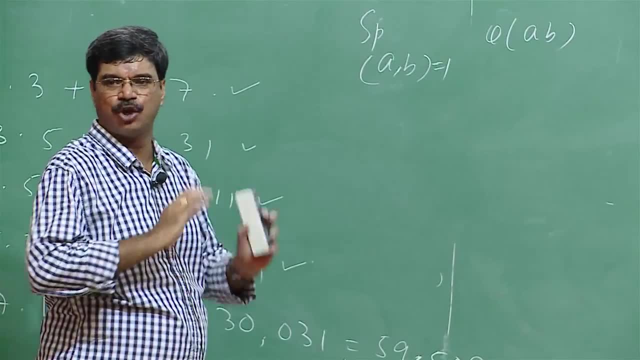 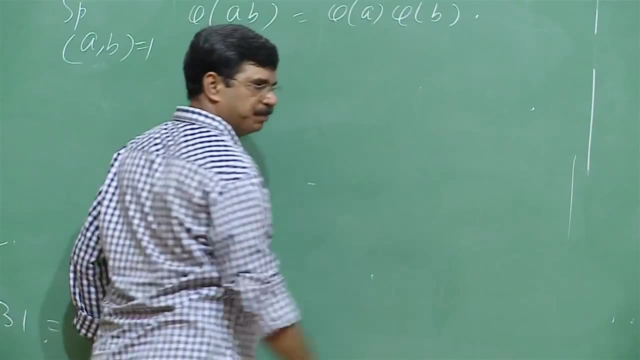 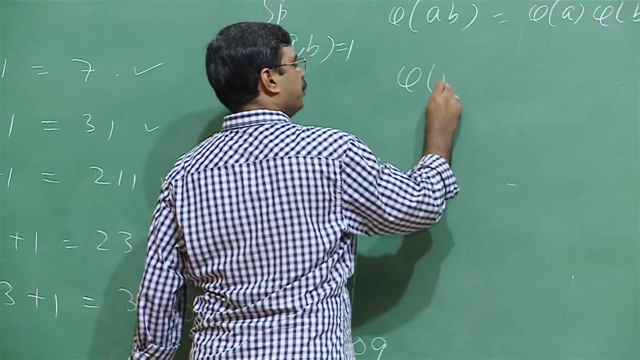 so phi of a- b? suppose a and b are co prime. a and b do not have any common divisors, then phi of a, b is same as phi of a times phi of p. by the same argument, and for any integer n, phi of n, Suppose n. 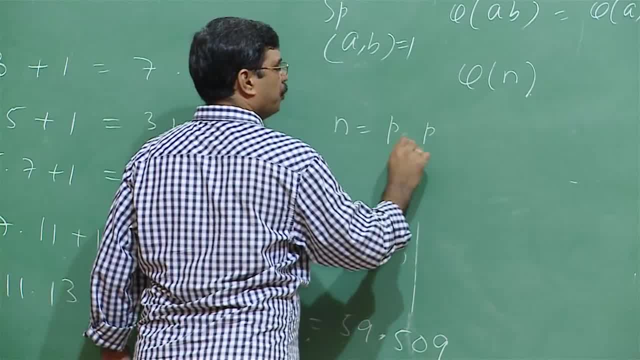 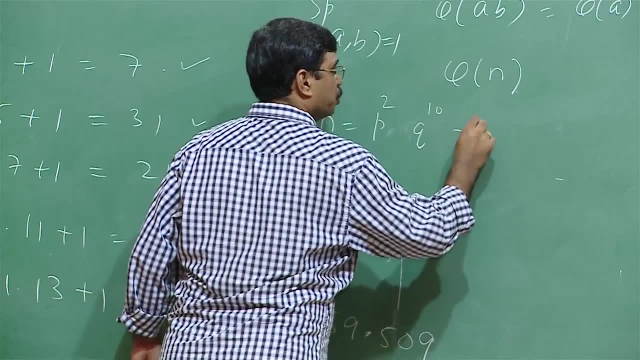 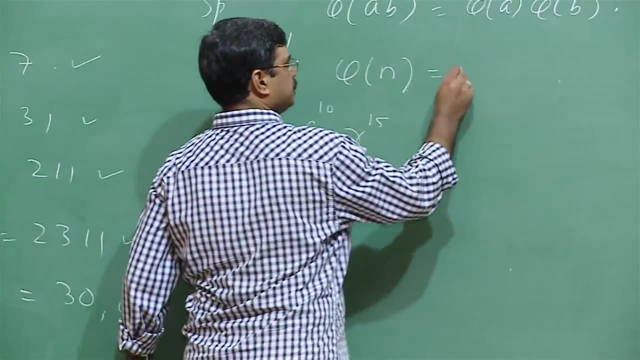 n is, n is p, 1, p, q, r, something like that p square, q to the power 10 and r to the power 15, something like this: n is a number. having this kind of thing, then phi of n is same as phi of p square. 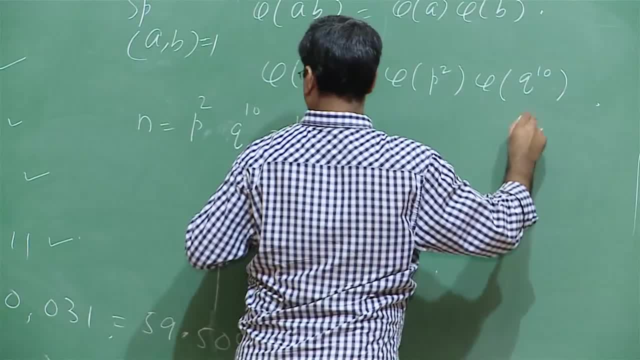 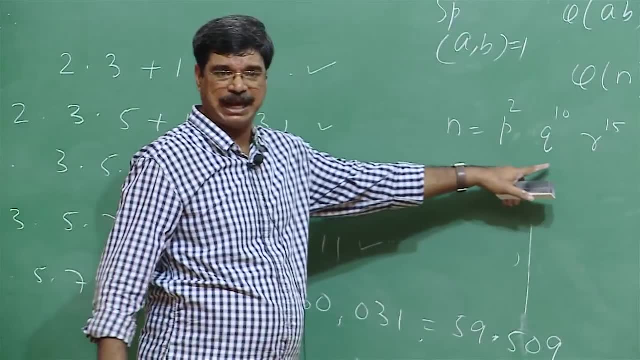 phi of q to the power 10 and phi of r to the power 15.. Then phi of r to the power 10, as well as phi of p square, which is same as phi of q to the power 15.. Where p, q, r are primes. 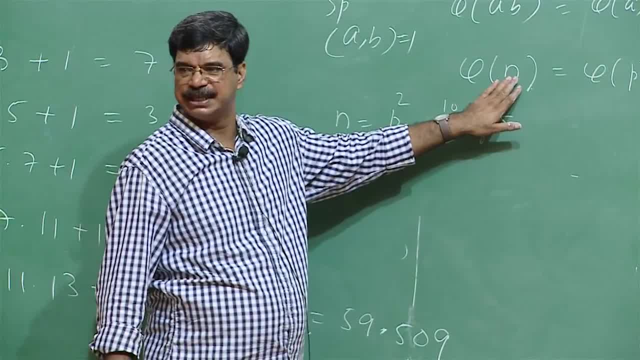 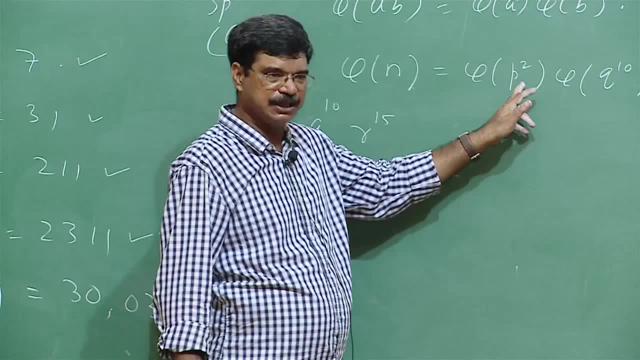 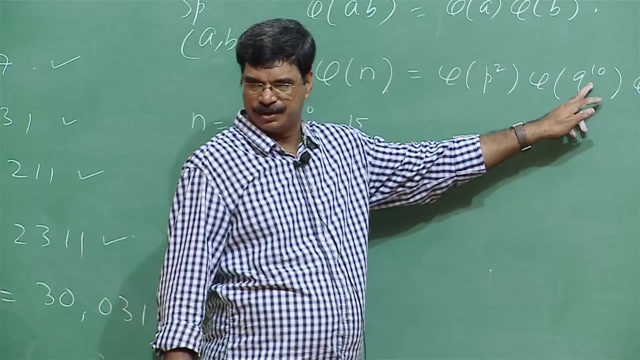 So finding how many numbers which are less than n co prime to n reduces the problem of finding how many numbers are there which are less than p square and co prime to p square times. how many are there less than q to the power? 10 relatively prime to 10 q to the power. 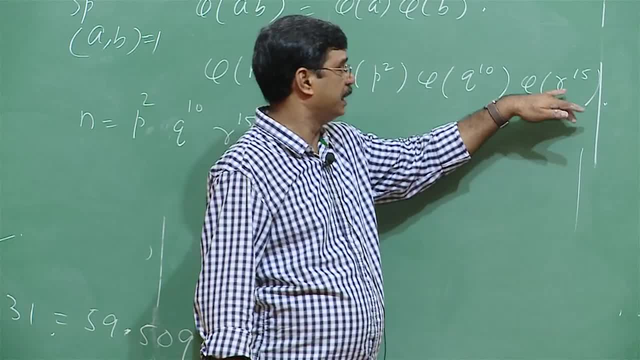 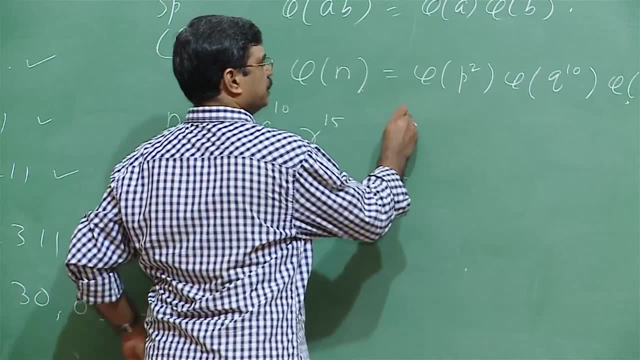 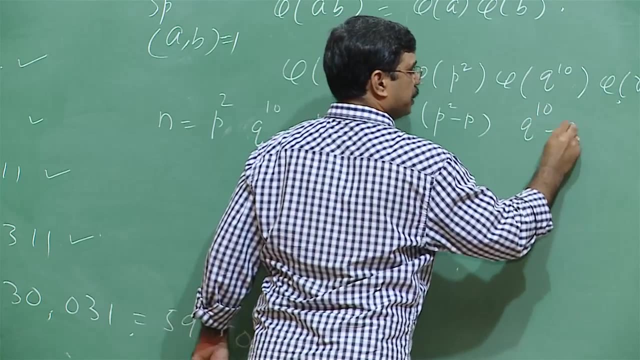 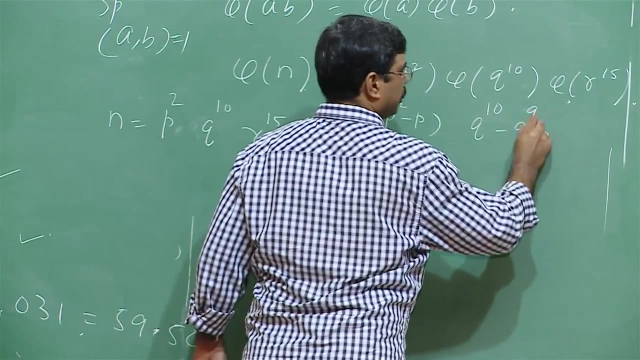 10.. What is this? q to the power, 15. q to the power, 10. q to the power, 15. 15 and relatively prime to 15, and for this we know that this is p square minus p. for this we know that is q to the power, 10 minus q to the power. how much? 9 for this. r to the 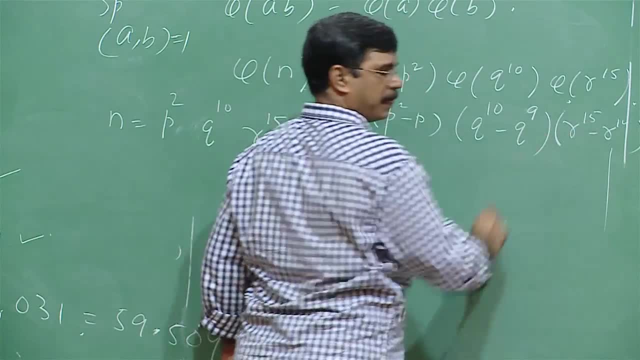 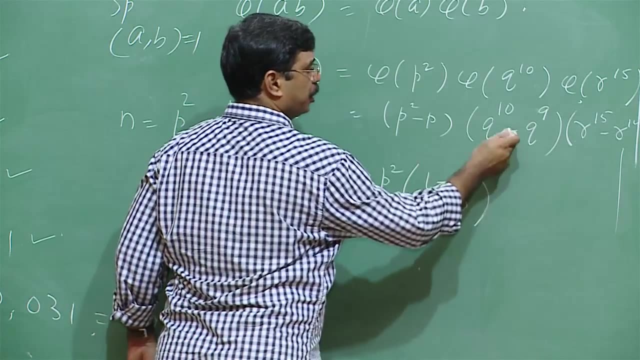 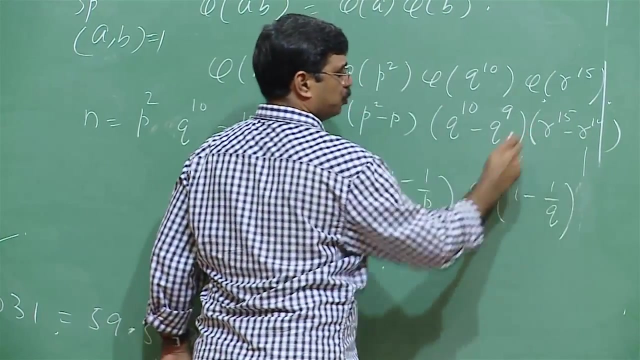 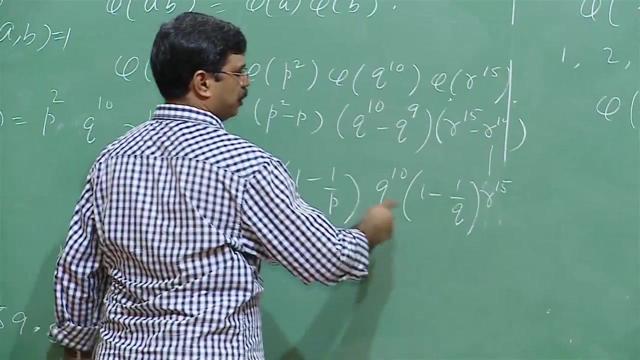 power 15 minus. if you take p, square, common here it is 1 minus 1 by p. if you take q to the power 10, common here this is 1 minus 1 by q. r to the power 15, if you so, this is 1. 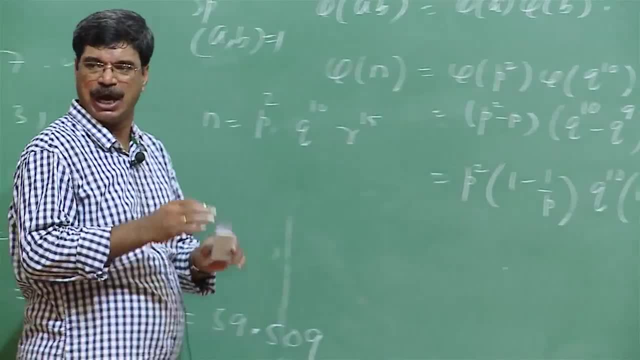 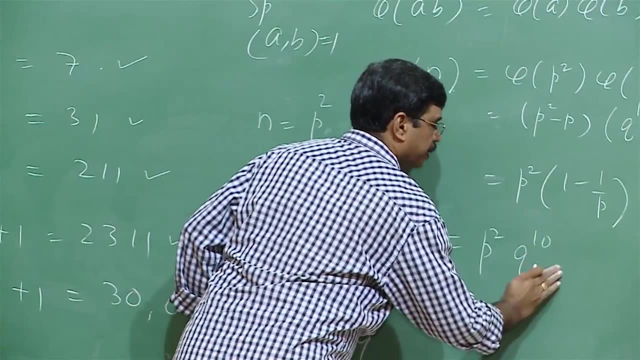 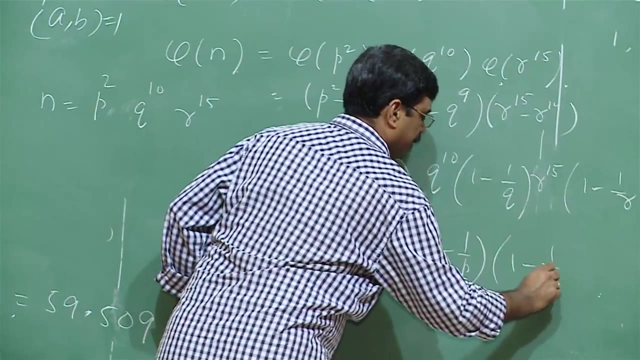 minus 1 by r. Where pq, Where pq, r are the prime divisors of n. therefore, this is p square q to the power 10 and r to the power 15 times 1 minus 1 by p, 1 minus 1 by q, 1 minus 1 by r. p square q to the power 10. 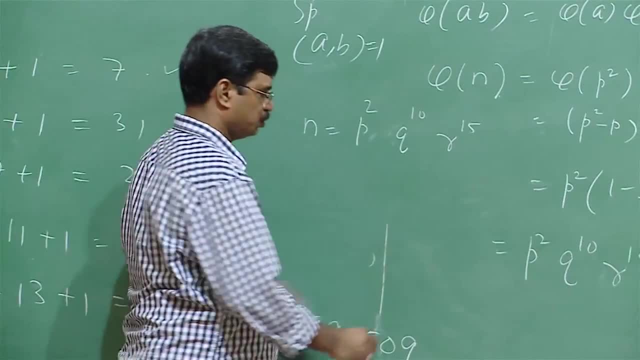 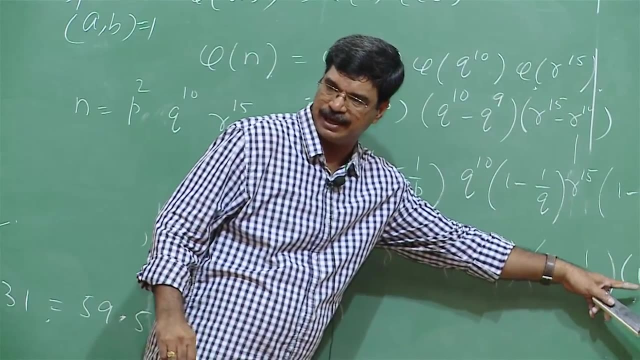 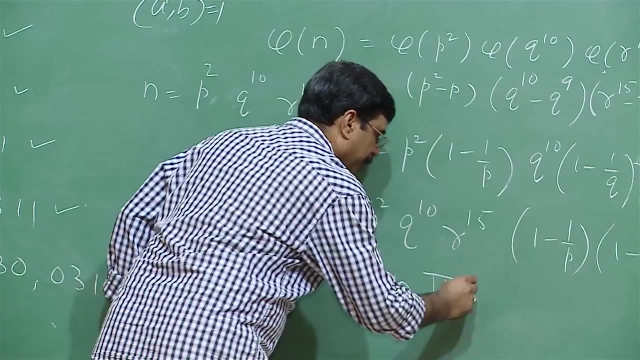 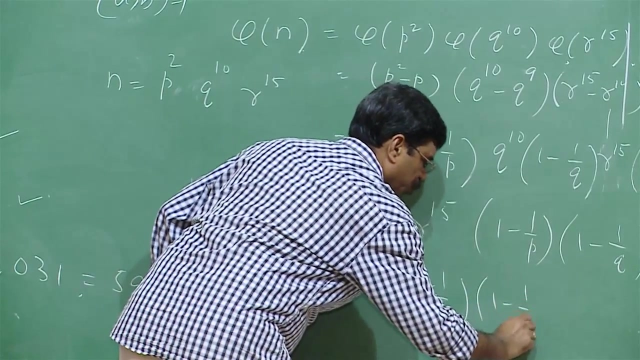 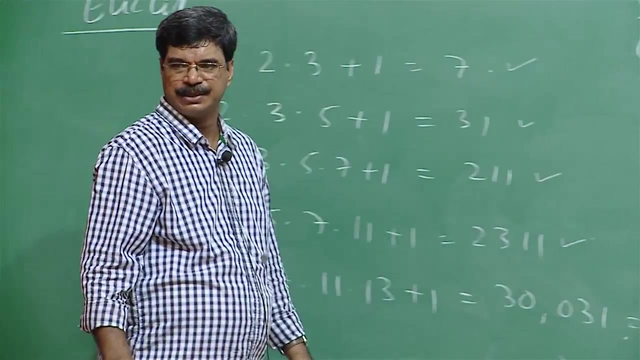 r to the power 15 is nothing but our n. so this is n. into what are these numbers? these are the prime divisors of, So we can write it as this is the notation for product, and let us not complicate the matters: 1 minus 1 by p, 1 minus 1 by q, 1 minus 1 by r. therefore, if I want to know how many, 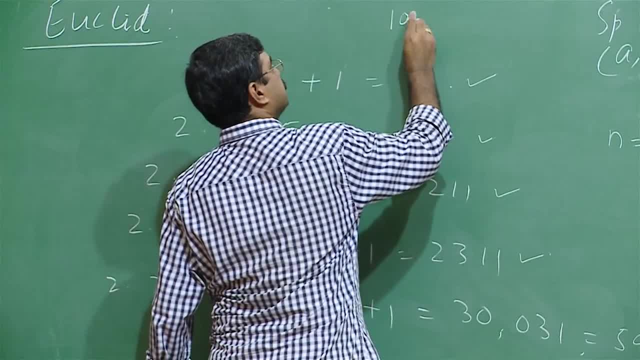 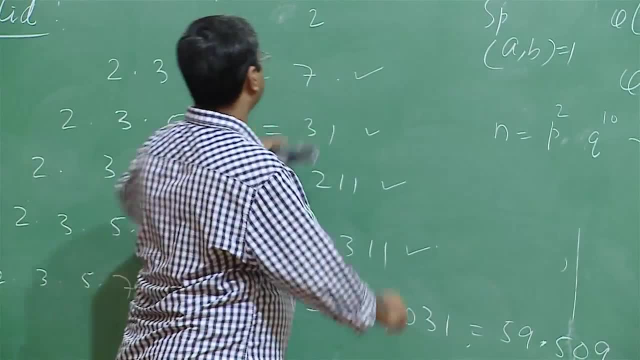 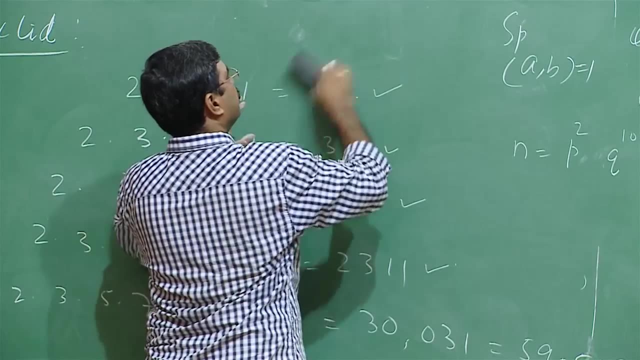 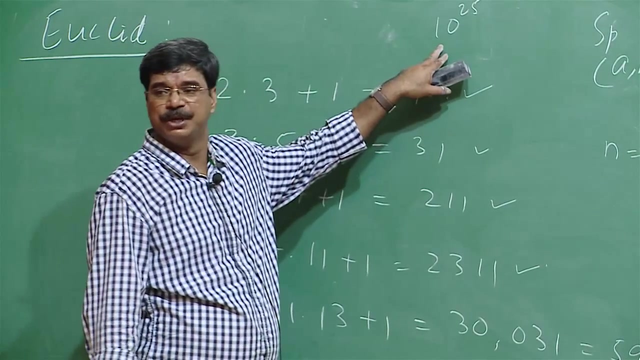 numbers are there which are co prime to. let us say 2 to the power 10 and then 5 to the power. or if I said 10 to the power, 25, something like this, how many number? this is a large number. how many numbers are there which are? 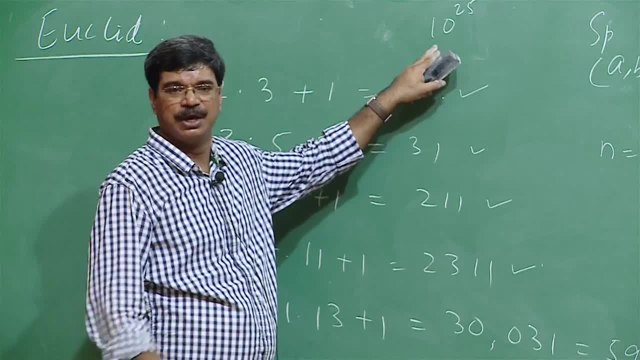 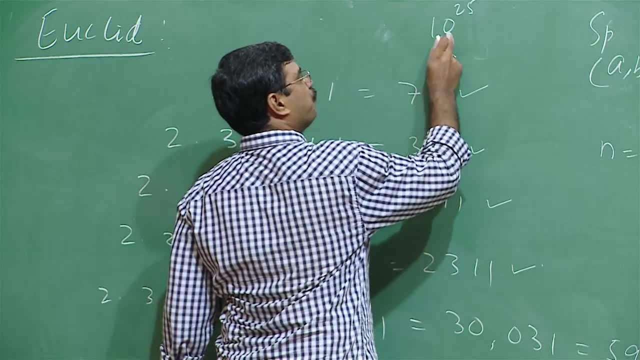 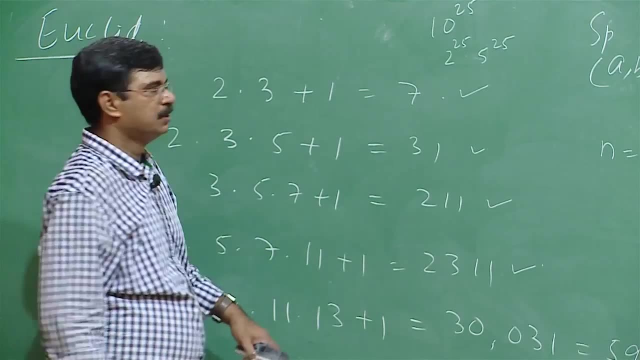 less than 10 to the power 25 and relatively prime to 25. counting by hand is difficult, So this is This is what happens is 2 into 5. so 2 to the power 25 into 5 to the power 25. so now phi. 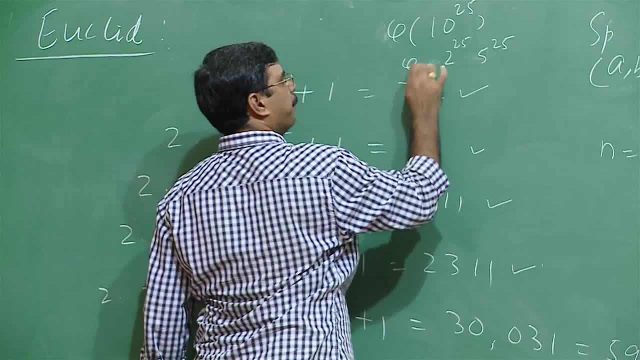 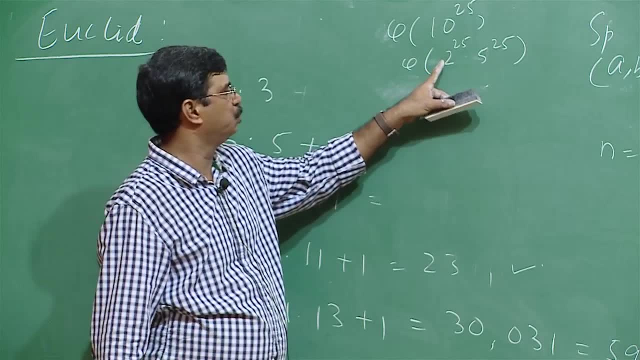 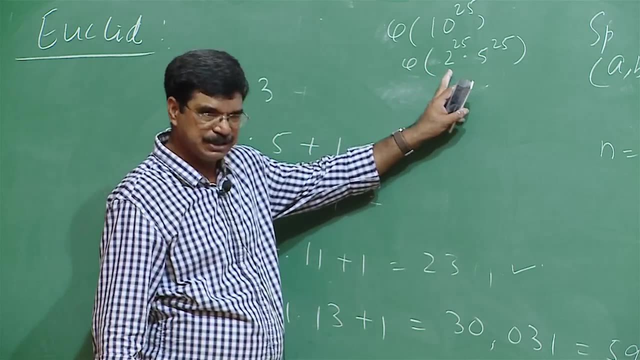 of this number is same as phi of this number, and we know phi of 2 into 5, 2 and 5 are relatively prime. So phi of this into this will be 2 into 5.. 2 and 5 are relatively prime. 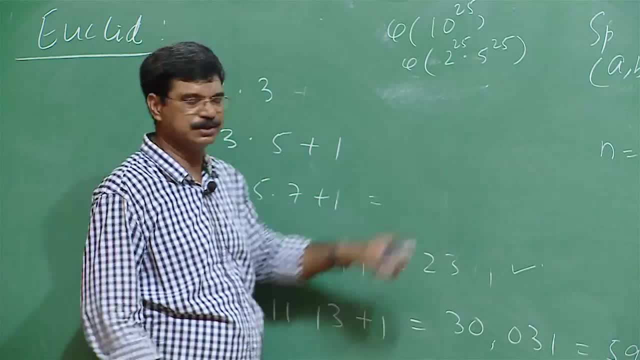 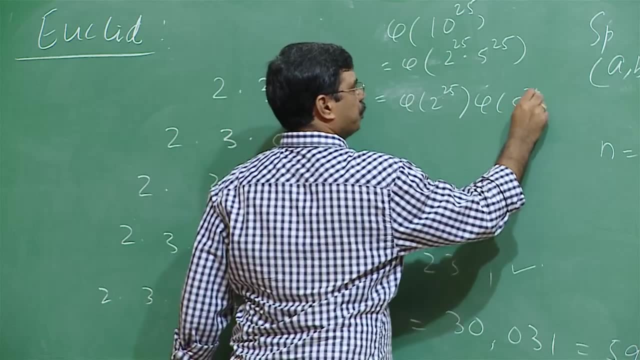 So phi of 2 and 5 are relatively or 3, and therefore this is phi of 2 to the power 25 into phi of 5 to the power 25.. But we know what is this much and what is this one. 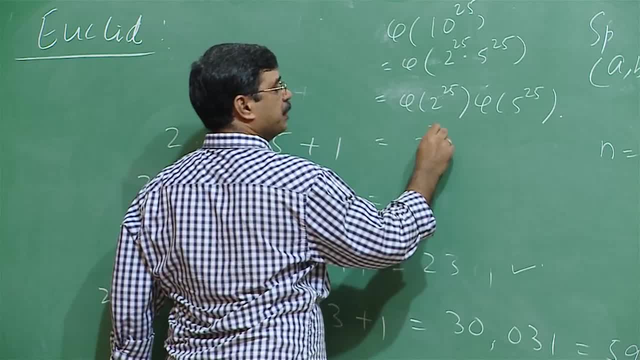 So this is 2 to the power 25.. So you can write it as by using that 10 to the power 25, 1 minus 1 by 2, 1 minus 1 by 25.. So this is the product or derivative. 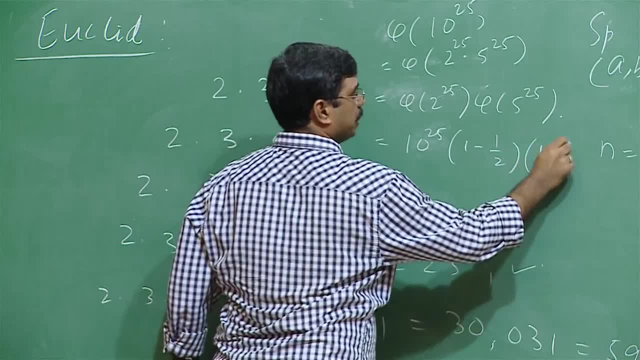 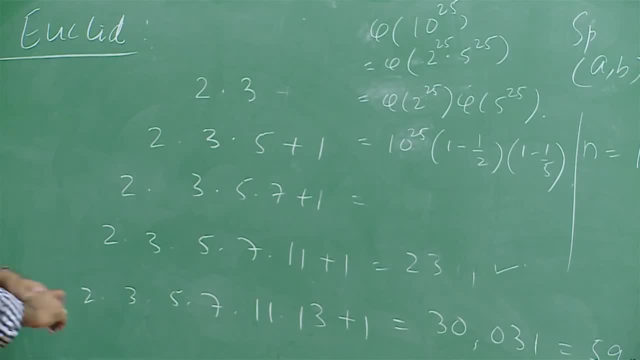 O n nahi hua. Yes, sir, despatch 1 minus 5.. One say 1 by this, much ok. or you can say that 2 to the power 25 minus 2 to the power 24 into 5 to. 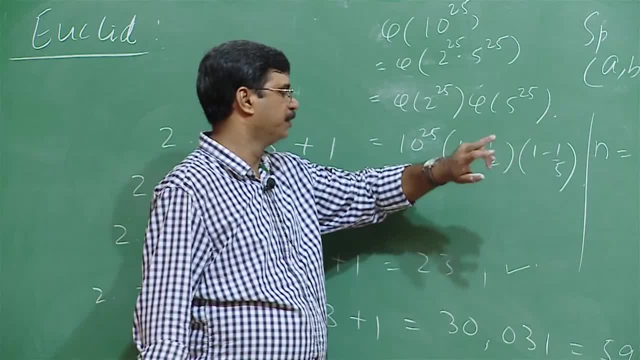 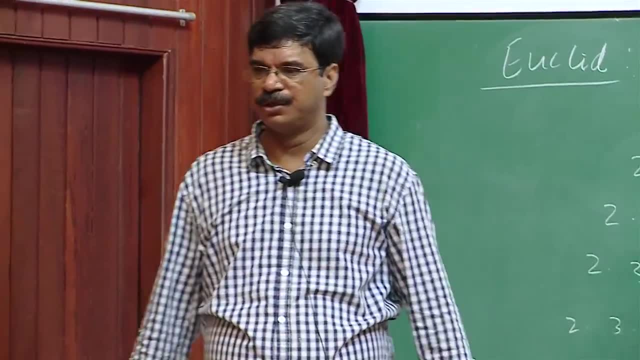 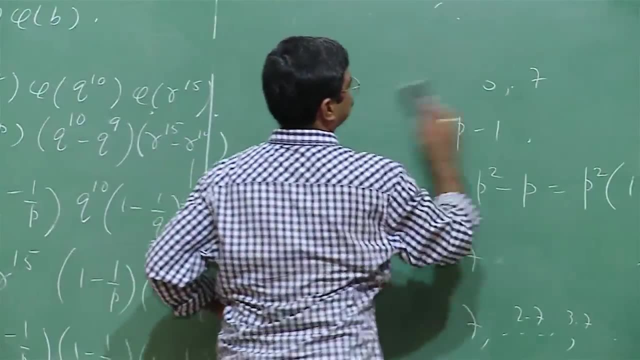 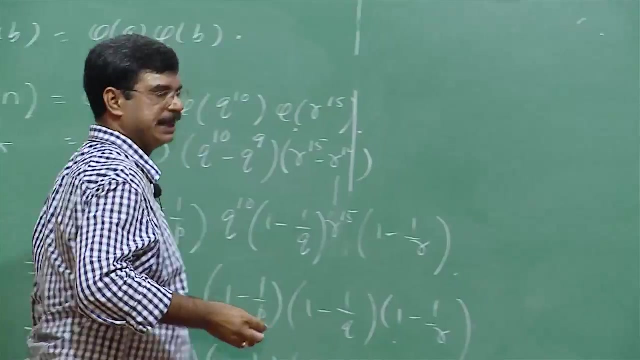 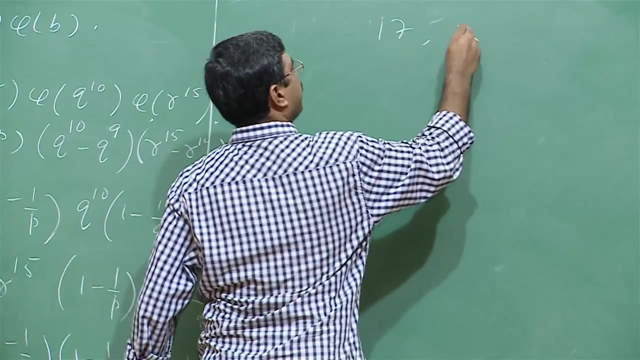 the power 25 minus 5 to the power 20. ok, So these are the thing. another thing I wanted to introduce was notation of congruences. ok, just let me define that one and then we will pursue it tomorrow. We say that two numbers of congruent- 17 and. 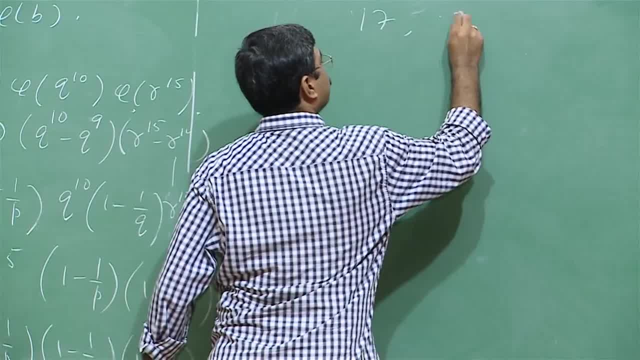 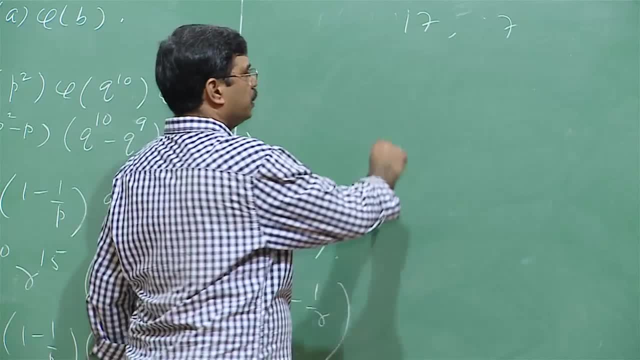 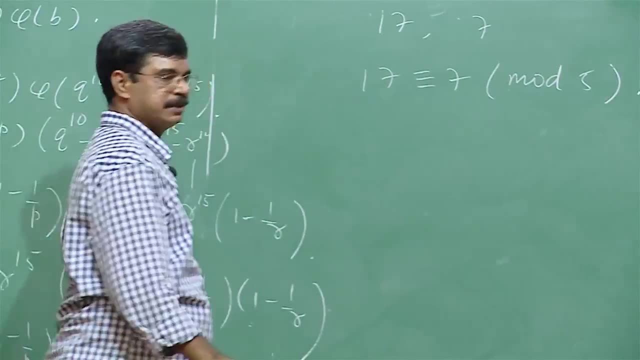 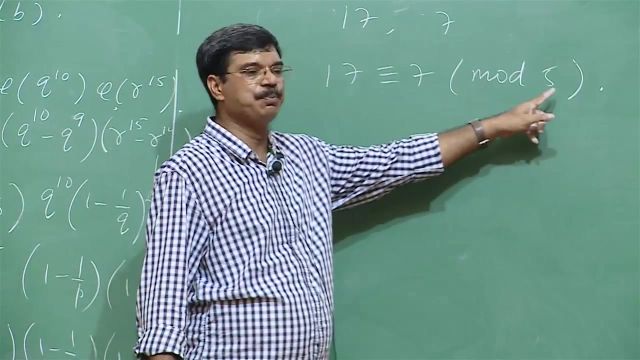 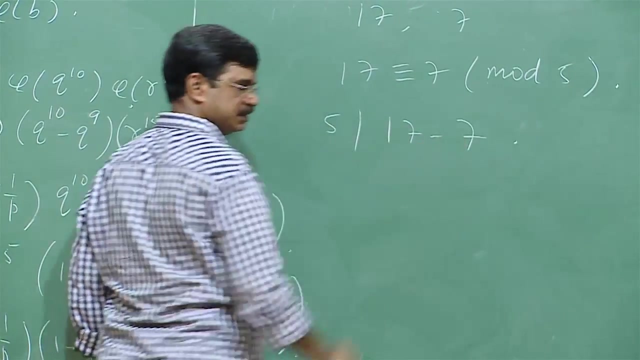 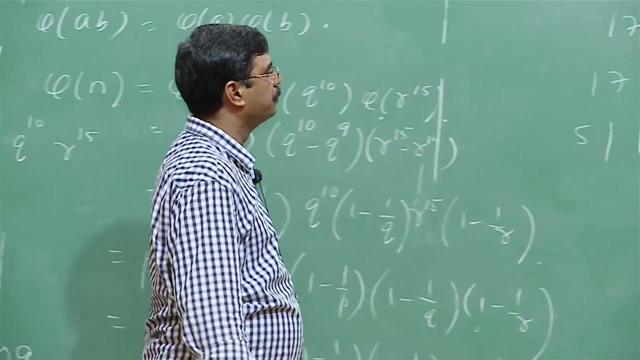 7 are congruent. modulo 5 means what That means. 17 minus 7 is a multiple of 5. this means 5 divides 17 minus 7. ok, So actually we need to write the 7 is less than 5.. 7 is. 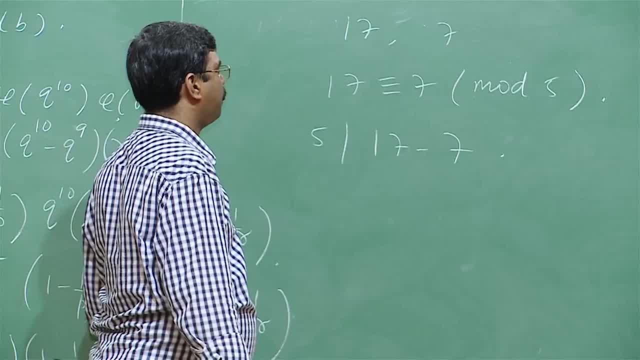 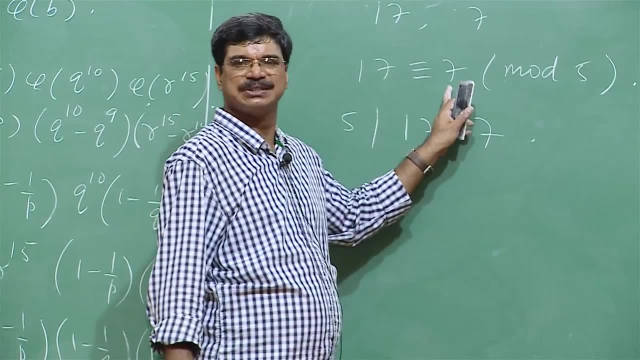 17. congruent modulo 17. congruent modulo 17. congruent modulo That number: 7 mod 5 instead of the d. d to the right that 7 has a less than 5.. Does not matter, 7 and 2 are same modulo 5. ok when we say modulo. 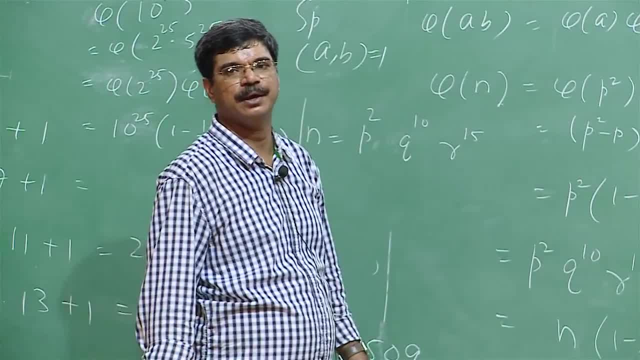 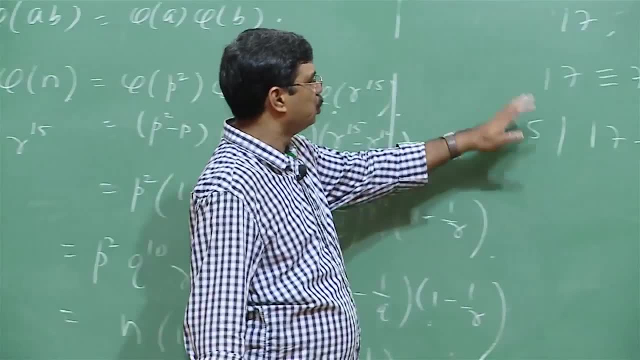 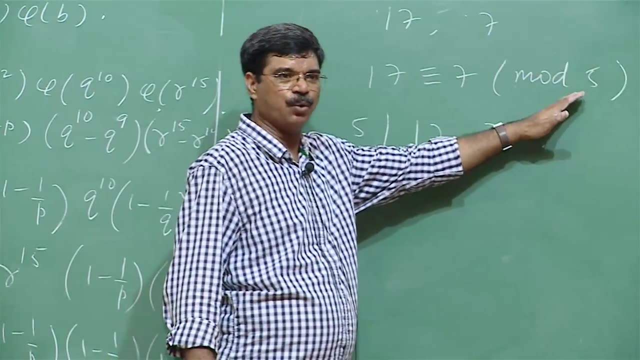 Because that is a residue. residue is always less than the device. I have not called residue so far. I have not used the term residue. ok, I am only introducing two numbers: a and b. by definition, a is congruent to b modulo m. What is the meaning of that? 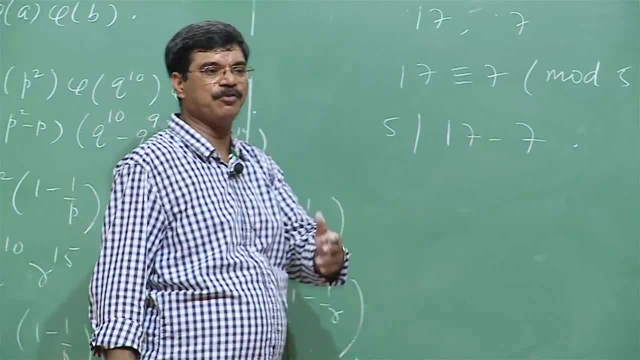 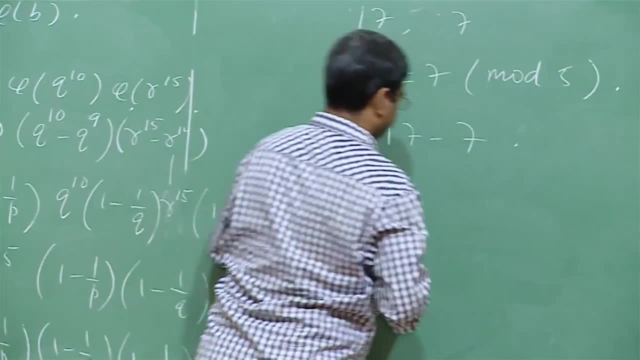 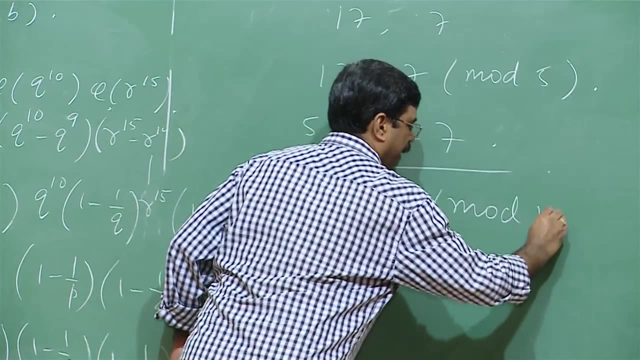 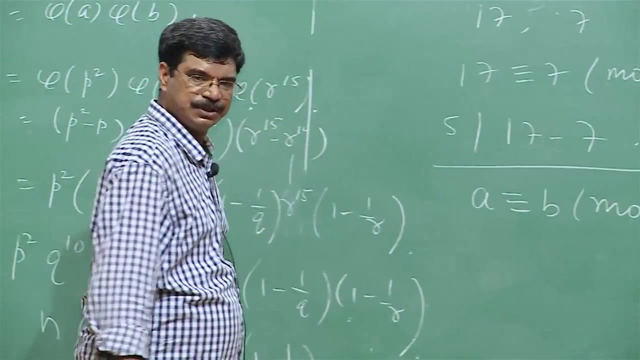 It means that a minus b is a multiple of m. that is all. Residues will come later. ok, So in general we write as: a is congruent to b modulo m, So we take m to be positive. ok, This means 17.. 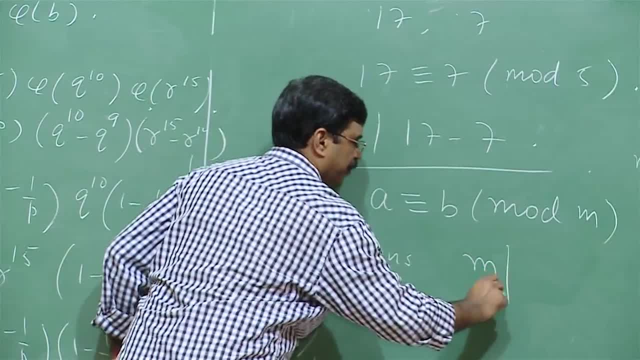 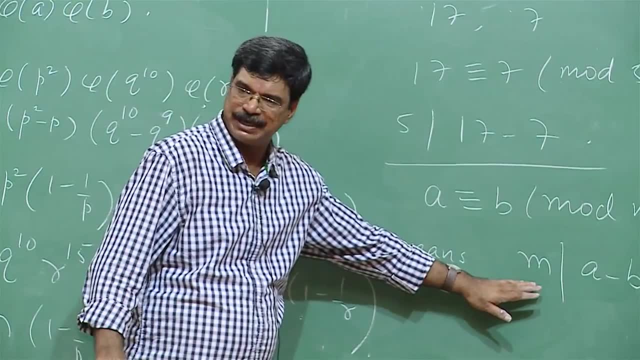 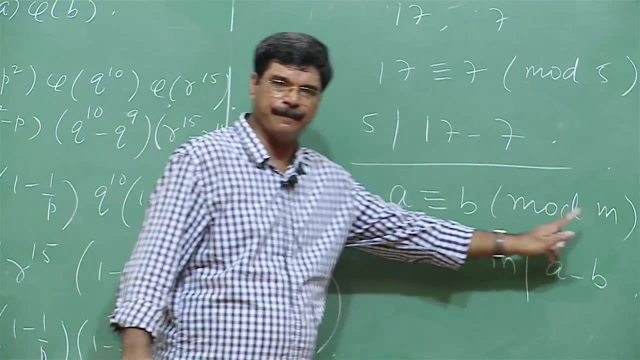 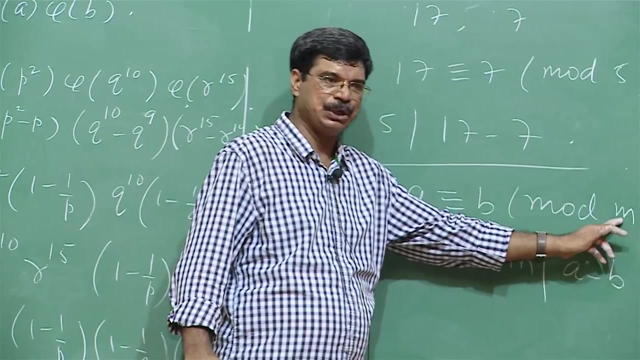 2. 4. 5. 0.. 1. M divides A minus b. Ok, Please pay attention. this also means that suppose you divide a by m, you will have a reminder r by division algorithm. you divide b by m. 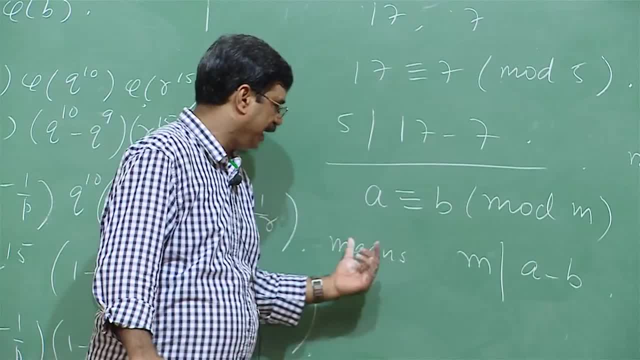 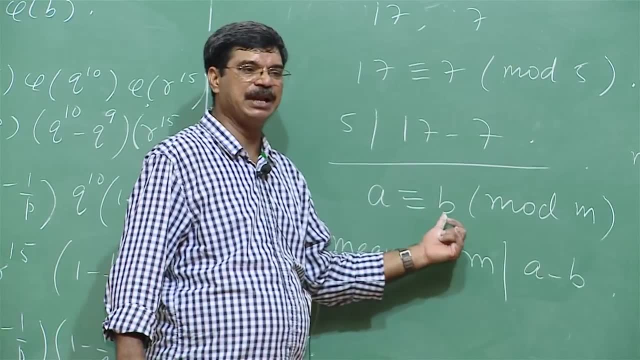 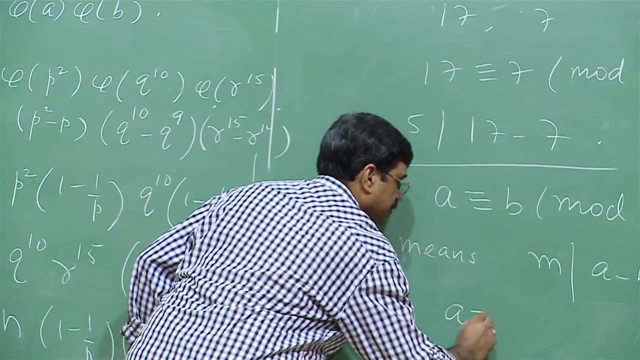 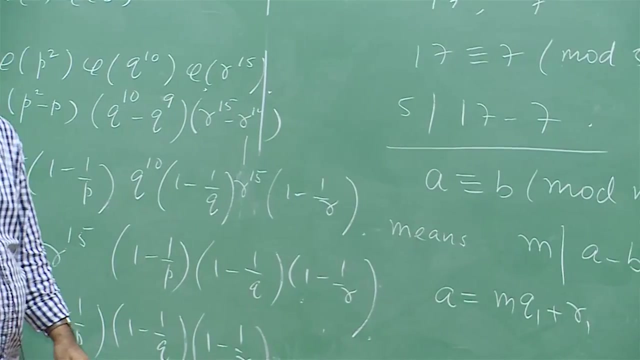 You will have a reminder r When a minus b- 0.1. is a multiple of M. that means both A and B will have the same reminder, so that reminders will get cancelled. So A is equal to M times Q1 plus R1, right by division algorithm. and. 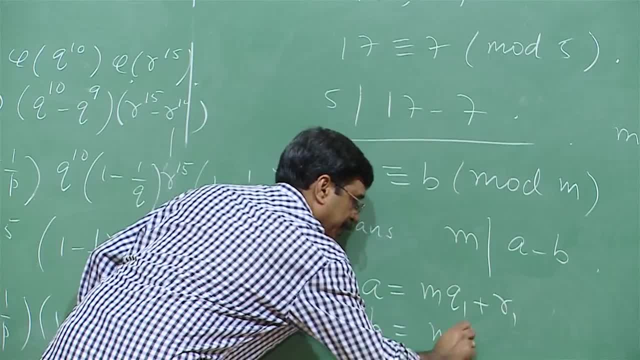 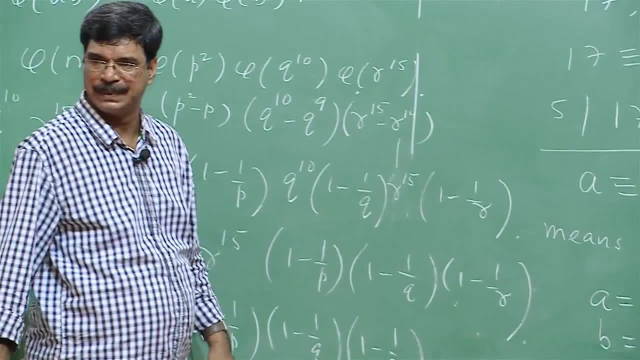 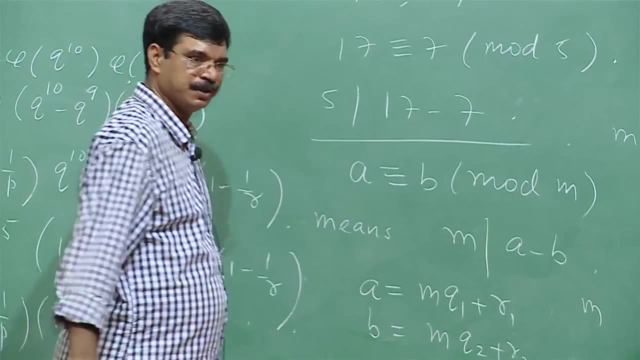 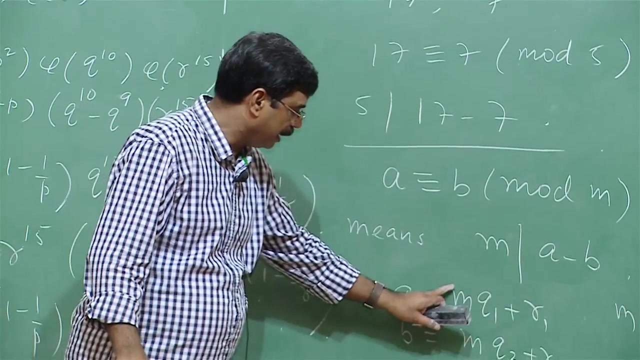 B is also when you divide it by M, Q2 plus R2, where R1 and R2 are less than M. okay, Now this statement: M divides A minus B. when is it possible? A minus B is M times Q1 minus Q2 plus R1 minus R2.. 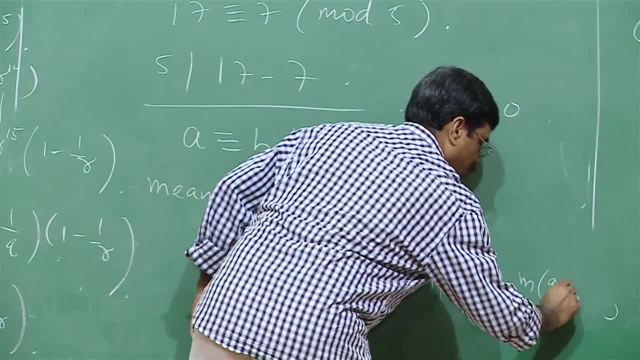 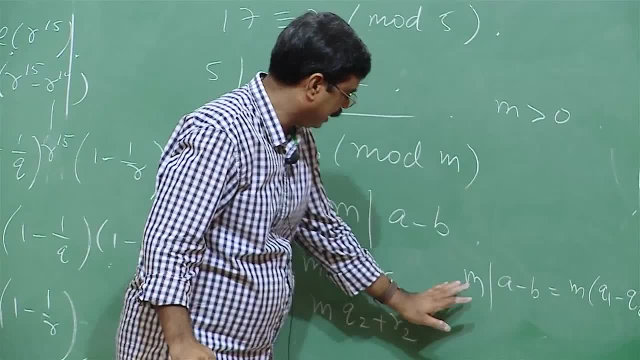 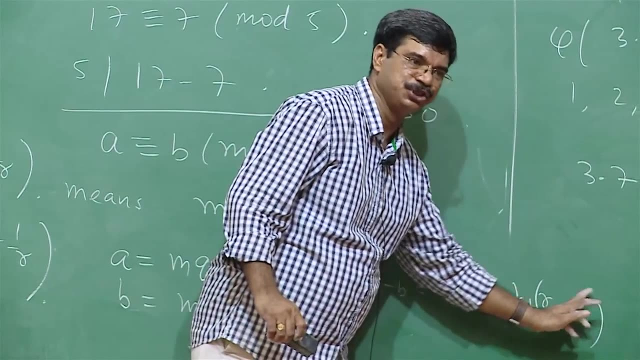 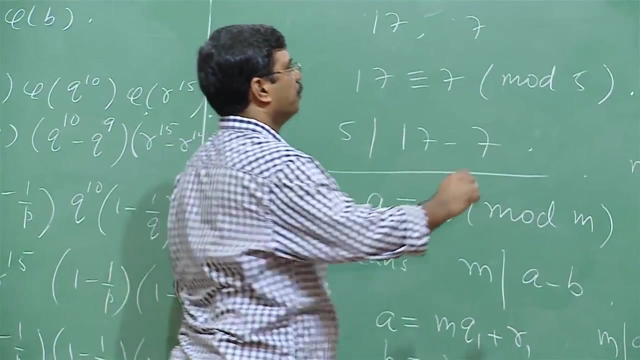 This is M times Q1 minus Q2, plus R1 minus R2.. So M divides, so this is already a multiple of M. therefore, this must be a multiple of M. that means there is 0, okay. R1 minus R2 must be 0, okay. So A is congruent to 0. modulo M means what? 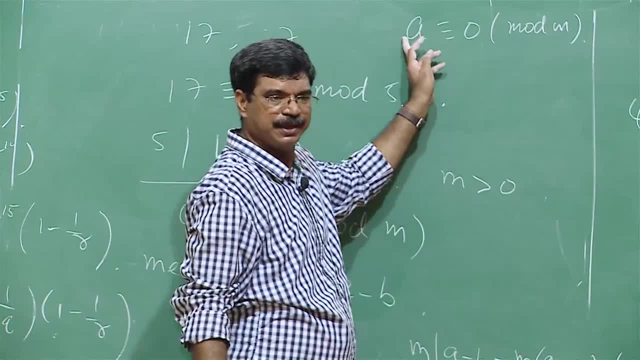 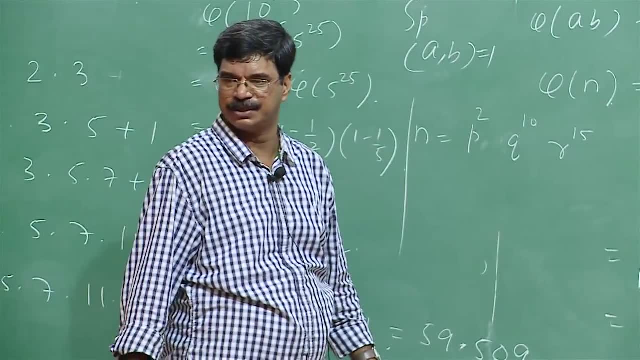 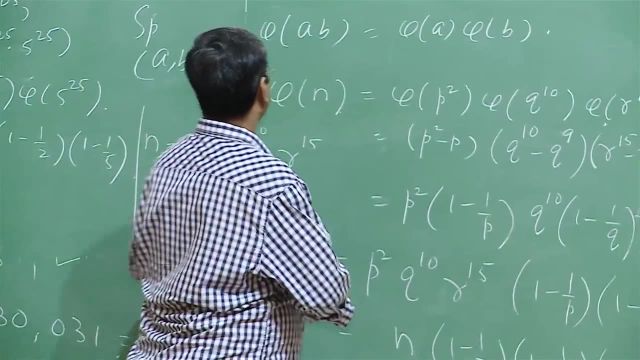 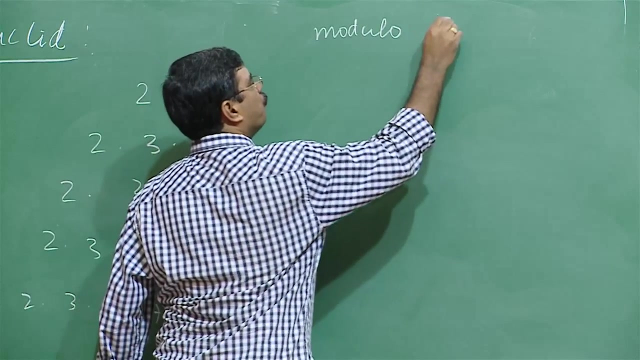 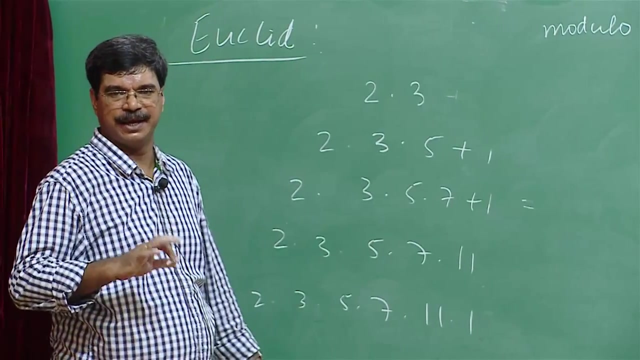 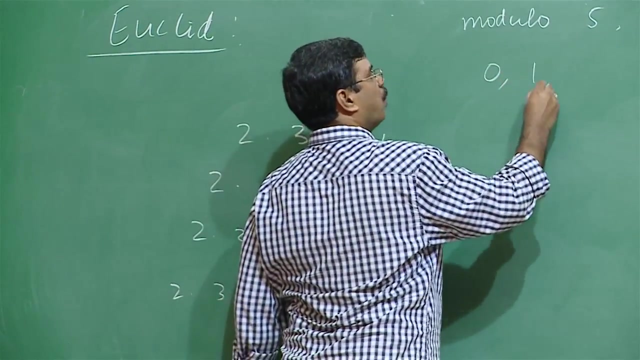 0. That means M divides A. okay, So two numbers are congruent, means they have the same reminders. and yeah, what you are saying residues is, when you look at these numbers, modulo 5, 5 is the modulus. okay, Take any integer N. when you divide it by 5, the possible reminders are 0, 1, 2, 3, 4, because 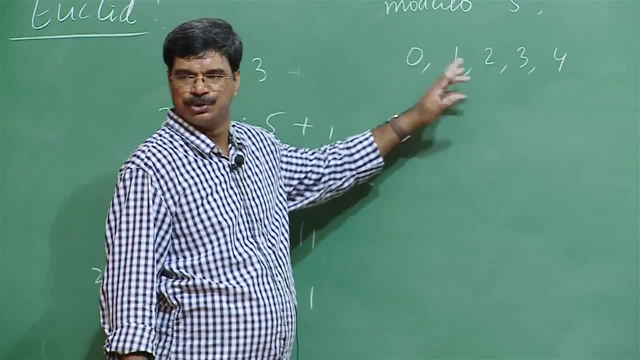 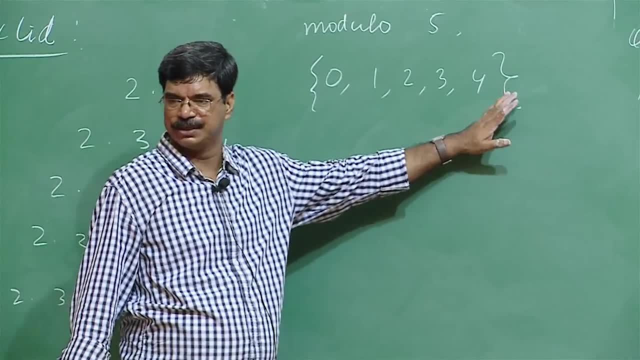 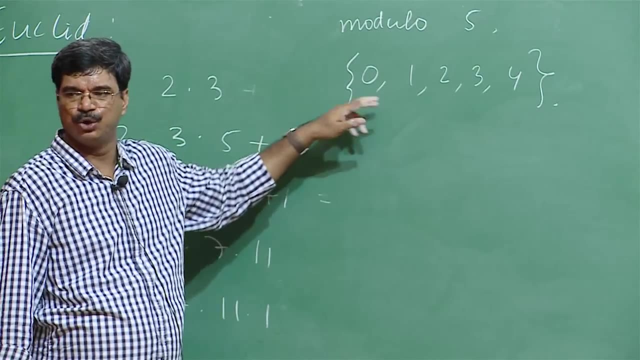 reminder is 5 means again it is 0. So all the reminders belong to this set. So modulo M- every integer is associated with this set. Okay, Okay, Okay. So modulo M- every integer is congruent to 1 of these elements. 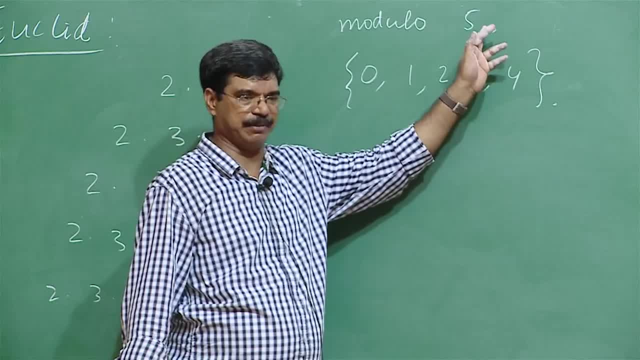 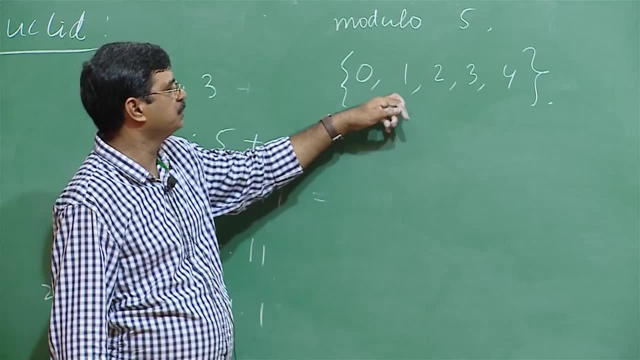 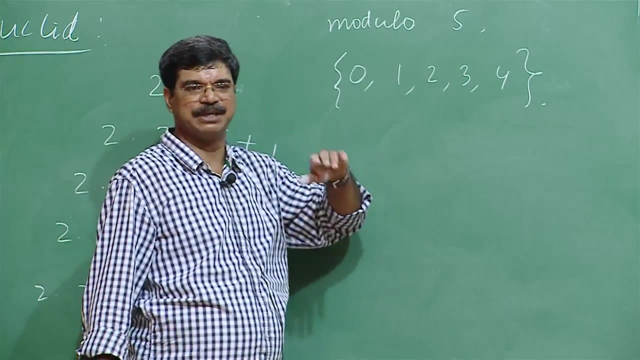 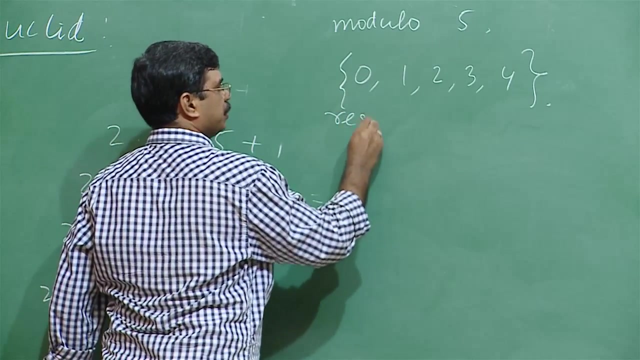 These are called the residues modulo M, modulo 5.. So these are the residues modulo 5. okay, and out of this, those residues which are co-prime to 5 have a special name. they are called reduced residues. okay, So these are the residues and the another one is reduced residues. 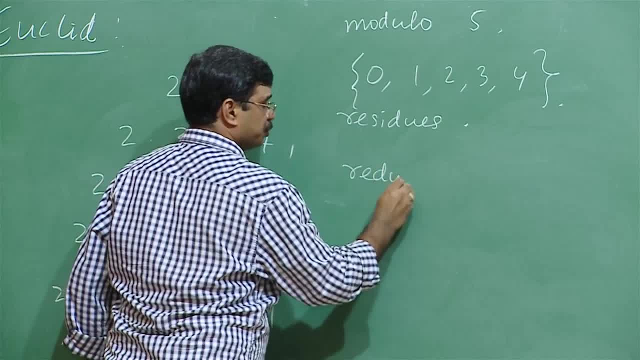 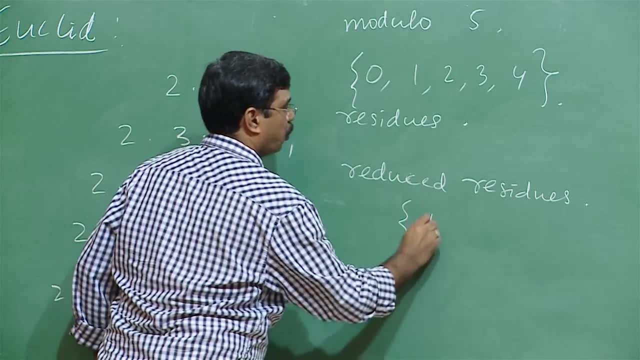 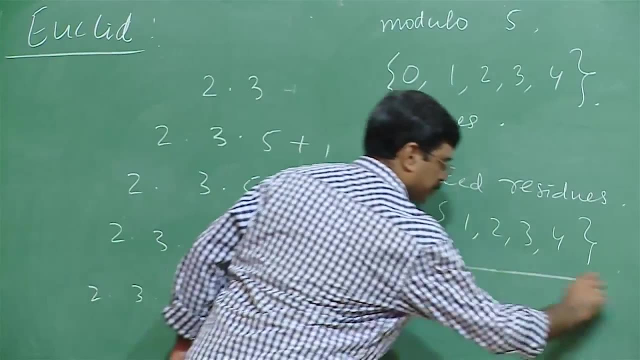 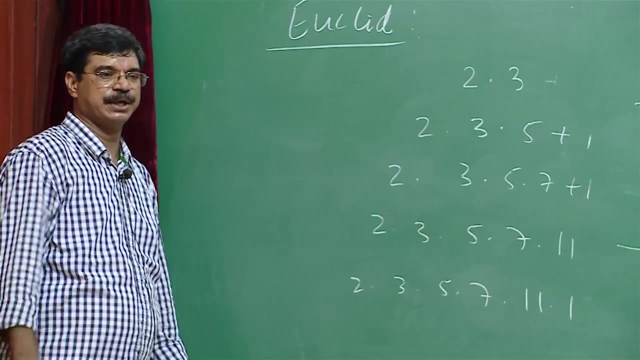 Okay, Okay. Reduced residues means these are 1,, 2,, 3,, 4.. One more example, and then we will stop. M is equal to 8. let us take modulus is 8.. What are all the residues? 0,, 1,, 2,, 3,, 4,, 5,, 6,, 7..